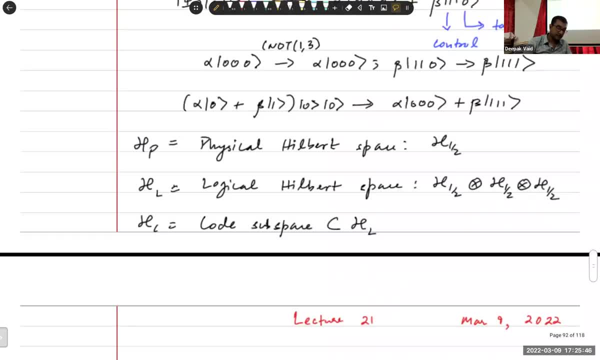 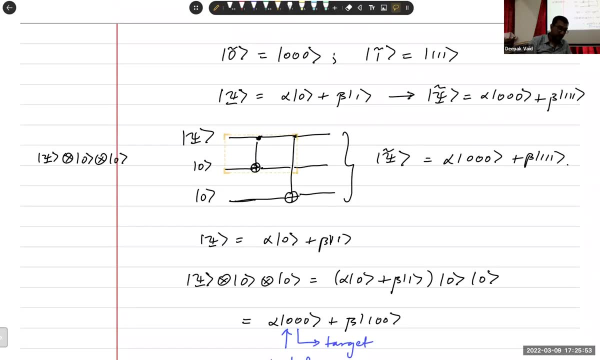 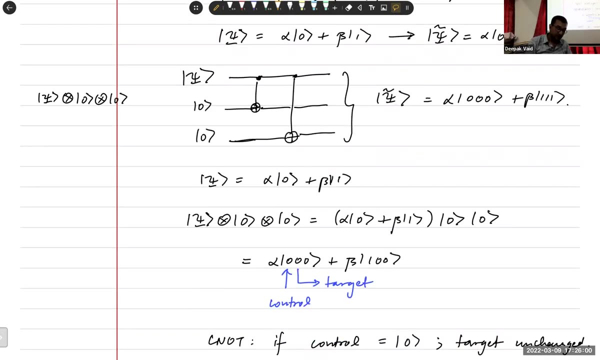 And, as I explained, if you take this circuit right And you apply first CNOT gate, so you write psi as alpha zero plus beta one, you apply the first CNOT gate- what happens? You start with this state, you apply the first CNOT gate. 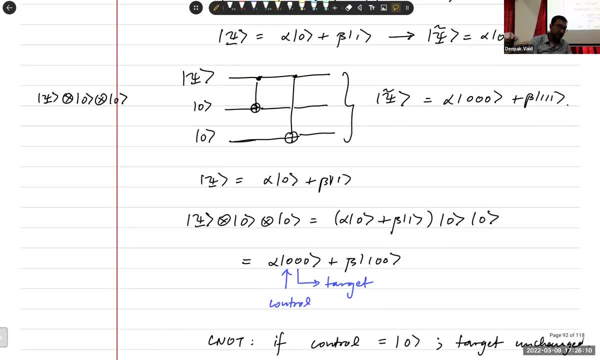 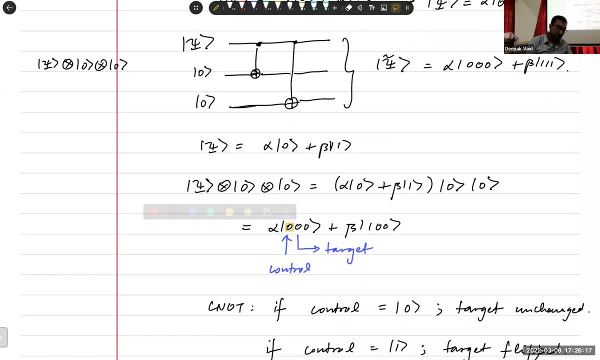 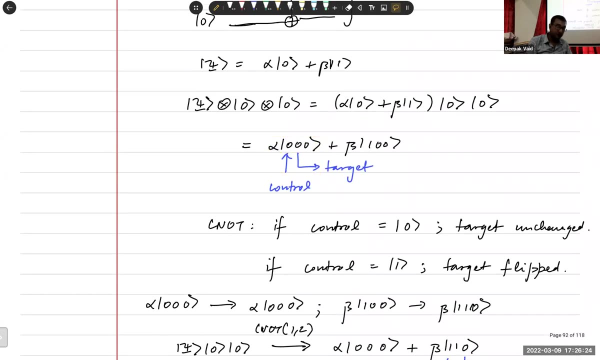 now, when you apply the CNOT gate. this is the control and this is the target right. So this first bit is the control, the second bit is the target. So in this state nothing happens, because the control is zero right. 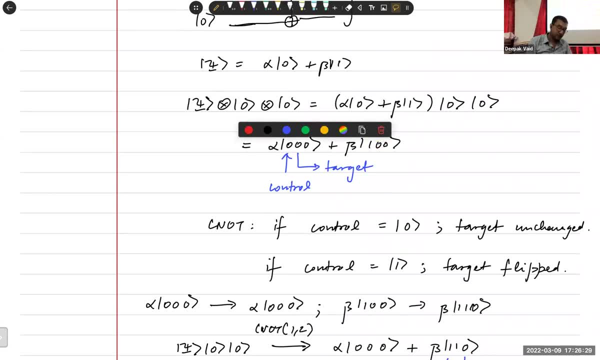 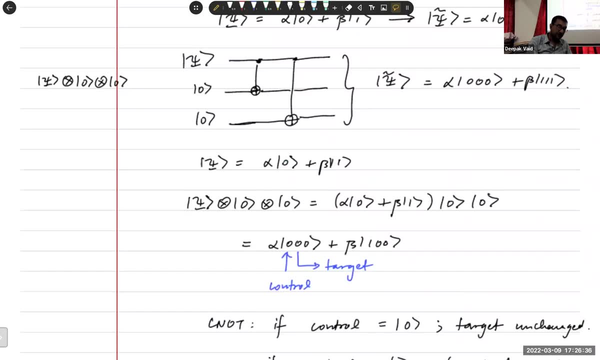 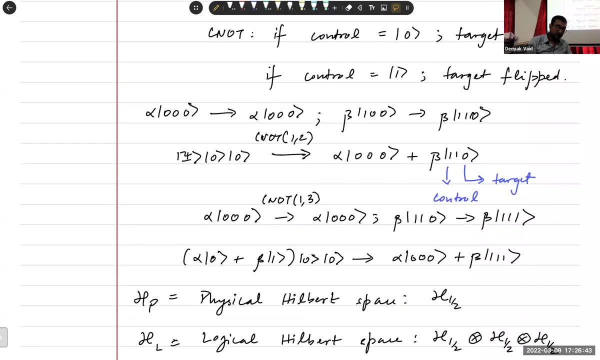 In this state the target is flipped because the control is one right. So you get beta one, one zero. Then you apply the CNOT gate again, using this as your control, and this is your target, And once again, so nothing happens to the first state. 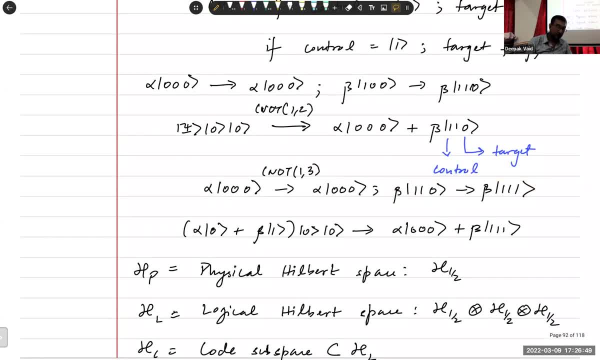 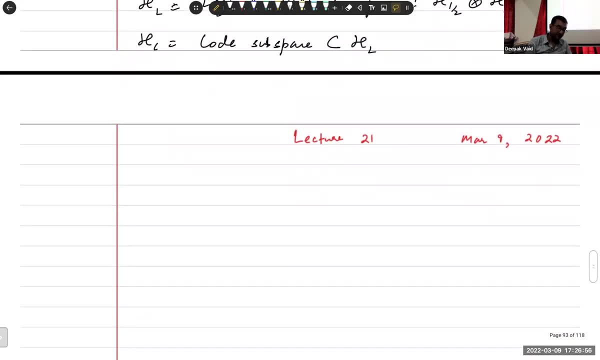 but the second state goes to one one, one right. So you end up in this, in this state, right, And this is called a. this is called a cat state. There's a word for it. States of this form are called cat states. 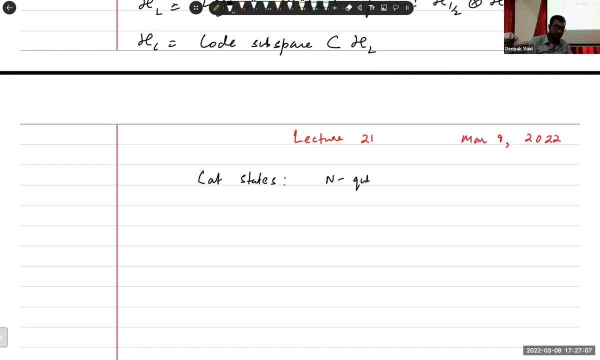 So, typically, if you have an N qubit, you have a state which looks like this, something like one by root, two, all zeros and all ones. So, first of all, this is a highly entangled state, right? There is no, you cannot factorize it, right? 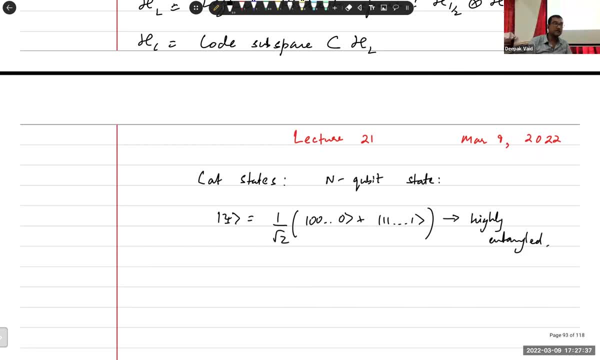 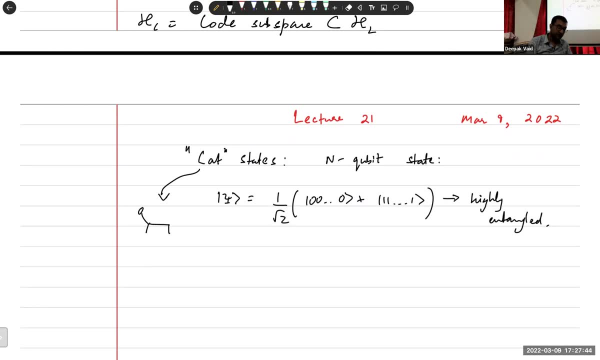 So it's highly entangled And the reason we refer to this state right, We refer to this as a cat state right, Because we are actually referring to Schrodinger's cat. that cat, okay, Because in the limit of large N right. 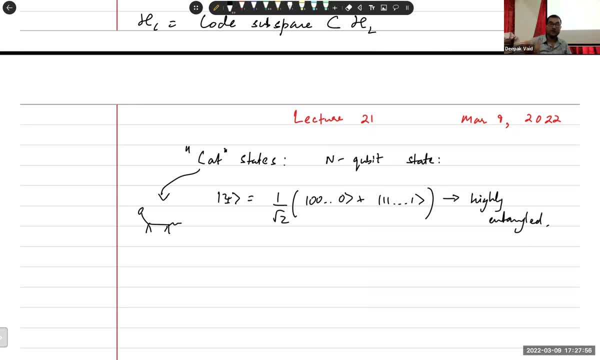 Your system becomes more and more macroscopic, right? So if you imagine that, that you have a system which is consists of a very large number of qubits, like enough to make a cat, and you put that system in this, this kind of a state, 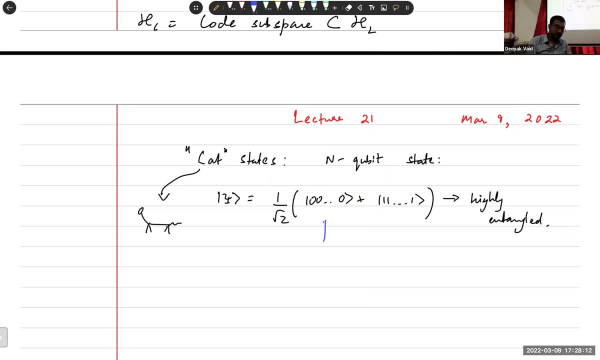 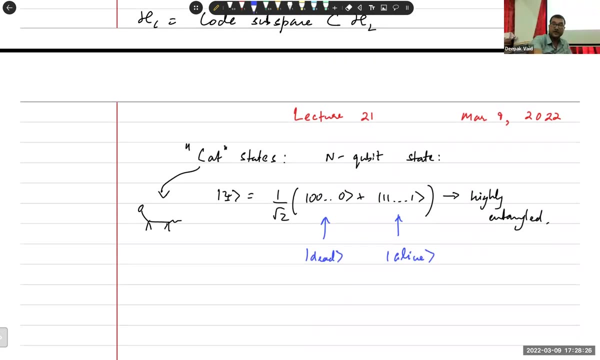 this would correspond to, let's say, this could be something like dead and this could be alive, right? So this would be the statement of Schrodinger's cat, right? Okay? so now let's talk about error correction. So how can we? 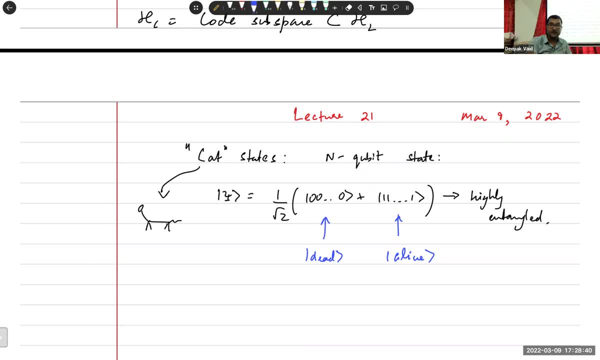 how can we correct errors in our system? Okay, So we have to perform a measurement. Without performing a measurement, we can't tell if there is been an error or not. But the problem is that typically, measurements will cause your quantum state to collapse. 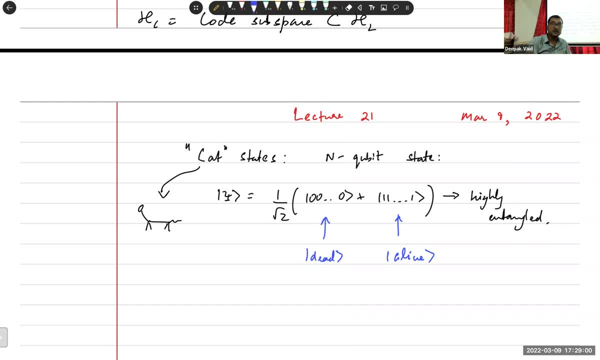 You will lose quantum, you will lose the quantum correlation, right, And you don't want that to happen, right? So you want to perform measurements, but you want to perform them in a way that your quantum state, or at least the information, 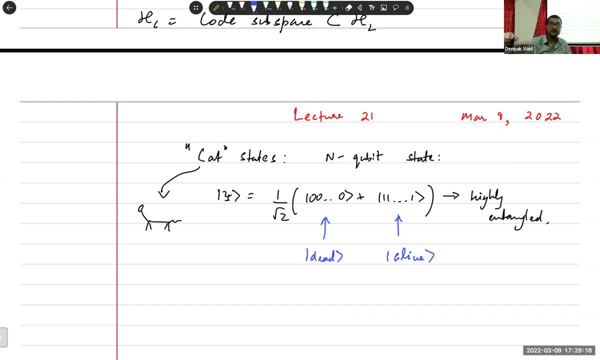 the quantum information that you want is left undisturbed, And you can do that using these operators. So these are projection operators. okay, I hope that you all remember what a projection operator is right. A projection operator is something of the form. 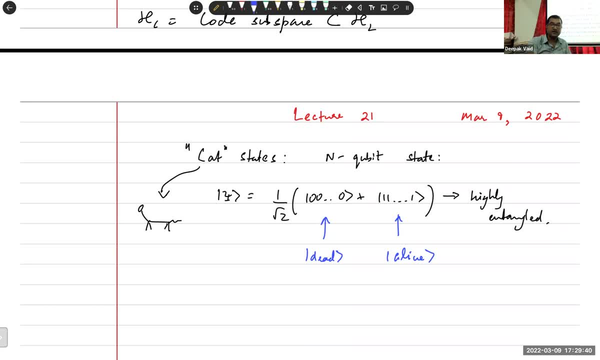 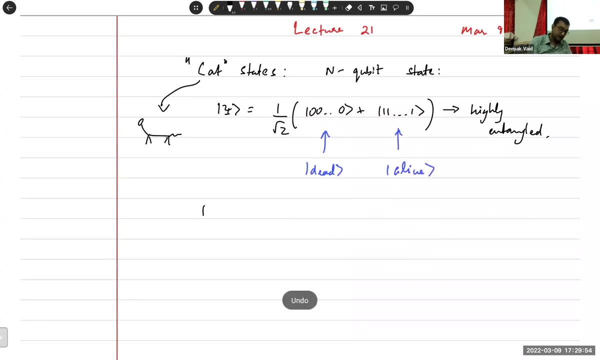 bra phi, ket phi, right. And so this is a projection operator: 0,, 0,, 0, and this is another projection operator, right? What will be the effect of this projection operator? So let me say that I have. 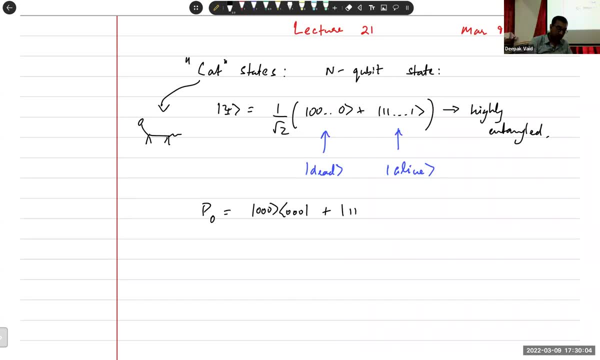 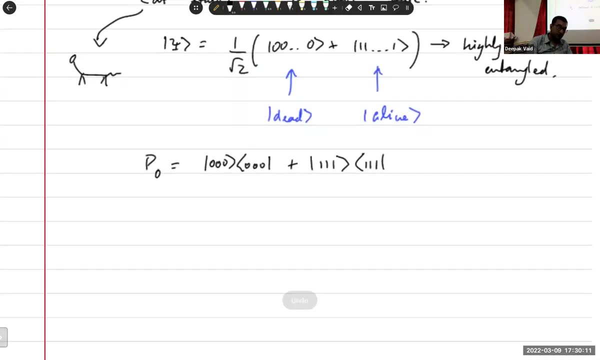 is this too small? I think maybe it's a little bit small. I'll try to write a little bigger so that you can see a little bit better. I'll try to go clearly. What will be the effect of this projection operator on our logical, on our encoded state right? 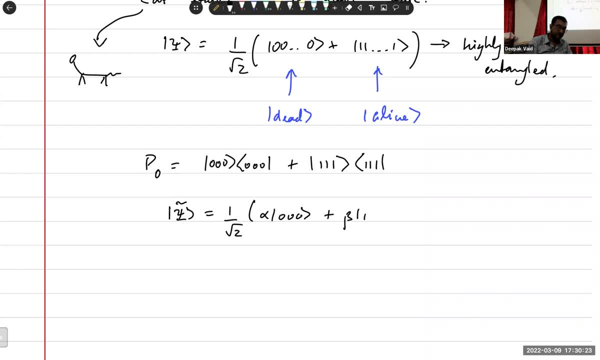 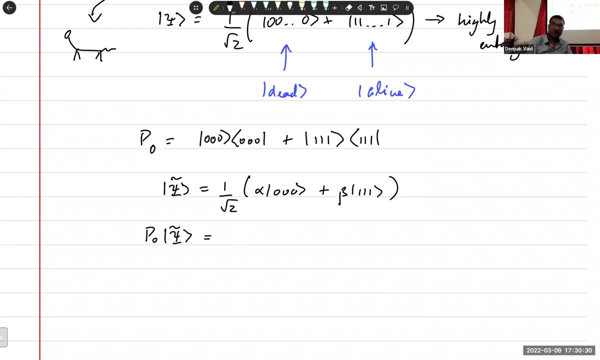 So this is our encoded state and we act on this state with p non right. So we have this guy and acting on on this fellow right Now, the first set of 0, 0, 0,. 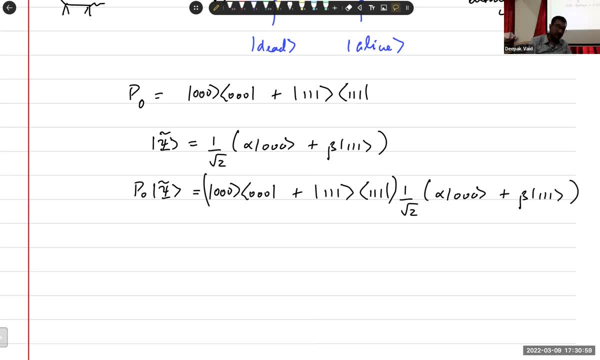 that operator will annihilate the second, the second component, because 0, 0, 0, is orthogonal to 1, 1, 1, and similarly 1 1, 1 will annihilate 0 0, 0. so you will be left with with side right. so 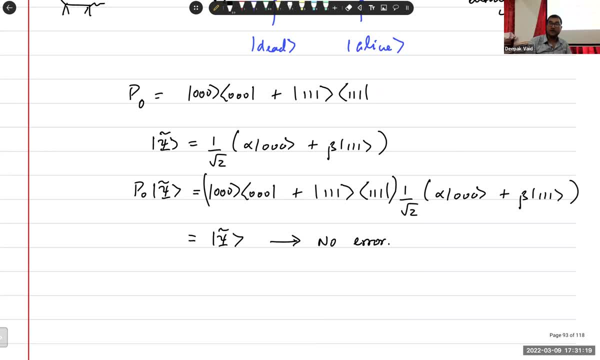 this means there is no error, right? similarly, we can construct other projection operators, okay, and here we are, given a set of three projection operator, right, and we want to look at. in this case, we are first looking at. i'm sorry about you guys, but the people on on. 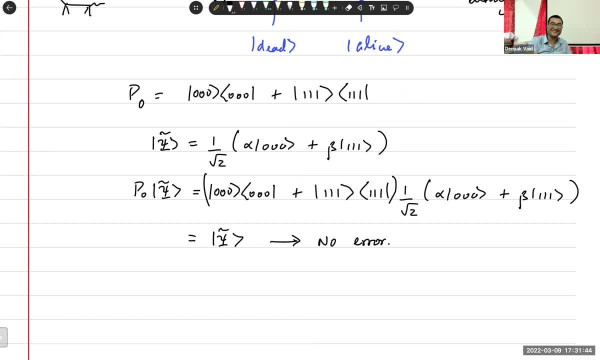 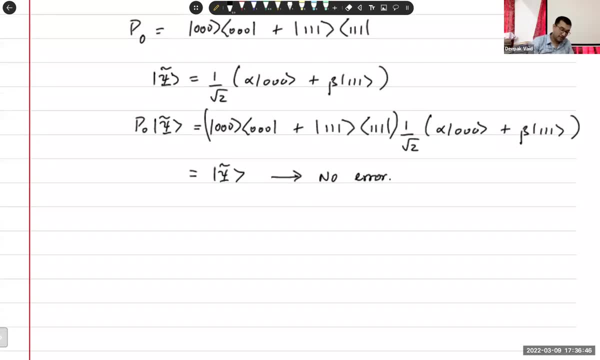 zoom can see this just fine. so then, we have. now we have a set of four other projectors, okay, which have the similar form: one zero zero. one zero zero. can you guys see it on your phone? okay, good, right, so this, what is this projector doing? right? this is projecting onto the case. when there is a single bit, flip right, there's a. 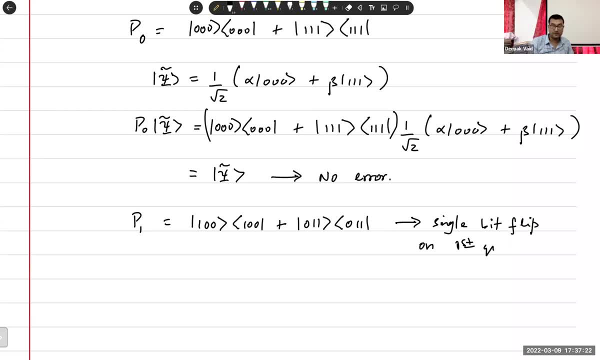 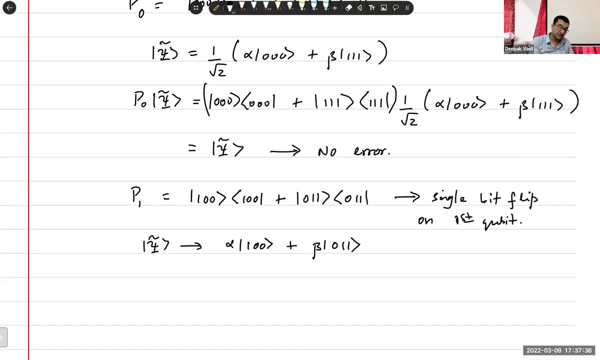 single bit flip on the first qubit. so if there is a single bit flip on the first qubit, what will what will happen to size? i will go to 100, 011, right, and so that's what the second, this projector, is doing. this state is 100 and the state is 011. so, once again, if you act on- and so let me call this, 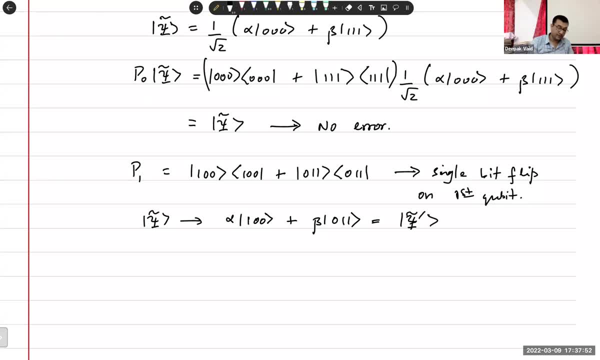 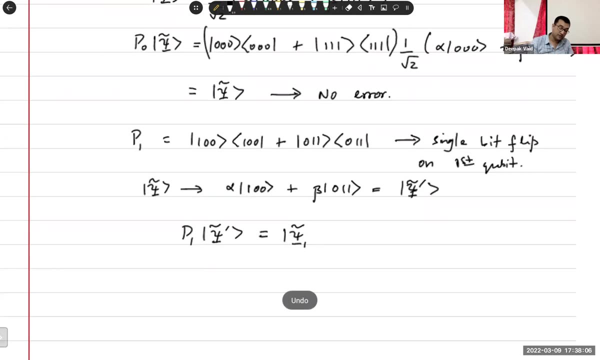 i don't know what to call it. let me call it si prime. if you act, if your state happens to be si prime, si tilde prime, and you act on it- P1,, you will get psi tilde prime. Okay, sorry, there's no 1 over there. 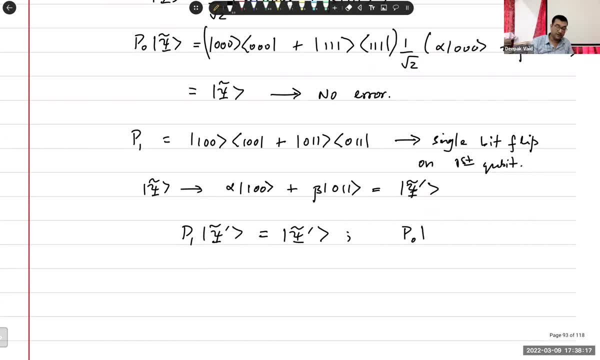 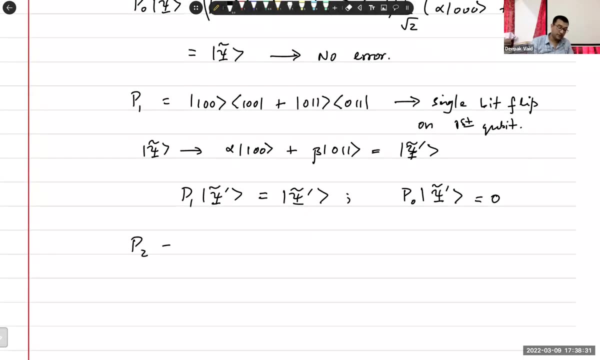 Right. And what happens if you take your projector P0 and you act on the state psi tilde prime. what will you get? 0. Right. So similarly, we can define projectors for a single bit. flip on qubit 2.. 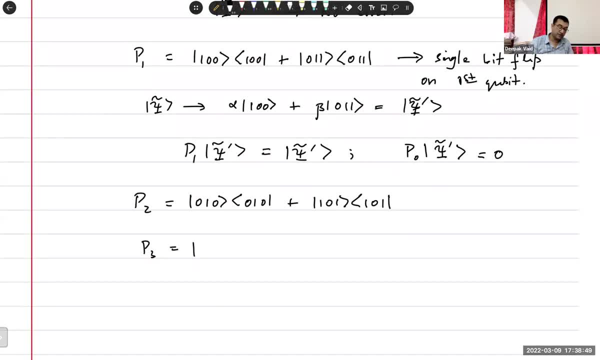 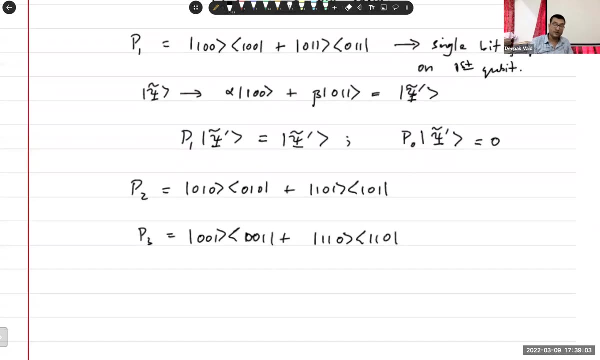 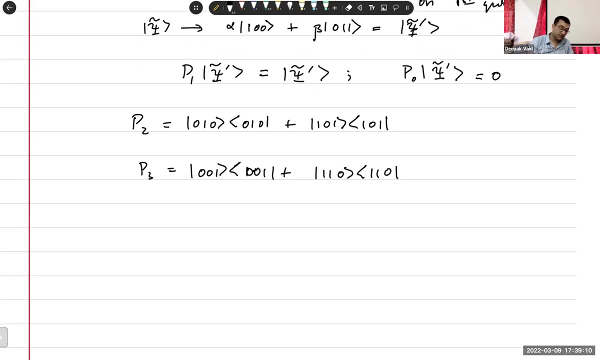 Then we can define a projector for a single bit. flip on qubit 3.. Okay Now so if you measure, if you measure your state right, You will get 0. if the condition, if the i-th condition, is false, Right. 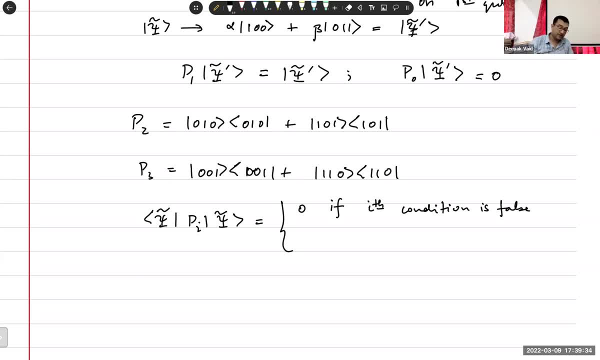 i-th condition means i goes from 0,, 1,, 2,, 3.. Right And 1, if it is true. If i-th condition, i-th condition meaning referring to these projectors, So each projector corresponds to a condition. 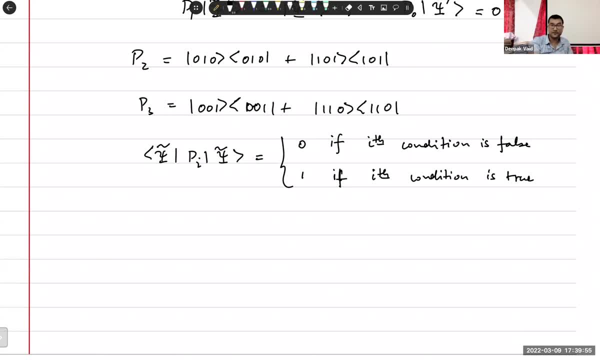 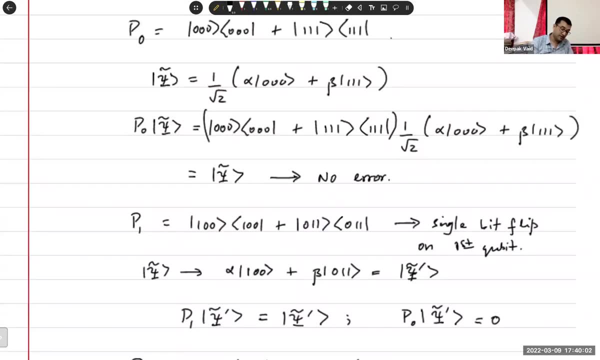 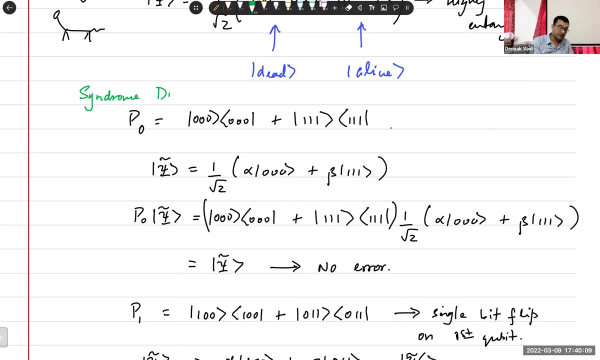 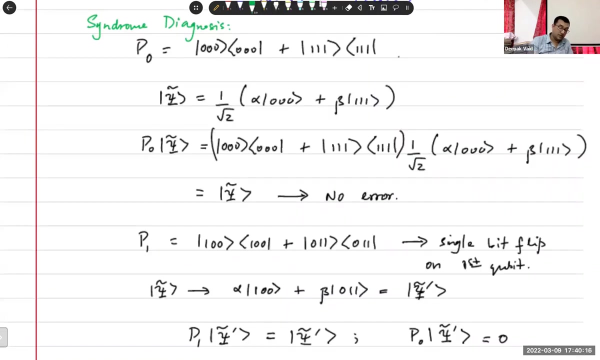 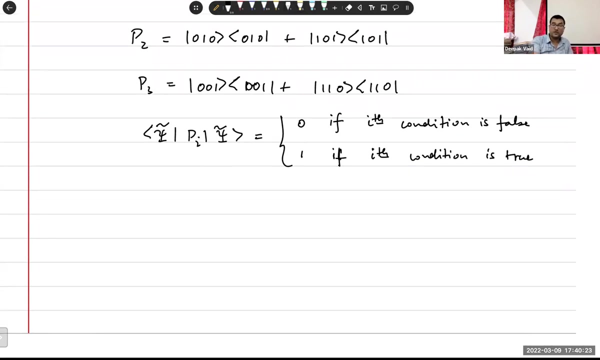 that there has been a bit flip, Right, So this is called. this is called syndrome, syndrome measurement, Okay, Or syndrome diagnosis, Okay. Now what is the nice thing about this syndrome diagnosis is the following: What happens to the state after you make a flip? 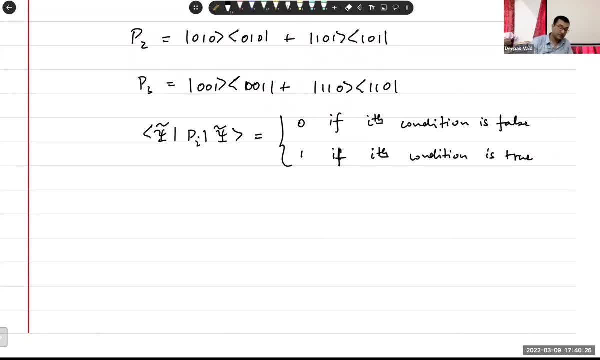 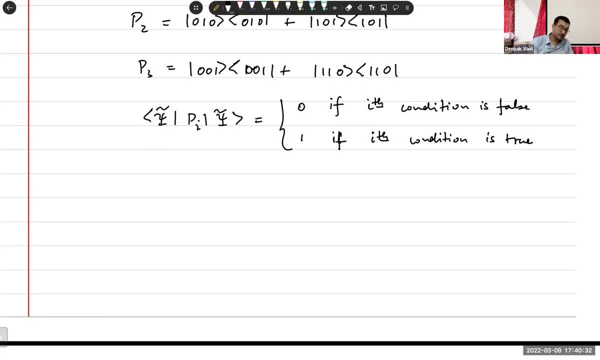 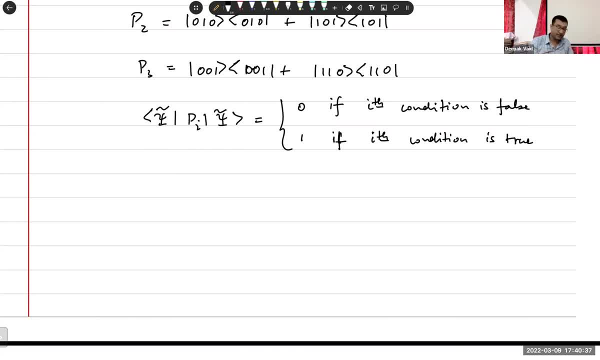 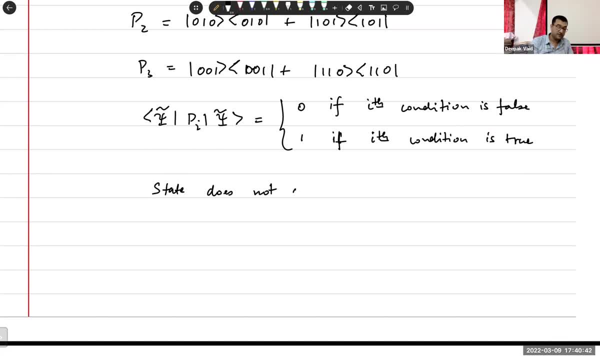 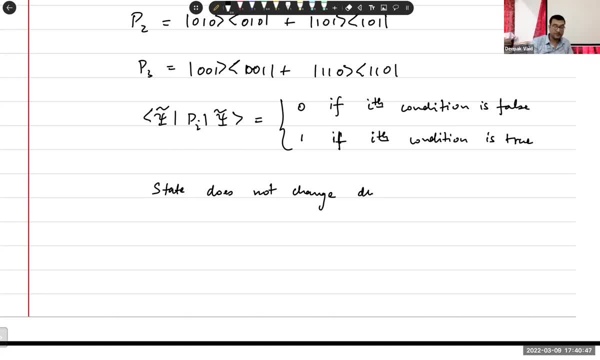 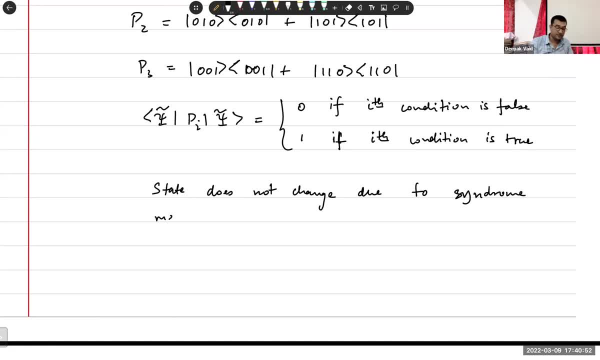 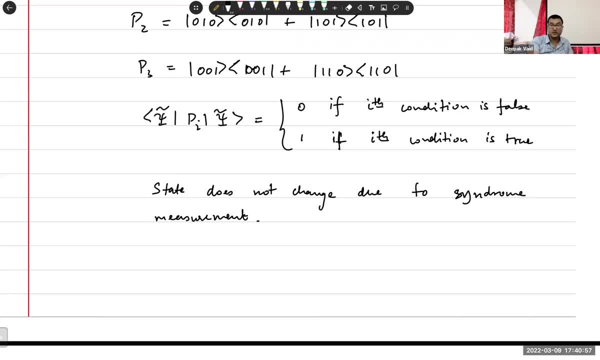 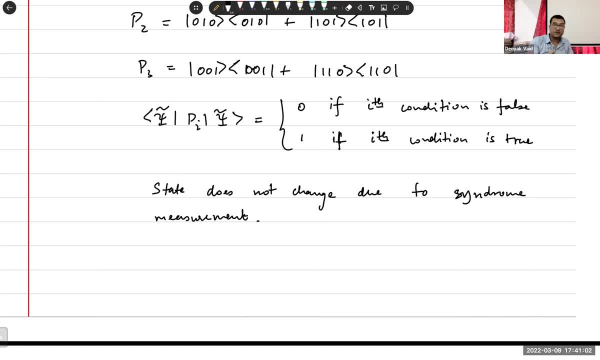 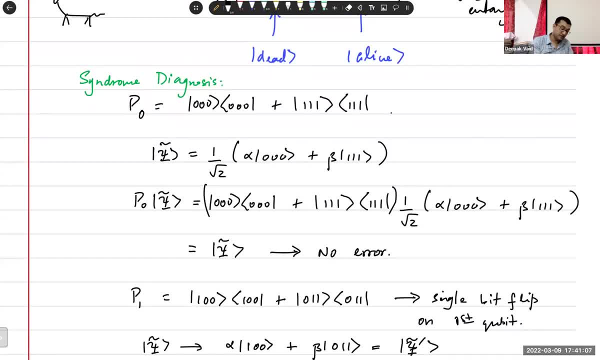 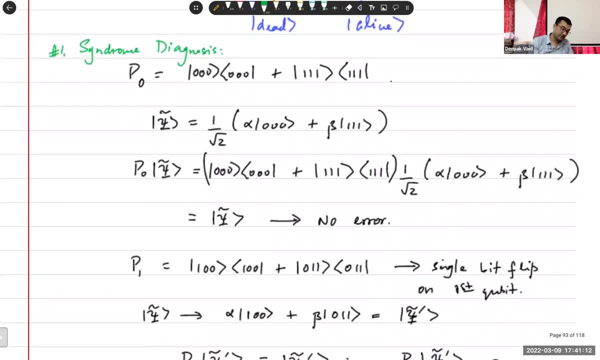 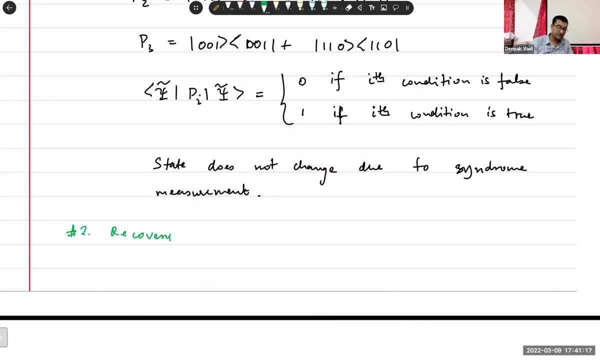 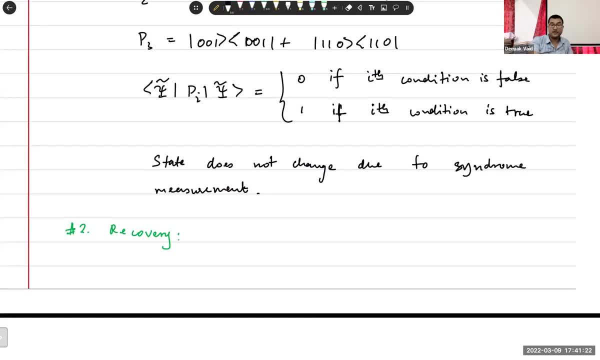 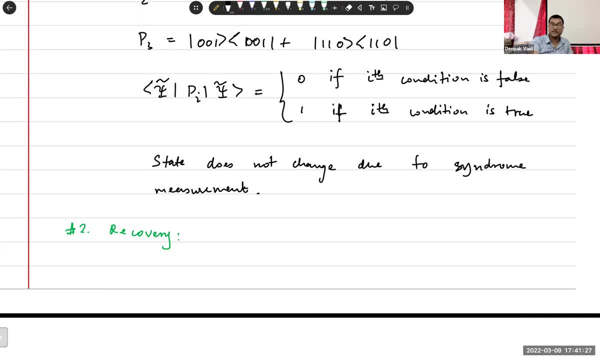 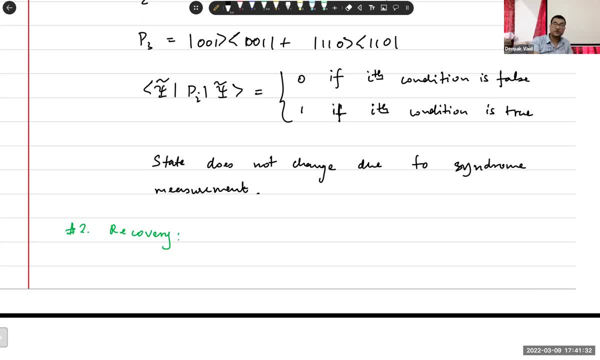 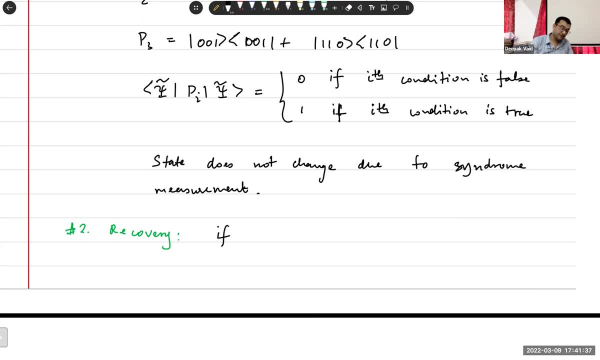 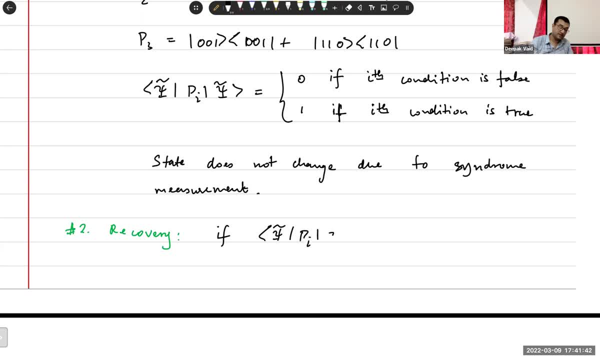 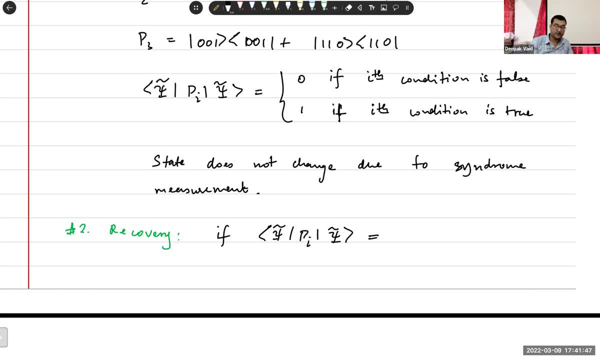 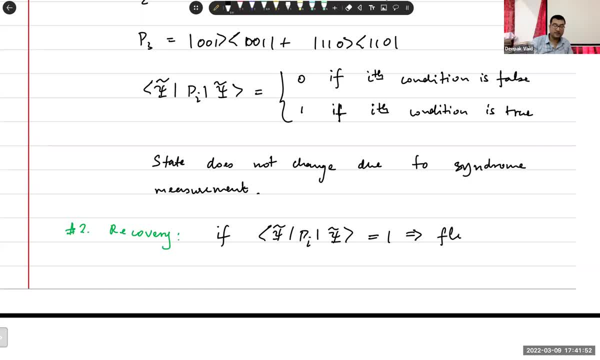 What happens to the state after you make the measurement 1, this implies that you flip the ith qubit and that will correct your state And we will see why this doesn't affect the state itself. We will look at the circuit in a little bit. 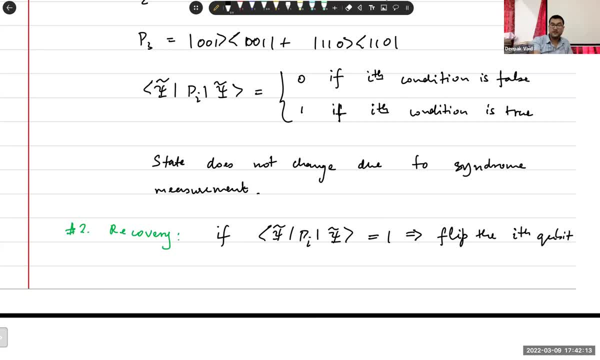 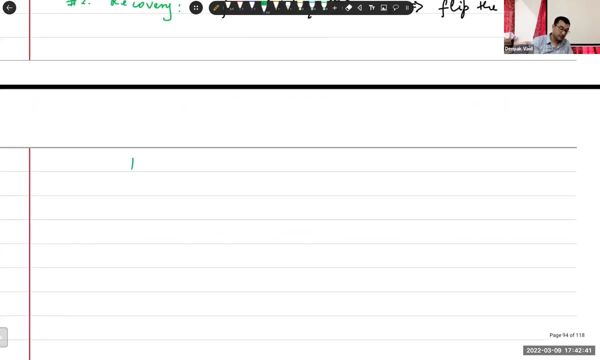 And so this procedure works perfectly, provided that bit flips occur only on one or none of the qubits. In the event that you have more than one bit flip, it won't work, right? Okay, Now let's see. Let's talk about phase flip errors. What is a phase flip? Right? So the 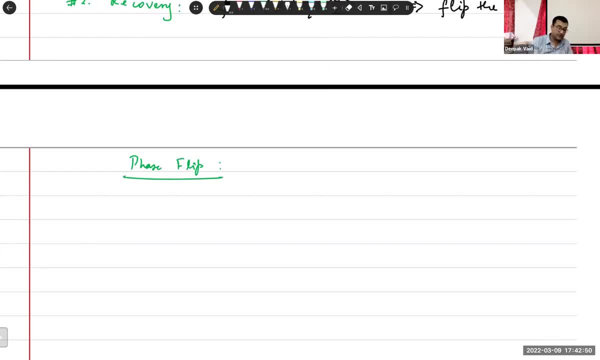 phase flip is, as I've mentioned, a phase flip error. As I've mentioned to you before, you have some state right: Alpha 0 plus beta 1 in your computational basis. A phase flip is when the relative phase between the two qubits. 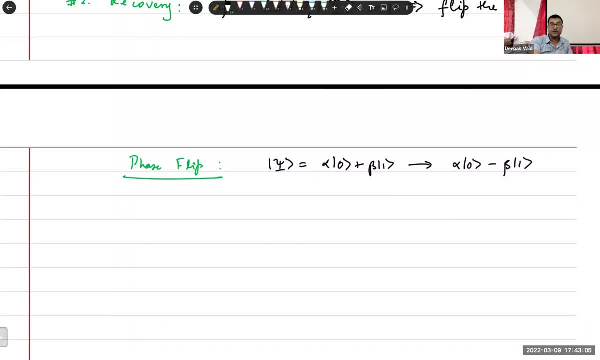 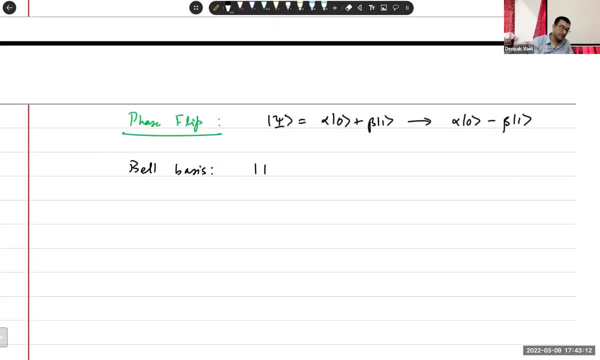 flips, Okay. And if you work in the Bell basis, right. So the Bell basis plus minus state is given as 0 plus minus 1.. By root: 2, right. So in the Bell basis you can write psi as. so if you, you can invert. 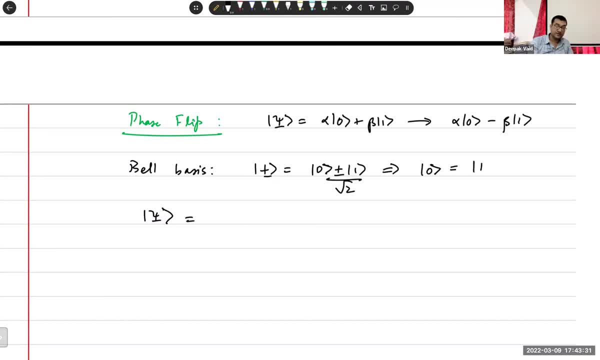 this relationship. you can write 0 as this and 1 as plus, superposition of these two states, right? So if you, if you substitute these expressions for 0 and 1 into into your state right, what you will find is: let's see, we'll get alpha by root, 2 minus and then. 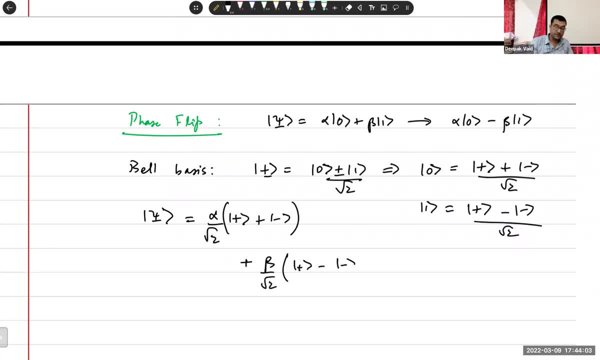 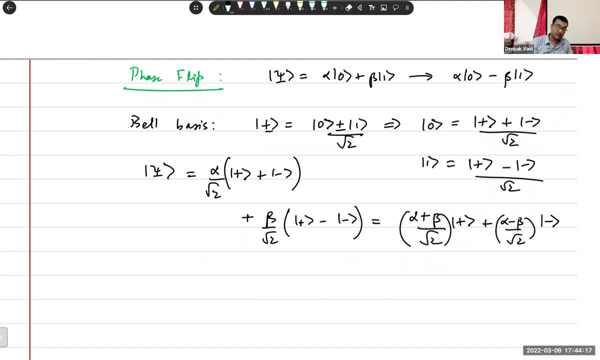 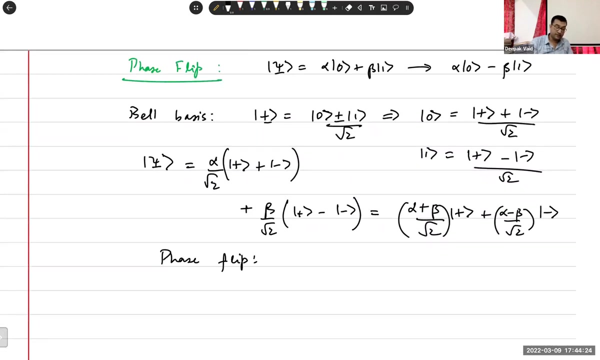 beta by root 2 right. So we can write that as alpha plus beta by root 2 plus right, And then plus alpha minus beta by root 2 minus. So a phase flip: plus minus goes to minus plus right. 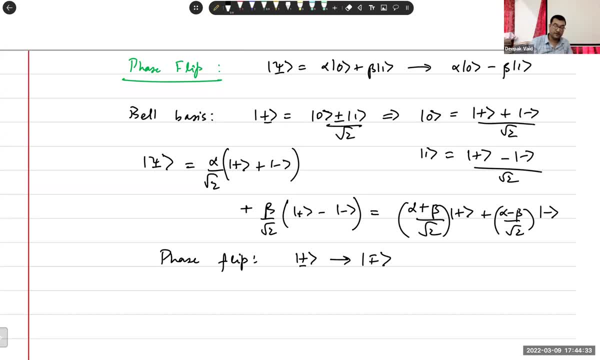 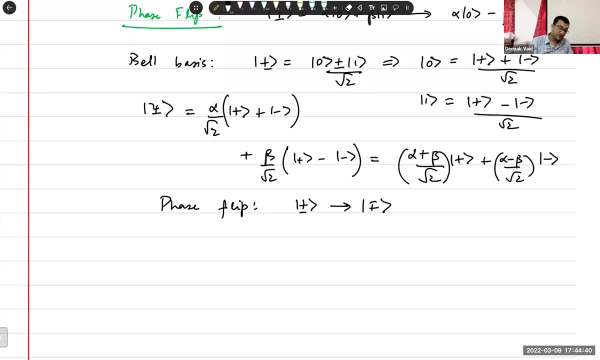 In this basis you can see that if you have a phase flip that corresponds to bit flip in the bell basis right. So in the bell basis under the phase flip you would go from alpha plus beta by root 2, this would become the minus state and this would become the plus state. 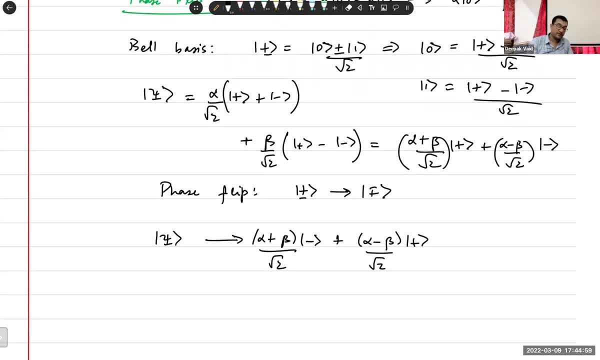 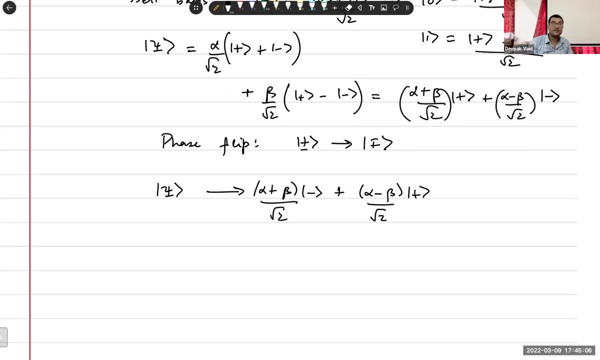 So the question is that we want to protect against phase errors, right? So if you want to protect against phase errors, this suggests that we can just work in the bell basis And we use the three-qubit code or this three-qubit redundancy, but now in the bell basis. 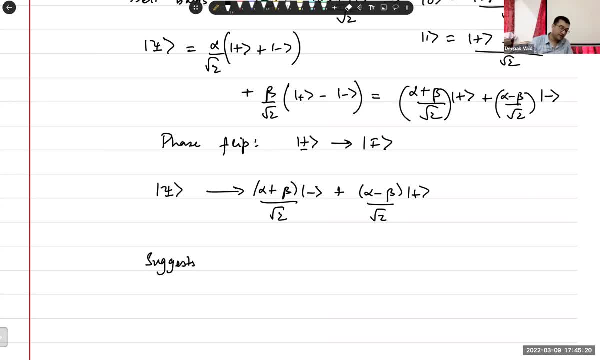 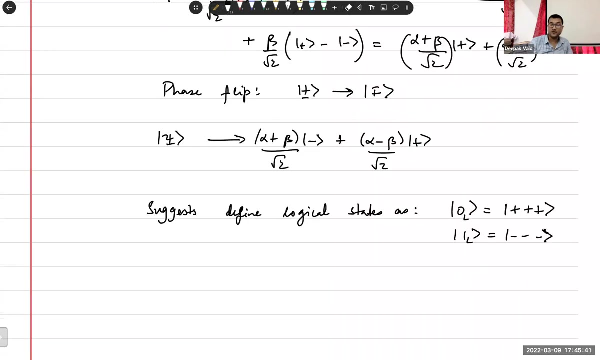 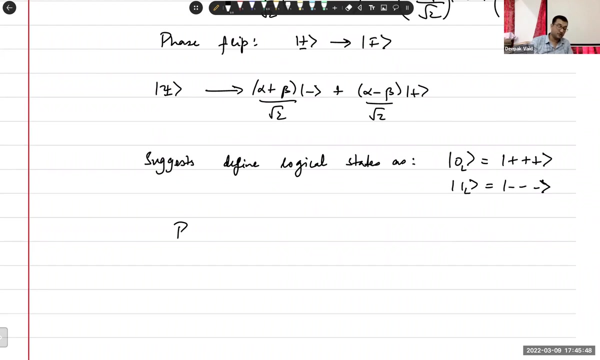 So that means we define these logical states as follows: So your logical zero can be written as plus, plus, plus, and your logical one can be written as minus, minus. So then exactly the same procedure would follow through. You would have syndrome measurements, right. 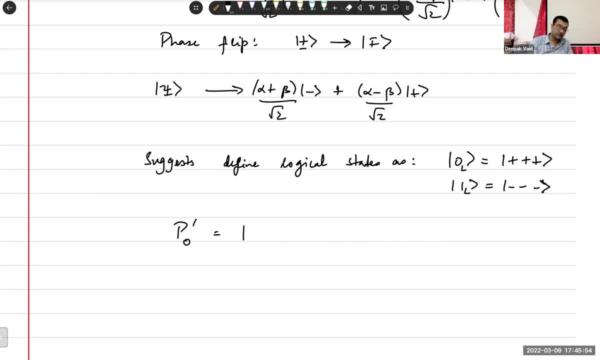 Operators for syndrome measurement, which would be of the same form, But now, of course, in the bell basis. So this is the bell basis. Okay, so I'm just. This is just to show that all the qubits are the same, except for the ith qubit which is flipped in this projector. 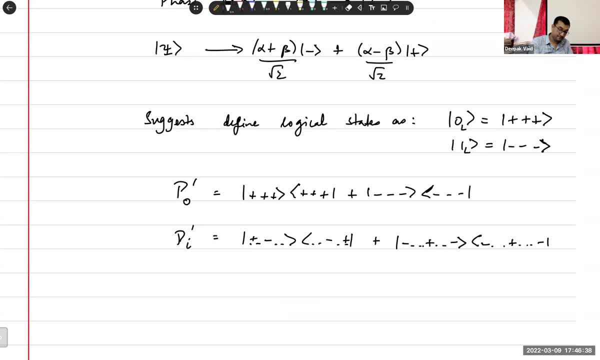 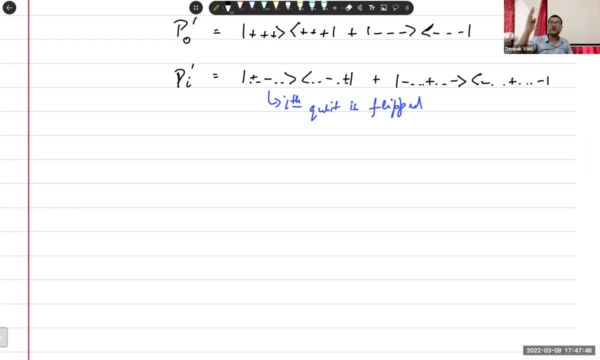 Yeah, So we're sure that there won't be a bit flip in the bell basis. But the thing is that what one does is we concatenate all of these possibilities. So we'll look at the circuit implementation in a second right. 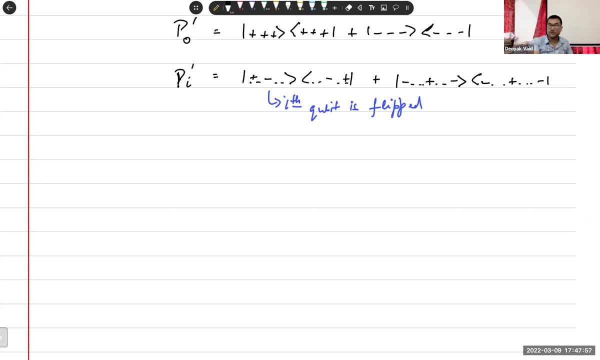 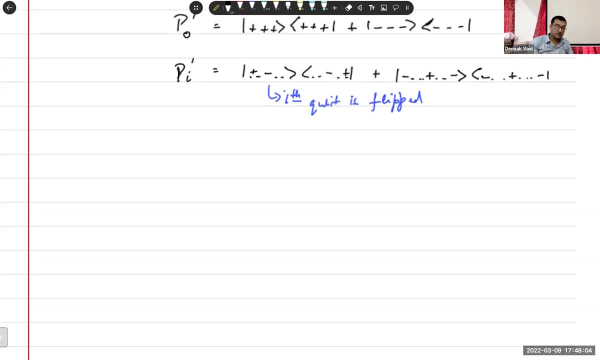 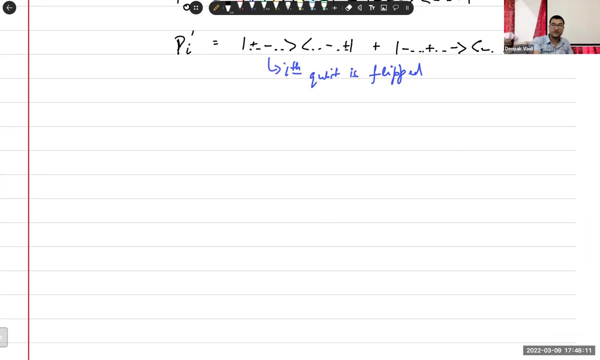 And hopefully you will see what is going on. Okay, just hold on for a little bit. Now again, how do we encode our state in the bell basis? So for this phase, flip code, let's write down the circuit for that. 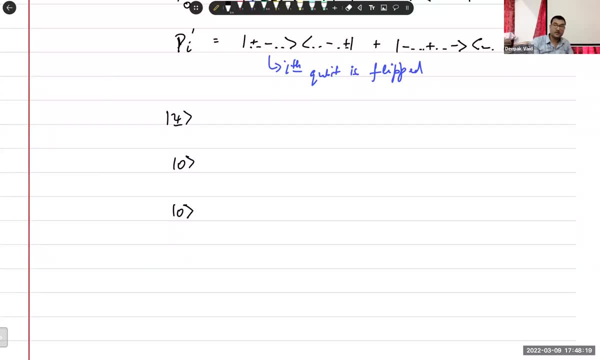 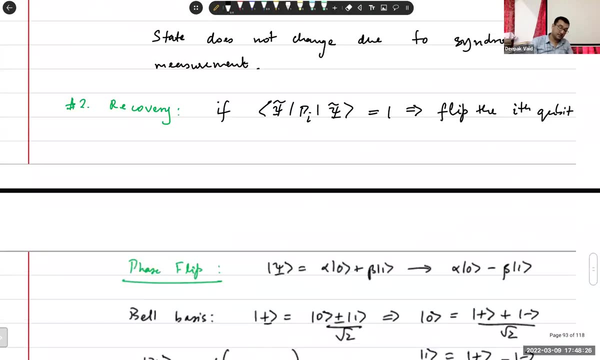 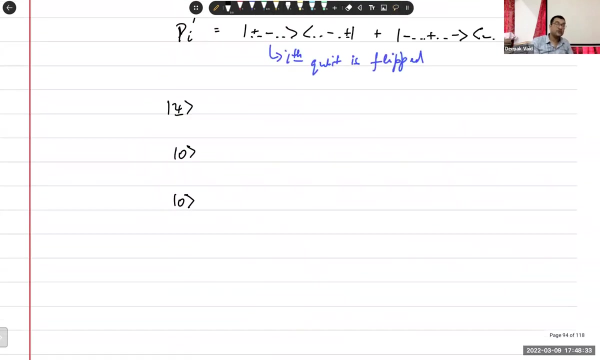 Can anybody think what the circuit might look like? If you want to generate this state, the plus plus plus state, right? Huh, What would you do? Adamard, Adamard, Adamard is our friend, right? So we do our usual C naught first, okay. 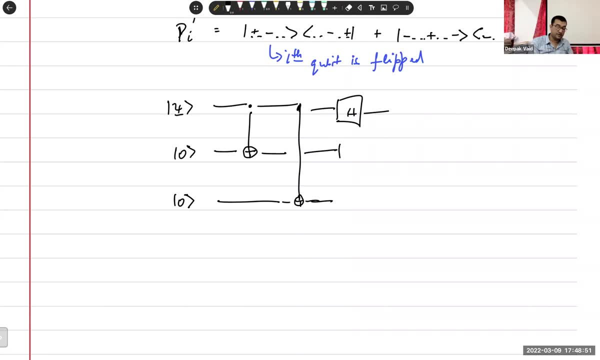 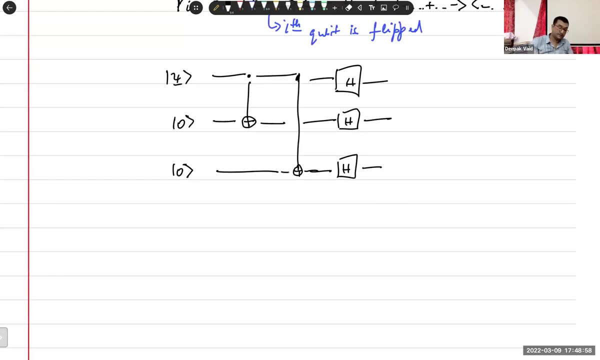 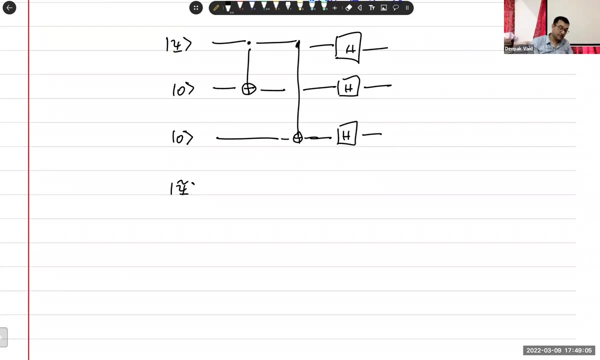 And then we apply a hard amount on each one of these qubits, right? So if you do this, what happens? Well, you end up with: First, you end up with this state. So you end up with this state, right? 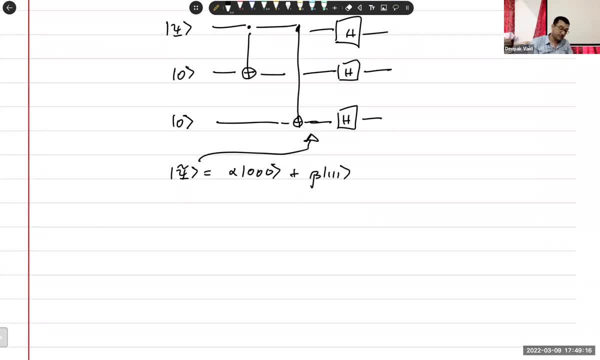 At this stage, after the first two C naught gates. And then when you apply a hard amount, what happens? Alpha 0, 0, 0,, for instance, goes to alpha by root 2, right, So you replace each 0 by a superposition of plus and minus states. 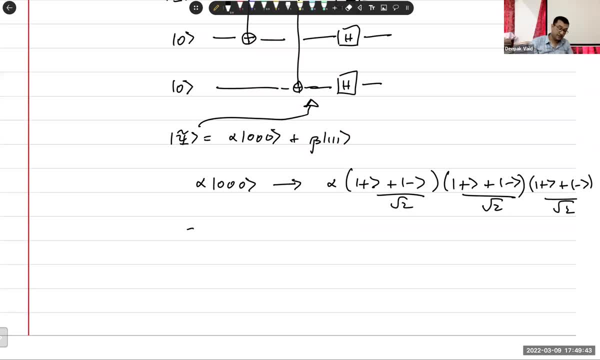 Like this: Okay, And so what will you get? You'll get alpha by 2, root 2.. Now you'll get plus plus, plus, plus, minus, minus, minus, plus, plus, right, Like this: 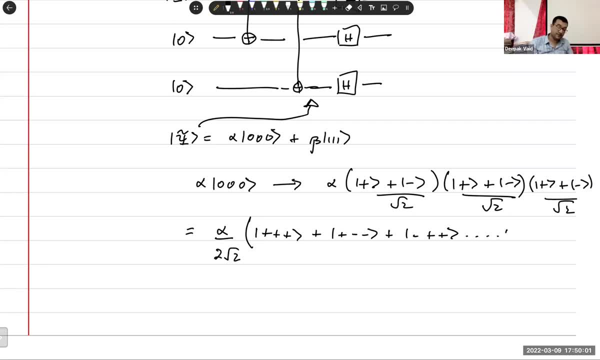 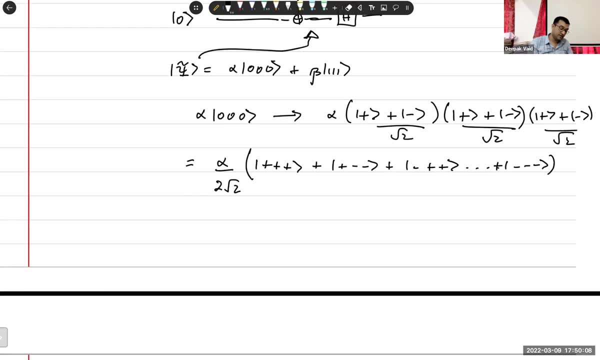 How many of these? There'll be eight of these, right? So you are getting all of the permutations of the plus and minus states. This is what happens to alpha. What happens to the beta one, What happens to alpha two, Exactly? 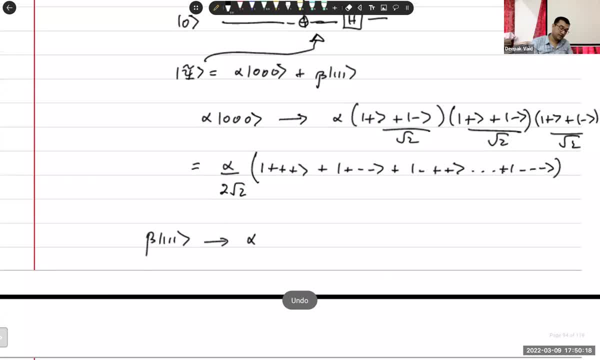 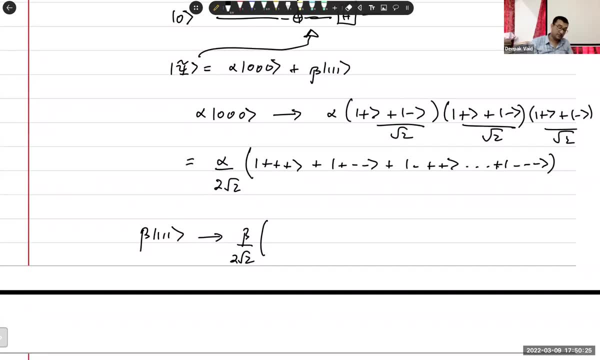 You get. You get alternating signs depending on the number of minus qubits, right? So you will get plus plus plus right, Plus minus minus. But then if you have one minus, you get plus plus plus plus right. 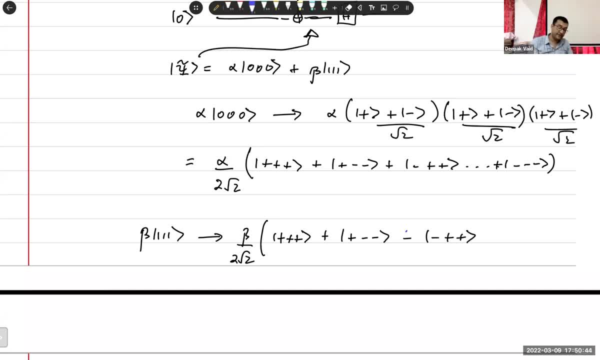 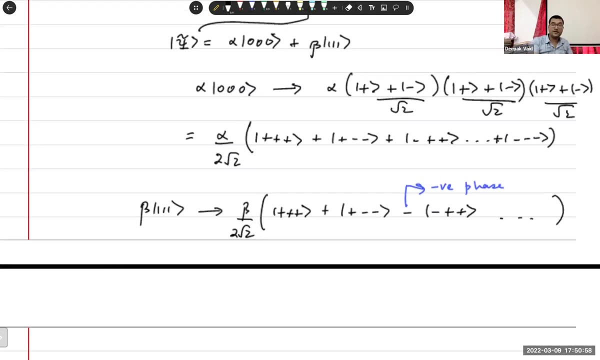 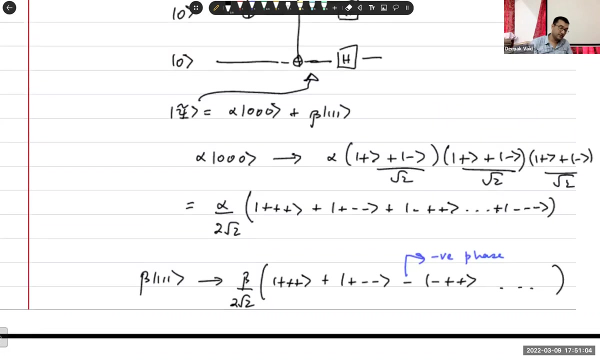 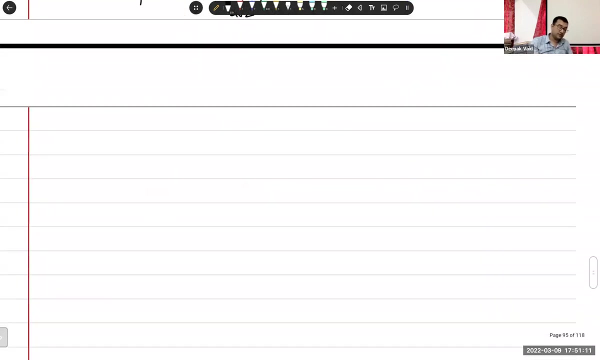 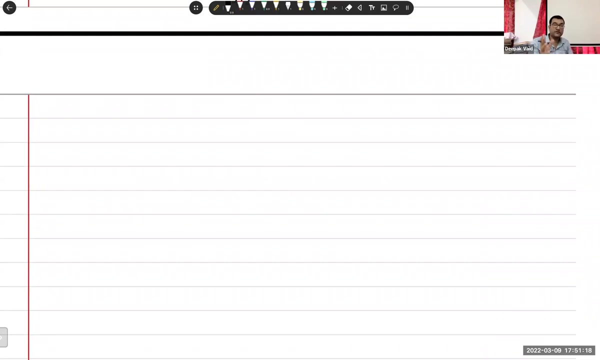 you'll get a negative sign, you'll get a negative phase, Okay and so on. Now, okay, and again we can define this thing: similar syndrome measurements. Now we would like to combine both of these into a code which allows us to correct for arbitrary bit flip. 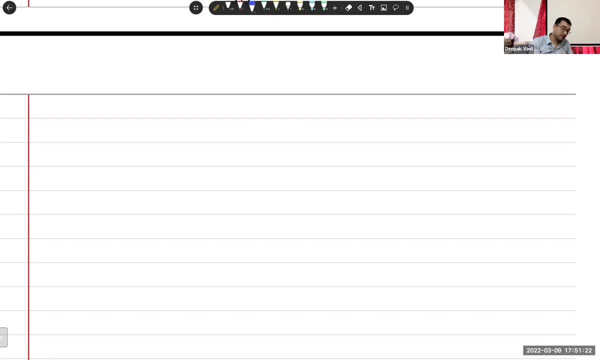 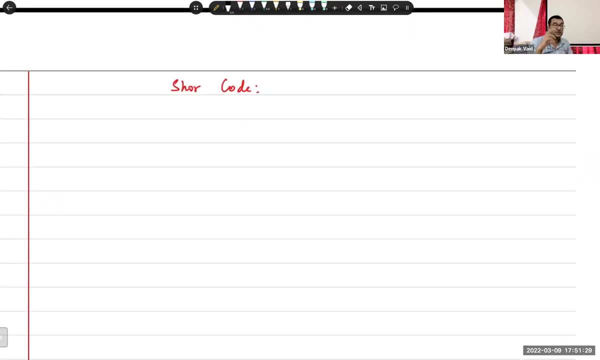 and phase flip codes. okay, So that is called. that code is called the Shor code. Of course, this Shor code is not the simplest code which is capable of doing this, but it is the first code which was discovered And, of course, it was discovered by Peter Shor. 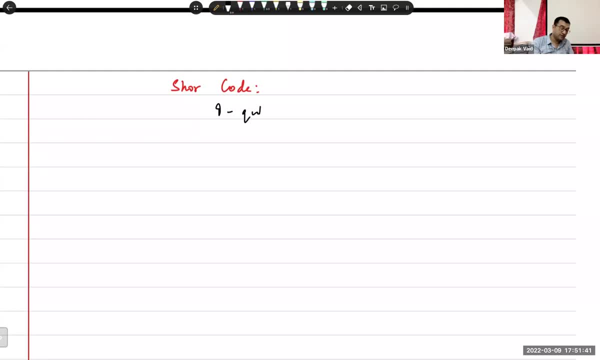 And it's also goes by the name of the nine codes. It's called the nine-qubit code because we encode one logical qubit in nine qubits. So how do we do that? Okay, So first we perform an encoding of each qubit into the bell basis. 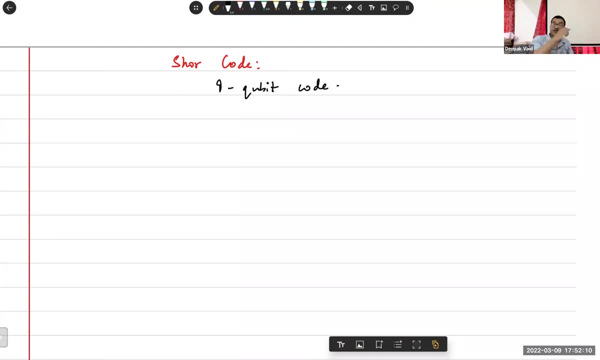 to protect against phase errors. And then we nest that coding within the bit flip code. Okay, so let me write down the state and then I'll explain. then you will see what exactly is going on. So your logical qubit is written as follows: 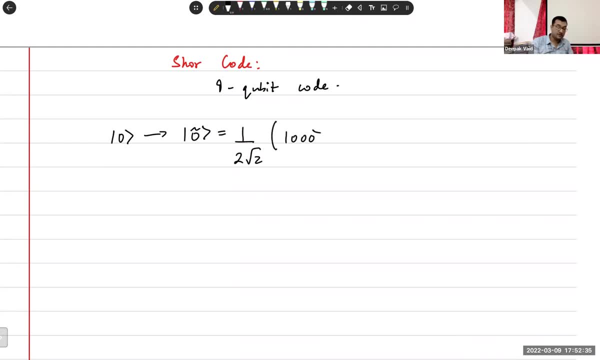 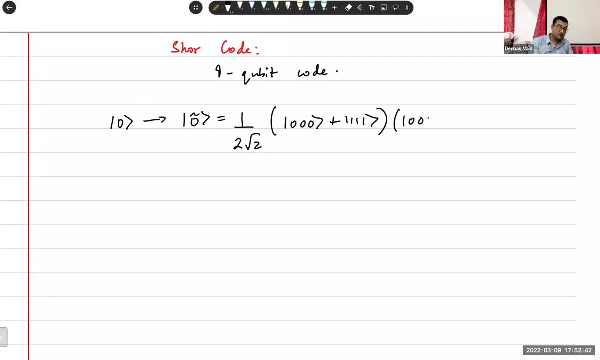 Okay, so if you're using the logical qubit, I'll just write this one over here And then you can see some olsa. so let's come back to that first one. So your logical qubit is written as let's see. 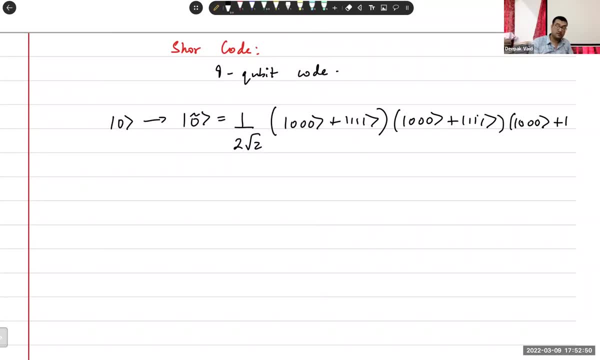 number one, one, one one. It should be returned as one, one, one, One one one. Okay, And then similarly, your logical one is written as less than that, the same expression, but, but with a relative negative sign. 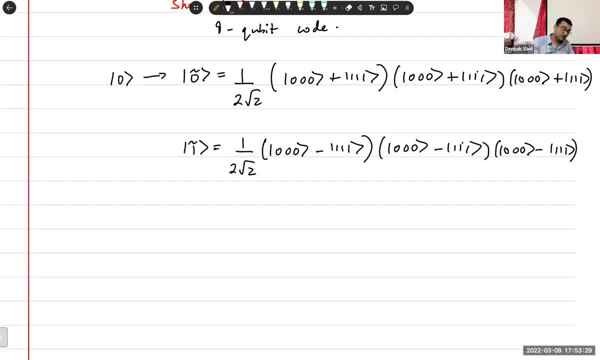 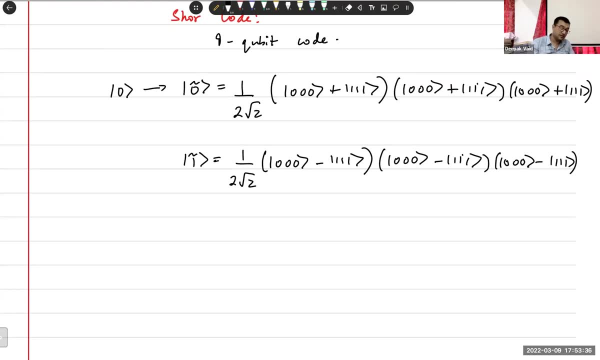 Okay, so now what will happen if there is a phase error on any one of the qubits? So phase error will cause one of these signs to change. So, for instance, if there is a single phase error, again this will correct for an arbitrary error on a single qubit. 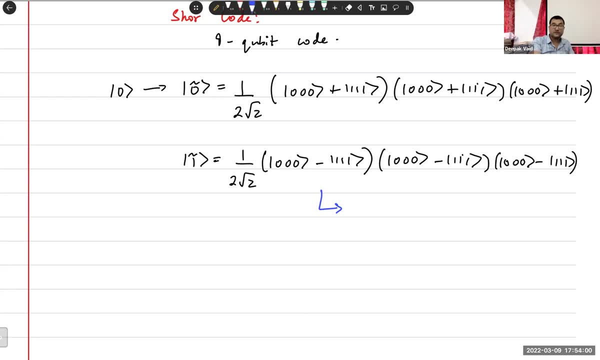 Whether it's a phase flip or a bit flip, But if it's on more than one qubit, it won't work. Okay, so we're going to look at only what happens if there is an error on one qubit. So let's say that any one qubit there is a phase flip. 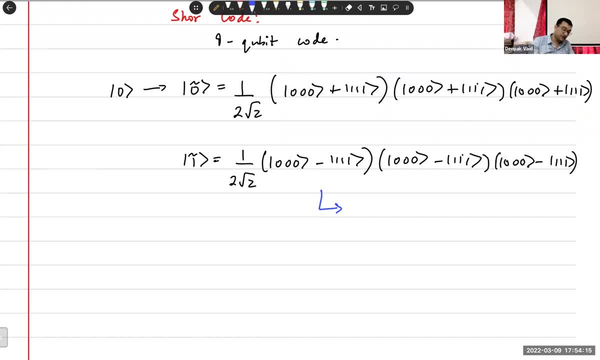 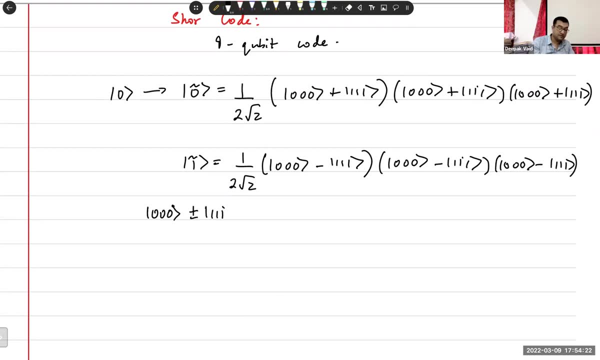 If there is a phase flip. what would happen? If there is a phase flip? this state would: you would get a change of sign right, 0, 0, 0 plus you'll get a change of sign, And then, similarly, if there is a bit flip, well then we know what to do, right. 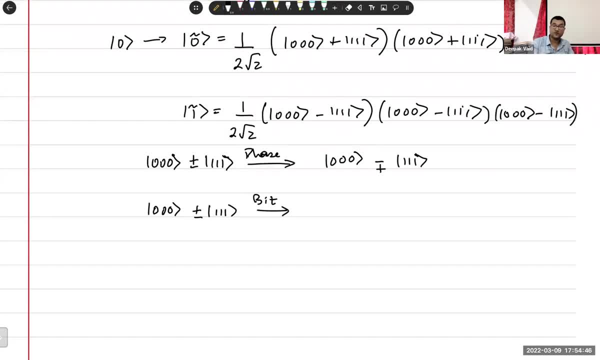 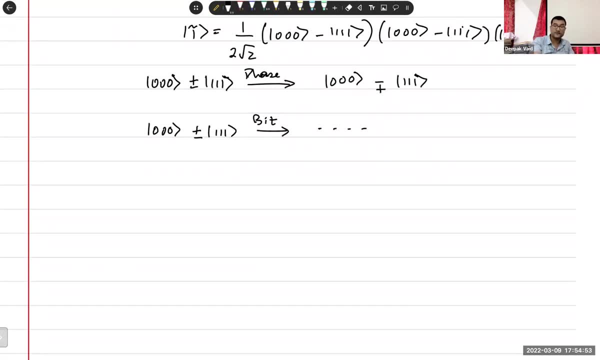 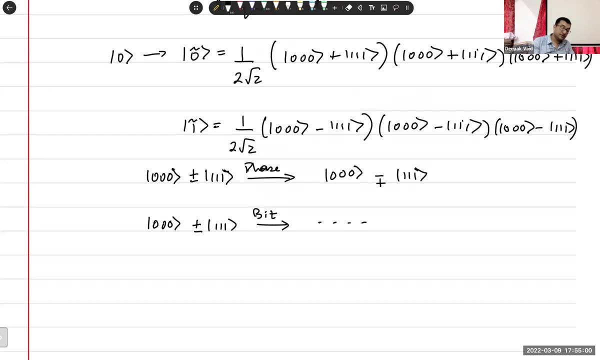 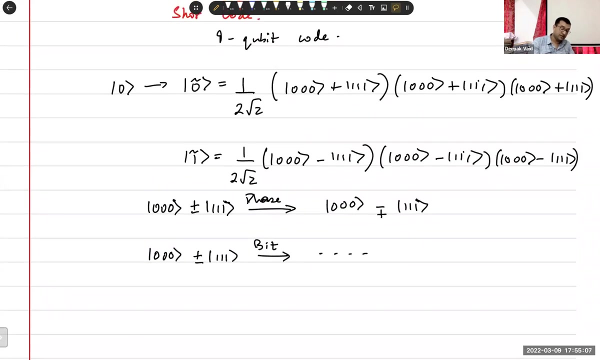 So then we have our projection operators with our syndrome measurements, We can use that technology. So again, let's see what the circuit is for making these states right. So what do we want to do? We want to take our state, which is alpha 0 plus beta 1, right? 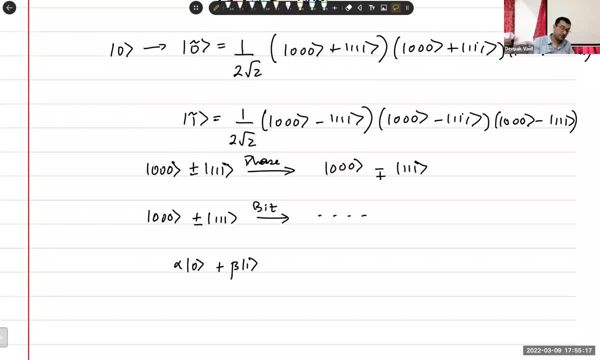 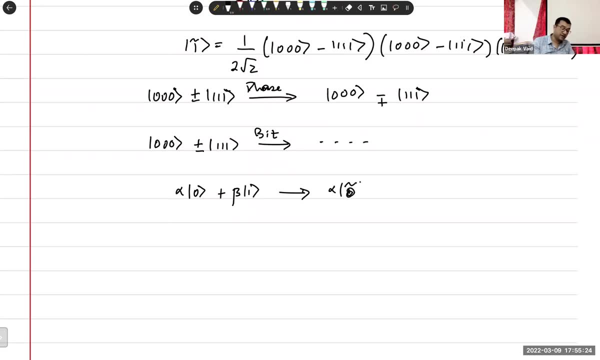 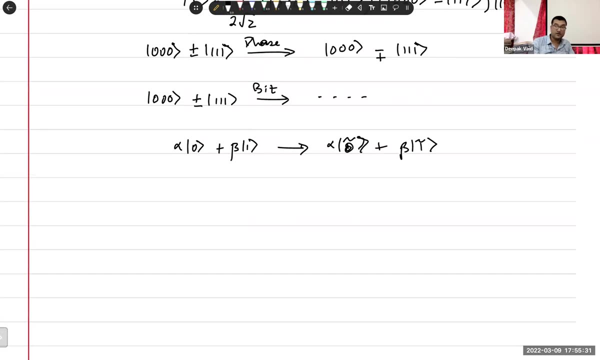 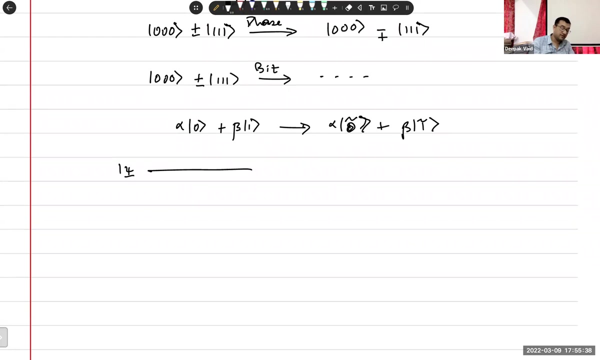 And we want to encode it into this basis. So we want our final state to be alpha tilde 0 plus beta tilde 1 or logical 1, okay, So let me draw the circuit. There are. this is our state. 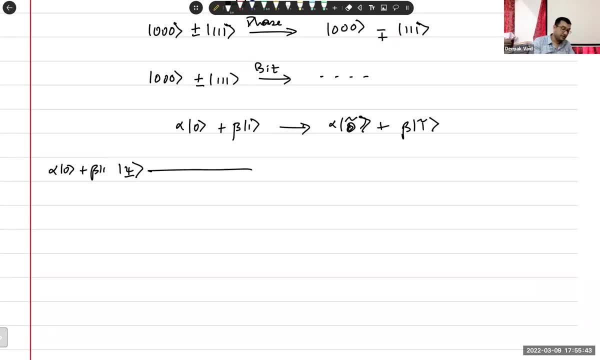 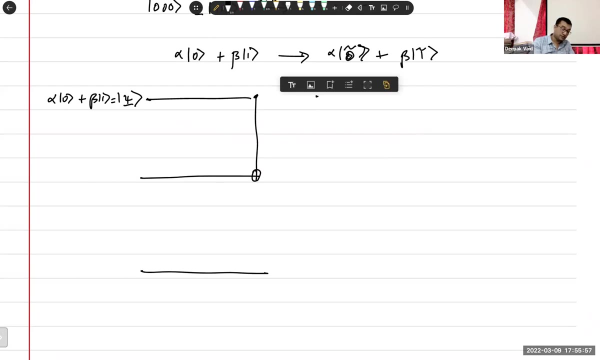 This is our initial state: alpha 0 plus beta 1.. And then we'll have our auxiliary qubits, And then we'll do theimo-part-synthetic- " Right, So if you, you, you send it through these, through this circuit, you get the 0, 0, 0 plus 1, 1, 1,. 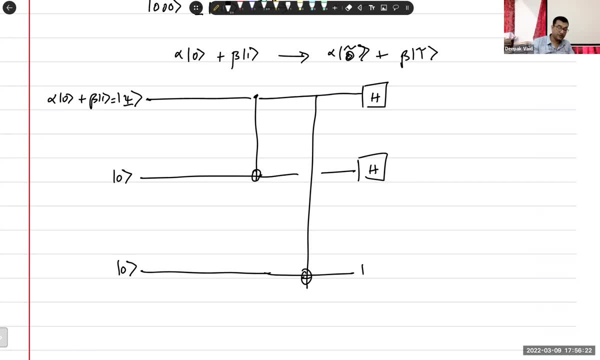 then you put the Hardamard gate on each one of these, put it between these gate and then you can draw the nth. 2, 1,, 2, 3, 2, 3, 4, 5, 5, 6, 7, 6, 7, 8, 9, 10, 10, 10, 20, 20, 21,, 21,, 21,, 22,, 22,, 23,, 23,, 24,, 24,, 25,, 26,, 27,, 27,, 28, and then you're done. 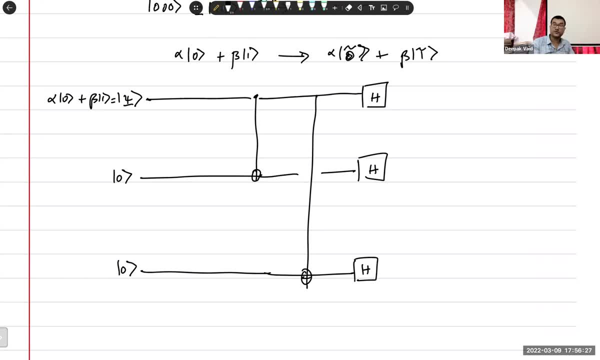 putting the Hadamard gate, does that transformation to the Bell basis, Then, like I said, you nest these two procedures. So nesting means we have another level of complexity nested within this one. So that means we introduce two qubits here and we'll introduce two more qubits at the next level. 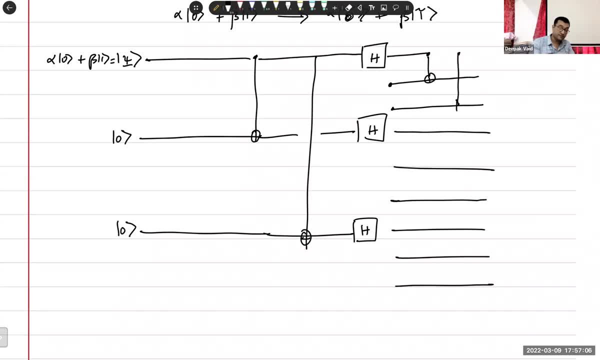 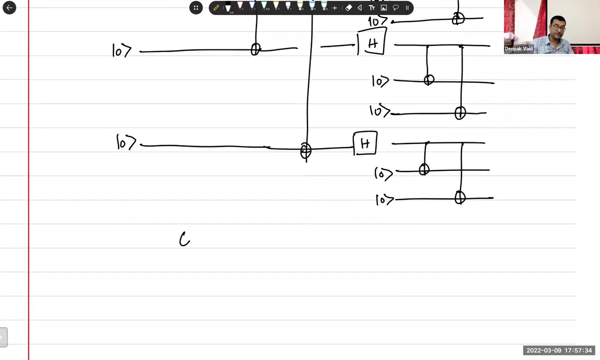 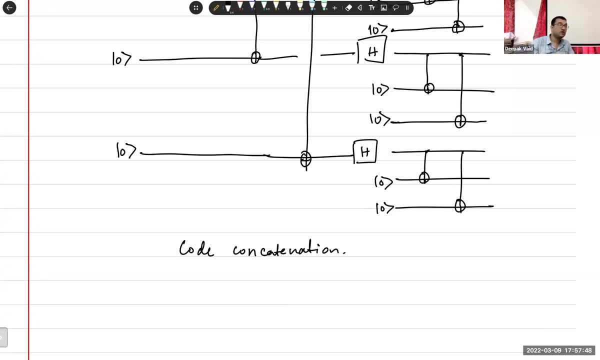 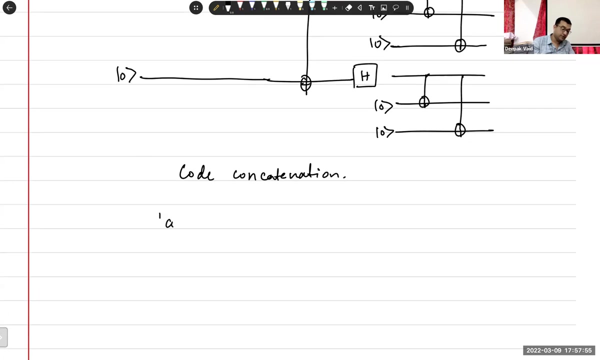 At the next level. So this will be zero, zero, one right Share of the of the circuit, This kind of code concatenation. So it's like you have taken one code and concatenated it with another node. So concatenation is the term that you use, for instance, when you want to take two strings. 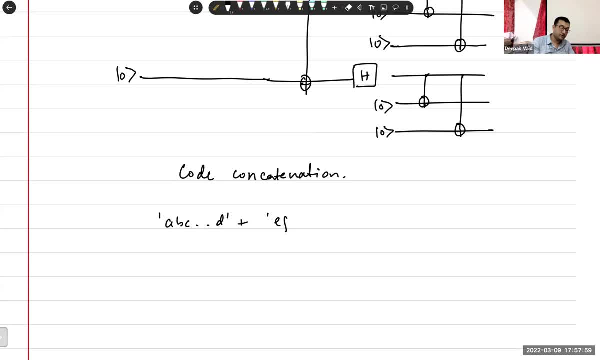 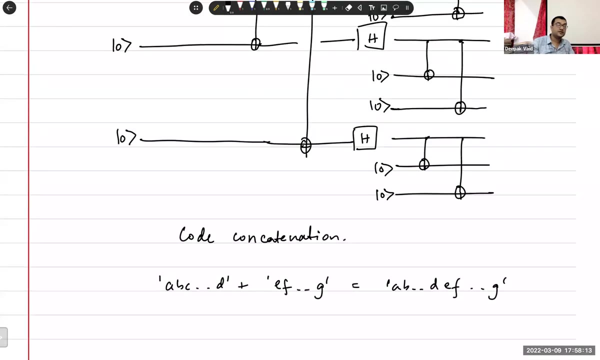 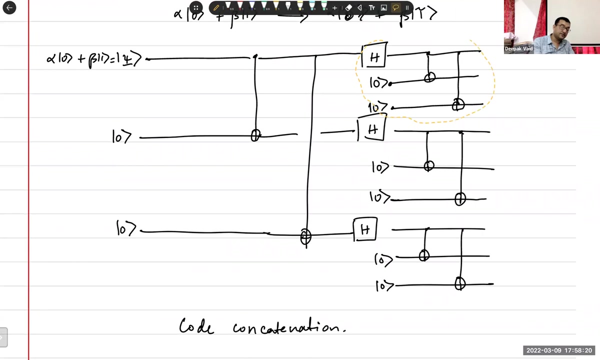 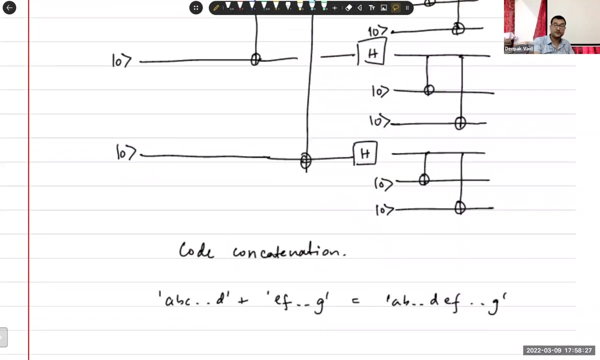 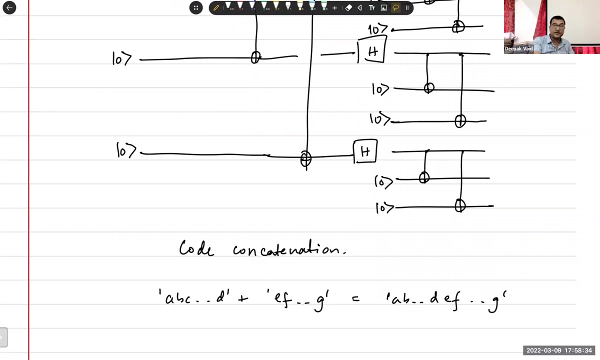 in computing and you want to join them together. That process is called concatenation. Of course, in this case, concatenation has a slightly different manifestation in that it is something that is happening as a nested procedure rather than as a linear procedure. So rather than concatenation, I would call it something else. I would call it, maybe, nesting. 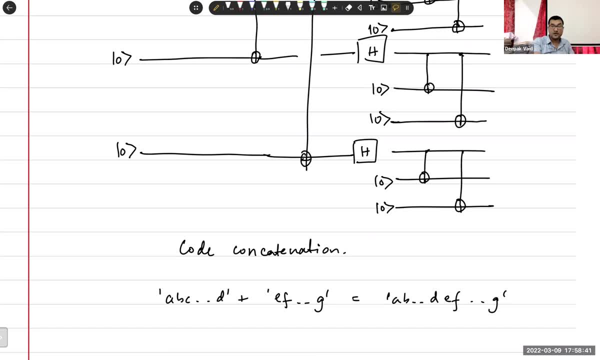 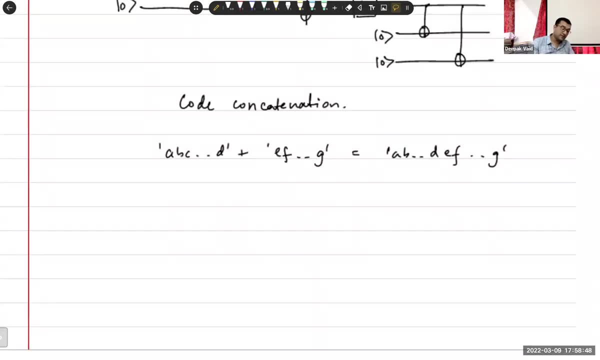 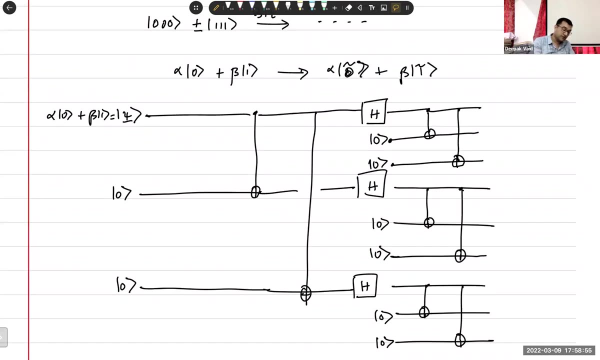 or something else, But anyway. So now let's try to see what happens once again to this circuit. So as you come out of the first two CNOT gates, let's say you end up with cy1 over here and then we'll call whatever you get out here. 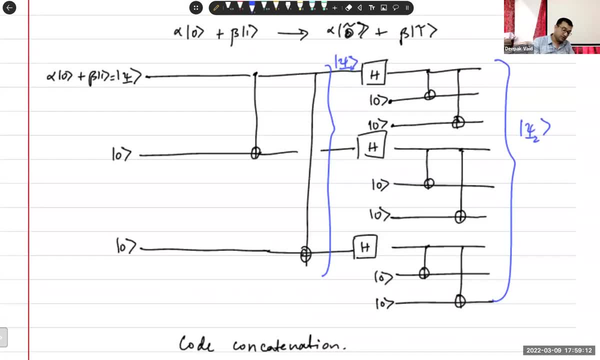 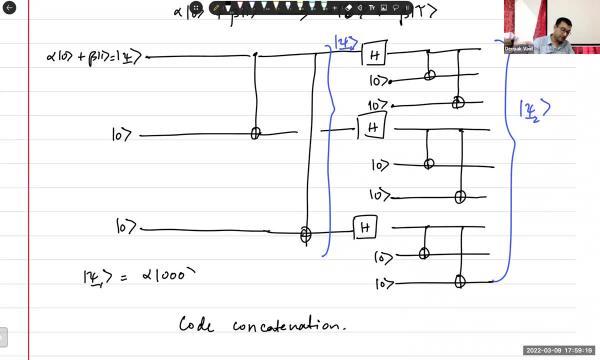 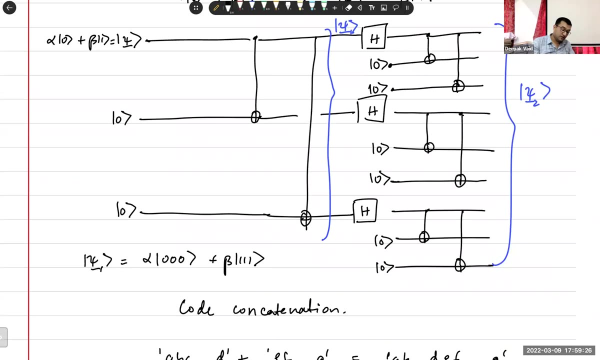 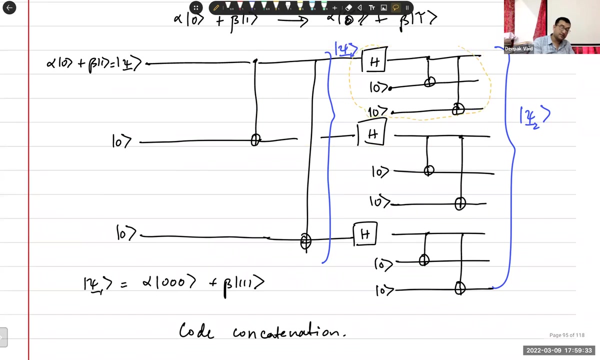 So the first one is cy2.. So cy1, right, of course we know what that is. that's alpha 000 beta 111.. Now, when we act, let's look at what happens with this sub-circuit. right, And this sub-circuit acts only on the first two. 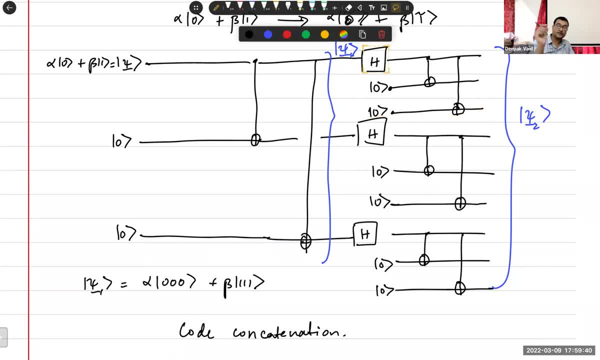 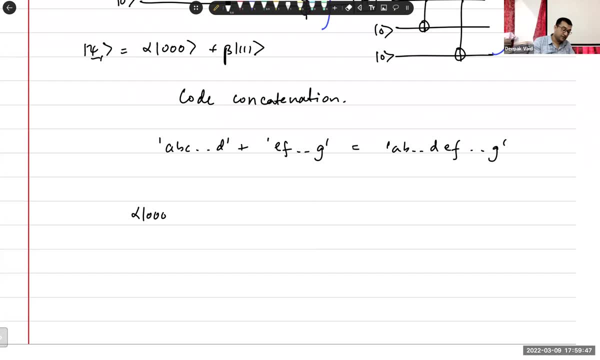 So alpha 000 beta 111.. So alpha 000 beta 111.. first qubit, and then it concatenates two more qubits, right? So we have alpha 0, 0, 0 beta 1, 1, 1, right. 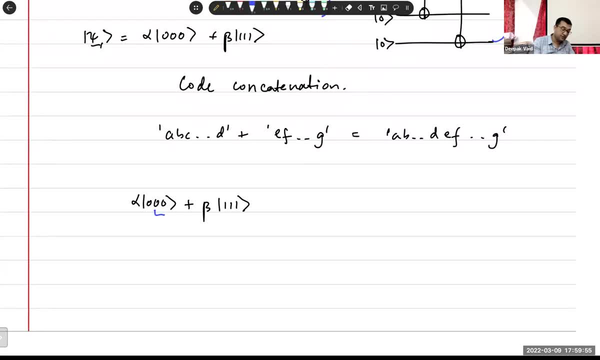 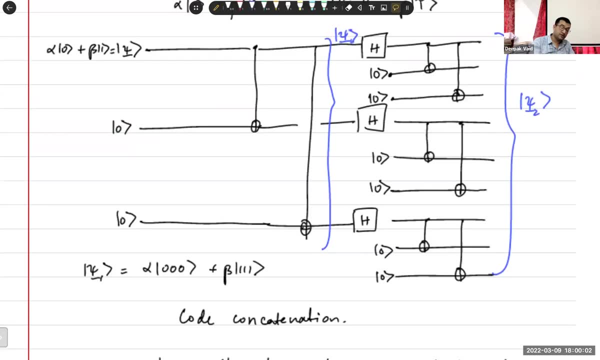 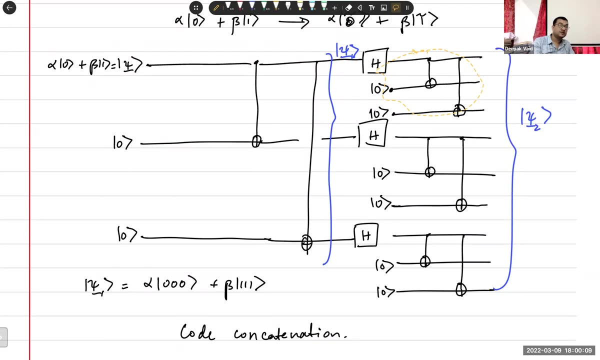 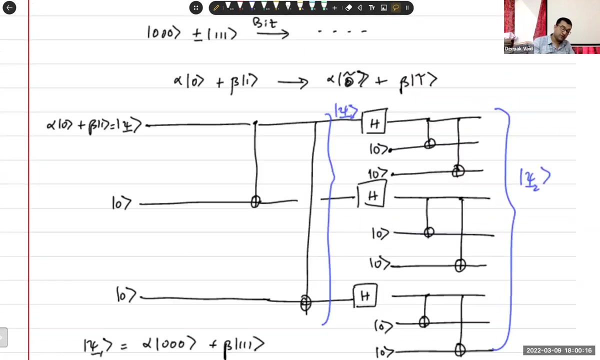 But we can just take these two qubits and put them aside for the time being right, Because these operations over here at the second level of this code will not affect the second and third qubit right. And so what will be the effect of this? 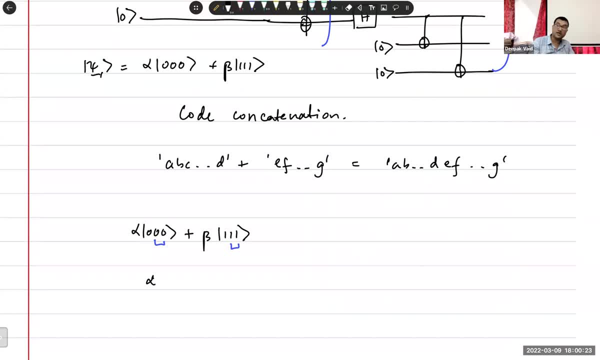 You will go from. if you apply the hard-amard, you'll go from alpha by plus beta, you'll go to the hard-amard basis. right, And now what I'm doing is I'm working only with the first qubit. I put the second and third qubit. 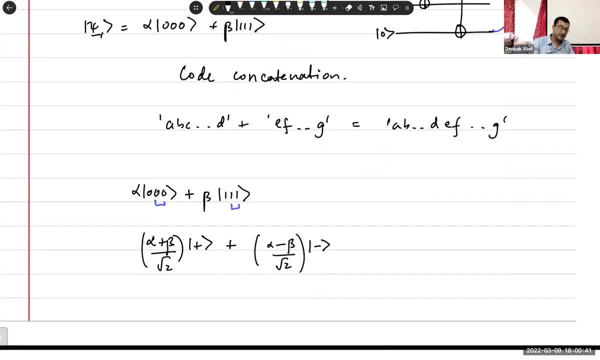 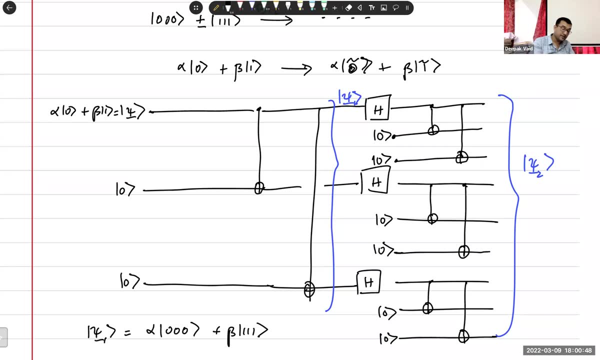 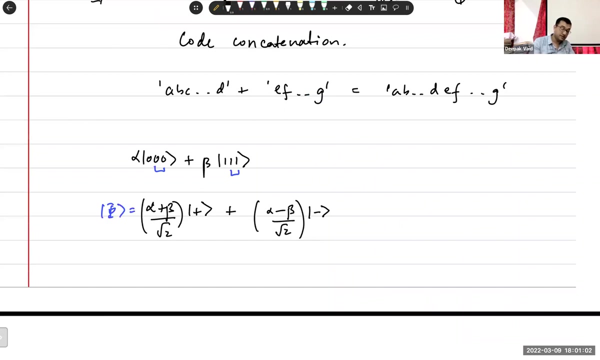 in hibernation, right, And then after this, hard-amard is applied. so let me call this state something else over here. Let me call it phi. This state is phi okay With qubits two and three. if you look at the guy in the top. 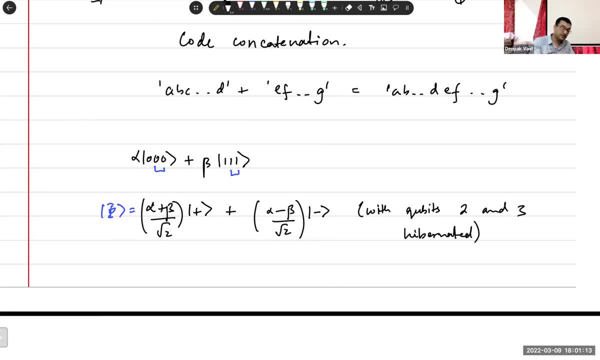 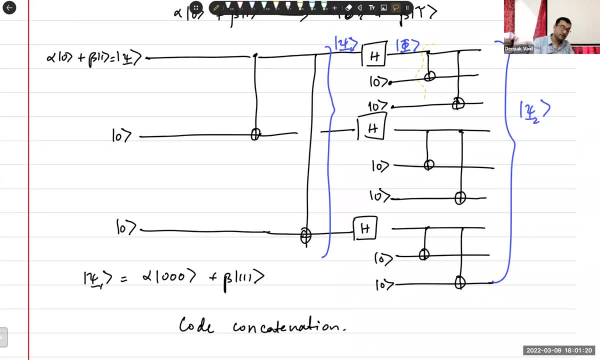 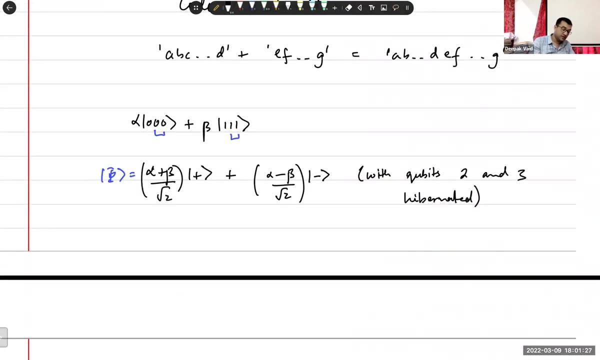 this is the same take. put: he is in hibernated, Okay, Meaning they are there, we're just not worried about them. We know what the state is. And then, once again, we are applying the CNOT gates. What will happen if you apply the CNOT gates in this order? 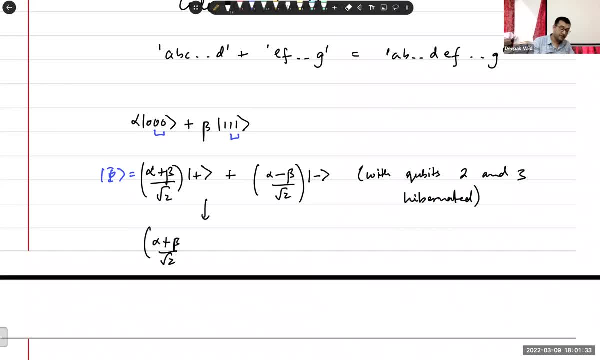 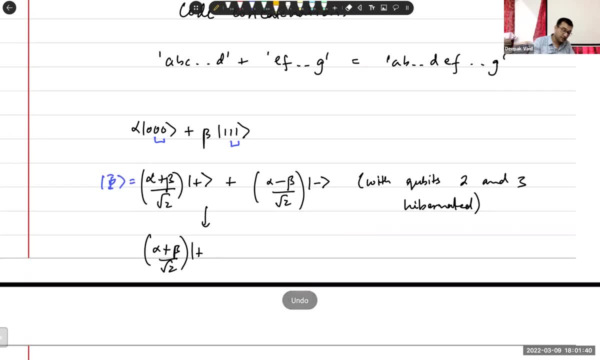 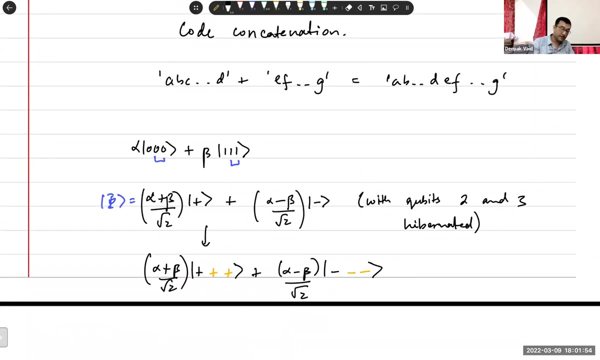 We will get alpha plus beta, by root, two plus. and now I'll just type it, And now I'll just put the other two qubits in a different color, Right, And what are these two qubits that I put in a blue color? 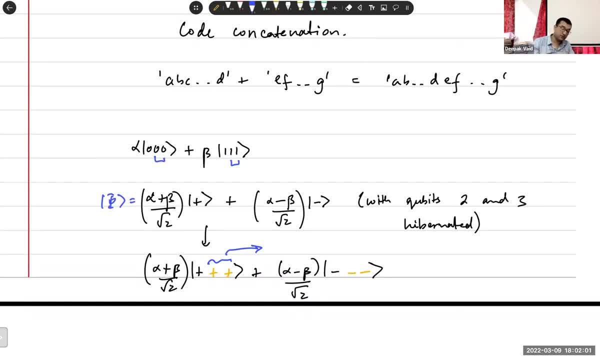 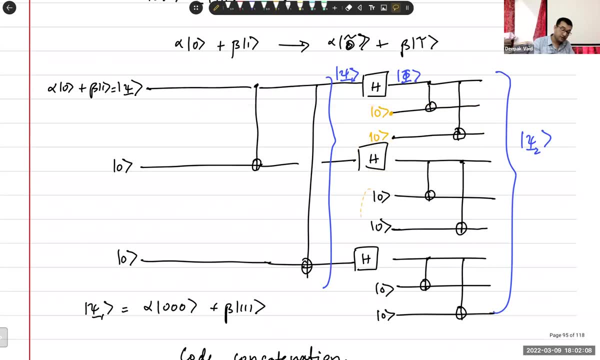 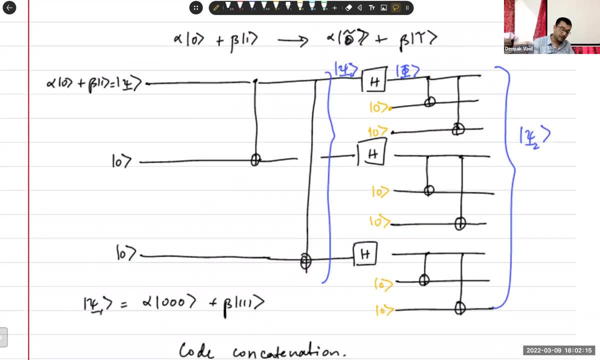 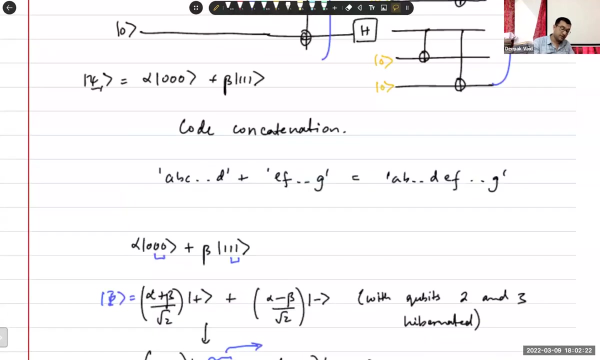 These are my, my second level over here. Right, These qubits which I've introduced At the second level of my code. This is what I'm writing with the with the orange color. OK, So This is what happens to the first qubit, right? 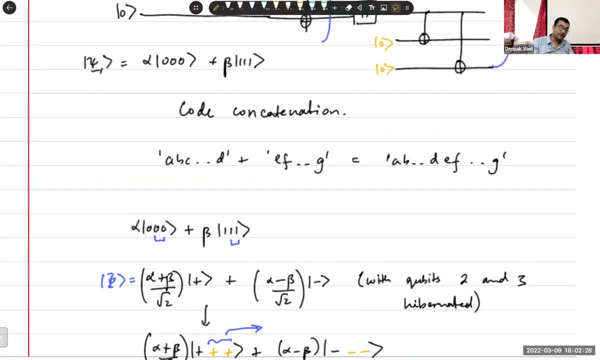 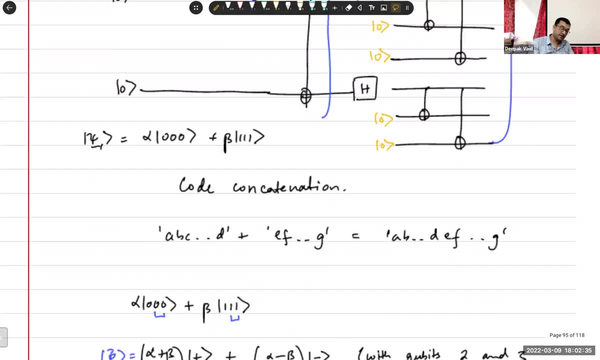 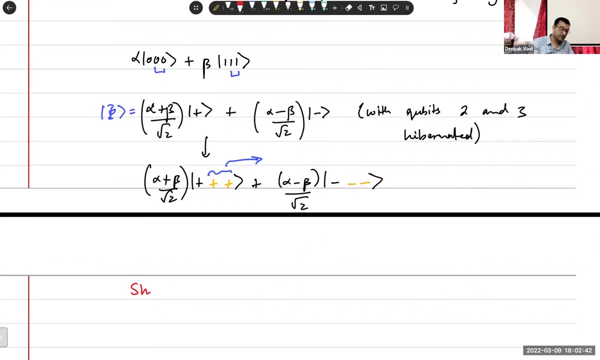 The same thing happens to the second qubit in the in the middle, And then the same thing happens to the third qubit, again in the middle Right, And I'll leave it as an exercise for you to work out to show that The circuit Works as intended meaning. 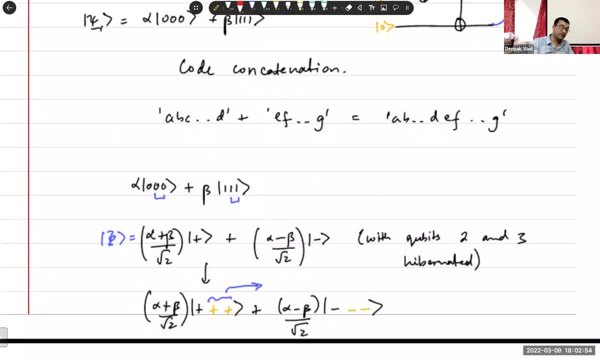 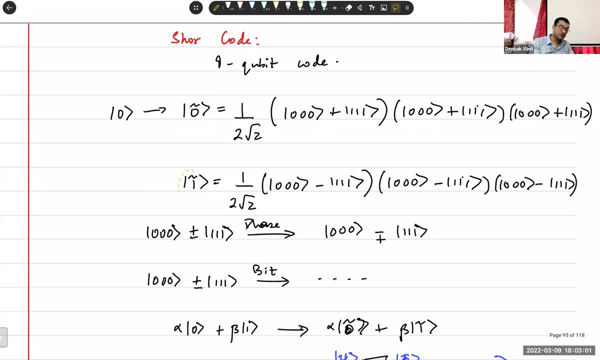 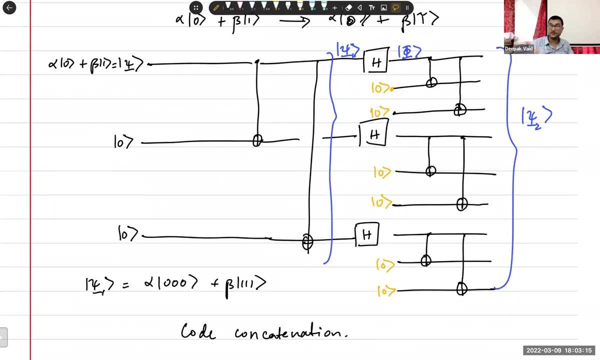 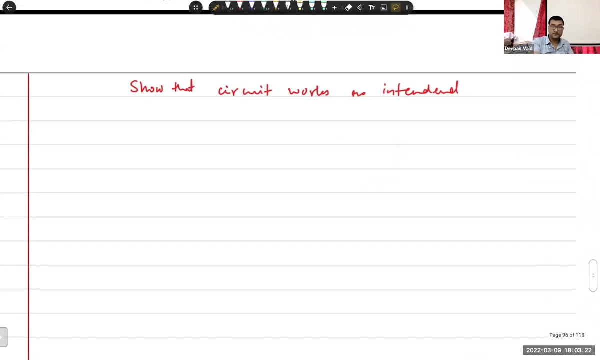 That it takes our state alpha plus beta and returns the state alpha Times, logical one and logical zero, Where logical zero is this state and logical one is this. OK, But I hope that you all can, look at this, Feel reasonably confident, from what you know so far, that this will indeed be the case. 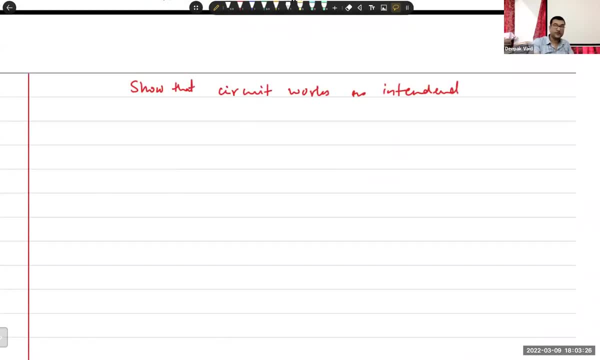 But it's not completely trivial. So you should definitely sit down and work it out, because there are all kinds of signs, Pluses and minuses That one should take into account. OK, So now, What about? how do we perform the? 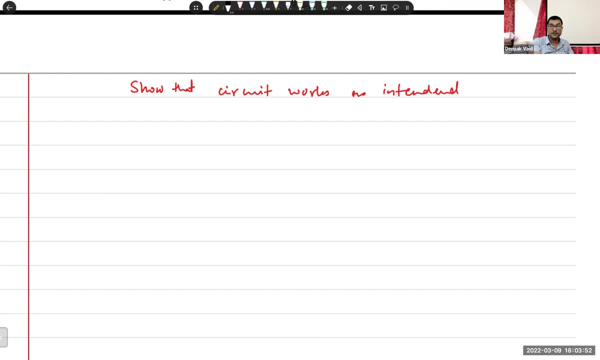 The error recovery. Right, How do we? how do we do the error recovery? So let's say that there is a bit flip error On the first qubit, OK, So if there is a bit flip error on the first qubit, 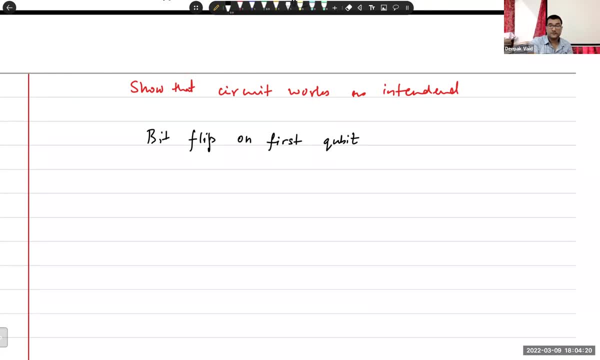 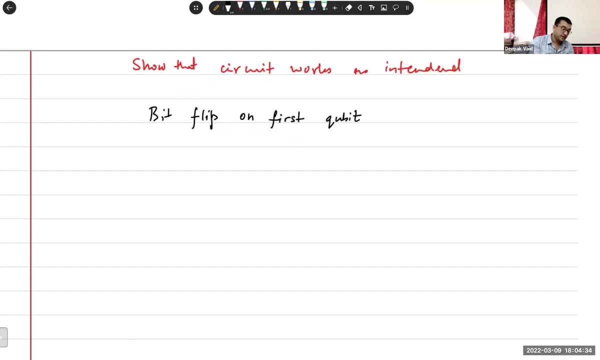 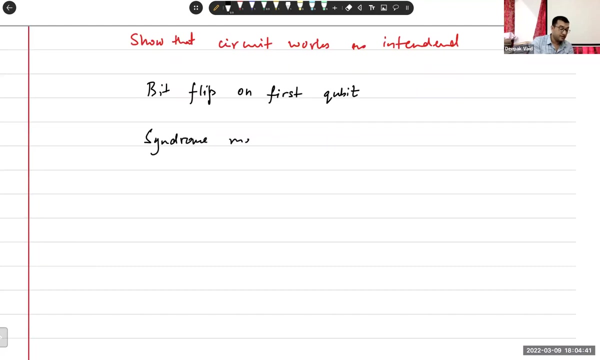 We OK. So before that, actually let me go back a couple of steps and Tell you a little bit about The syndrome measurement From a slightly different perspective. So I skipped that part. Let me go back to that. So we'll go back for a for time being. 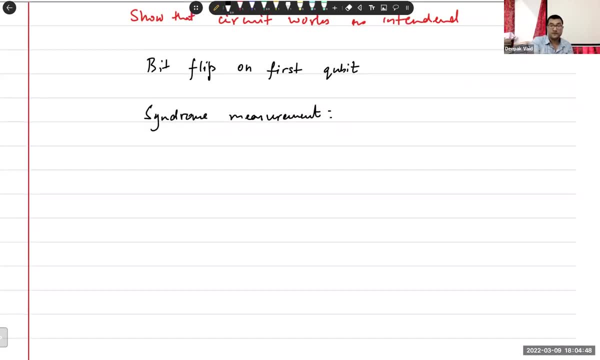 To our three qubit code. So We remember that you have these three, these three projectors, Right For the single bit flip. Now, Instead of using these projectors, let's say that we use a different set of observables. 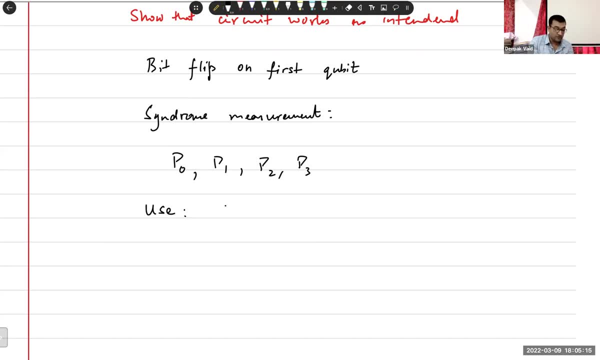 OK, These observables are as follows: Z1 and Z2.. Z1 product, Z2.. Now, whenever I have An expression of this form, What does this actually imply? Z1 is acting on the first qubit. Z2 is acting on the second qubit. 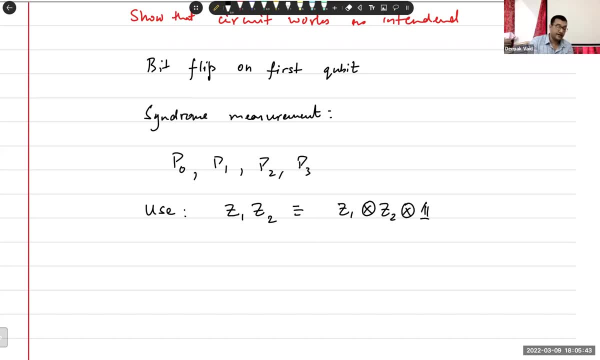 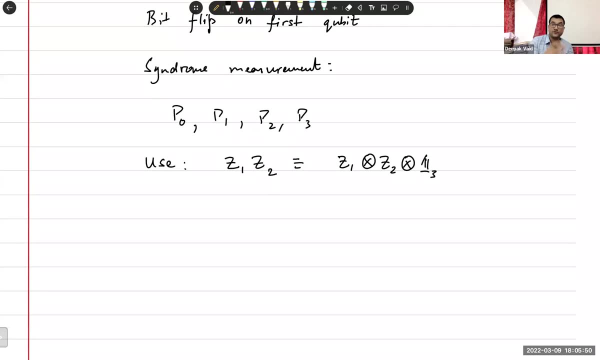 And what is acting on the third qubit, Identity. OK, so we'll be using this kind of an of notation. So, for instance, Z2, Z3. Will be I identity, Then Z2.. Then Z3, and so on. 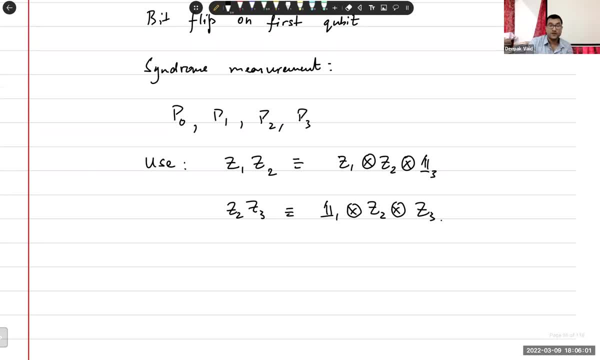 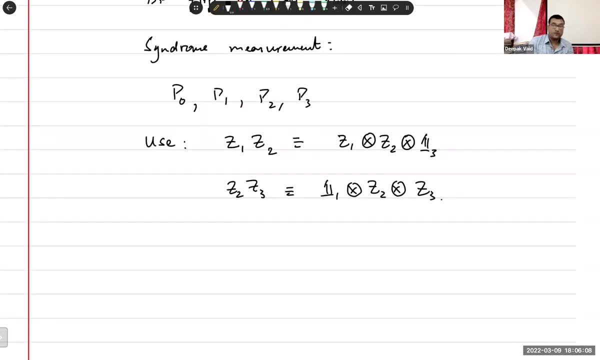 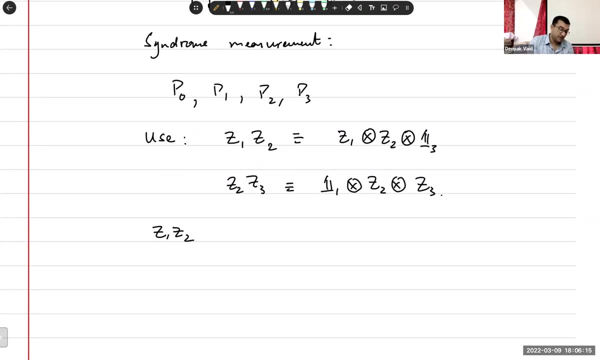 OK, Now If you ask what is the eigenvalue of this, of this observable Z1, Z2.. OK, so just to be Just for the sake of clarity, I'll put a one at the end. OK, To indicate that fact that this is a three qubit operator. 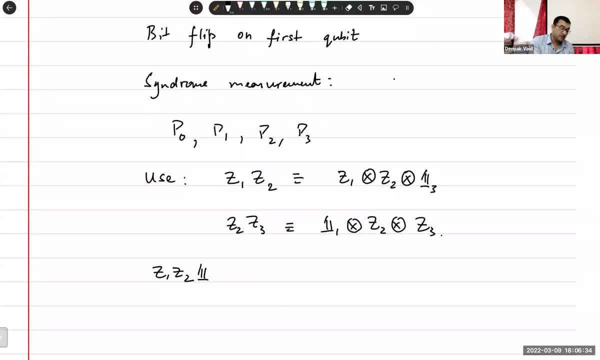 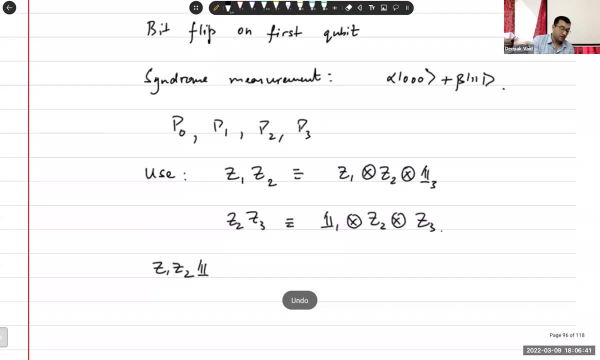 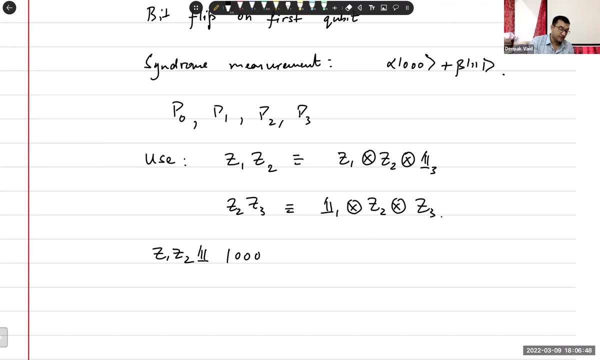 And now we are going back. We are talking about our Three qubits. So If I ask, what is the eigenvalue of this, of this operator, Right, What are the possibilities, What are the possible eigenvalues? What is the eigenvalue of the Z operator? 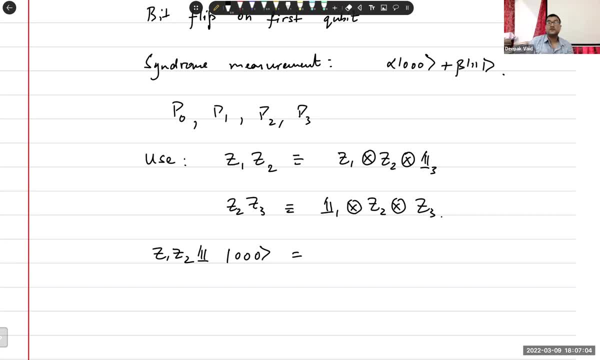 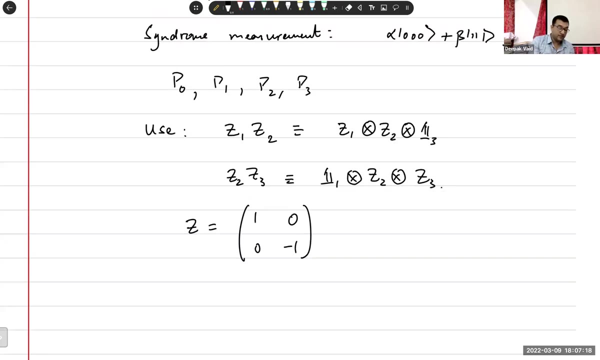 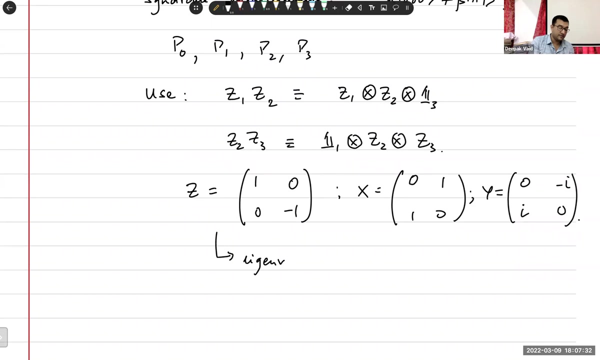 On a single qubit. The Z operator, poly Z operator: One zero, zero. Poly Z operator Is one zero. No forget about the H bar. Just One minus one, Two. So the eigenvalues of this of the Z operator are one plus and minus one. 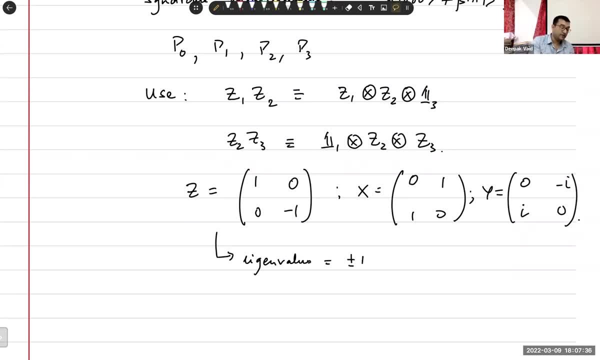 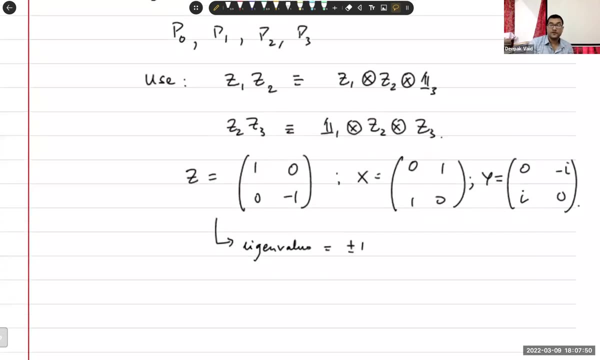 Right. So what will be the eigenvalues of any product of Zs? It can only be plus one or minus one, Right You can. you will have some combination of pluses and minuses that we give you at the end, Plus or minus one. 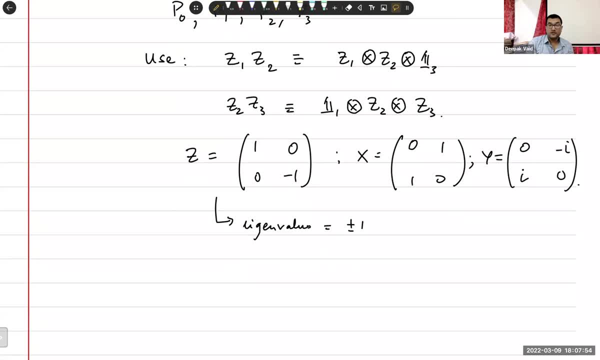 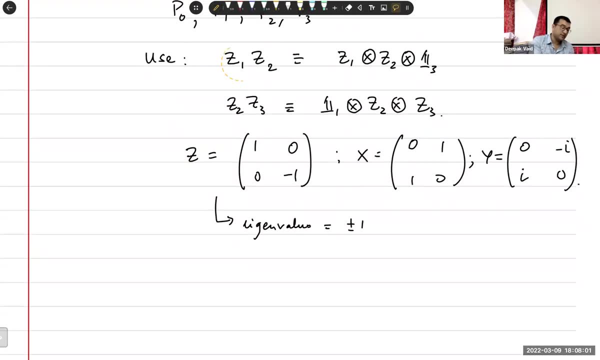 So So let's say that we have, We use two of these observables. We use Z one, Z two, And then we use Z two, Z three, And we perform a measurement of both of these, Right? So this? 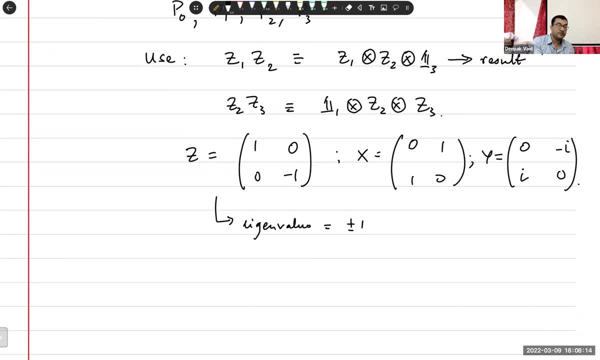 This gives us as a. as a result, if you perform a measurement plus or minus one, This gives us an eigenvalue: Plus or minus one, Plus or minus one Right. So each one of these is giving us a single bit of information. 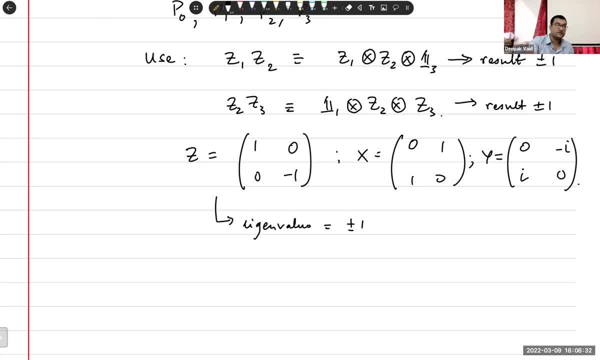 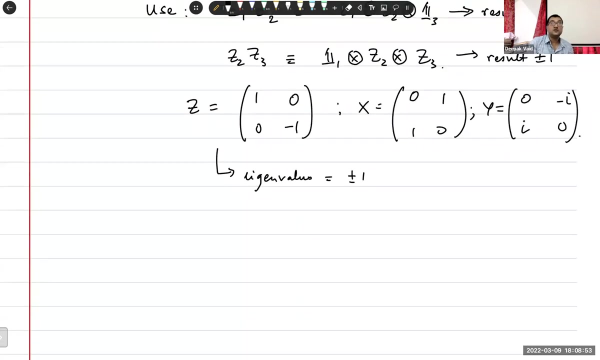 What's up? Can you just Go and, like, Tell those people to quiet If they're still there? Or, Okay, Go and shout at them. Yeah, So Which one? Sorry, Like We need, We have to be. 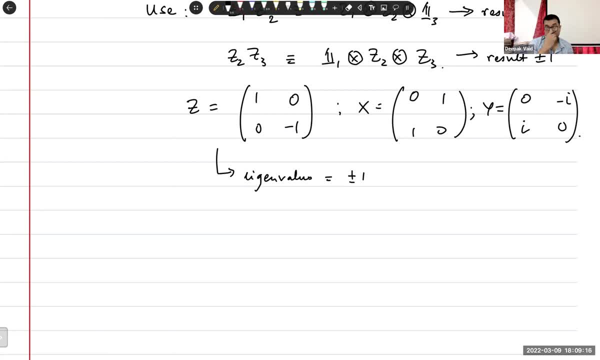 Right, You One, One Space Space, You No, No, No, Yeah, We don't want to know. how does it If we just- Okay, I can just, And You No, No, So you. 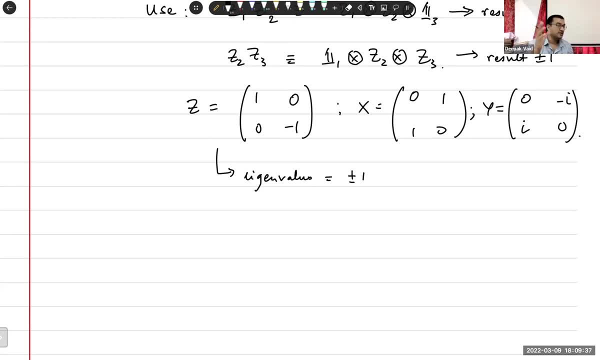 You. You cannot do P1. P1. Tencer Identity. P is Already a three qubit operator. So if you take P with tensor identity, How many qubits are you active on? Nine, No, So we are not talking about the nine qubit code. 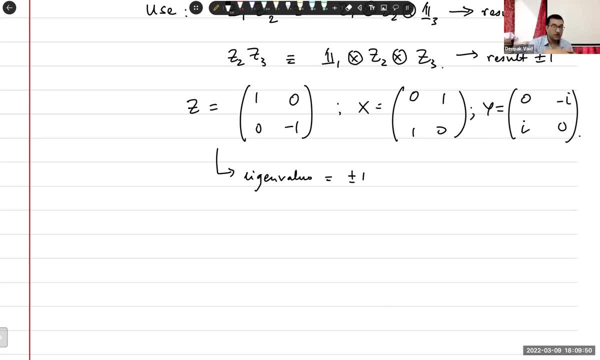 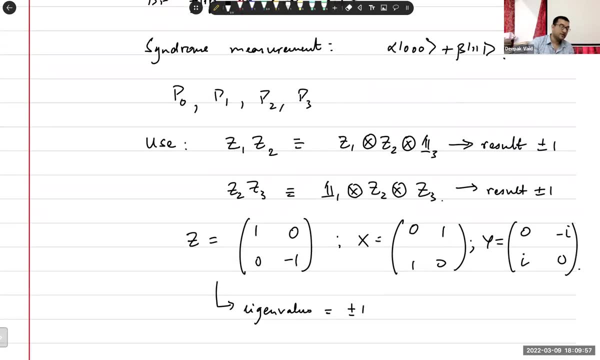 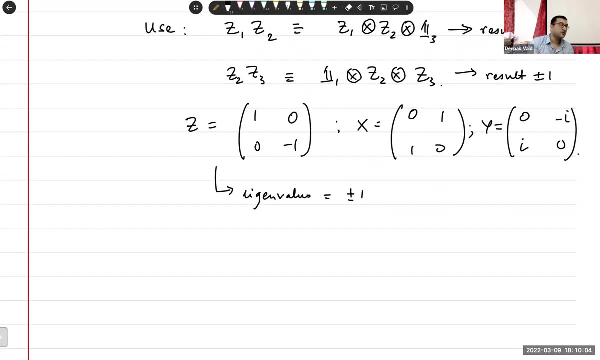 Yet code. yet We're talking about the. we're looking at this three qubit case and, instead of looking at these projectors, I'm talking about doing measurements on a different set of operators And then in the nine qubit case, because this will lead to a simpler way of doing things. 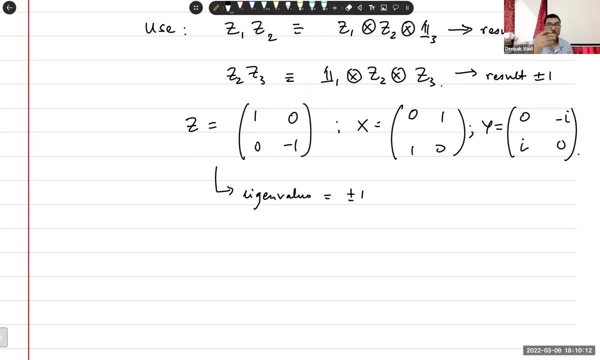 what you are saying is technically correct, right, That in the nine qubit case you can construct a set of projectors, as you said, which goes as a PI, tensor identity on three, tensor identity on three. But there is a simpler way of performing the measurements, Okay. 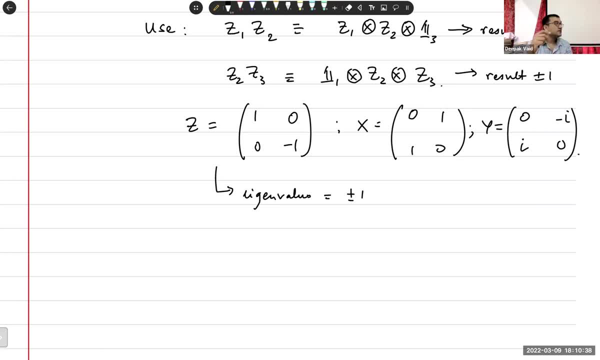 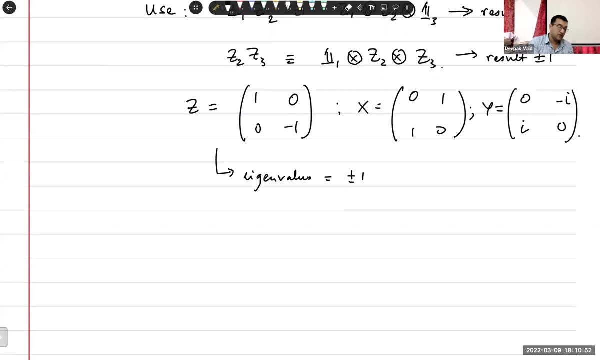 So the reason for this would be: well, we'll see as we go, Okay, But yeah, technically I mean, I suppose you are correct Now, and so these are called polys, by the way, These are known as these are all the poly gates, but when we talk about them, multiple strings. 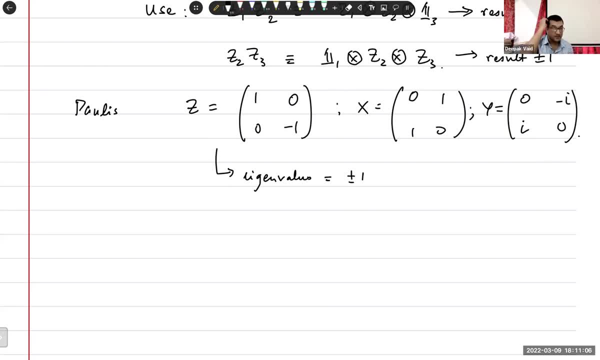 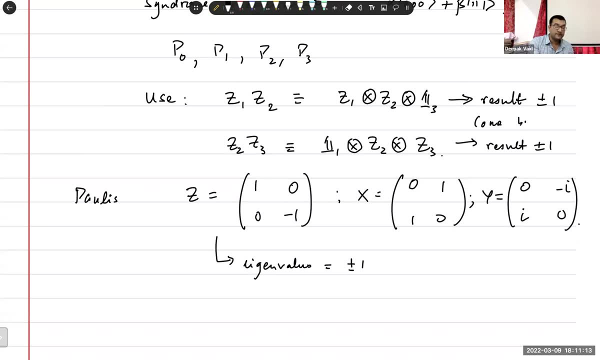 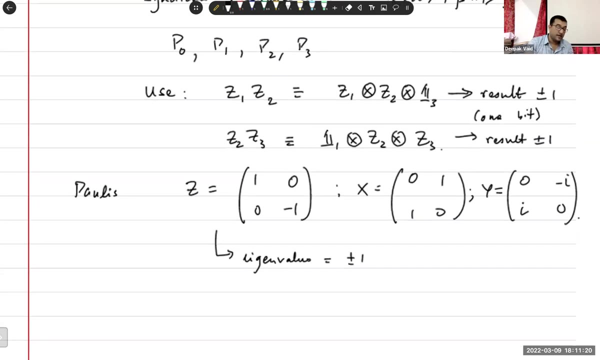 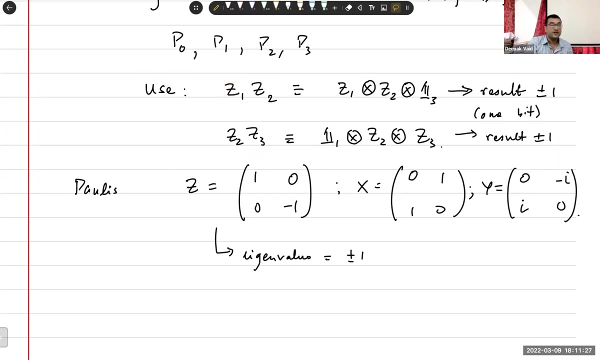 of such operators. we call them polys, And each such poly is giving us one bit of information, right? Because it's plus or minus one. So that's one, one classical bit of information, right? So if you make a measurement of two such operators, what do we get? We get two bits of information. 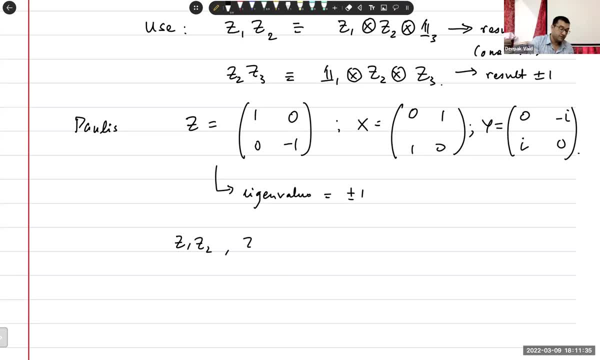 right. So Z1, Z2, Z2, Z3 together gives me two classical bits of information about the state right? Okay, That means I will get two classical bits, means I will get four possible outcomes right: 0, 1, 2, 3.. 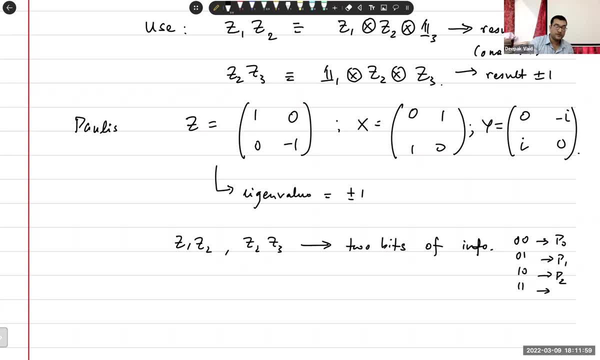 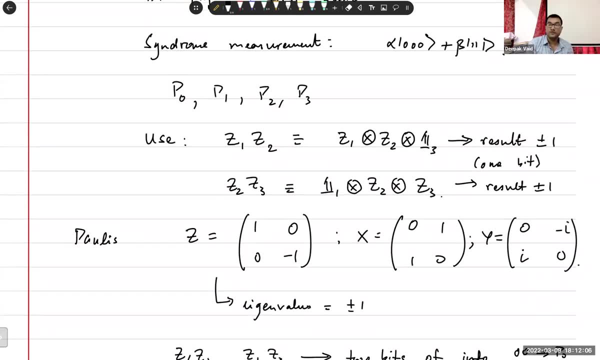 These can be put in correspondence with each of the syndrome measurements: P0,, P1,, P2, and P3,. right, Because P0,, P1, and P2, and P3, their measurement gives me either 0 or 1, right. 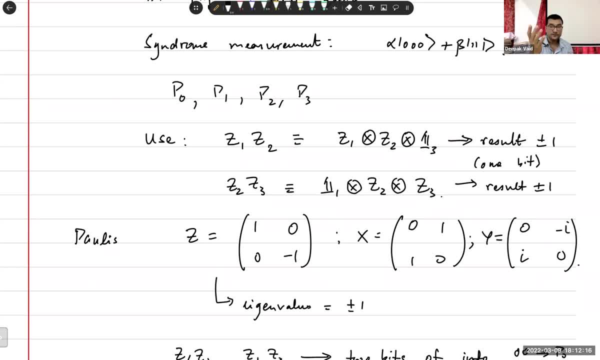 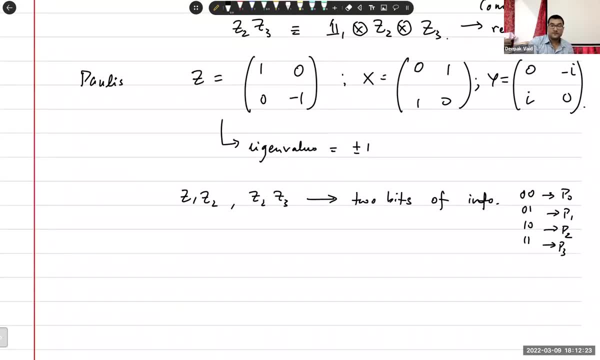 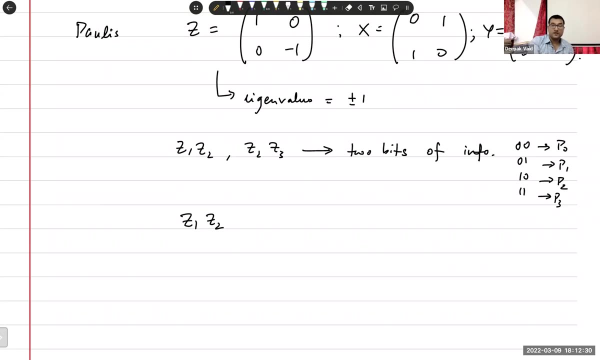 And there are four such values right Now. this first measurement, Z1 and Z2, what is it? Why are we doing it? What does it tell us? physically? It basically says that what we are doing is compare the first and second qubit, okay, to see if they are the same or not. 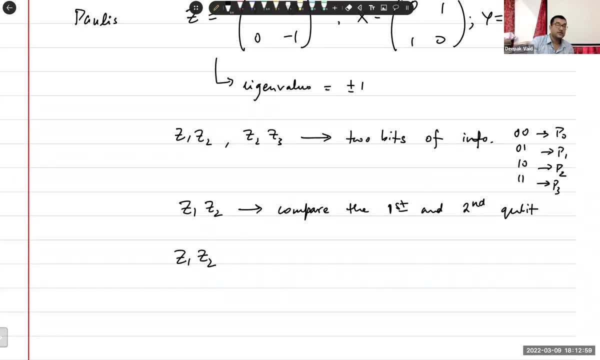 Why is that the case? Because let's take Z1, Z2, and act on the state 0, 0, 0, or on the state 1, 1, 1, right, What will be the eigenvalue? 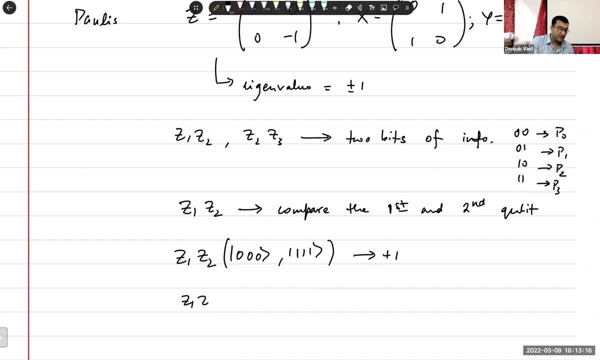 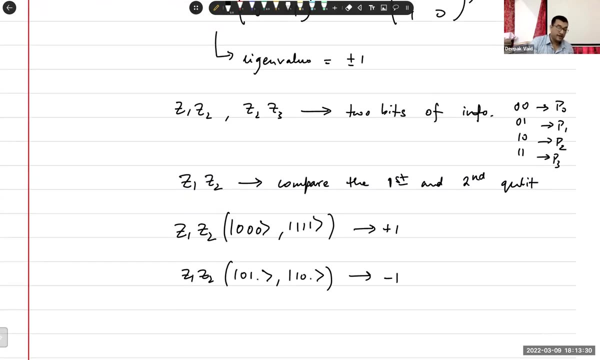 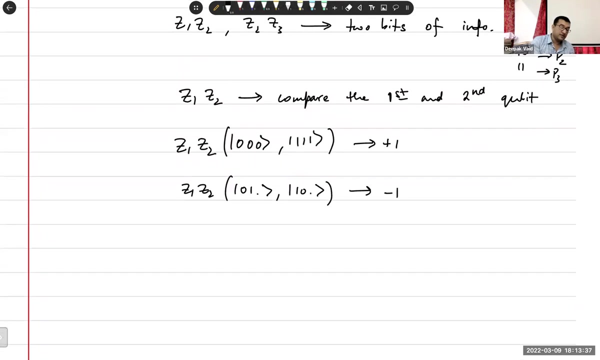 It's plus 1.. And if the first two qubits are different, right, then the eigenvalue will be minus 1, right. So the result of Z1 and Z2 gives us a comparison of the first and second qubits. 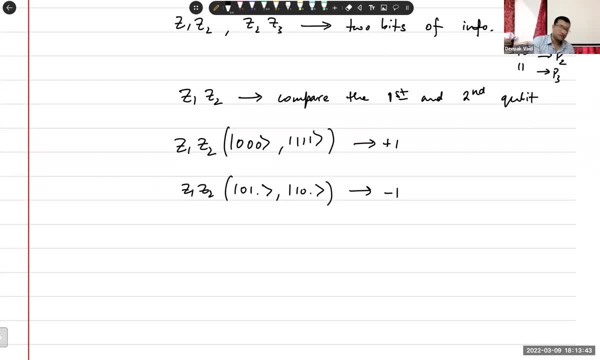 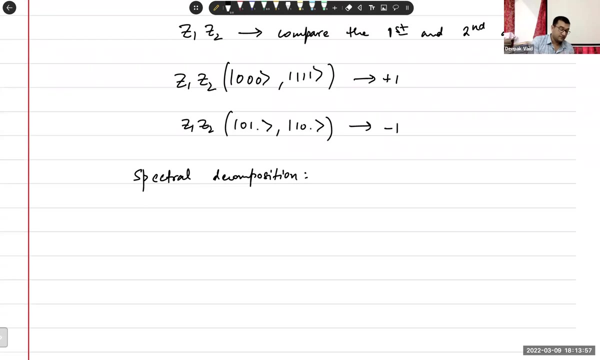 We can also. Okay, So we can rewrite, we can ask: what is this spectral decomposition of this operator, which will give us the same information, but in a slightly more mathematical expression. So, first of all, what is the Z operator? 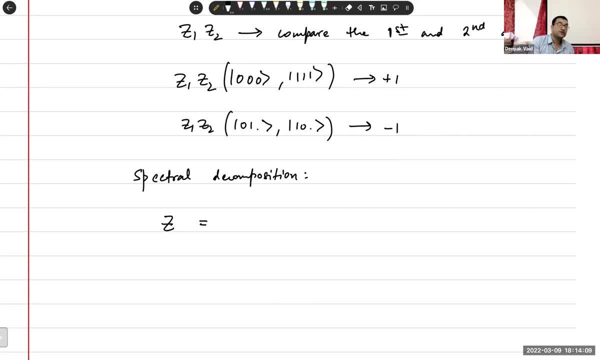 The Z operator can be written as follows: in terms of projection operators: right. What is it? Does anybody remember? So if I want to write Z as a sum of projection operators, what will it be? Right, 0, 0,. then minus 1, 1, right. 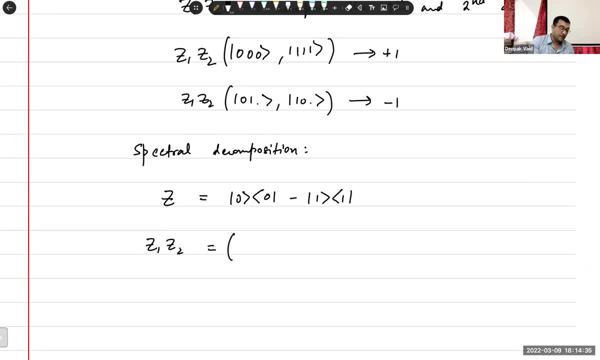 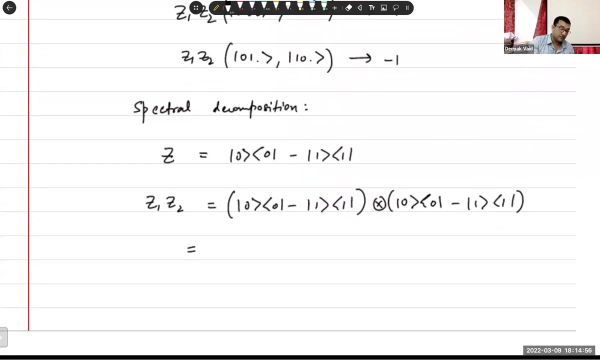 So Z1,, Z2, I can write as this, only Okay, And then Tenser with the same expression. but now, acting on the second qubit, Okay, And I'm not putting those indices because that will take up too much space. 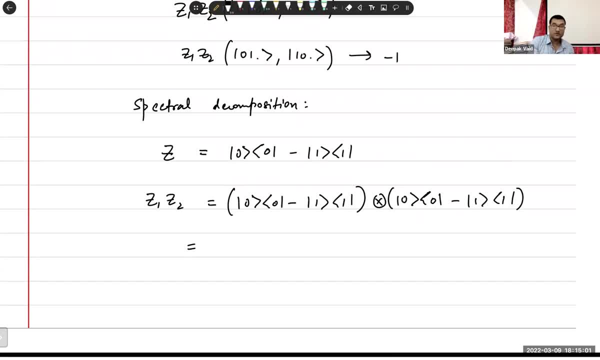 So when you tensor all of this out, right, what will you get? You will get 0, 0, 0, 0, right. So if you look at the first two terms, for instance, that will give you this: 0, 0, 0, 0. 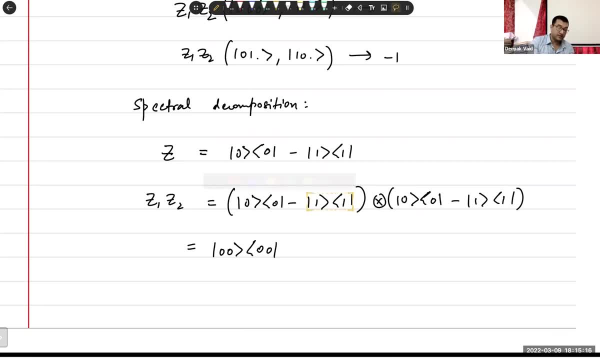 Then you look at the second terms: 1, 1,, 1, 1,. that will give you plus right. Then we can write that as: and then all of this is tensor with the identity. on the third qubit. 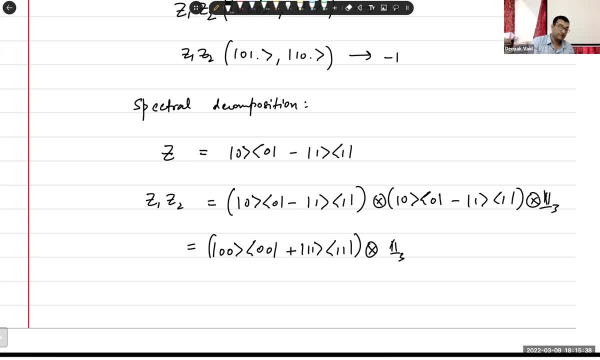 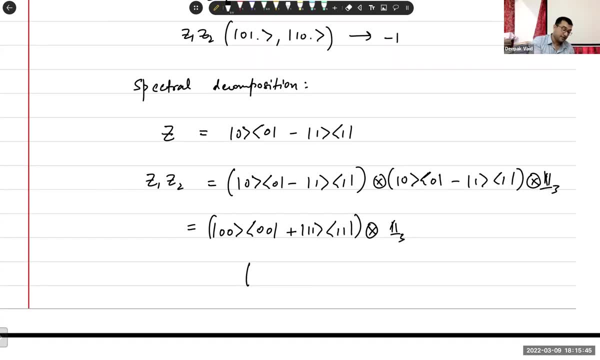 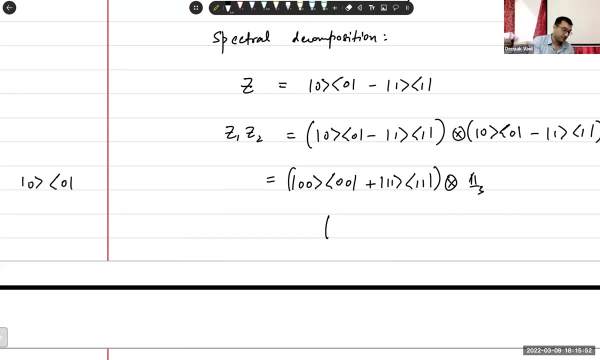 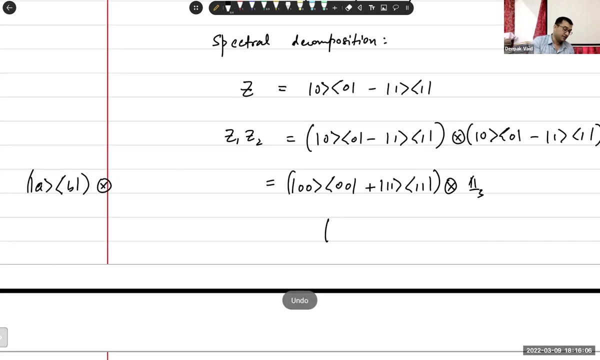 So we'll put a identity here on the third qubit And then we'll get two other terms. What are those two terms? So I hope that you can see, just to clarify that when I take this 0, 0, and I tensor it, or to be a little bit more general, I guess if I take A, B and I tensor it with C, D, what do I get? 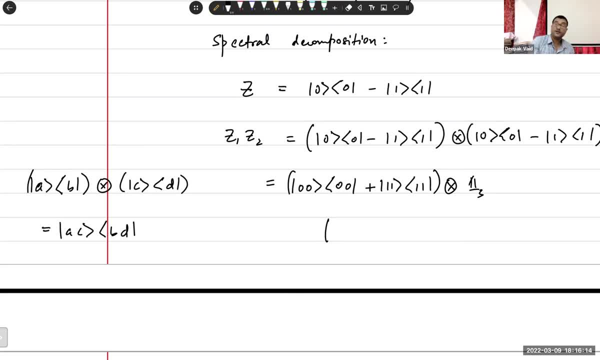 I get A, C, B, D, Okay, Where A and C act on the first qubit, B and sorry- A and B act on the first qubit, so they're in the first slot, And C and D act on the second qubit, so they're in the second slot. 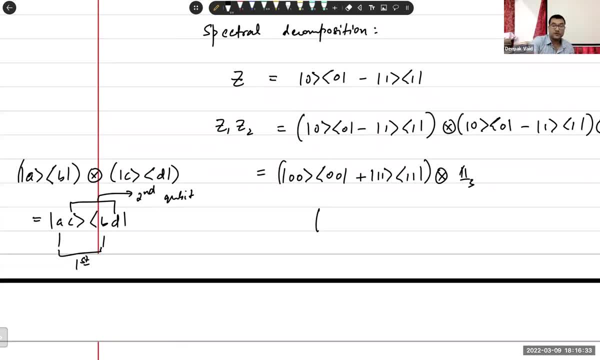 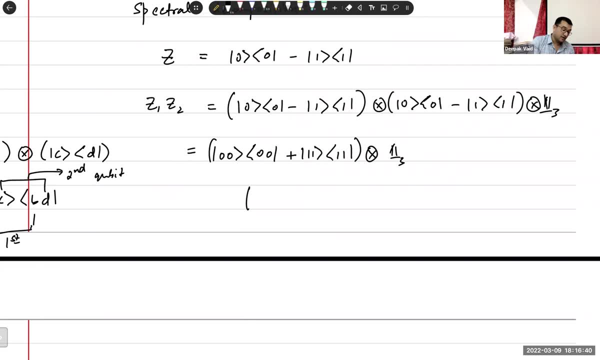 Please make sure that you get this notation. If you don't, you know there will be. you will face confusion later. Okay, So we get these two. So we get these two terms, and then the cross terms will give us what. 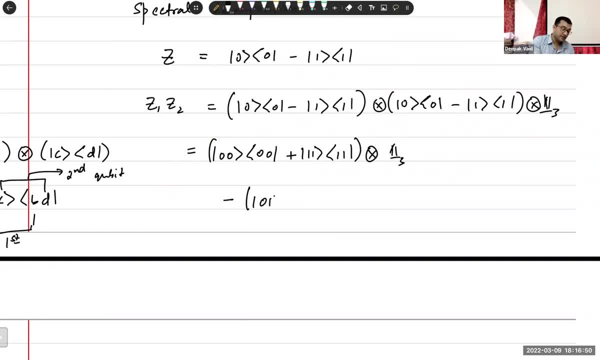 The cross terms will get a minus sign. then we'll get 0, 1, 0, 1, then 1, 0, 1, 0,, like this tensor. So this is Z1, Z2.. 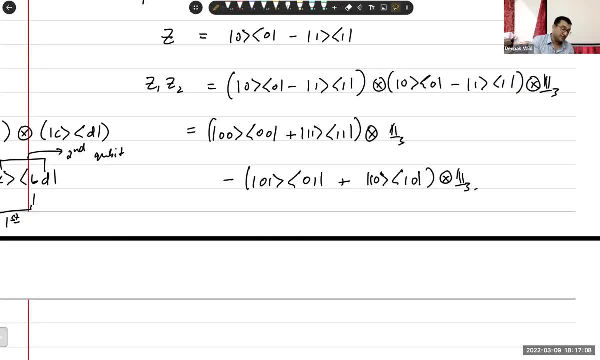 Okay, And we can see that it is a sum of. we can think so: this is a projector And this is also a projector. This is the first term- is projecting onto the case when the first two qubits are the same. 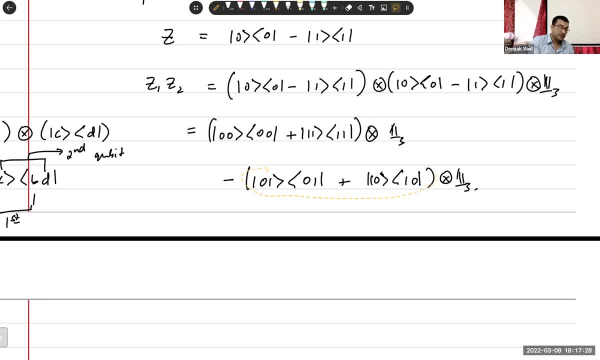 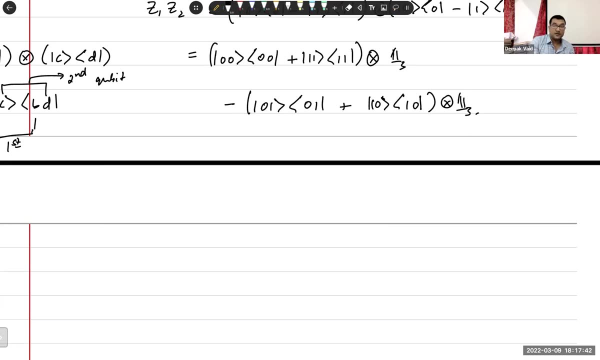 Right. So if the first two qubits are the same, the action of this part of the operator on the state will be 0. And if the first two qubits are different, right, So these are projectors. Okay. 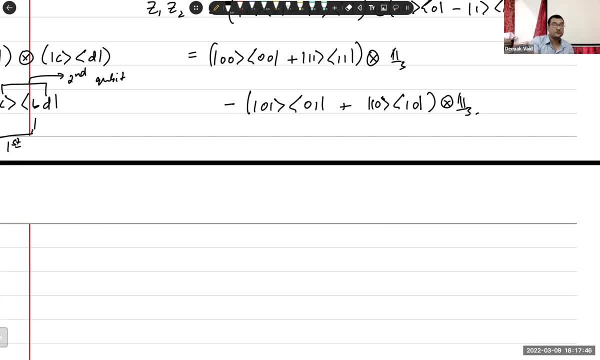 So, in this sense, Z1 and Z2 gives us a measurement of whether they are the same or not. Same thing for Z2, Z3, and Z1, Z2, and so on and so forth. Okay, Okay. 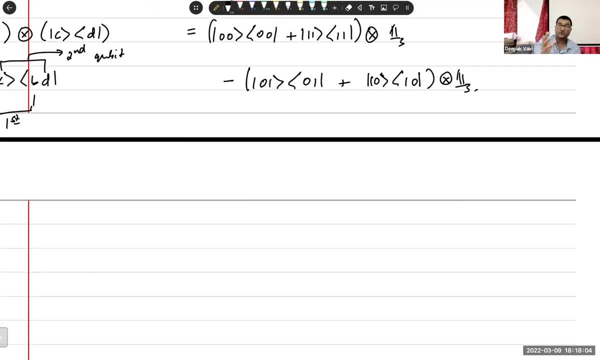 Now. so now what we can do is we can take these different sets and we can measure them in success. Okay, so let's combine one of these right. So let's say that we measure Z1, Z2, and this gives us plus 1.. 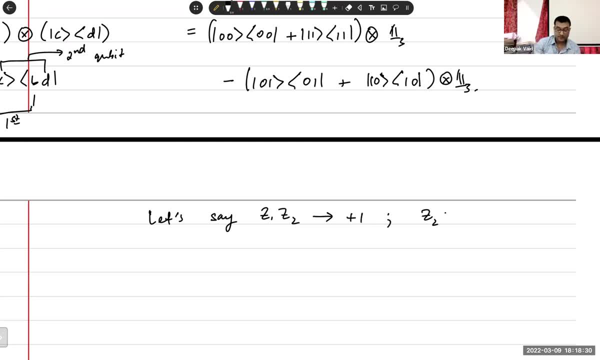 Okay, And then we measure Z2, Z3, this gives us minus 1.. What can we say about the state? What information does this tell us about the state? It tells us the same Third qubit, right, So we can say with confidence that it is the third qubit which has flipped. 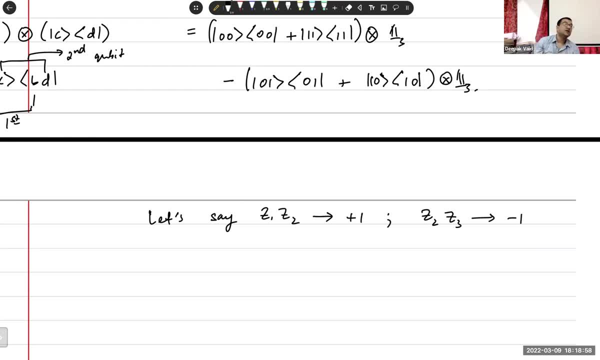 Right, Assuming what One qubit error, Because if there is a two qubit error, then you can again get the. well, you would actually need a Yeah, Yeah, Yeah, Yeah, Yeah, Yeah, You would need a two qubit error. 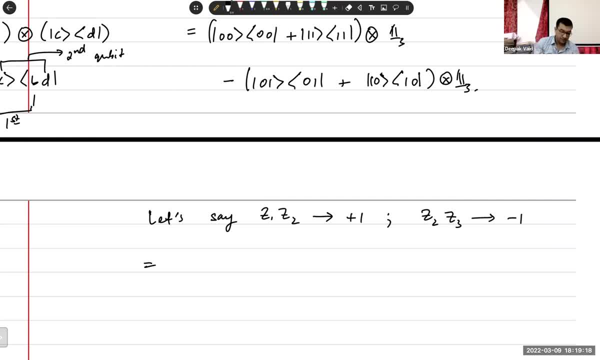 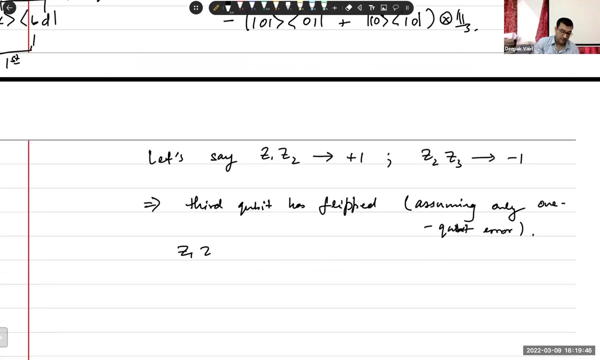 So, assuming there are no two qubit errors, this tells you that the third qubit has flipped. Assuming only one qubit error, Okay, What if both of these give you minus 1? Right, Then that tells you that it is Z2.. 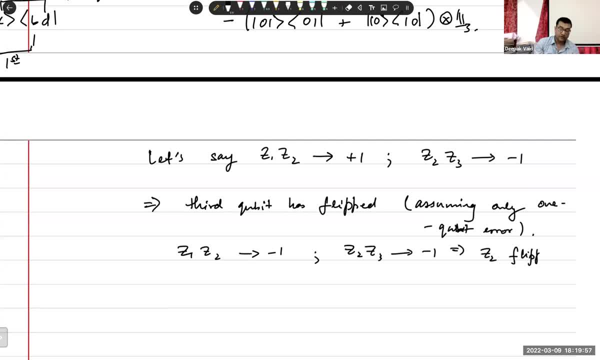 Right, Z2 has flipped, Or qubit 2 has flipped, Q2. Q2. Q2., Q2. Q2.. Now again, one might ask: in doing all these measurements, am I not destroying my state? 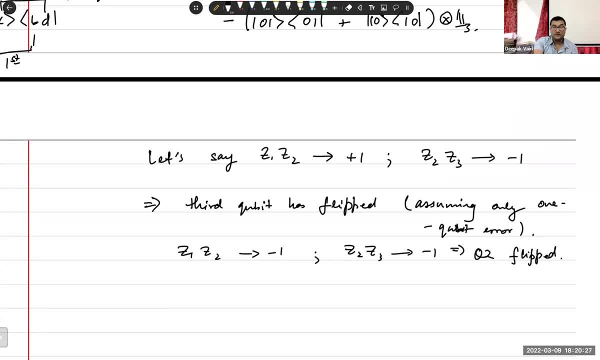 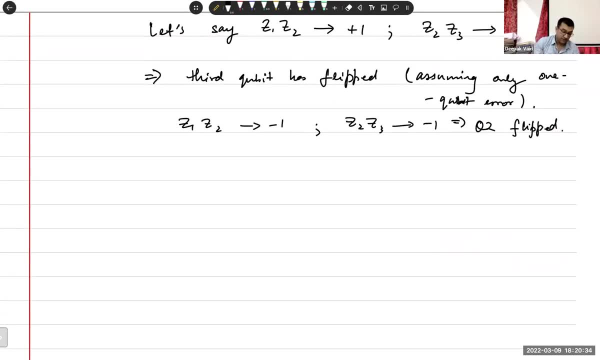 Okay. So let's look at what happens when you take one of these measurements and act on the state. Okay. Okay, So if you take, If you take Z1,, Z2, right, And you act on the state alpha. 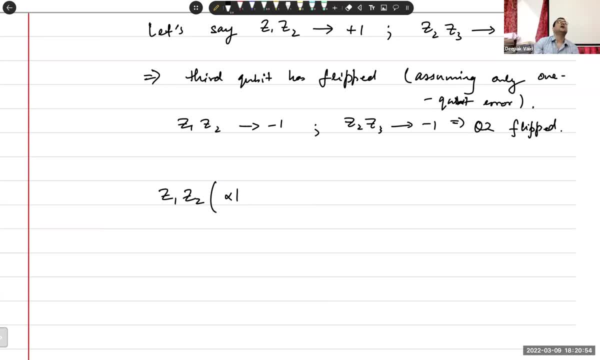 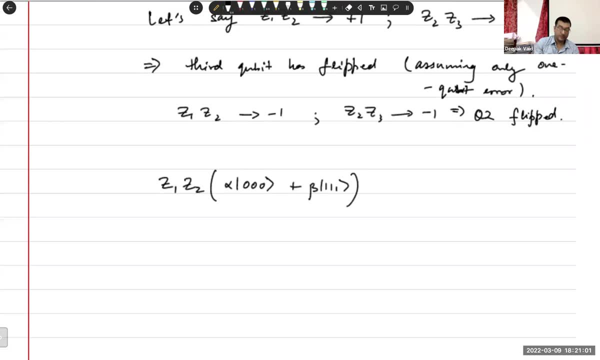 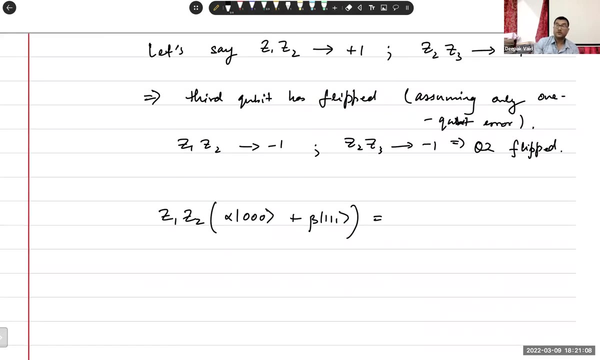 Well, I'll write it like: How should I write it? Well, let me just say 0, 0, 0.. Plus beta: 1, 1, 1.. Right, right, And what is the answer? This is an eigenstate of z1 and z2,, right? So if I act, 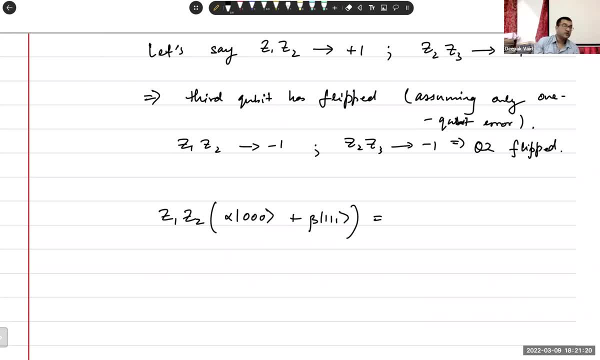 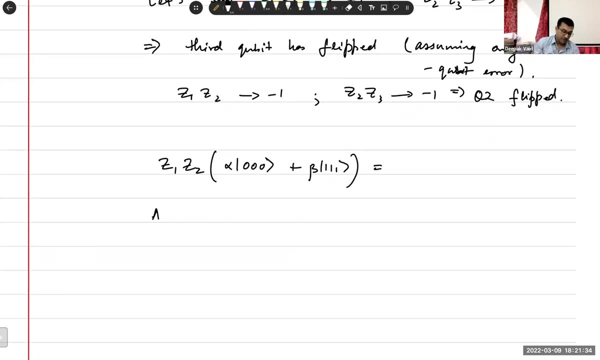 on this with z1 and z2, will the state collapse into something else? No, Why, Because it's already in an eigenstate of the operator that is being measured. So if you measure an operator A on some state, psi right, what does the measurement? 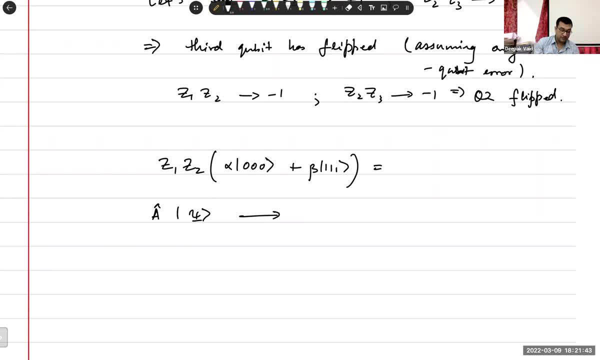 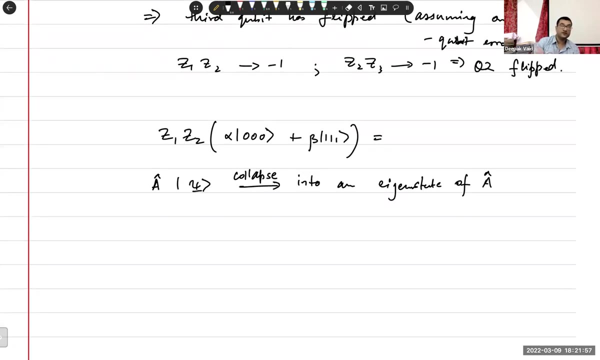 postulate tell you. Measurement postulate tells you that the state collapses into an eigenstate of A right, But if you are already in an eigenstate of A, then your state will not be changed. So this is the sense in which these measurements are not changing our state. Is this, Aditya? 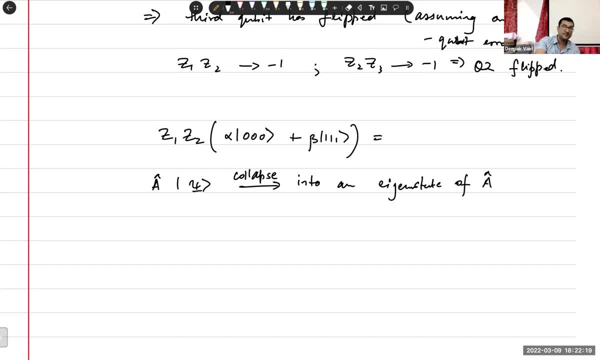 is this making sense? Little bit, Huh, Little bit, Little bit. no, That's why I could feel that there was a disturbance in the force. Yeah, Yeah, Yeah, At this stage, Star Wars is also so old that none of you get these, get these references. 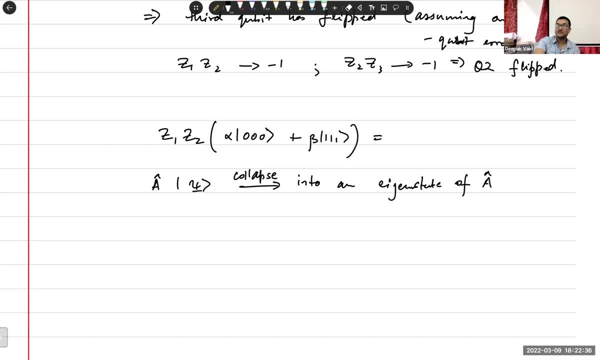 right, It started in the… Right. These days, I mean the Fast and Furious references, you might have understood them. That too, I mean, has become a classic. The art form, Hmm, The art form, That too, I mean has become like Ramayana, right In in in, maybe like the 20th version. 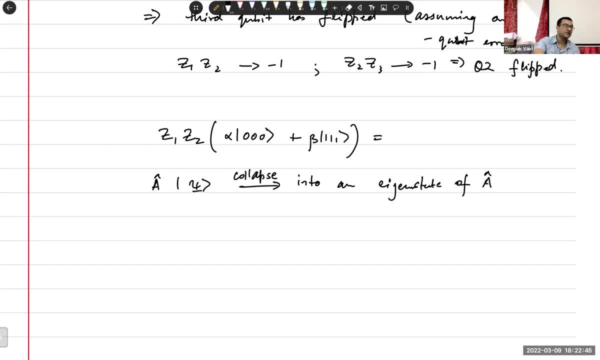 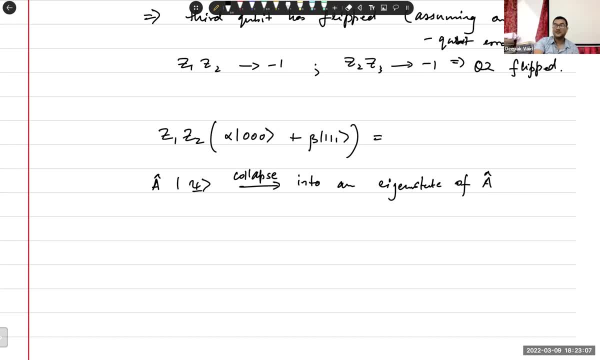 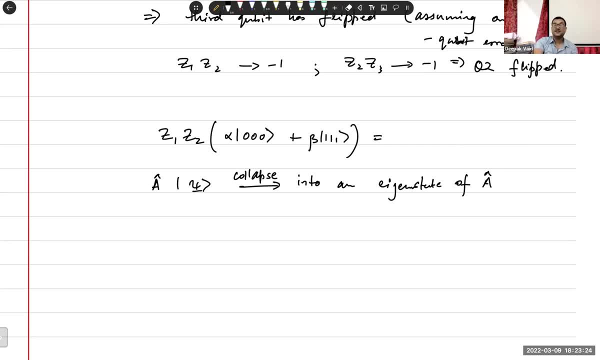 Yeah, Yeah, Yeah. A person should be able to help this one. What happens when you measure an operator A on some state side? It's that its state collapses into the eigenvector of that Eigenvector of that state A of that operator A. Now, if the operator A is Hermitian? 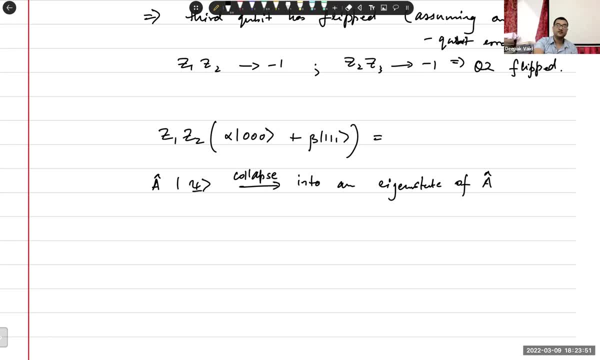 what can you say about the eigenstates of that operator? It's real and positive, Right. but what about the eigenstates? The eigenstates? they can be made orthogonal. They are orthogonal. What else? So you can normalize any state, All of the eigenstates of an Hermitian operator. 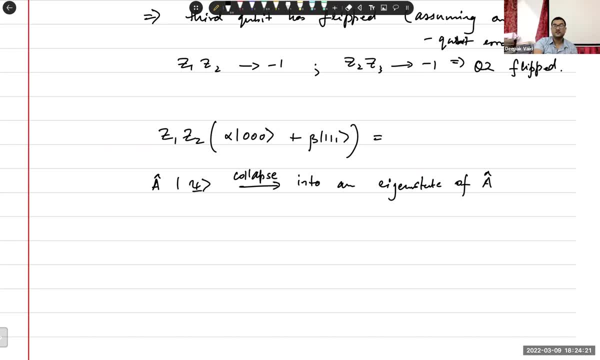 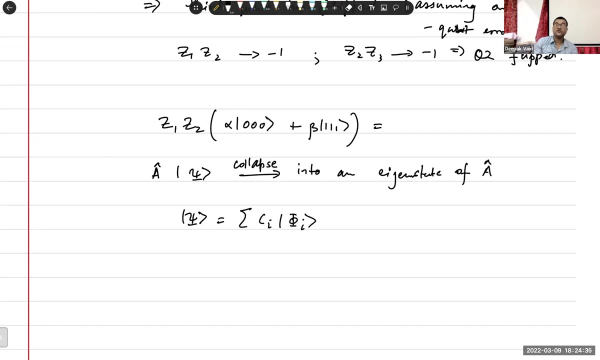 span the entire Hilbert space. So they give you a basis for your Hilbert space. This is the important part. So you can take any state psi and write it as a superposition of eigenstates of this operator A, if A is Hermitian. 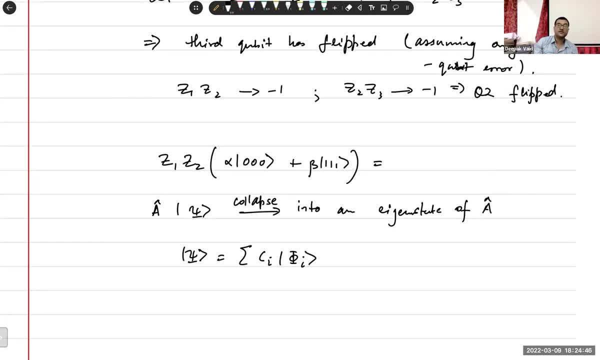 And all of these operators are Hermitian: Z1, Z2,, Z1, Z2.. All of these operators are Hermitian And, moreover, the states that we are measuring are eigenstates, so there is no collision. So you understand that if you measure, if you have a qubit which is in the spin-up state, 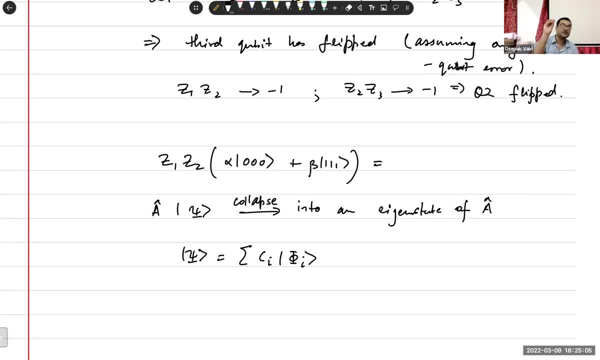 fine, I measure the poly z on that qubit. what will be the state of that qubit after measuring? It's a plus or minus. No, If it's in the zero state up state right, That is already an eigenstate of the z operator. 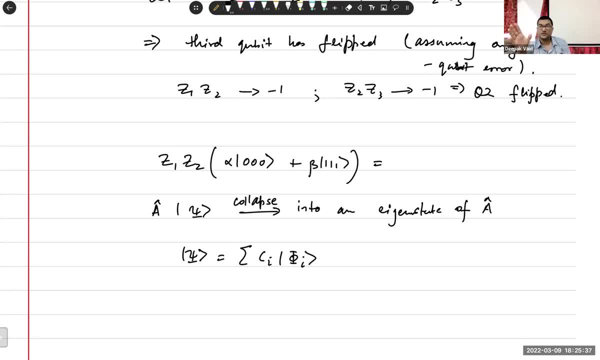 It's an eigenstate of z with eigenvalue plus one, So there is no reason for it to collapse into anything else. There are two eigenstates of z: zero and one. If I start with zero, I'll stay in zero. Make sense or not? 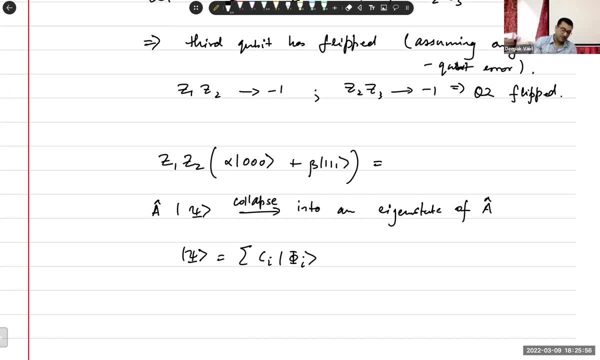 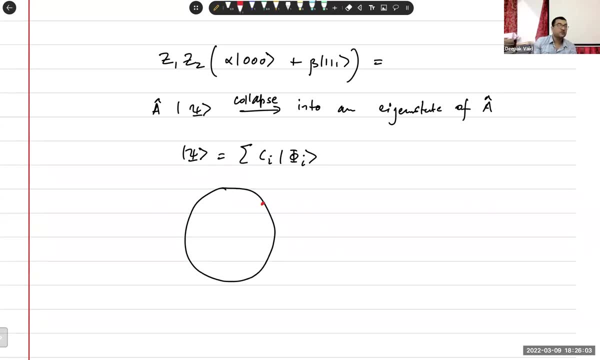 Yeah, makes sense. Think of it like this: That you have a Bloch sphere, right? You think of this Bloch sphere picture. Your state is a dot on this Bloch sphere, right, And there are two eigenstates of- and you're talking about measuring- zero and one. 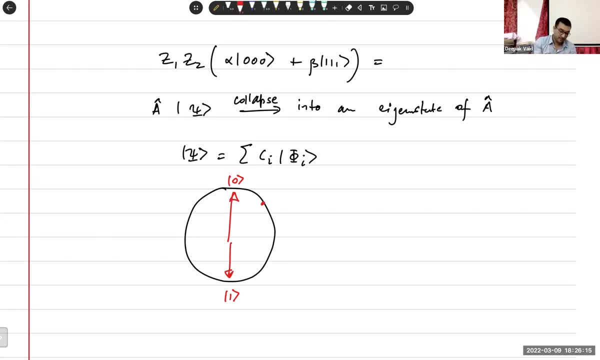 Now I know many of you get this, but I'm just emphasizing this. And so your state, psi, let's say your dot- is closer to the north pole than it is to the south pole Right Now. when you make a measurement of z, is your state going to be more likely to collapse into? 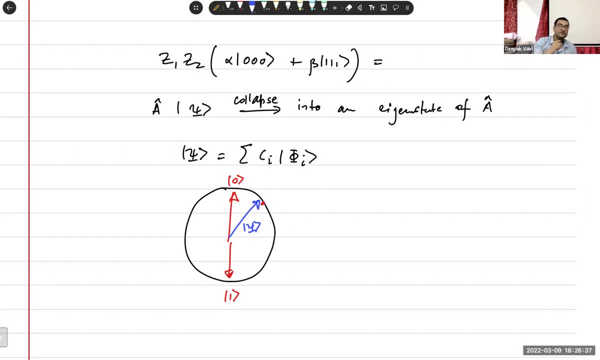 the north pole, which is zero, or the south pole, which is one North pole, And if your state so, as you go closer and closer to the north pole, the probability of collapse will become equal to one. You can think of it that way if you want, When you're talking about plus and minus states. 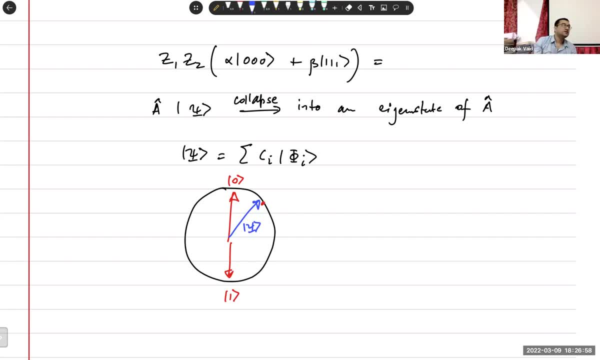 plus and minus are eigenstates of which operator. X Plus and minus are eigenstates of X and Iy. Okay so if you are measuring the x or the Iy state or Iy operator and your initial state is 0 or 1, then it will collapse into which state. 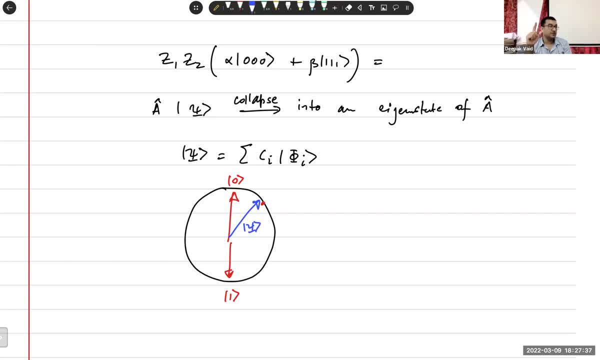 If your state is initially to begin with 0 or 1 and you measure the x operator, what will be the outcomes? What are the eigenstates of the x operator? Plus and minus. So what will be the outcomes? Either the plus state or the minus state. 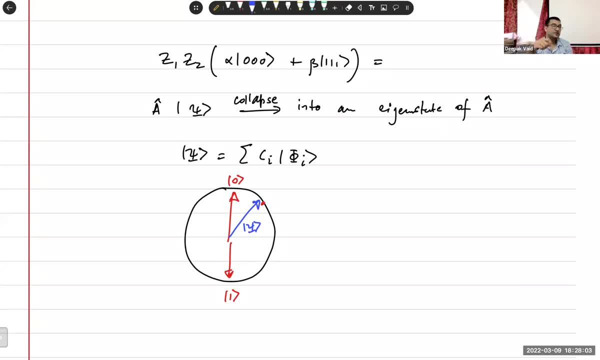 And with probability, half each. If you don't understand this, Zoom people and people here. please just think about this. This is a seemingly very minor point, But it lies at the base of everything That is going on: The fact that you can perform a measurement of these operators. 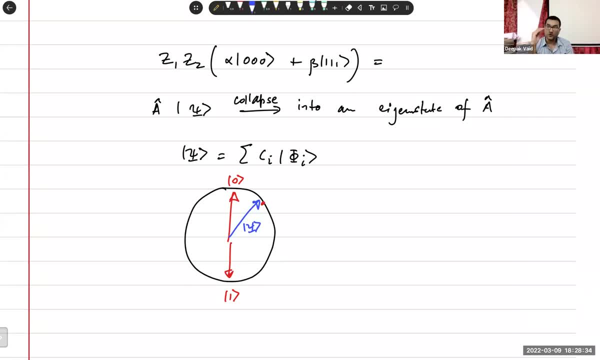 without destroying the state, Because if you cannot do that, then nothing that you want to do as far as correcting your errors without changing the state, without destroying the quantum correlations, is possible. Okay, Yeah, This is fine, But are we able to measure that measure of systems in plus or minus? if you're doing x, 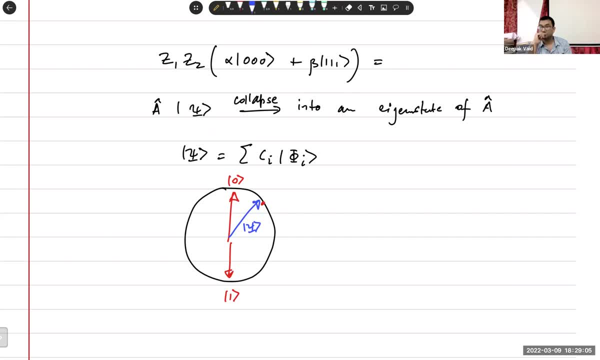 Or on or minus one state. Are we able to measure that without arming that state? No, no, So that depends on what your state is. This is the whole point. No, That see. in this setup, all our states are superposition of 0 and 1.. 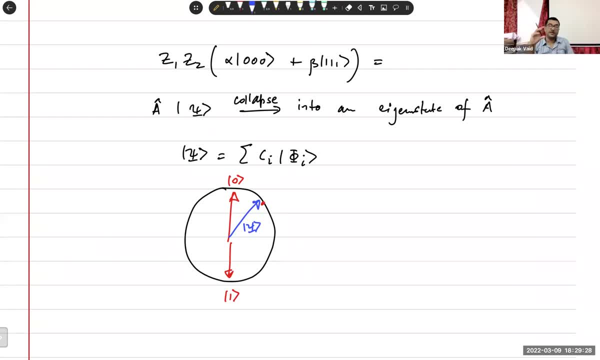 So if I measure any of the z operators right, I'm always in some eigenstate of those operators, So my state will not collapse. So you don't collapse, Right? Are we able to make out that it is in the plus state? 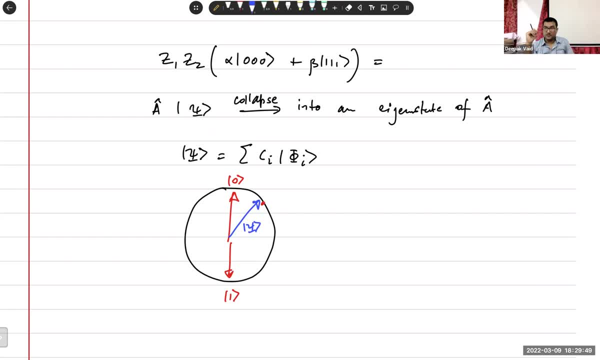 Or the issue is, if it is in one state, we're going to say that there are no, the bits are the same, But the thing is so, the thing is so. here's the thing. No, That okay. So let me, let me show you again. 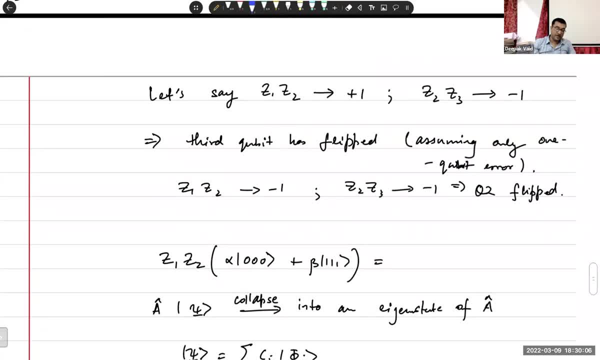 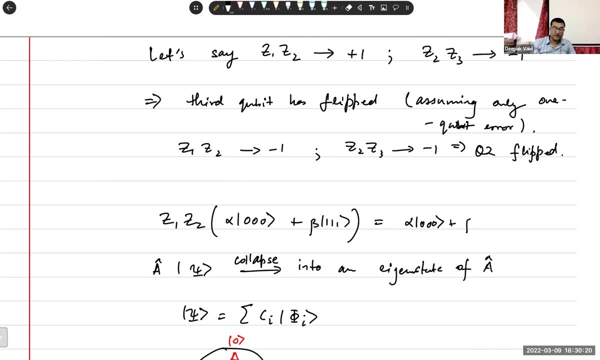 If you take z1 and z2 and you act on alpha 000 plus beta 111,, what is the? what is the result? It's equal to alpha 000 plus beta 111,. right Is the state. So the state changed. 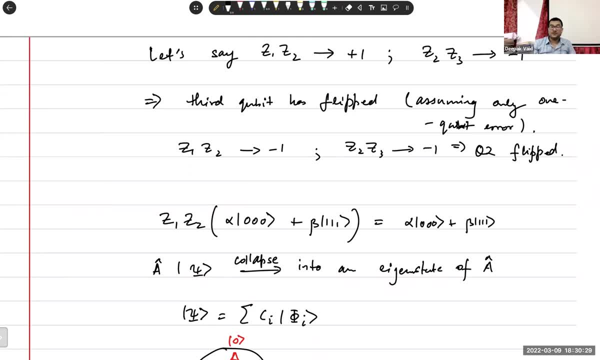 Changed, But do we know that it changed? Like, if we know that the state didn't change, then we can say: the bits are the same, But we do not know. that right, No, no, But, but. but as far as the mathematical theory is concerned, these two operators will not cause the state to change. no, 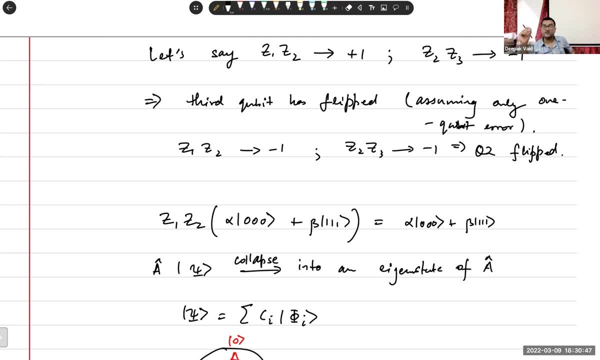 Practically No, no, So practically there might be some, some errors in the measurement, in the, in the way you implement this measurement, Which might constitute a separate source of errors. Right, So there might be an error in the syndrome measurement itself. 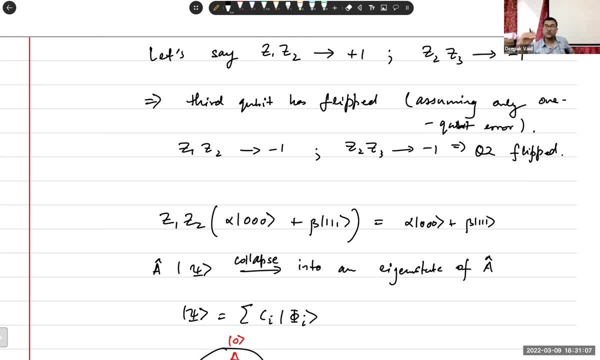 But assuming that the syndrome measurement can be performed without making an error Right Now. your question actually has a very nice answer. I just didn't go into it because it requires a little bit of math, which is It involves some error. 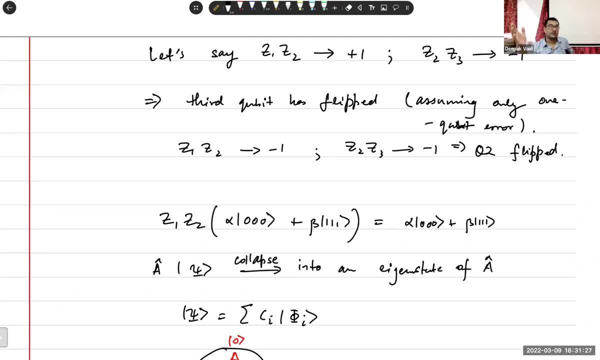 Right, It involves something called the notion of fidelity in mixed states, Right? So exactly what you're asking is that how can you tell whether there is an error, which is big or which is small? Okay, Why? Because these quantum states live in this continuous space. 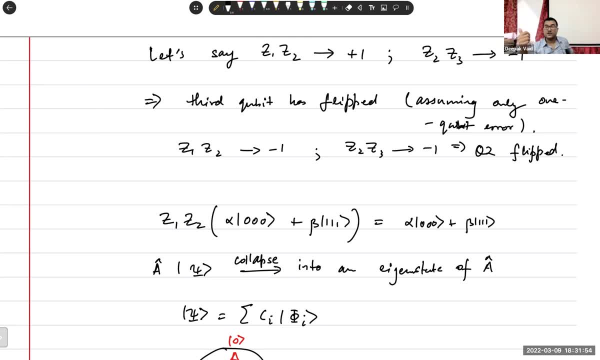 Right. So let's say that you have a bit flip error, which is generated by which? which poly Aditya bit flip is caused by which poly X. Excellent. Now, if I start with the with the state plus and I act on it with X, what happens to that state? 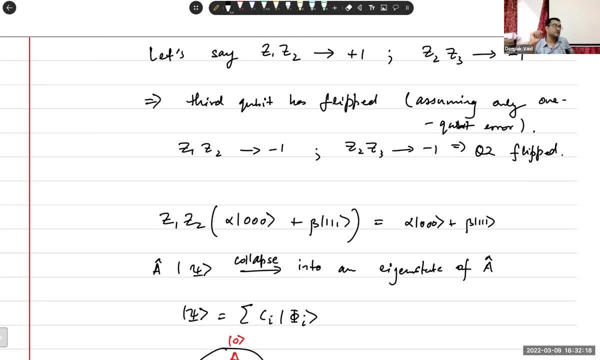 But is the qubit flipped? The qubit is flipped. no, Zero goes to one and one goes to zero. Right, But nothing happens to that state. On the other hand, if I start with the zero state and I and there is a single qubit error generated by X, what happens? 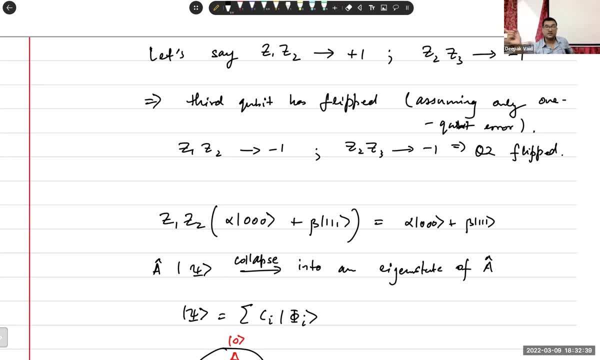 It goes to one If, I, if, if the error no, no, X acting on zero will give me one. So my point is That: how do I quantify? So in one case, in both cases, an error is taking place. 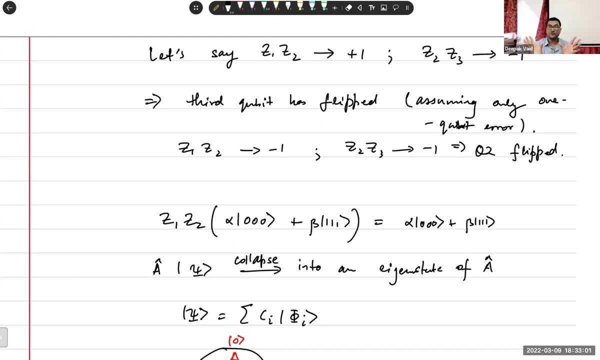 Which is a bit flip, is happening. I know that for sure, Right. But in one case the bit flip leaves the state invariant. In the second case, the state becomes orthogonal to itself, Right? So in the first place I should not worry about that error. 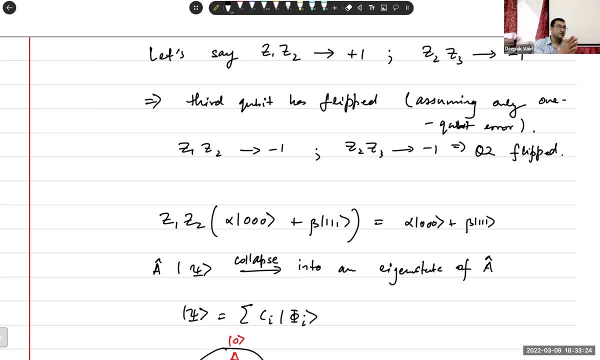 I don't care, Because I only care about those errors which cause my state to change into something that is orthogonal to itself. So this question is answered. This is answered by the notion of fidelity. Right, Fidelity is the term that one uses to describe the quality of sound. 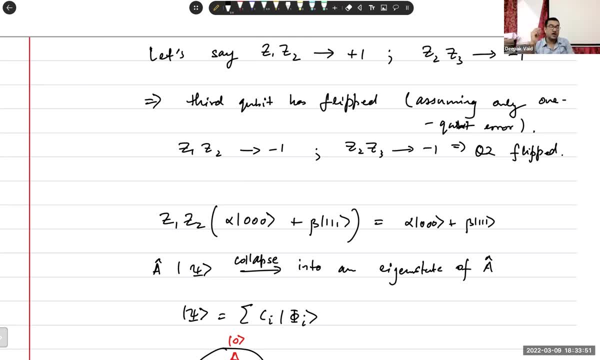 Right, Normally. How true is it to the original? So for this, fidelity is basically the overlap of two states. Okay, So if you take two states, psi and phi, and you overlap, you take the inner product. If those two states are the same, you get one, otherwise you get zero. 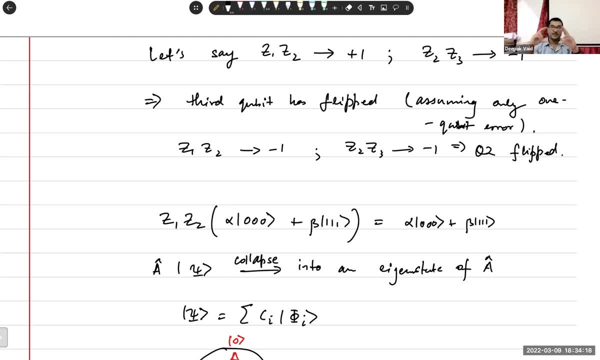 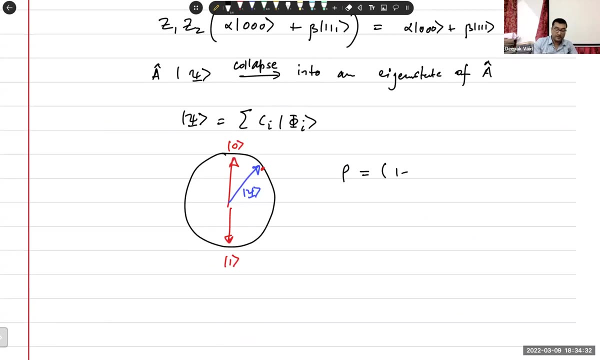 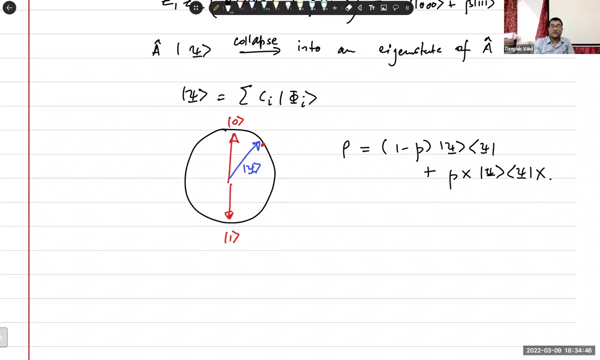 Right, So the fidelity is essentially given by this quantity. So now what one does is the following: You write down an operator which looks like this: I'm assuming that all of you can see what I'm writing. Okay, What is this operator doing? 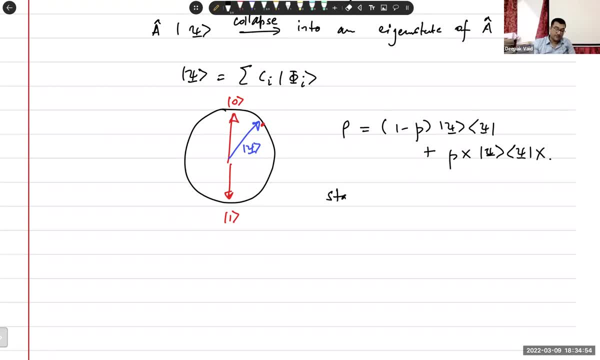 Our state phi or state psi is the state of interest. Okay, This is the one that we care about. The number p is what? Number p is the probability. What is it? The probability of bit flip Right? What does the first term tell you? 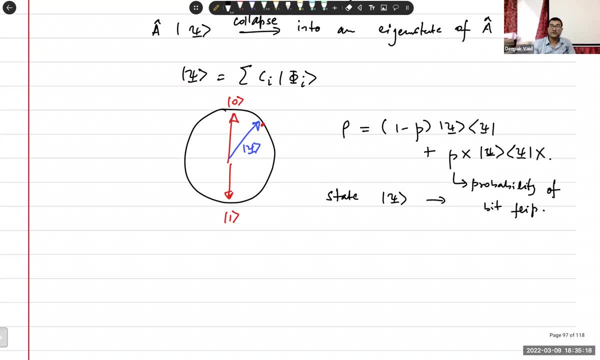 The first term tells you that no bit flip is happening. If there is no bit flip, then the first term tells you that your state doesn't change. What about the second term? The second term tells you that there is a bit flip. That is expressed by the presence of the x operator. 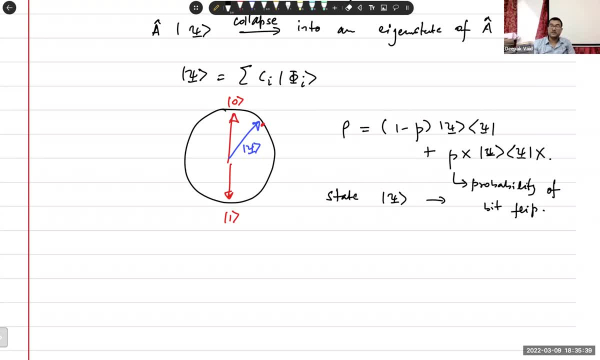 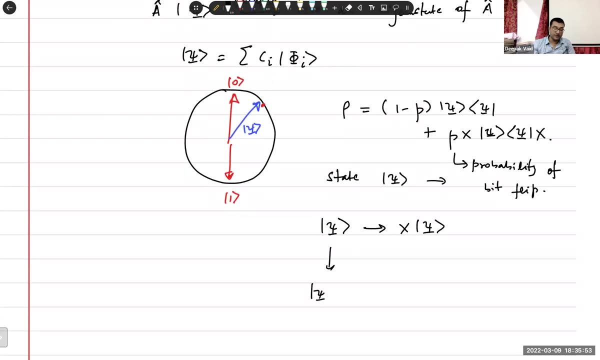 But note the way in which this projector is constructed. We take our state psi and we flip the bit So we get zero. We flip the bit So we get x psi. This is the state with the flip bit, Right. So if you want the projector for the state psi, you take bra psi. 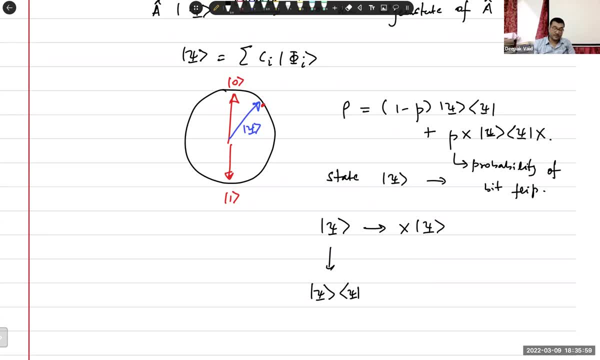 So you take ket psi and then adjoint ket psi. If you want to construct the projector for the flipped state, what do you take? You take the adjoint of the x psi. So you will get what You will get: x, ket psi, adjoint psi. 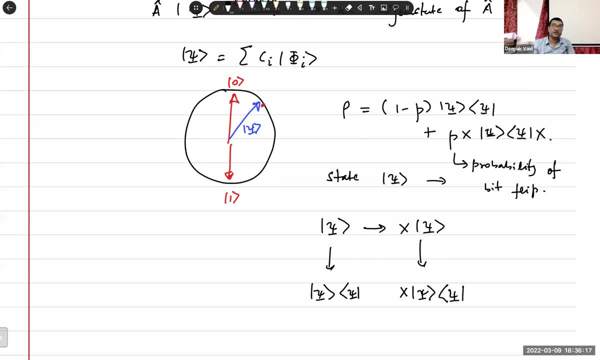 And then again Adjoint x. What is adjoint x? It's x only. So this row that you have here, right, This row is what we refer to as a channel. Okay, It represents. so something is happening. You are sending your state from point A to point B. 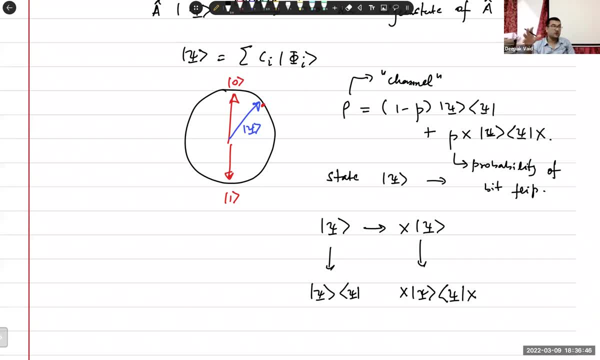 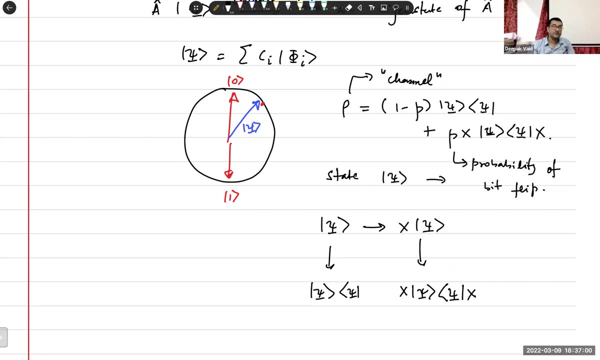 Right, And presumably it comes out on the other end: Something happens to it, Right? Either there is a bit flip or there is no bit flip. If there is a bit flip, that is represented by the second term. Otherwise it's represented by the first term. 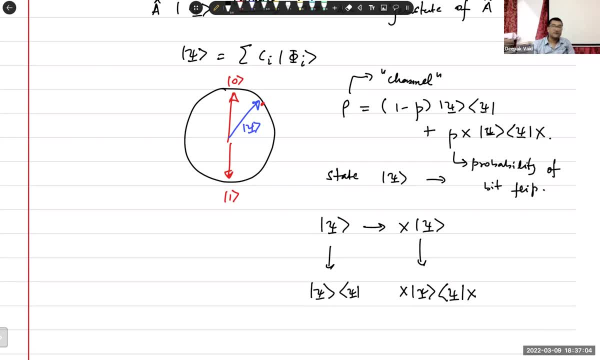 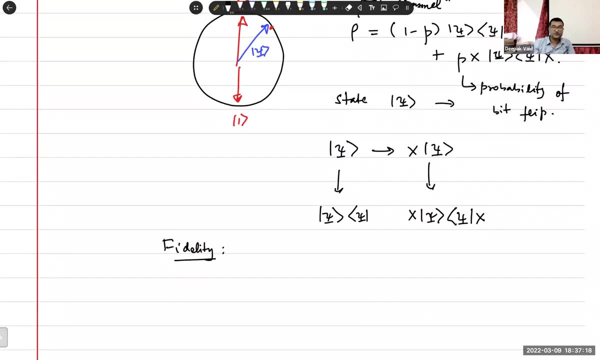 And so this row is an operator Right And it's called a. I mean, that's how you represent channels in quantum information. Okay, Now how do I define the fidelity? Okay, So the fidelity is written, defined as follows: 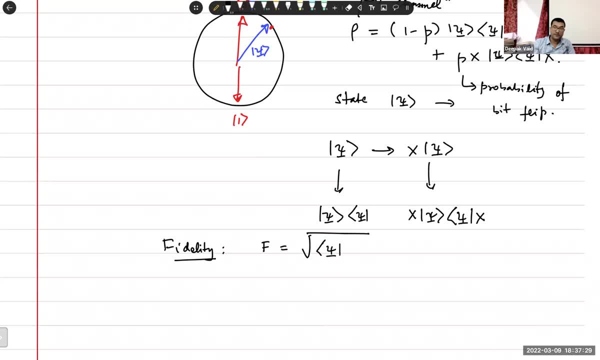 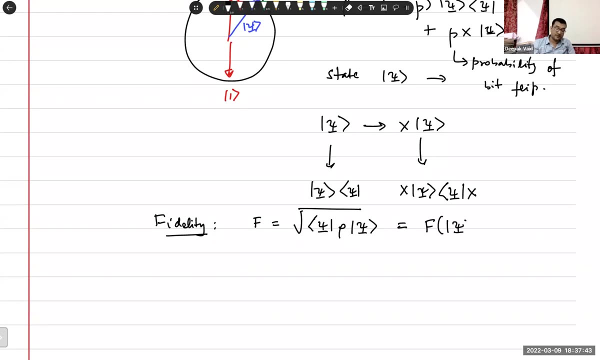 And, technically, what rho is. rho is what is called a mixed state, And this is the Greek letter, rho, by the way, not p. Okay, So the fidelity is defined as, as this expression, Fidelity is a function of two things: two inputs: 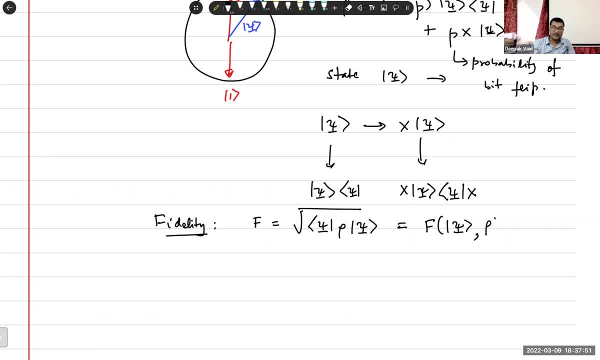 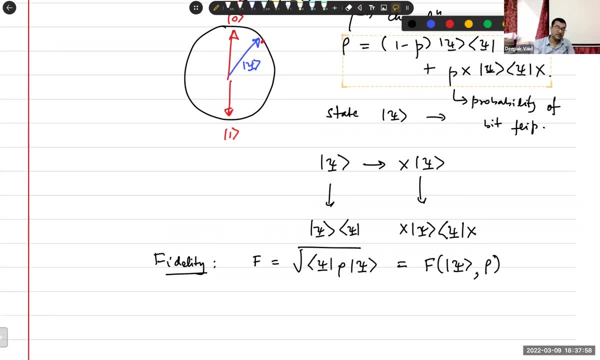 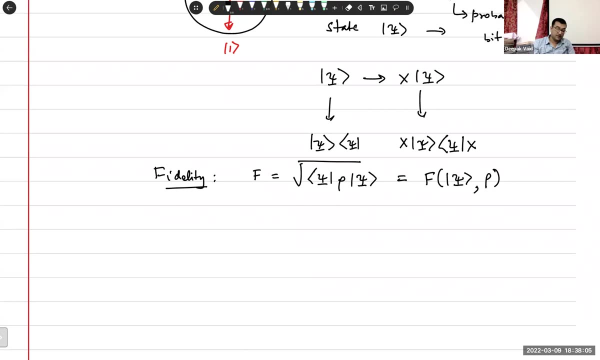 It takes in a pure state, psi, and it takes in a mixed state, rho. Okay, And that's what this rho is. This is a mixed state. Okay, And don't worry about what mixed states are for the time being. Now we can do this calculation. 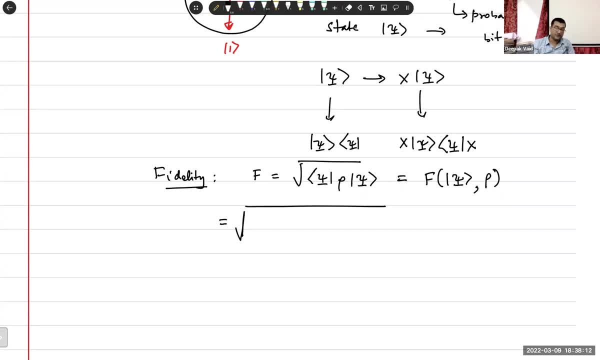 By putting the expression for rho in a product right. So we get psi. And then we put one minus p Right, Plus x p times x psi, psi x Right. Okay, So this is our fidelity. Now what will happen? 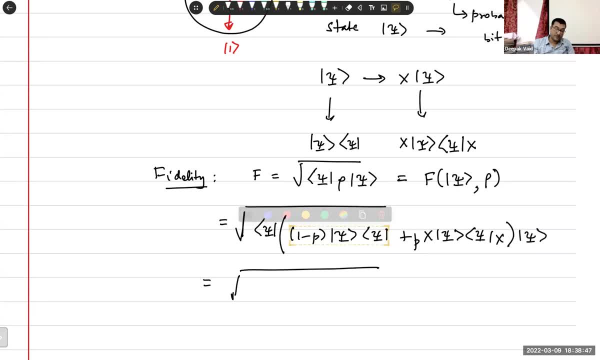 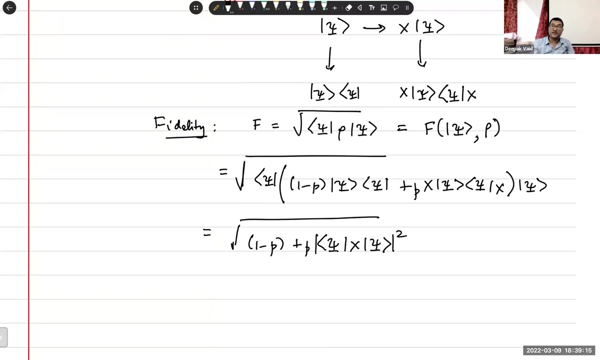 The first. the first term will just give us one minus p, Right, And the second term will give us the following: Expectation value of p times the expectation value of x acting on psi whole squared, Okay, You get psi x- expectation value of psi and then psi x- expectation value of. 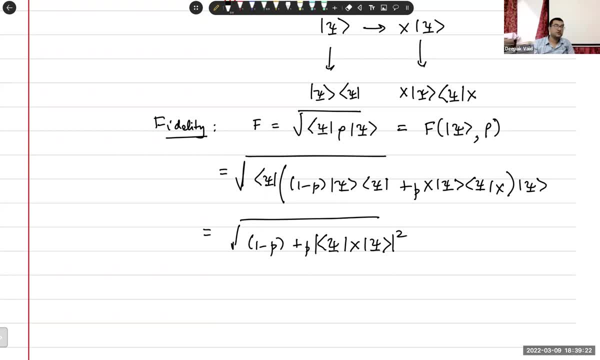 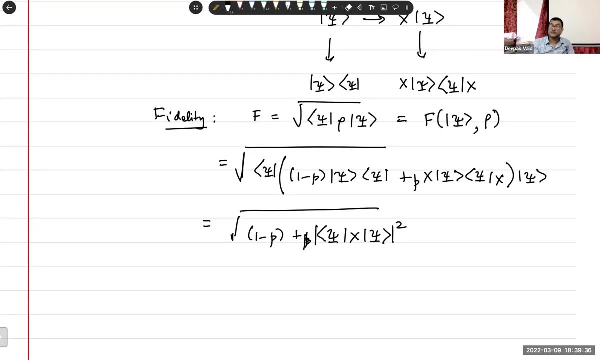 So you get that twice. So that's why I'm writing that as whole squared, And there's a magnitude, because there is an adjoint in there. Okay, Now, both of these terms are positive definite, So this one is positive definite. 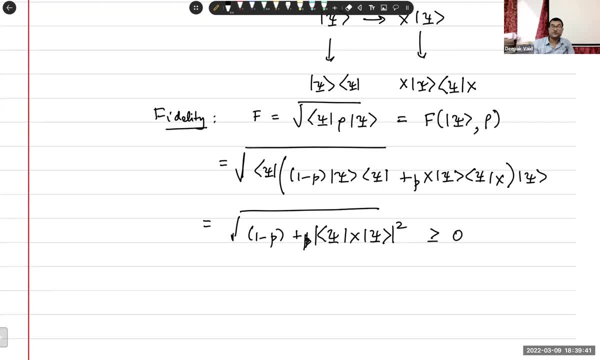 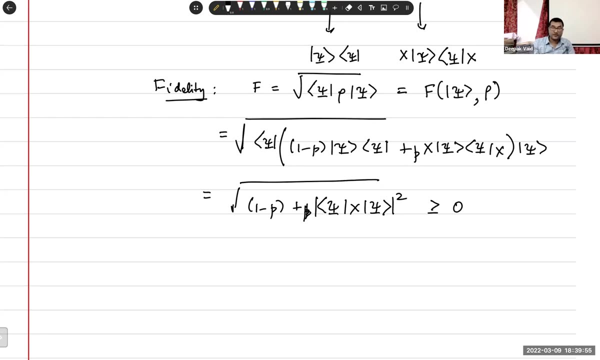 Right. This fidelity is always greater than or equal to zero. Right And the second term. So the second term is also non-negative. When is the second term zero? When psi is equal to either zero or one, the second term goes to zero. 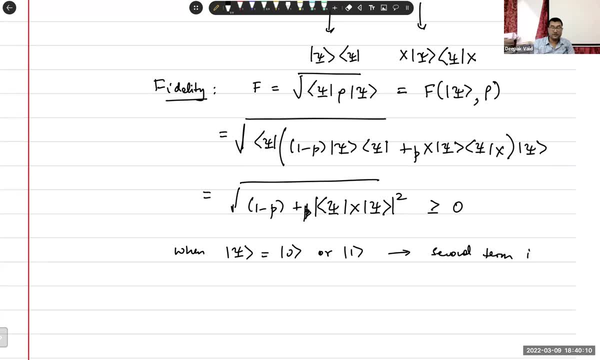 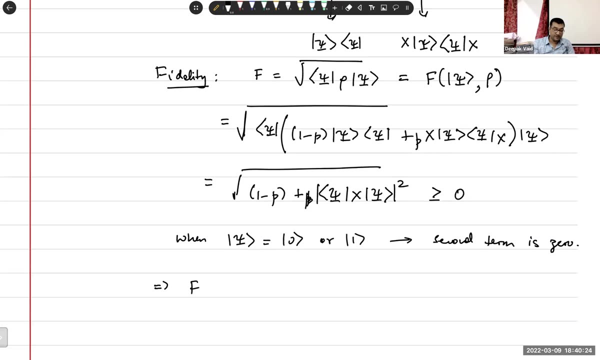 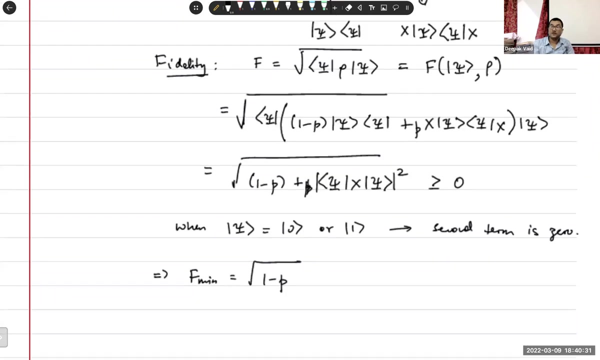 Right. So now the second term is positive, definite. So that means the minimum value it can have is zero, Right. So the minimum value of the fidelity is what It's a root of one minus p Right. This is the minimum value of the fidelity in this particular case. 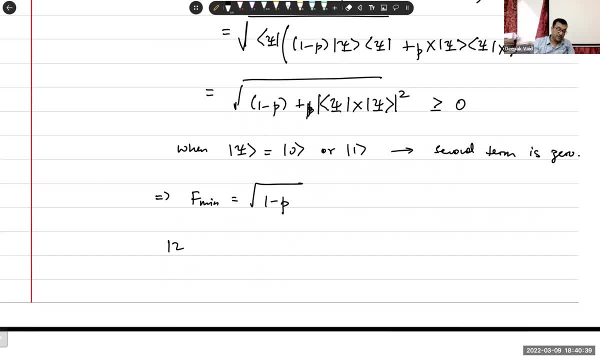 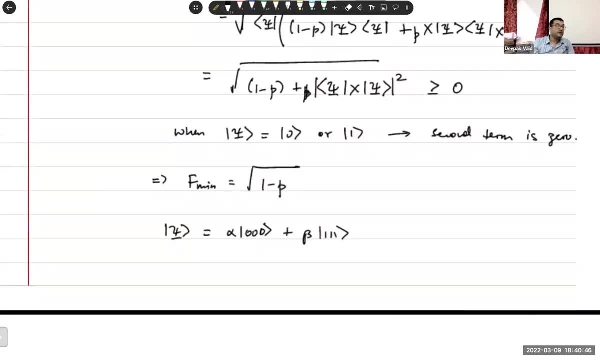 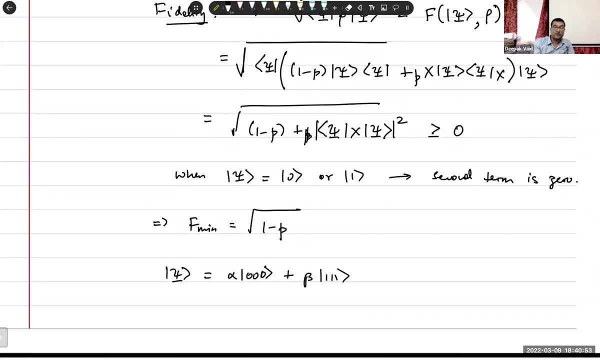 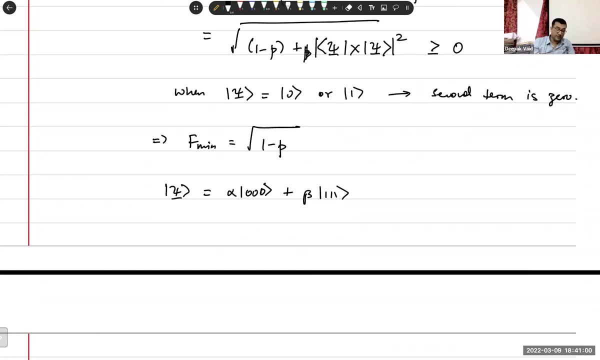 Let's go back to that three qubit encoding alpha, zero, zero, zero, beta, one, one, one Where we did this probability analysis Right And what was the probability of having a bit flip on either one or less of the qubits? I'll write down the expression. 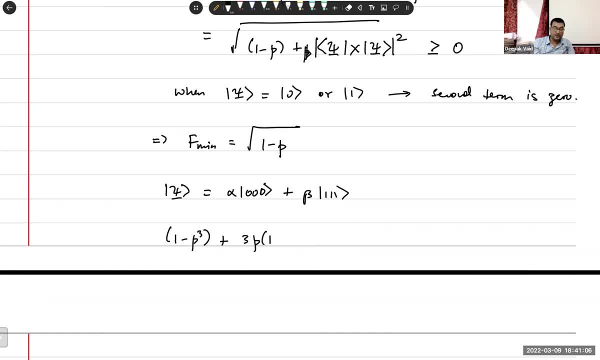 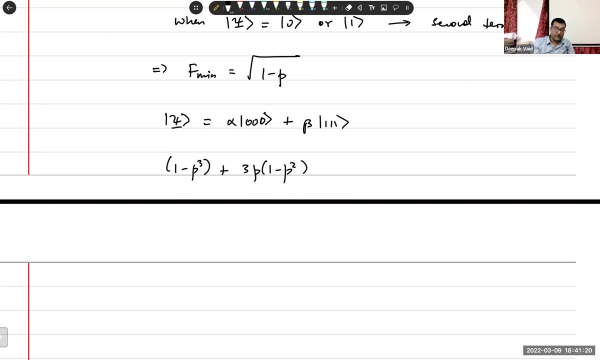 It was one minus p cube plus three p, One minus p square, Right? We derived this in the last lecture, I believe. Right, So we can write this in terms of rho. Okay, We can translate this into an expression for rho. 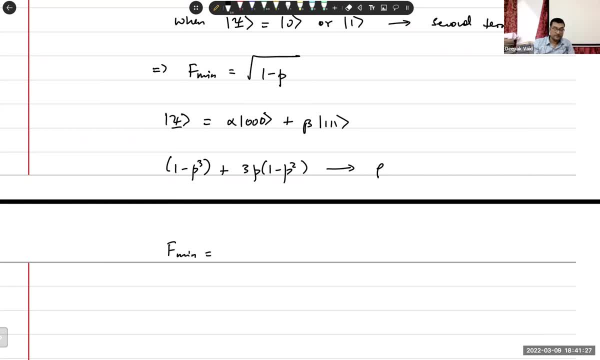 And then we can calculate the minimum fidelity. The minimum fidelity turns out to be one minus three p square plus two p cube. I'll leave it as an exercise for you for now, And then in the next class we'll work it out. 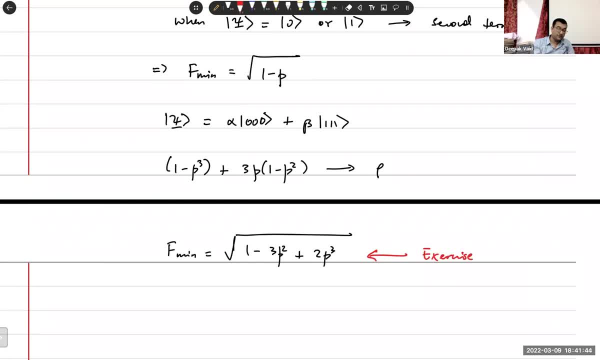 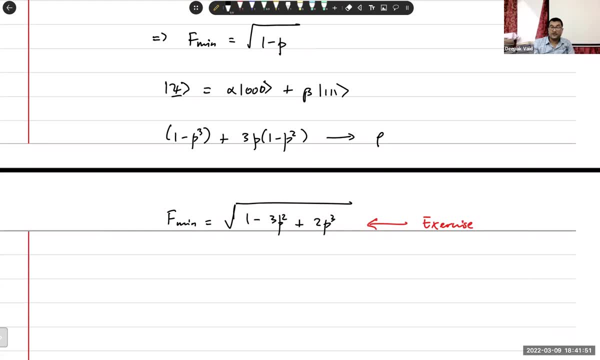 If, which is tomorrow, If you don't see how to get this And this fidelity. this is the minimum value. Okay, And remember that only when p is less than or equal to half does the three qubit encoding have any advantage. 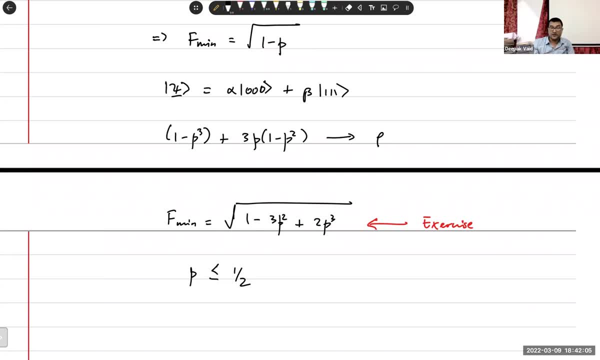 Right, And so this fidelity should be more than zero. Right, And the fidelity will be more than zero if p is less than half Right. So this tells you the same thing: that when p is less than half, your fidelity is less than zero. 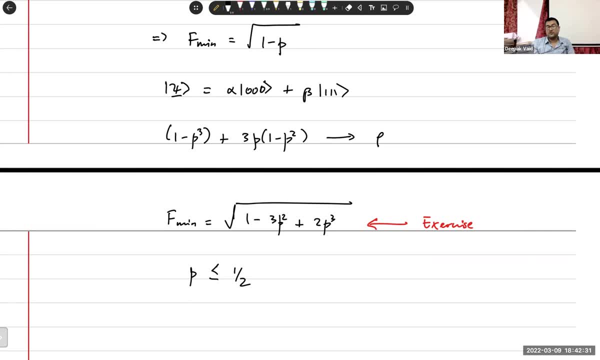 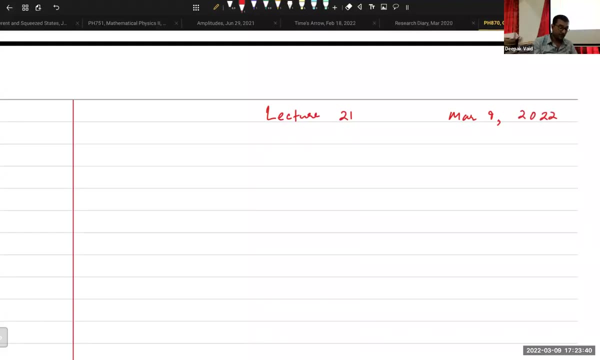 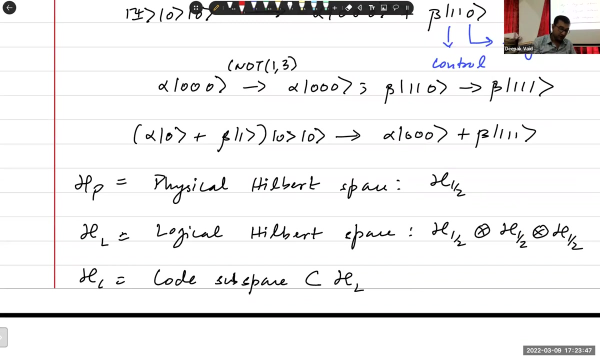 Now to I don't. I'm not sure whether or not it answers, Or whether I've led you down a path that is long enough that you don't remember where you started from. Yeah, All right, So what I have talked about in the 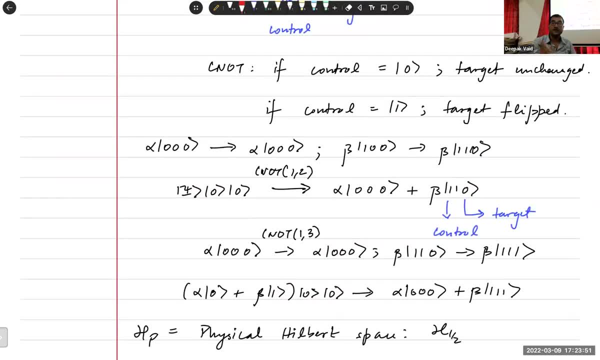 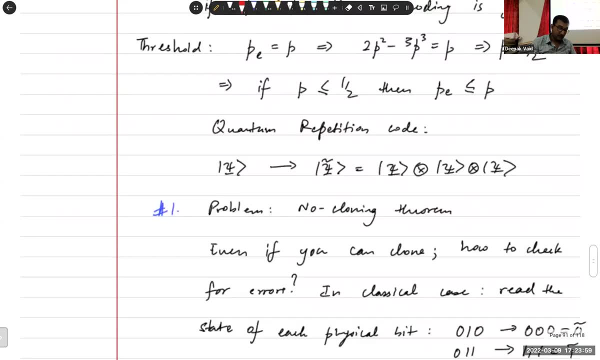 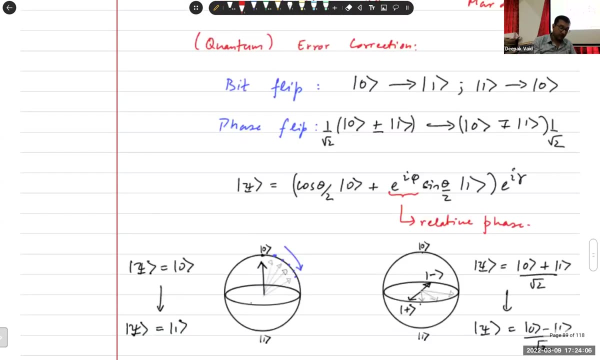 Till now in the previous lecture, and everybody can hear me in the classroom, right, Okay, Is that? error correction is all about redundancy, Right? So well, first of all, okay, let me just go over some of these things you might have forgotten. 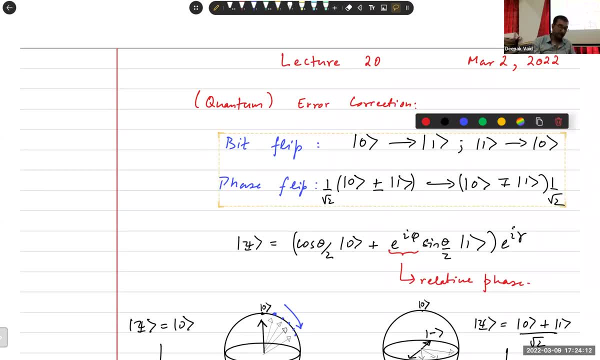 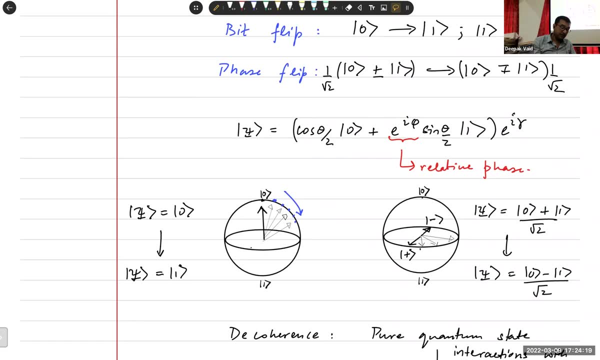 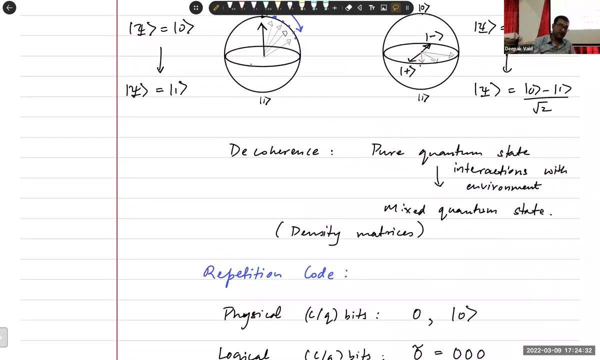 There are two kinds of errors: phase flip and bit flip. This is clear. Are there any doubts about this, Right? So bit flip you can understand as going from the zero state to the one state. Phase flip you can understand as going from the plus state to the minus state, as a bit flip in the bell basis. 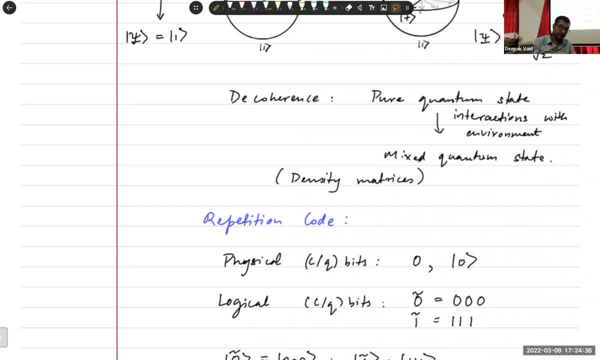 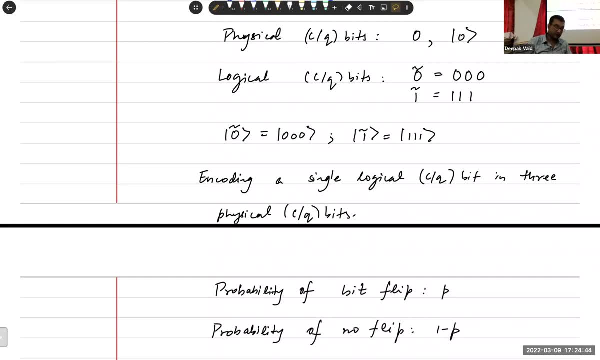 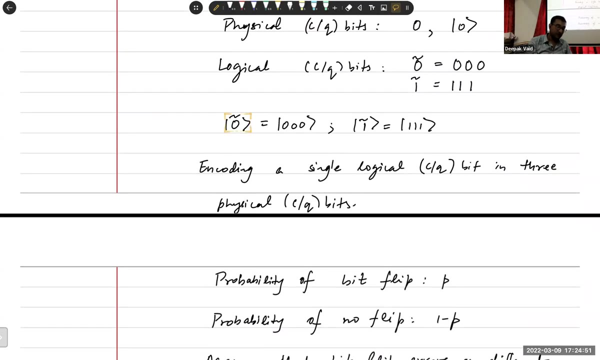 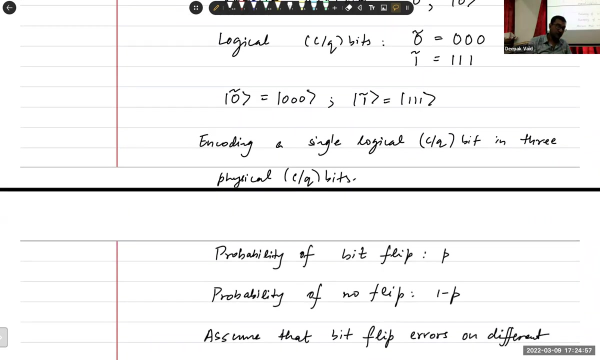 Right, So this is called the bell basis, the plus minus. So the simplest approach to error correction involves using redundancy. Right, So you encode a single qubit, a single logical qubit, using three physical qubits. So that way, if one of those qubits undergoes an error, you will still have two which are unaffected. 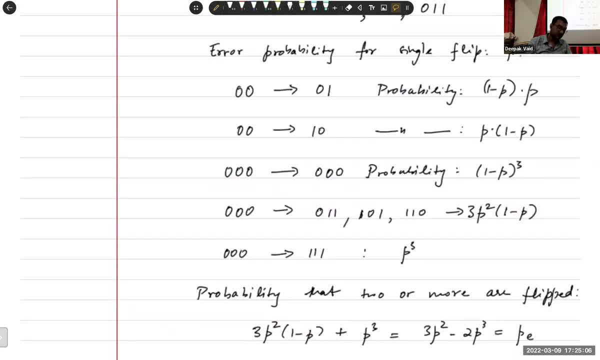 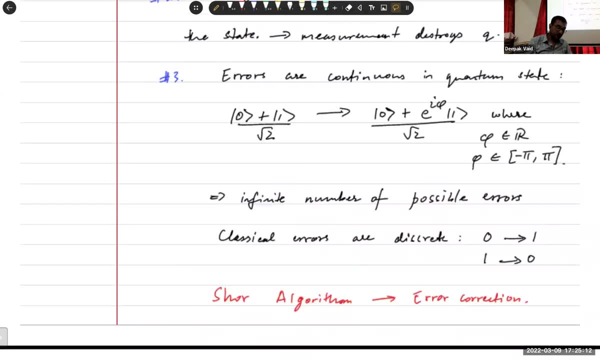 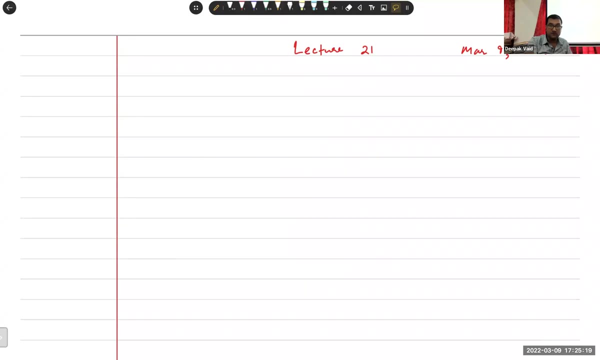 And maybe with some. Maybe there is some way then in which you can recover, Right. So what is the process Now? let me go to? Okay, So this is, Let's see, Right. So then we also talked about how to encode this logical qubit in the physical qubit. 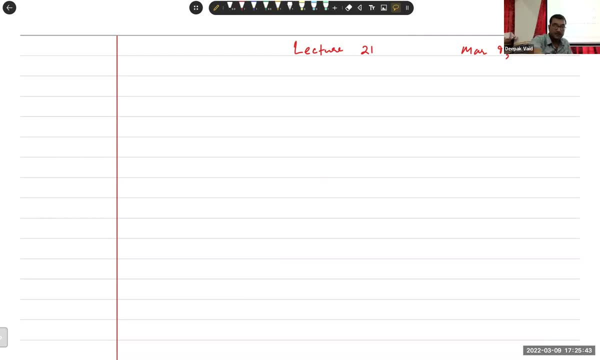 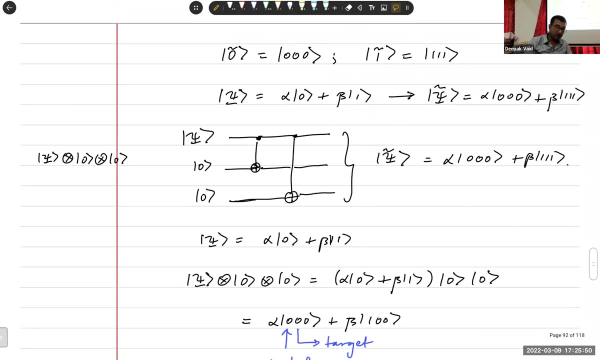 Right, This is your circuit And, as I explained, if you take this circuit right And you apply First CNOT gate- So you write psi as alpha zero plus beta one, You apply the first CNOT gate- What happens? 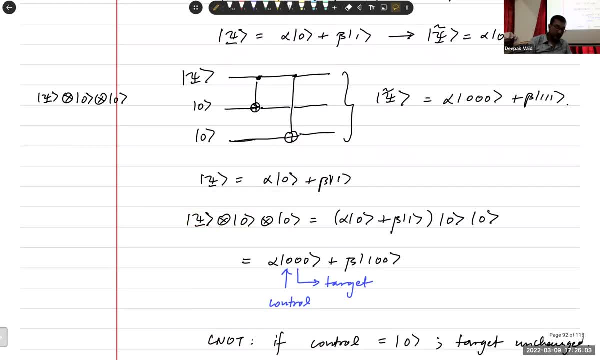 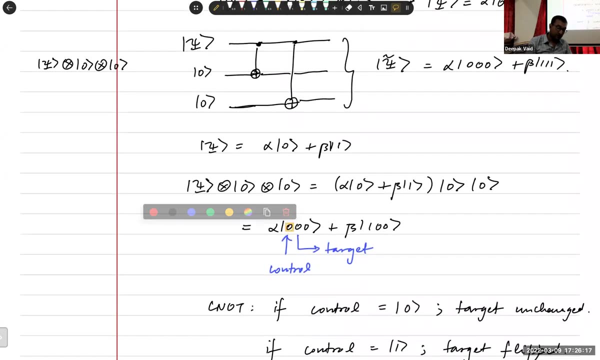 You start with this state, You apply the first CNOT gate. Now, when you apply the CNOT gate, this is the control and this is the target Right. So this first bit is the control, The second bit is the target. 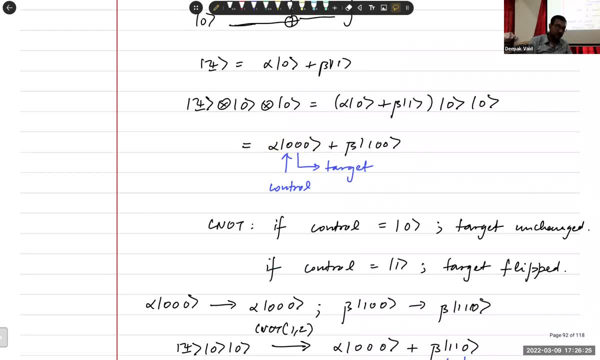 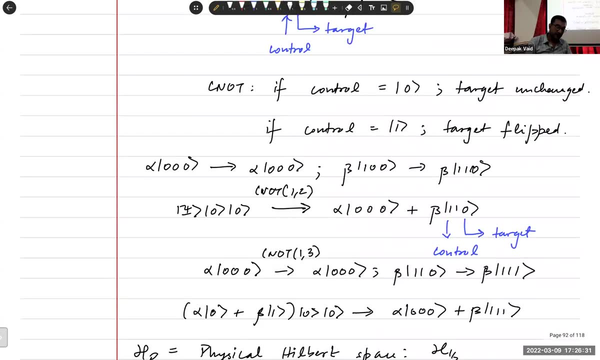 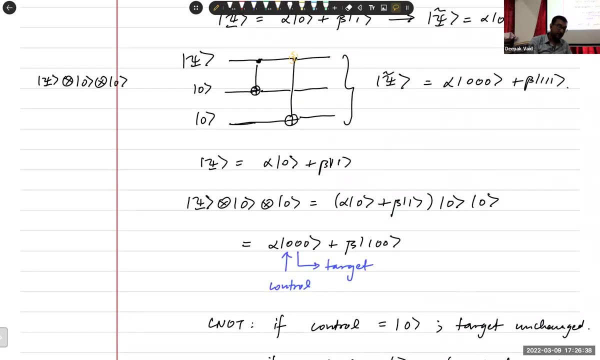 So in this state nothing happens because the control is zero Right. In this state the target is flipped because the control is one Right. So you get beta one, one zero. Then you apply the CNOT gate again, using this as your control, and this is your target. 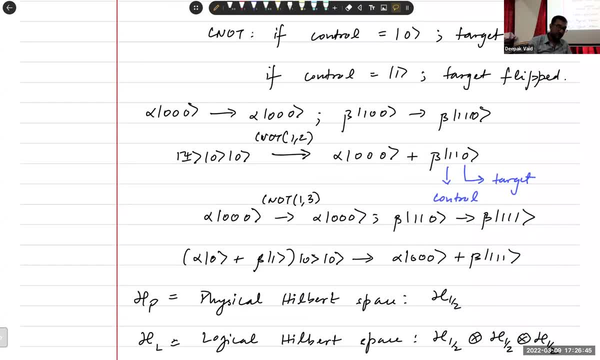 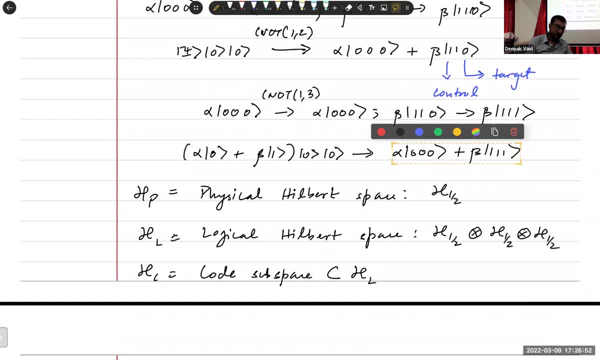 And once again. so nothing happens to the first state, but the second state goes to one one, one, Right. So you end up in this, in this state, Right, And this is called a. this is called a cat state. 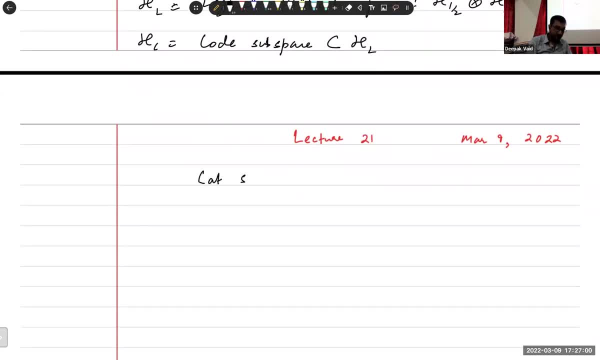 There's a word for it. States of this form are called cat states. So typically if you have an N qubit state which looks like this, something like one by root, two, All zero, All zeros And all one, So first of all, this is a highly entangled state. 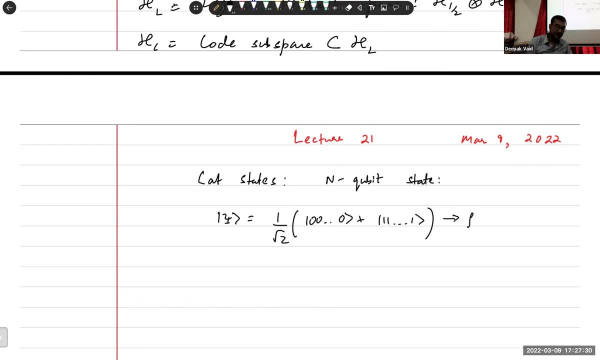 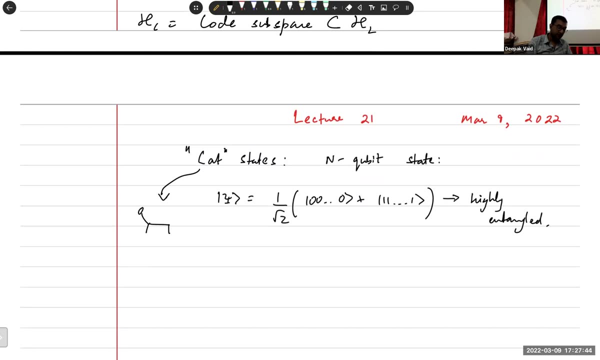 Right, There is no, you cannot factorize it. Right, So it's highly entangled. And the reason we refer to this as a cat state: Right, Because we are actually referring to Schrodinger's cat, That cat, Because in the limit of large N- right, your system becomes more and more macroscopic. 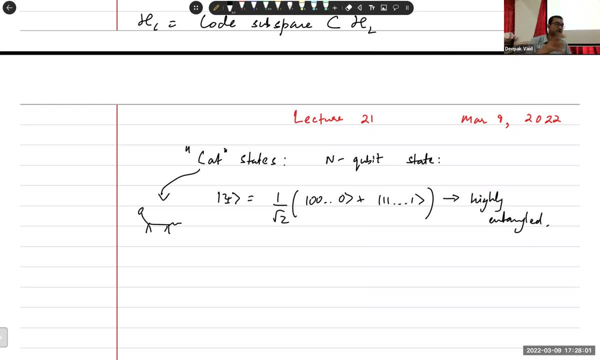 Right. So if you imagine that, that you have a system which consists of a very large number of qubits like enough to make a cat and you put that system in this kind of a state, this would- this would correspond to, let's say, this could be something like dead. 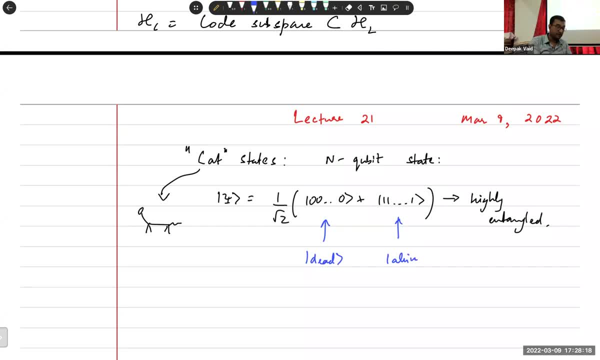 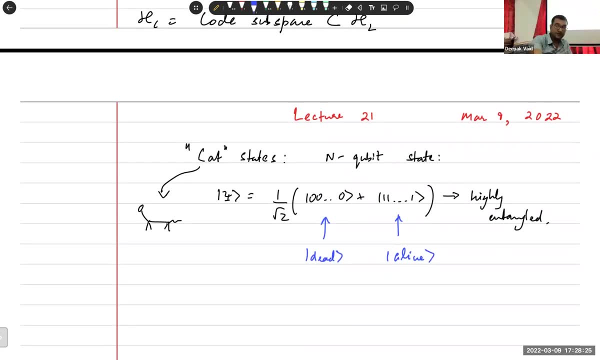 And this could be alive, Right? So this, this would be the statement of Schrodinger's cat. Okay, So now let's talk about error correction. So how can we correct errors in our, in our system? Okay, So we have to perform a measurement. Without performing a measurement, we can't tell if there is been an error or not. But the problem is that typically, measurements will cause your quantum state to collapse. You will lose quantum, you will lose the quantum correlation Right, And you don't want that to happen. 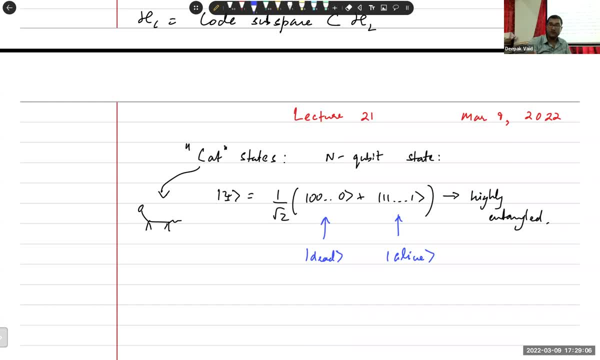 Right. So you want to perform measurements, but you want to perform them in a way that your quantum state, or at least the input state, will collapse. Right, Or at least the information, the quantum information that you want is left undisturbed. 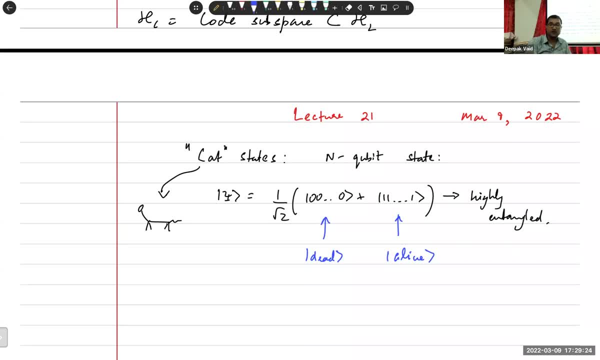 And you can do that using these operators. So right, So these are projection operators. Okay, I hope that you all remember what a projection operator is, Right, A projection operator is something of the form bra phi, ket, phi, Right, And so this is a projection operator. 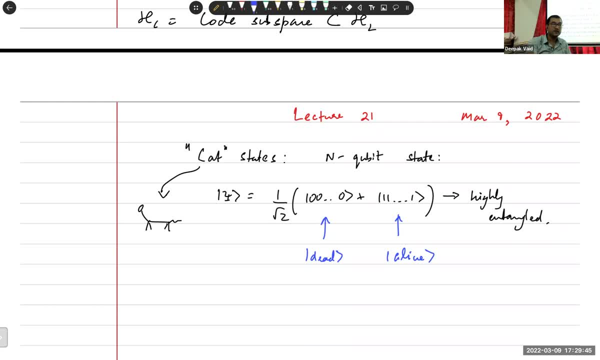 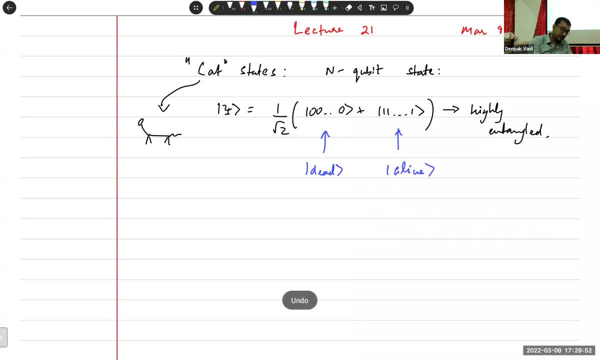 Zero, zero, zero. And this is another projection operator, Right? What will be the effect of this projection operator? So let me say that I have. Is this too small? I think maybe it's a little bit small. I'll try to write a little bigger so that you can see more clearly. 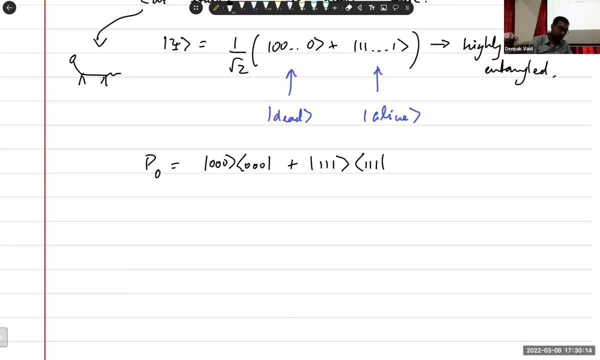 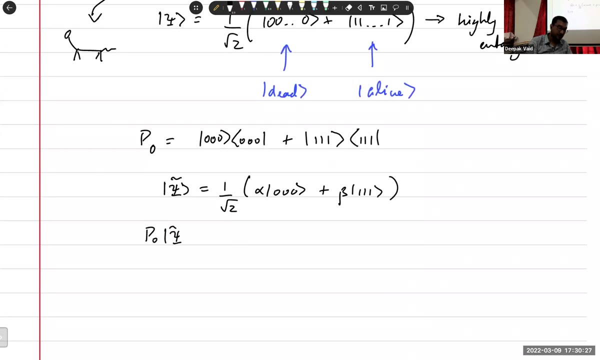 What will be the effect of this projection operator on our logical, on our encoded state? Right? So this is our encoded state And we act on this state with p non Right. So We have this guy and acting on this fellow. 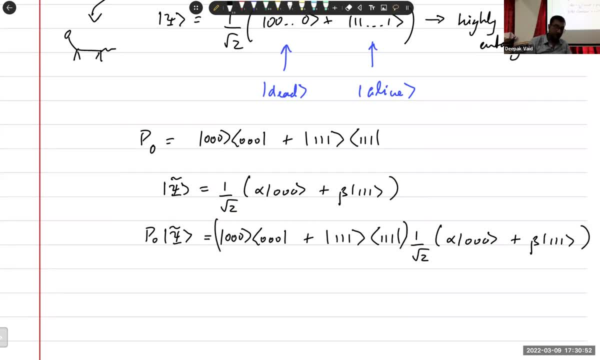 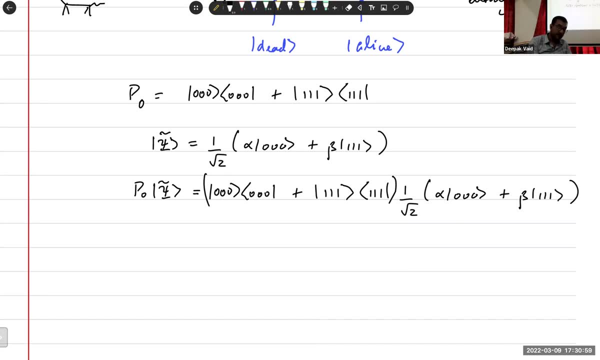 Right Now the first set of zero, zero, zero. that operator will annihilate the second component because zero, zero, zero is orthogonal to one one one And similarly, one one one will annihilate zero, zero, zero. 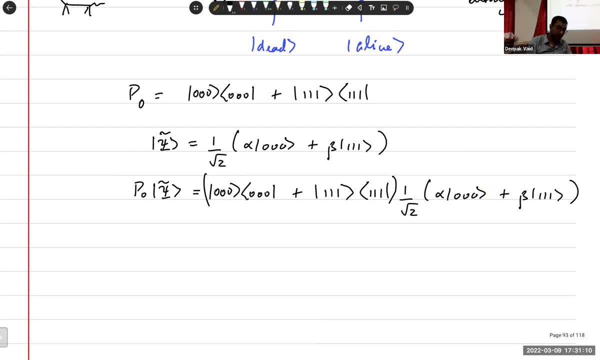 So you will be left with with psi, Right? So this means there is no error, Right? Similarly, we can construct other projection operators, Okay, And here we are given a set of three projection operators, Right, And we want to look at. in this case, we are first looking at a set of three projection operators. 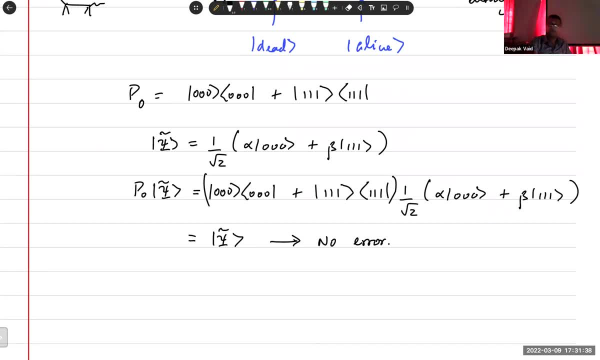 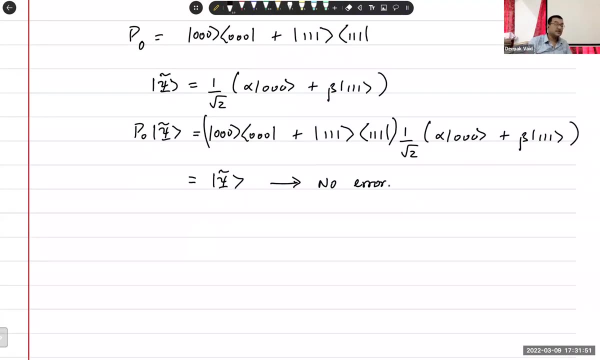 Okay, And we want to look at. I'm sorry about you guys, but the people on on zoom can see this just fine. So then we have- Yeah, Yeah, It had a power backup, but the thing is small. no, isn't it small? 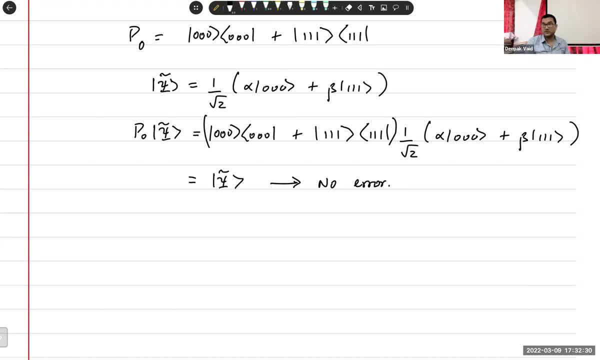 It's smaller than this also, And I will like talk to our office staff and tell them to display: this room has a UPS backup. Okay, But because it's not in use very often, That that those batteries there's been some problem or nobody has gotten it fixed. 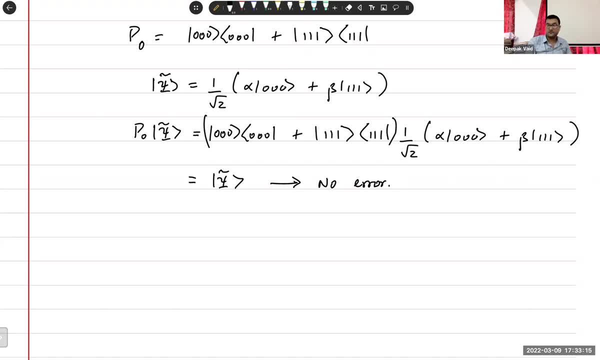 Okay, So yeah, this was a So sorry about that. Anyways, I even connected the projector, See, I even connected it to this This thing, which, which I was told has a backup, but maybe it does. 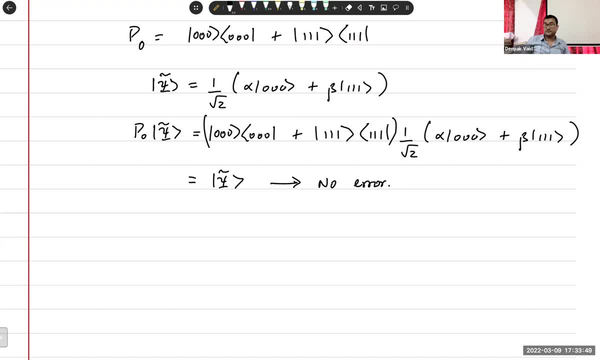 So Like another thing I can do is like I can just go to my office, You can go to your rooms, You have, you have computers. Does everybody have a have a PC or a laptop here? 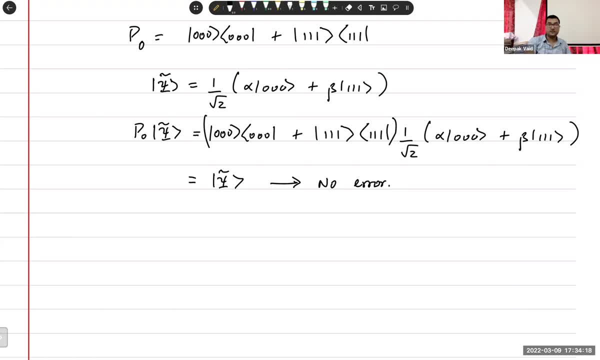 So you guys can go there And we continue this class. Mobile is fine with you. 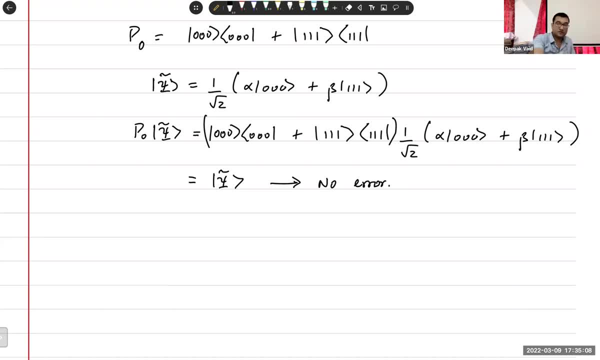 Who knows, maybe I'll just put it on like that. why bother Who is excited for tomorrow, Who is a Excited, Excited won, whoever who is not excited. everybody accepted, All right, All right. 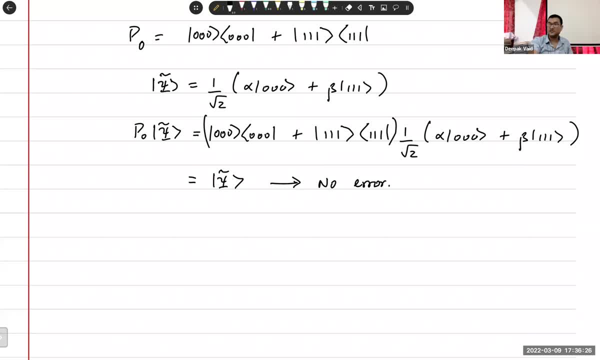 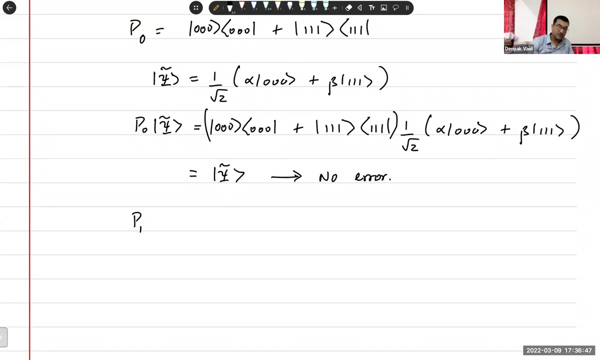 All right, I don't see any people have you all joined, okay, so let's. let's continue with our quantum error correction class. so now we have a set of four other projectors, okay, which have this similar form: one, zero, zero. can you guys see it on your phone? okay, good, right. so this, what is this? 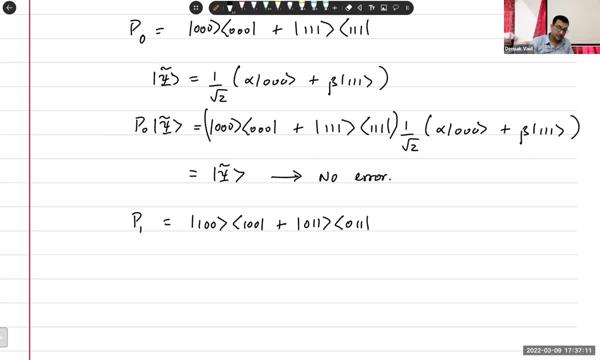 projector doing right. this is projecting onto the case when there is a single bit flip right, there's a single bit flip on the first qubit. so if there is a single bit flip on the first qubit, what will? what will happen to psi? psi will go to one zero, zero, zero, one one right, and so that's what the second, this projector, is doing. 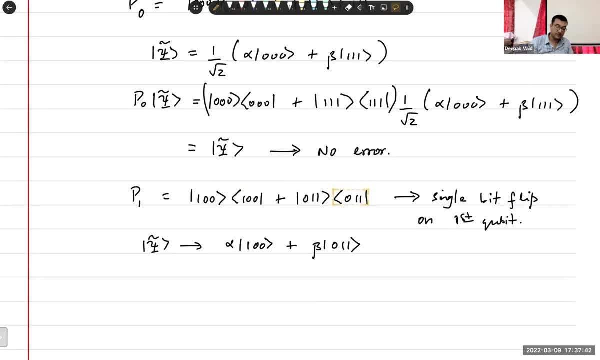 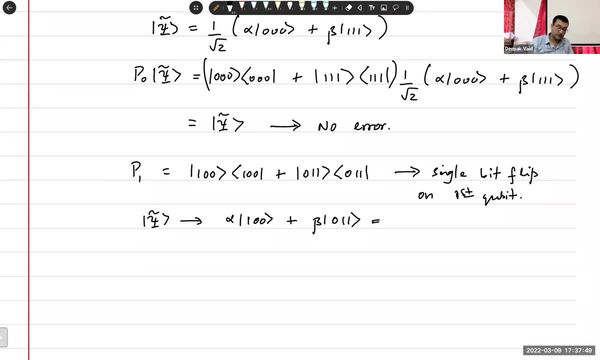 this state is one, zero, zero, and this state is zero, one, one. so, once again, if you act on- and so let me call this, i don't know what to call it- let me call it psi prime- if you act, if your state happens to be psi prime, 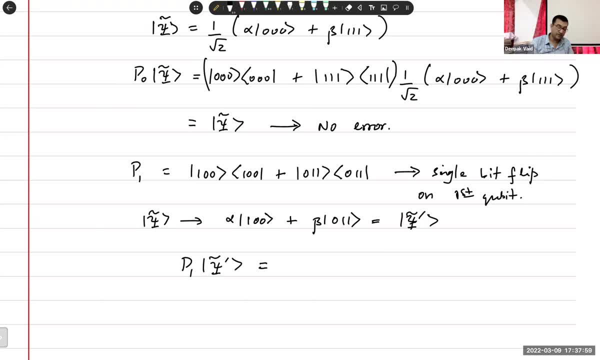 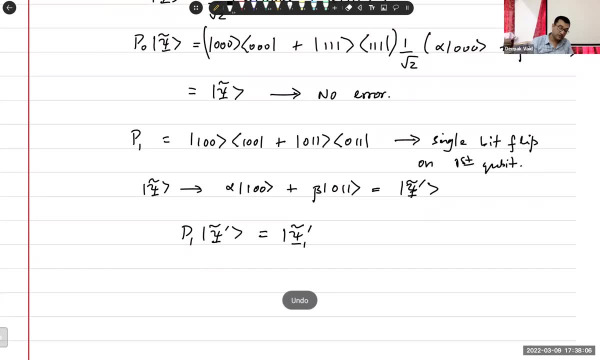 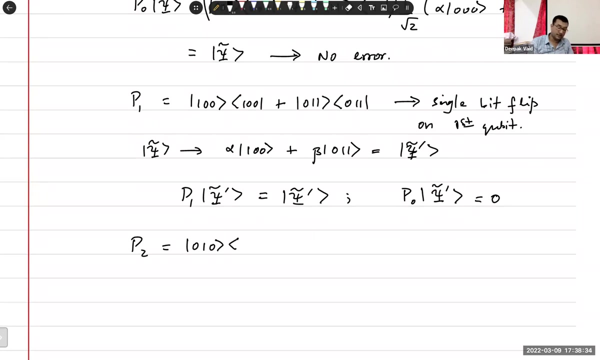 psi, tilde prime and you act on it- p one, you will get psi, psi tilde prime, okay, sorry, there's no one over there, right? and what happens if you take your projector p naught and you act on the state um, um, psi, tilde prime? what will you get? zero, right. so similarly, we can define projectors for: 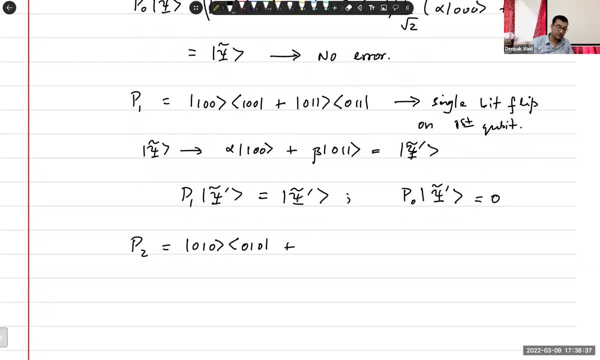 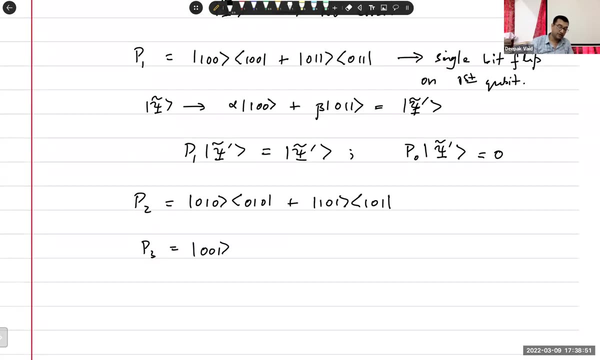 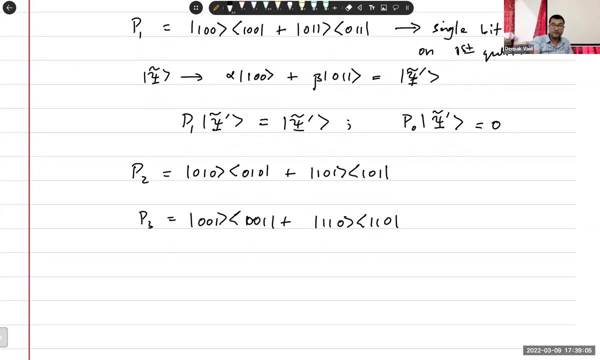 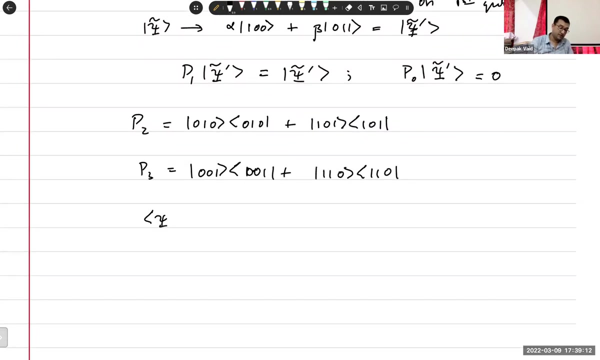 a single bit flip on qubit two, then we can define a projector for a single bit flip on qubit three. when I apply this, Sterling point angular. well, let me look at thisjay okay now. so if you measure, if you measure your, your state right, you will get zero. 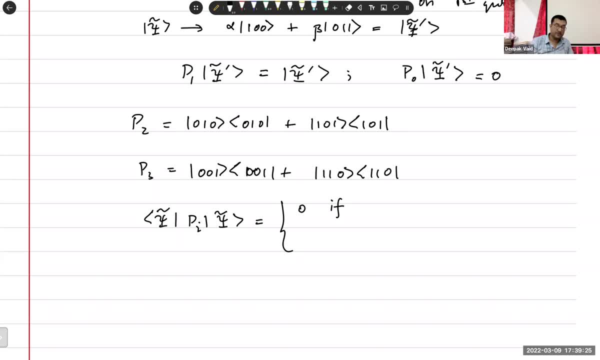 if the condition, if the i-th condition is false, right i-th condition means i goes from 0,, 1,, 2,, 3, right and 1 if it is true. If i-th condition, i-th condition meaning. 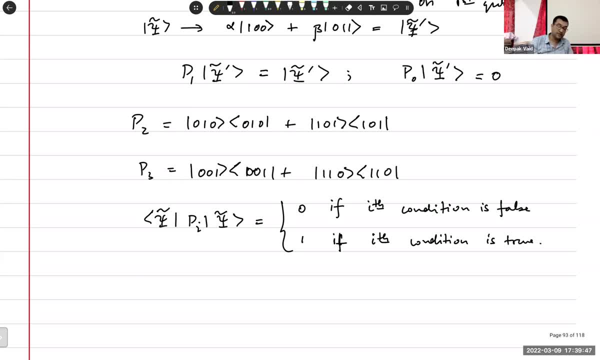 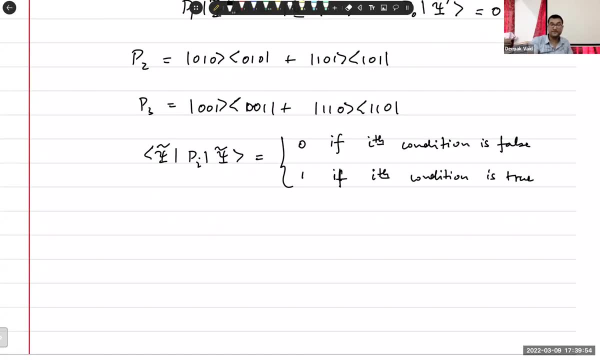 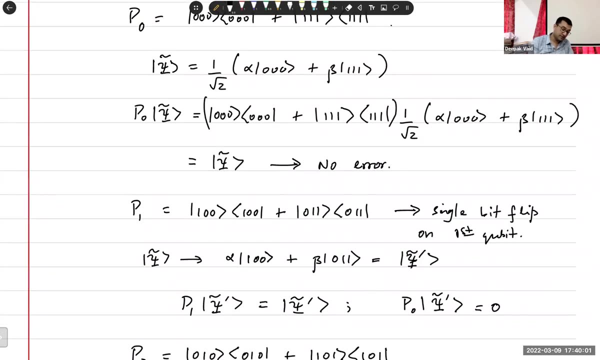 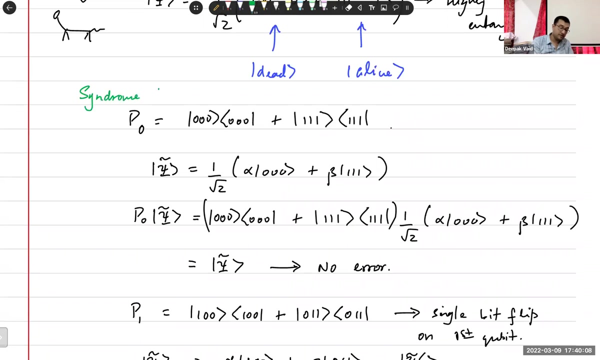 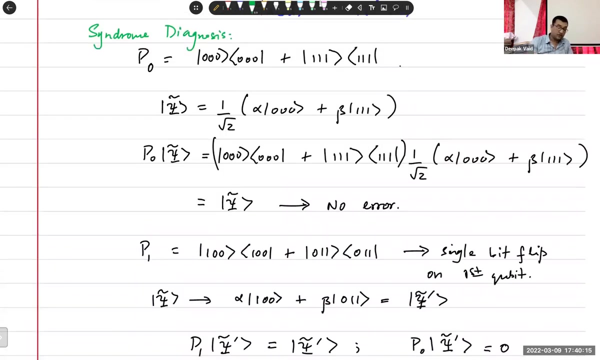 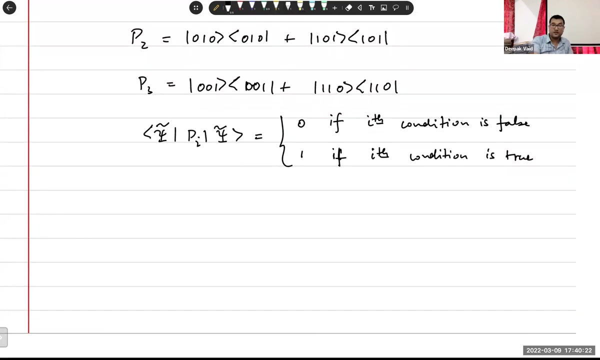 referring to the, to these projectors. so each projector corresponds to a condition that there has been a bit flip right. So this is called. this is called syndrome, syndrome measurement, okay, or syndrome diagnosis, okay. Now what is the nice thing about this syndrome diagnosis is the following: What happens to 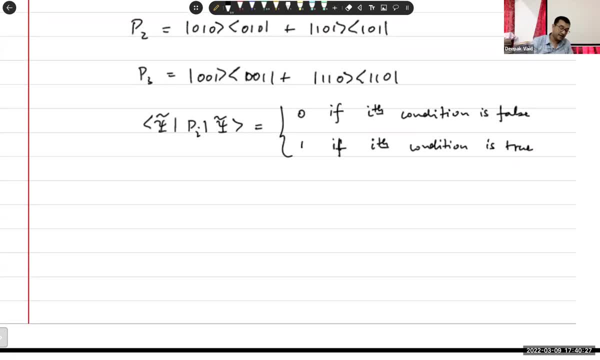 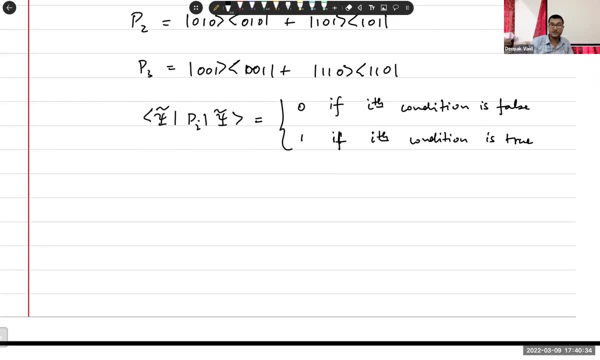 the state after you make the measurement right. So if I make the measurement of any one of these, these projectors, right, the state does not change. State does not change due to the syndrome measurement. okay, Now then the next. so 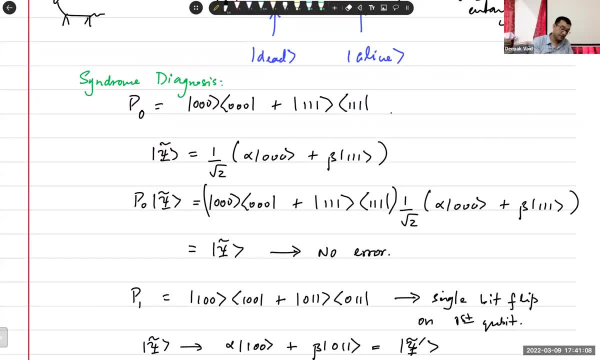 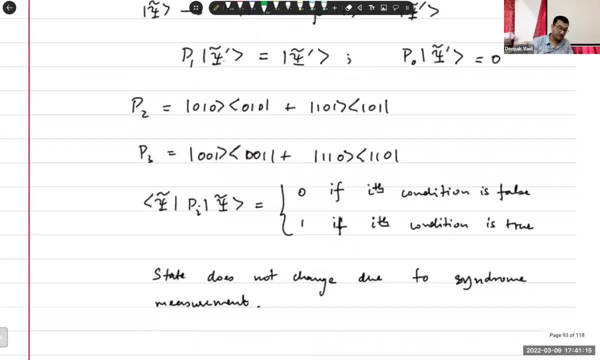 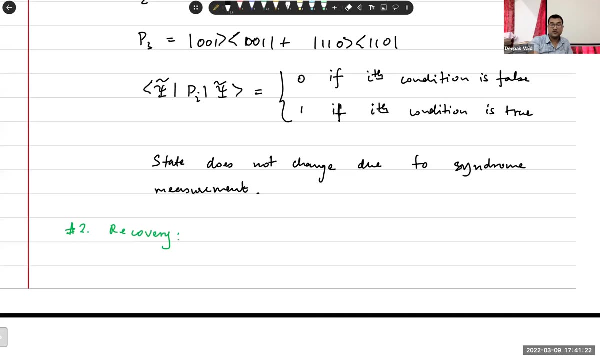 this is the first step- is syndrome diagnosis. The next step is recovery. Right? So the recovery procedure is relatively straightforward. It's that depending on your error syndrome, your error syndrome tells you what has happened, right? So if if you make the measurement of a particular situation, then the first thing is you measure theочкуpe. 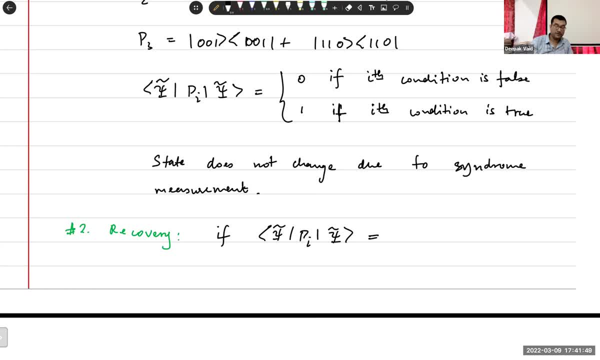 okay. and then the second step of this procedure is matrix. In the case of the matrix, you measure the control unit. Okay, So we measure the control unit, We measure the control unit. okay, So part of the control unit is: is a, is a, is a and this is value. 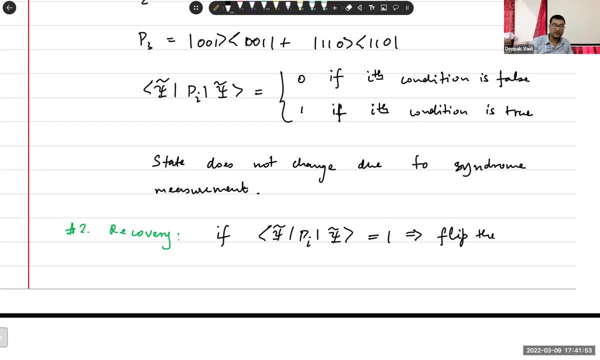 of the curve. So this value is one right. and if you measure the control unit here, Let's say we measure the curve, See that. you see this is this, is this expectation value is equal to one. This implies that you flip the i-th cubit and that will correct. 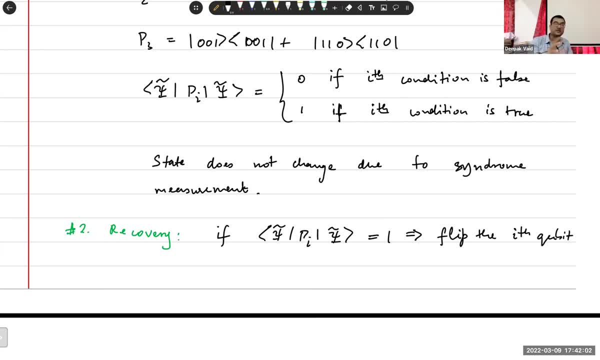 your state? Okay, And we will see why this doesn't affect the the state itself. Okay, We'll, we look at this. we look at the circuit in a little bit, and so this procedure works perfectly, provided that bit flips occur only on one or none of the qubits In the event. 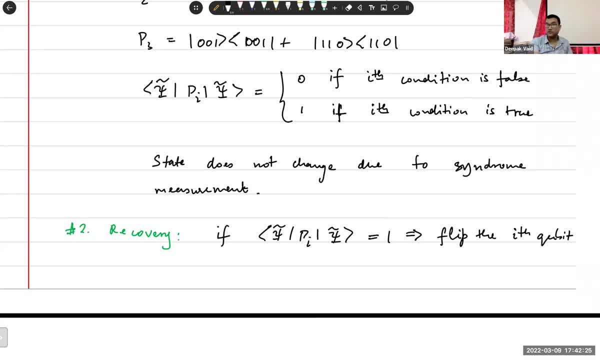 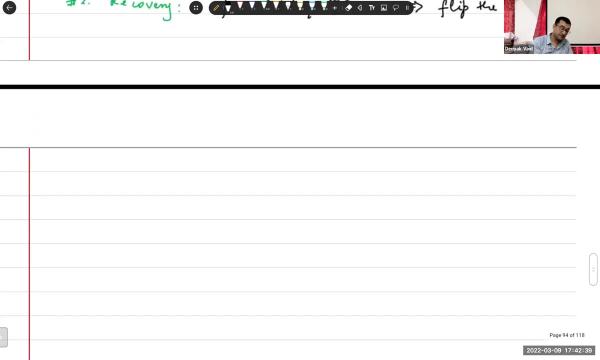 that you have more than one bit flip, it won't work. Now let's see, Let's talk about phase flip errors. What is a phase flip? So the phase flip is, as I've mentioned to you before you have some state alpha zero plus beta one in your computational basis- A phase flip. 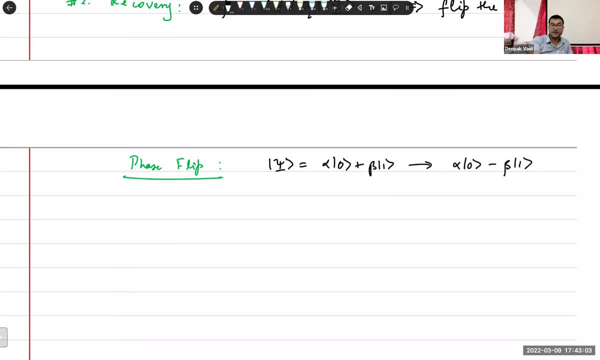 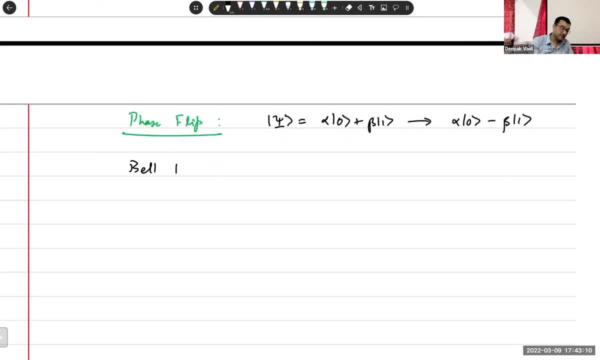 is when the relative phase between the two qubits flips. And if you work in the phase flip, in the Bell basis plus minus state is given as 0 plus minus one by root two. So in the Bell basis you can write psi as, so you can invert this relationship. you can. 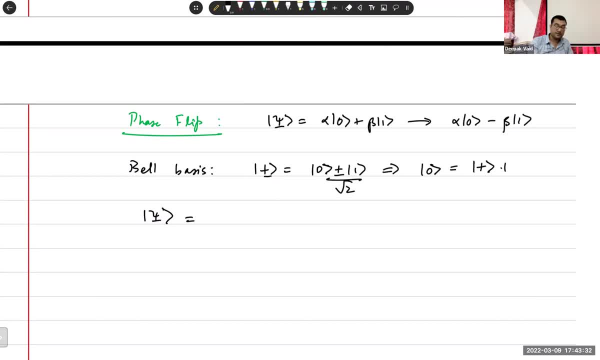 write 0 as this and one as this. Okay. so here we have a phase flip. Okay, as plus superposition of these two states, right? So if you substitute these expressions for zero and one into your state, right, What you will find is: let's see. 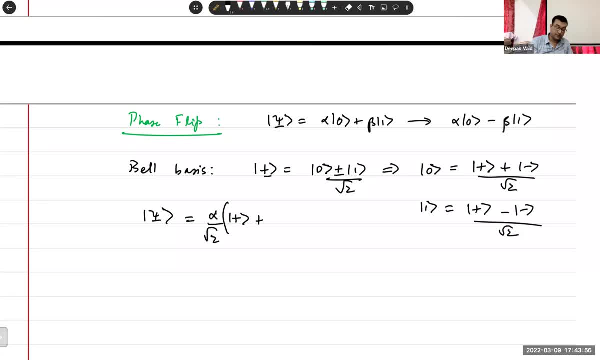 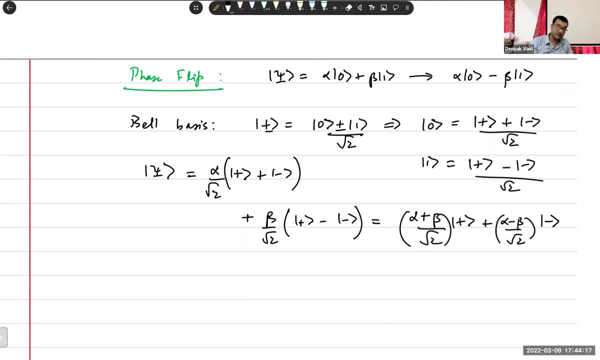 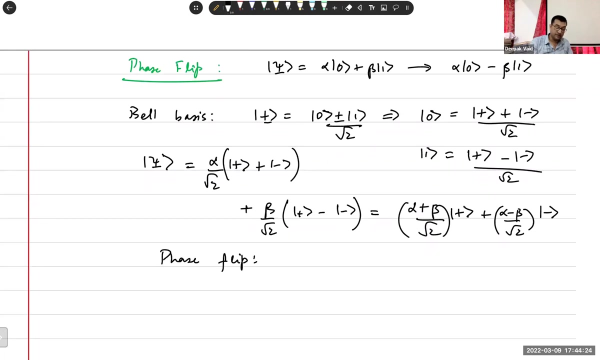 we'll get alpha by root two minus and then beta by root two right, So we can write that as alpha plus beta by root two plus right, And then plus alpha minus beta by root two minus. So a phase flip plus minus goes to minus plus right. 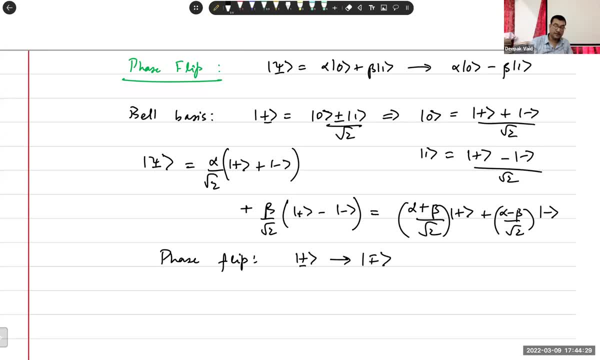 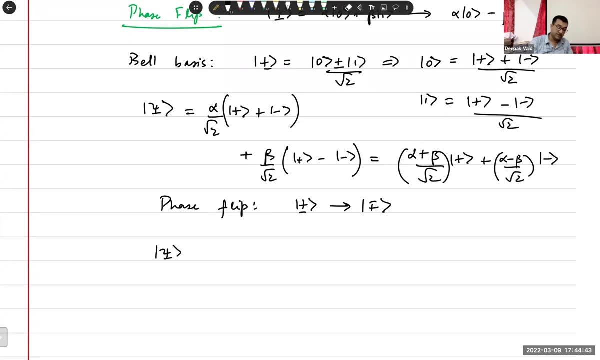 In this basis you can see that this is a phase flip right, Right. So you can see that if you have a phase flip that corresponds to bit flip in the Bell basis, right. So in the Bell basis under the phase flip. 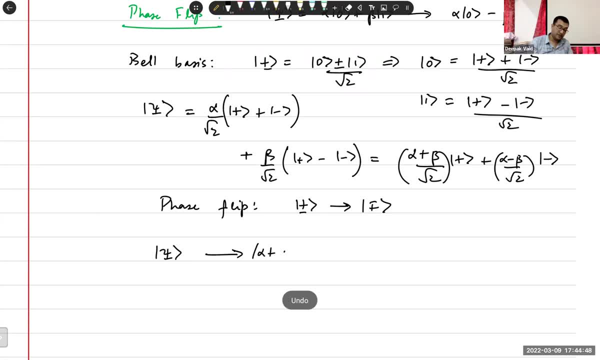 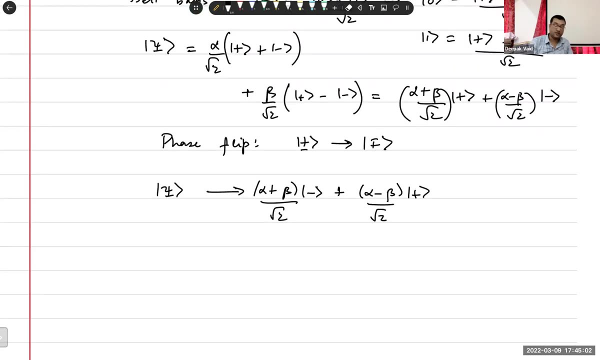 you would go from alpha plus beta by root two. this would become the minus state and this would become the plus state. So the question is that we want to protect against phase errors, right? So if you want to protect against phase errors, 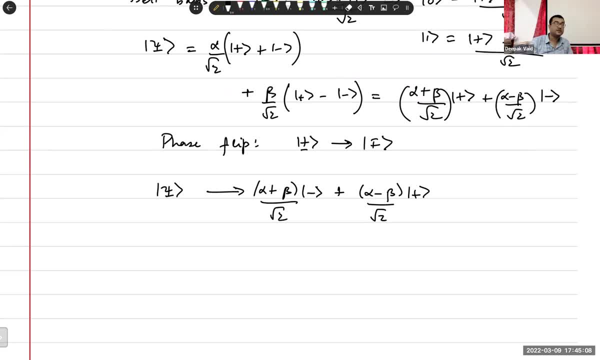 this suggests that we can just work in the Bell basis and we use the three qubit code or this three qubit redundancy, but now on the Bell basis. So that means we define these logical states as follows: So your, your, you know if 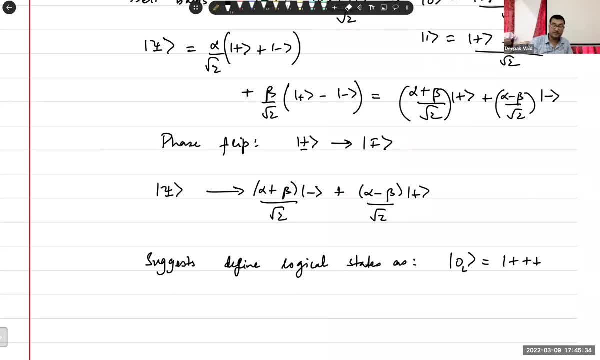 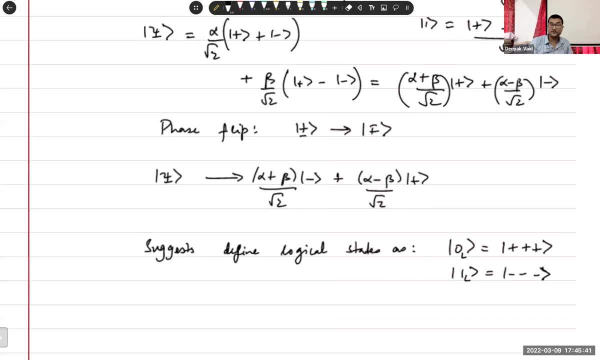 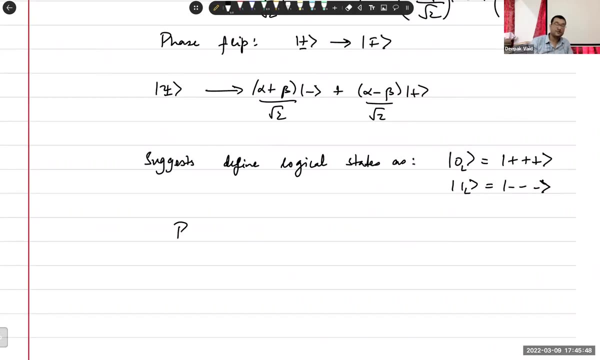 your logical zero can be written as plus, plus, plus, and your logical one can be written as minus, minus, minus. so then exactly the same procedure would follow through. you would have syndrome measurements, right operators for syndrome measurement, which would be of the same form, but now, of course, in the bell basis. 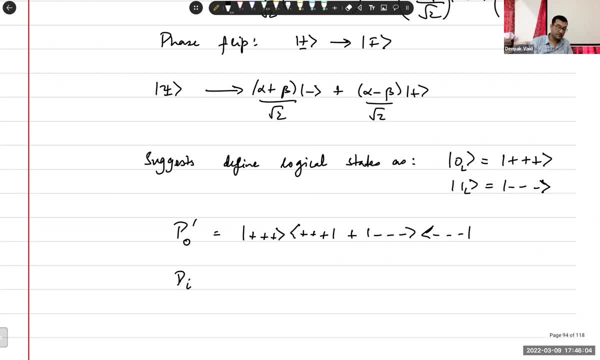 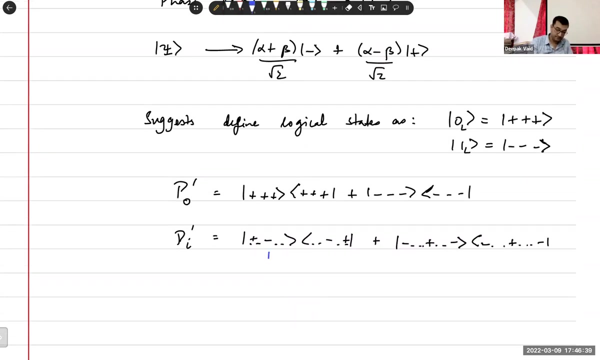 so, okay, so i'm just. this is just to show that all the qubits are the same, except for the ith qubit which is flipped in this projector. yeah, so, so like we're sure that there won't be a bit flip in the bell basis, right, no, no, no. so one second. 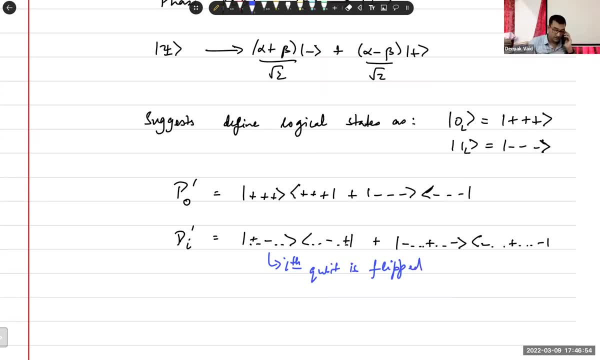 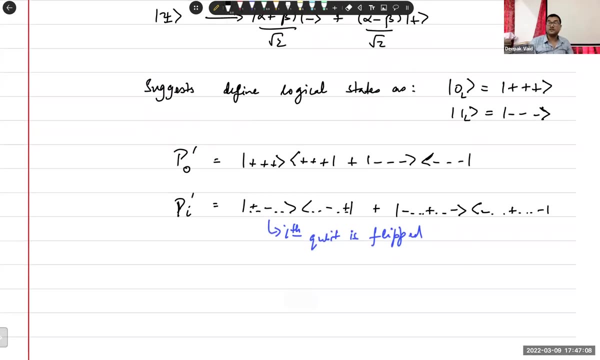 what's class is going on, so you have no idea how how much power a man has when he can hang up on his wife like that. trust me, you don't want to try it, and really you know- unless there's a damn good excuse, and being in class is a good excuse. 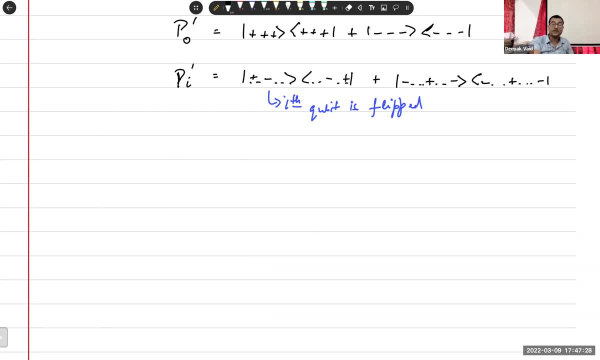 of course you won't be happy later she'd be like you hang up on me, but. but i had class, you know, okay, although you can see that i didn't see the right. so your question is that: can you not have a? uh, yeah, of course, of course you can. 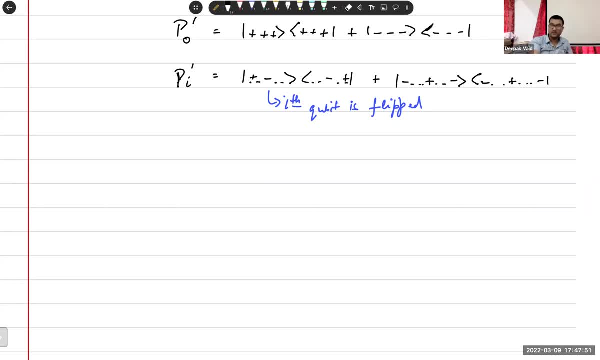 no, no, no. but the thing is that what one does is we concatenate all of these possibilities. so we will look at the, we'll look at the circuit implementation in a second right and hopefully you will. you will see what is going on. okay, just hold on to this for me, 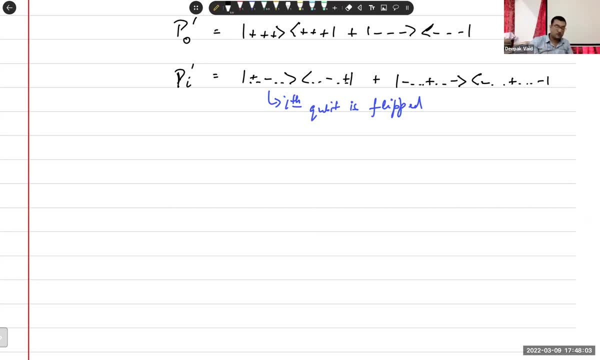 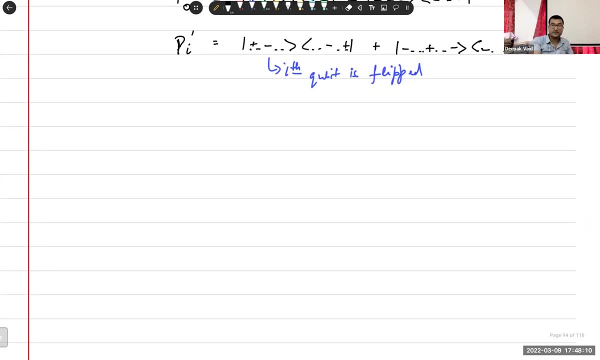 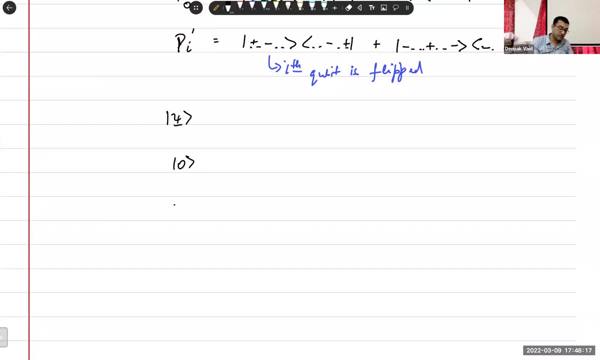 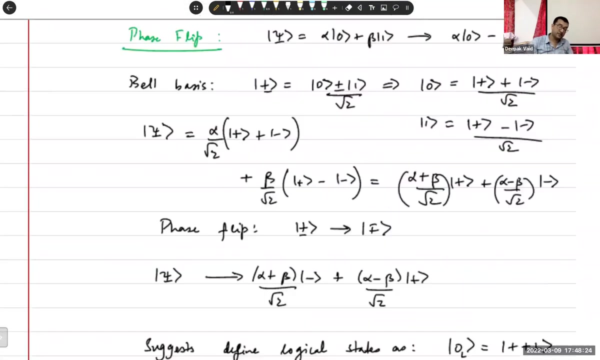 Hold on for a little bit. Now again. how do we encode our state in the Bell basis for this phase flip code? Let's write down the circuit for that. Can anybody think what the circuit might look like If you want to generate this state, the plus, plus, plus? 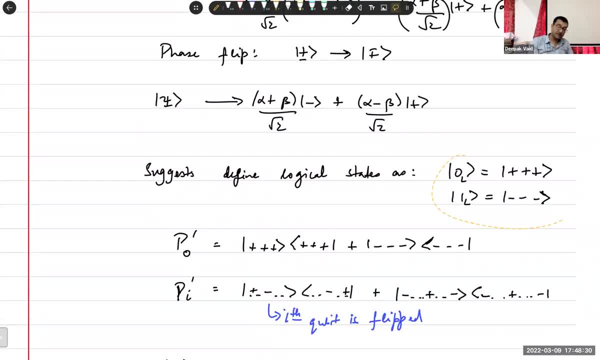 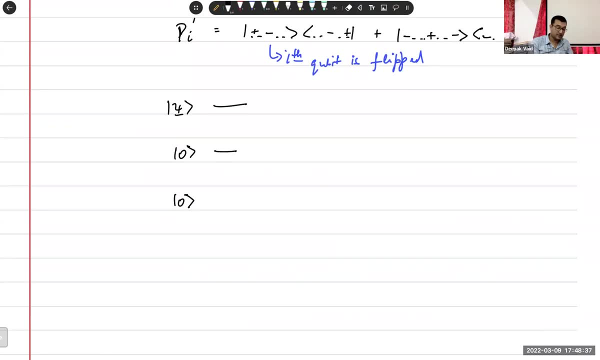 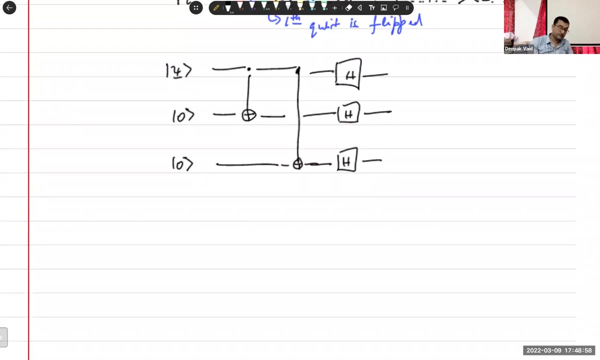 state: right, Yes, we should. What would you do? Harder mod, Harder mod, Harder mod is our friend, right? So we do our usual C0 first, OK, And then we apply a harder mod on each one of these qubits. 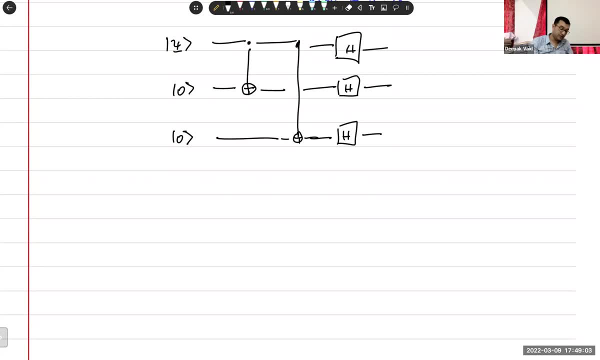 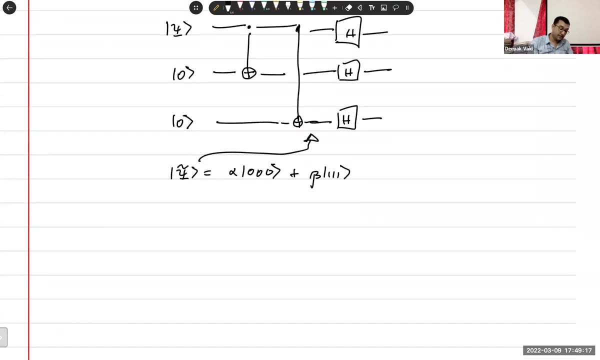 right. So if you do this, what happens? Well, you end up with: first you end up with this state right at this stage, after the first two C0 gates, And then, when you apply a harder mod, what happens? 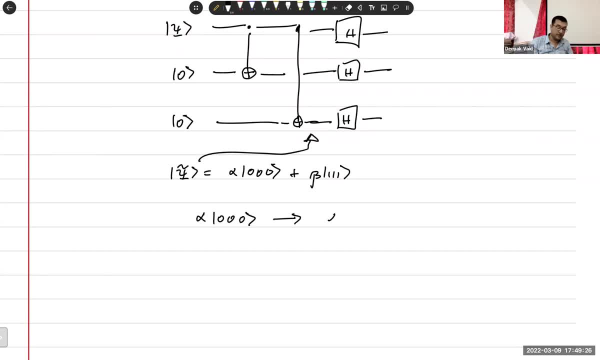 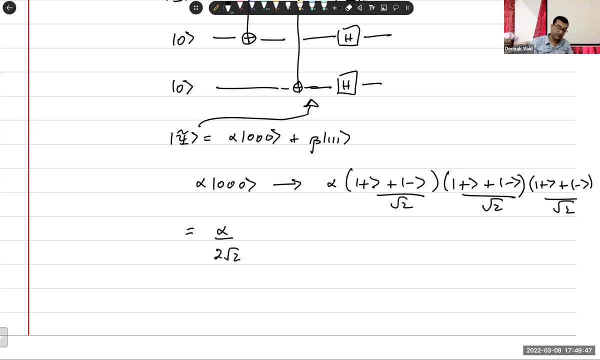 Alpha 0, 0, 0,, for instance, goes to alpha, So you replace each 0 by a superposition of plus and minus states like this: OK, And so what will you get? You'll get alpha by 2 root 2.. 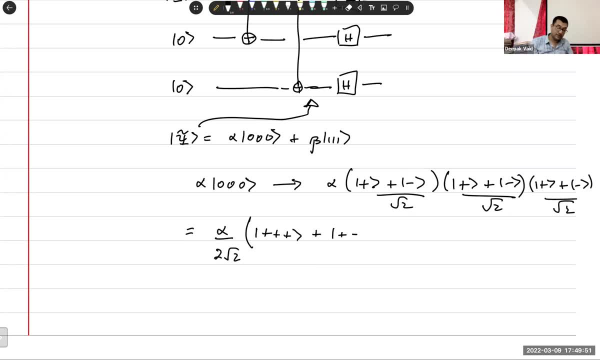 Now you'll get plus, plus, plus, plus, minus, minus, minus, plus, plus, right, like this. How many of these? There'll be eight of these, right? So you are getting all of the permutations of the plus and minus states. 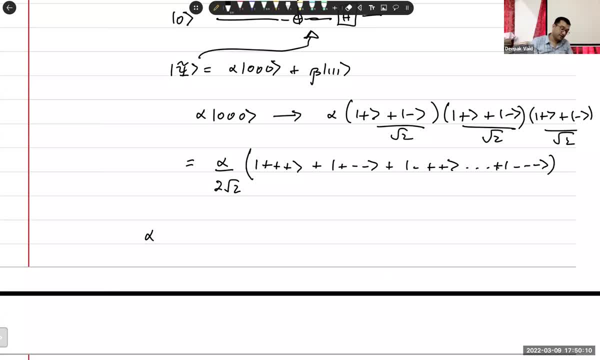 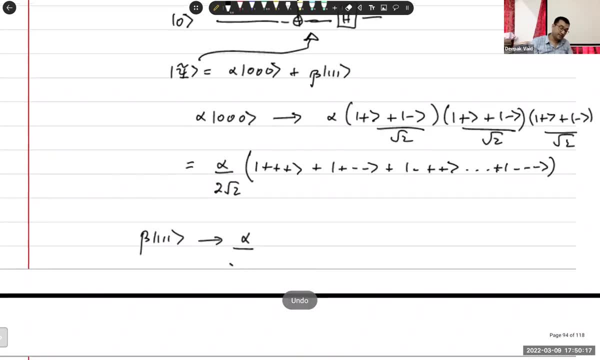 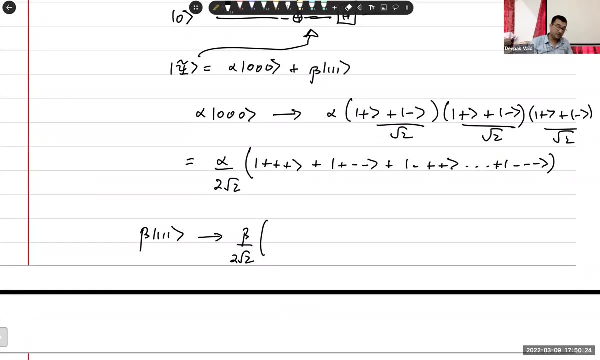 This is what happens to alpha, What happens to the beta one. Exactly, You get alternating signs depending on the number of plus, depending on the number of plus. So this is the time where alpha goes to alpha, If you can distance the number of plus from the number. 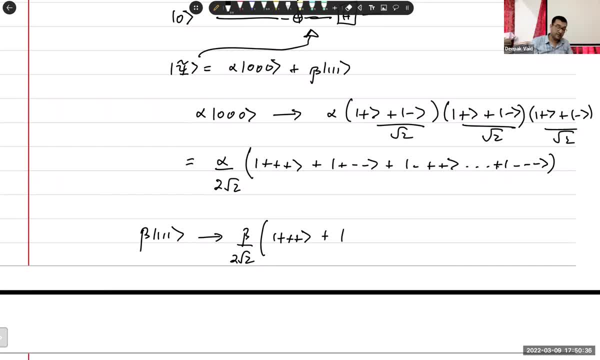 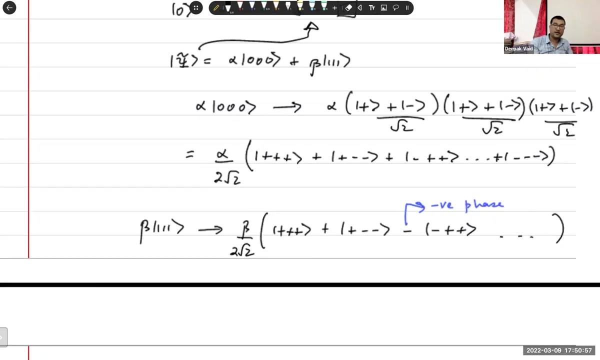 of minus qubits right. So you will get plus plus plus, right, Plus minus, minus. But then if you have one minus, you'll get a negative sign, You'll get a negative phase, OK, And so on. Now OK. 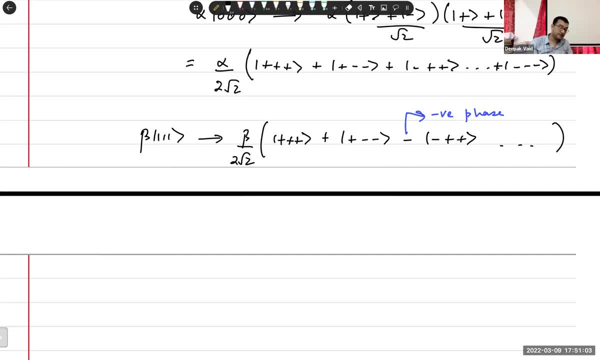 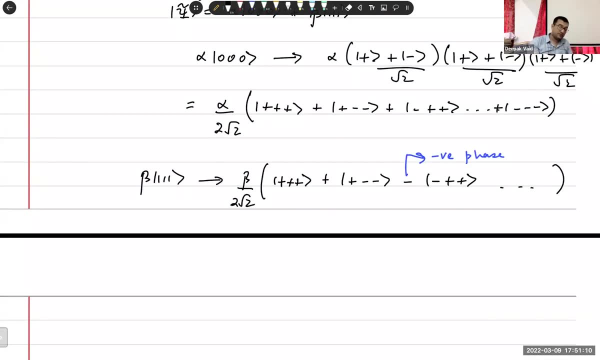 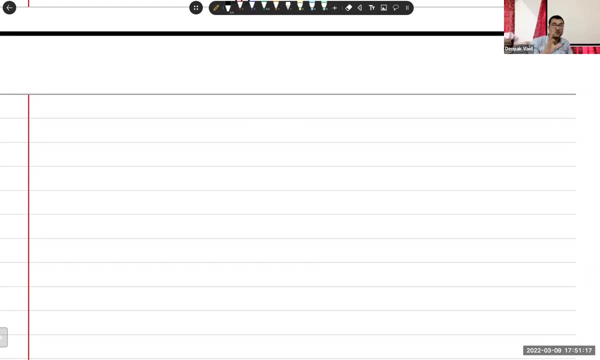 we can define this thing, similar syndrome measurements. Now we would like to combine both of these into a code which allows us to correct for arbitrary bit flip and phase flip codes. Okay, so that is called that code is called the short code. 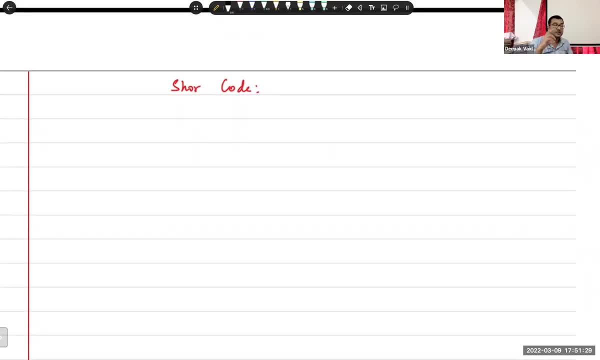 Of course, this short code is not the simplest code which is capable of doing this, but it is the first code which was discovered And of course it was discovered by Peter Shore, And it's also goes by the name of the nine qubit code. 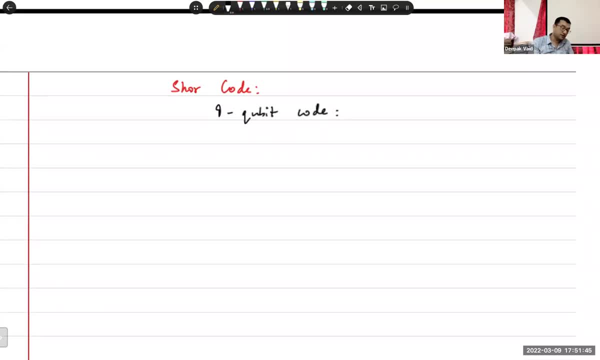 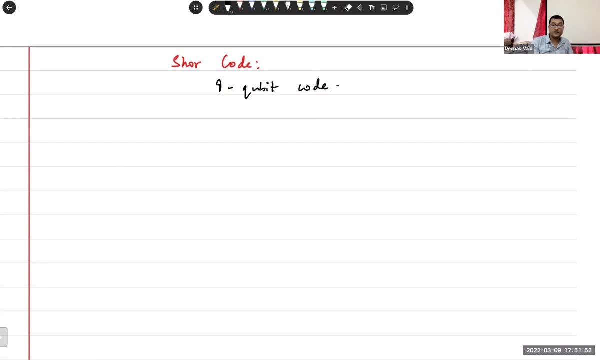 because we encode one logical qubit in nine qubits. So how do we do that? Okay, so first we perform an encoding of each qubit into the bell basis to protect against phase errors, And then we nest that coding within the bit flip code. 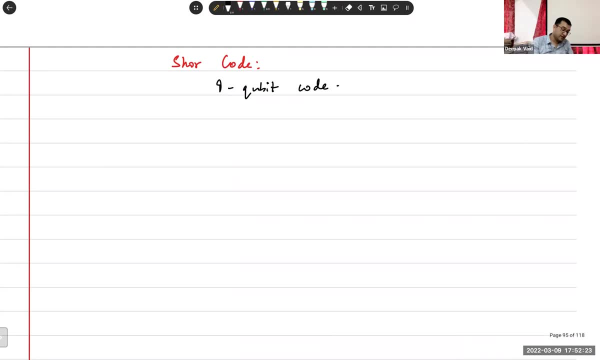 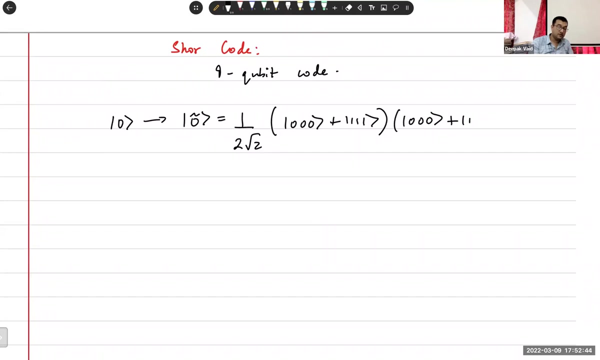 Okay. so let me write down the state and then I'll explain. then you will see what exactly is going on. So your logical qubit is written as follows: One one, one, Okay, and then similarly your logical one. 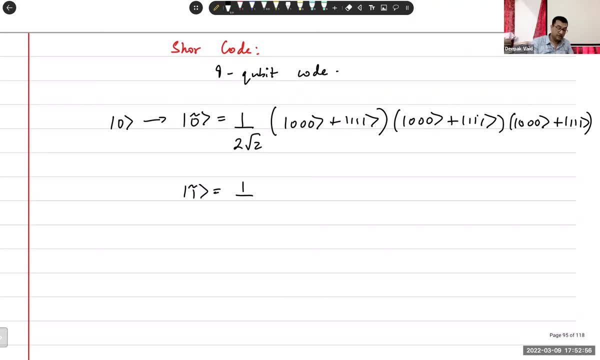 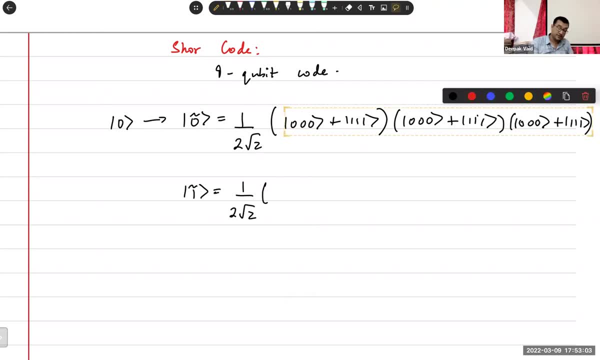 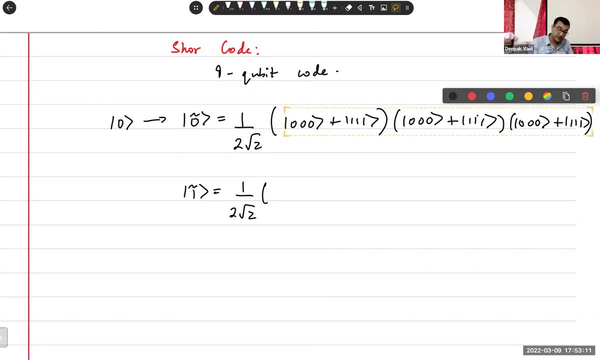 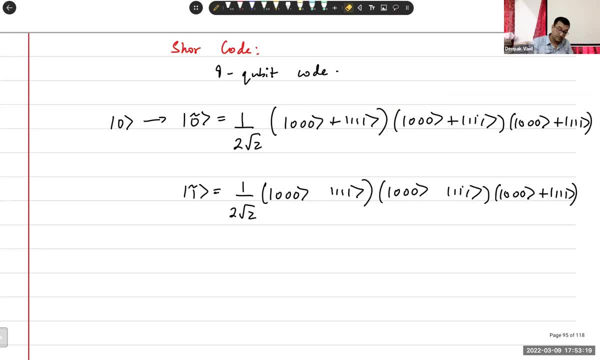 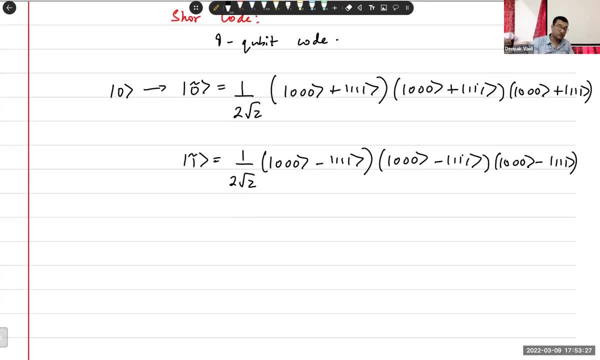 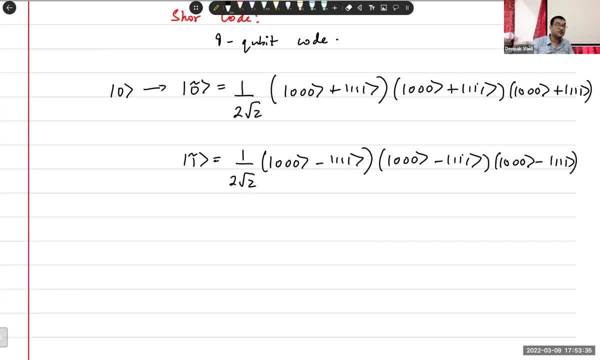 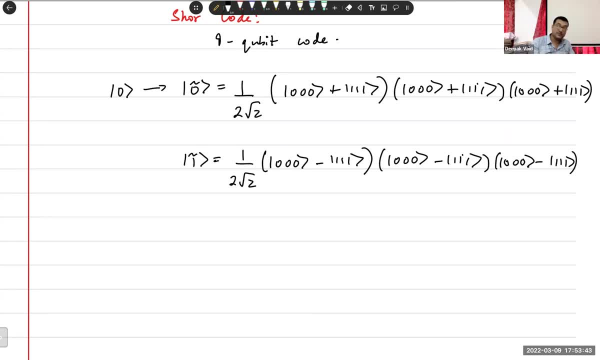 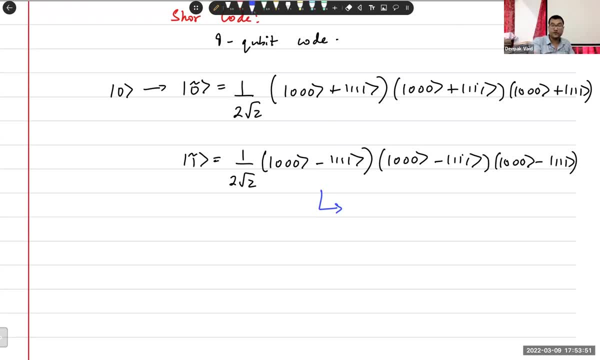 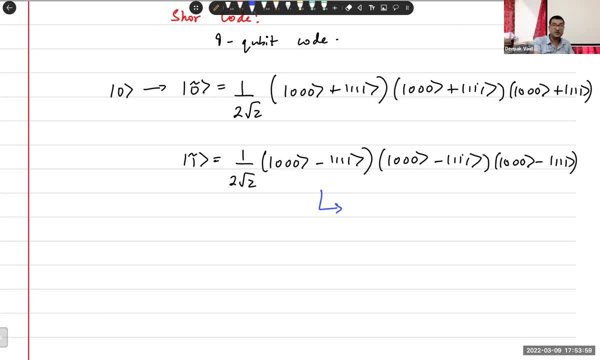 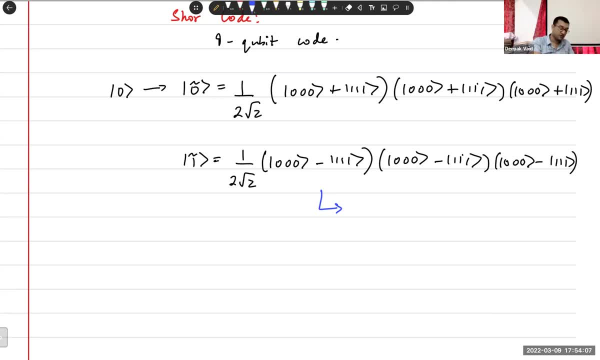 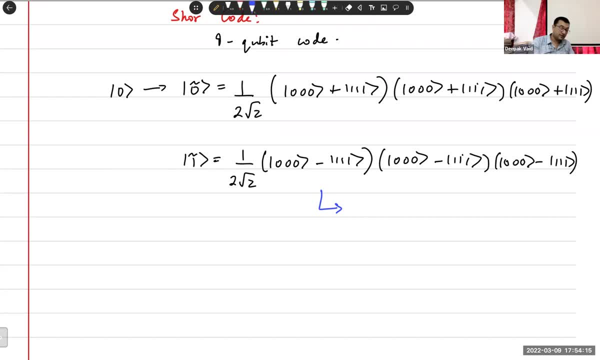 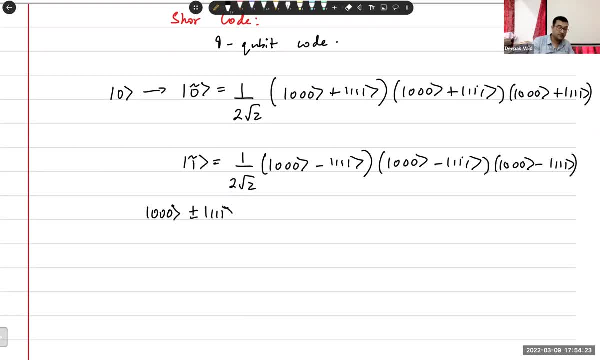 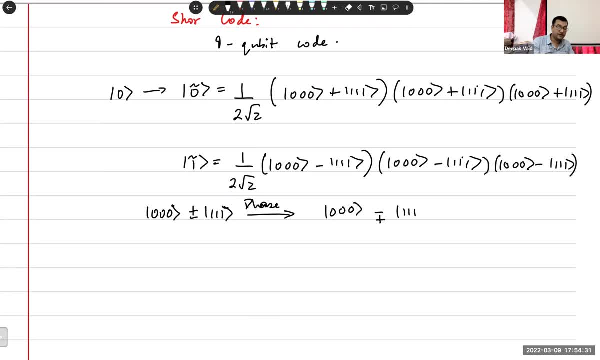 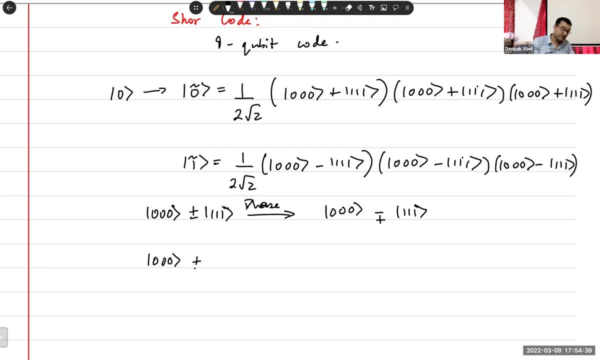 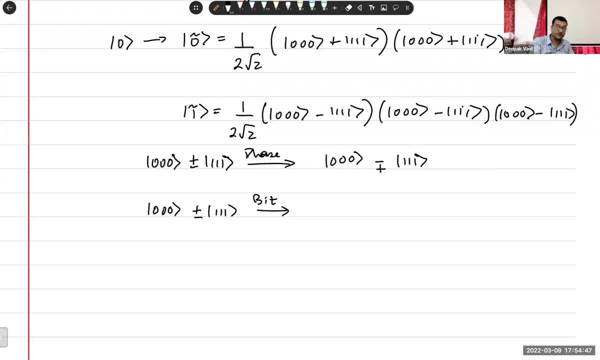 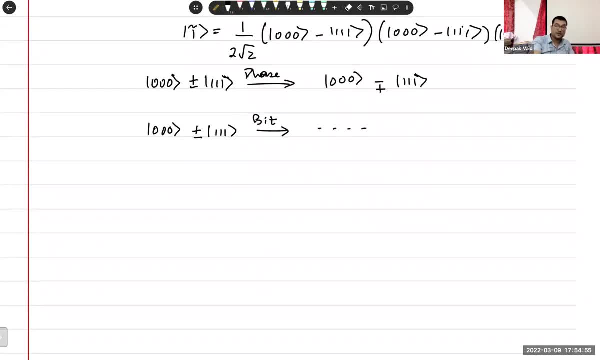 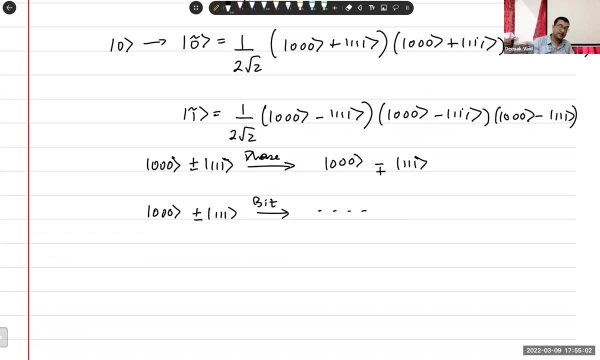 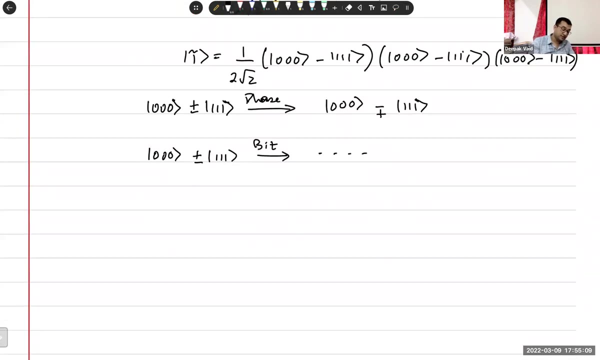 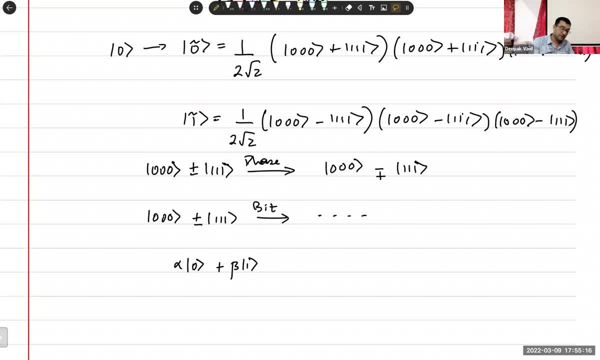 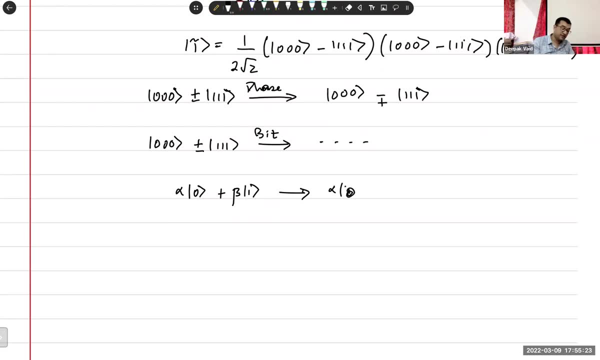 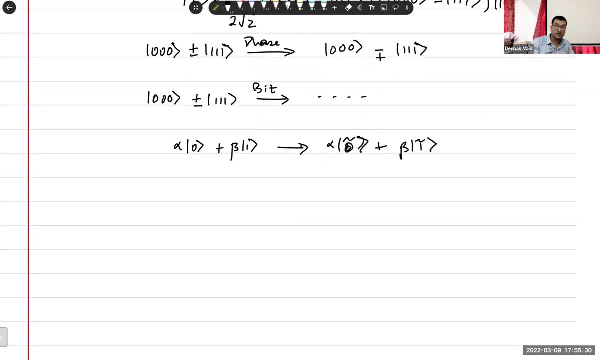 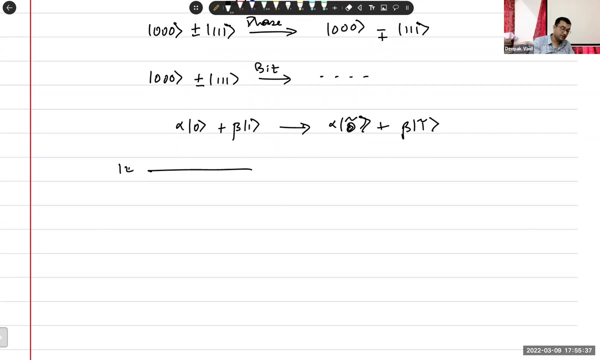 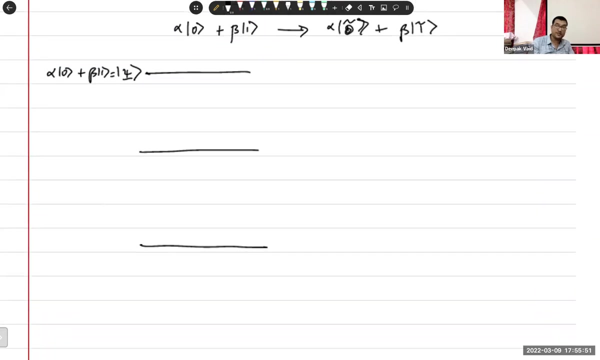 right And we want to encode it into this basis. So we want our final state to be alpha tilde zero plus beta tilde one or logical one. okay, So let me draw the circuit. This is our state, this is our initial state: alpha zero plus beta one, And then we'll have our auxiliary qubits. 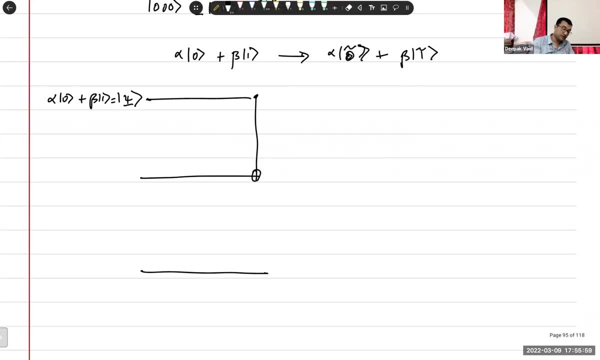 Which do the Right. So if you send it to these, to this circuit, you get the zero plus one, one one. Then you put the Hard-Mart gate on each one of these. putting the Hard-Mart gate does that transformation to the Bell basis. then, like I said, you nest these two procedures. 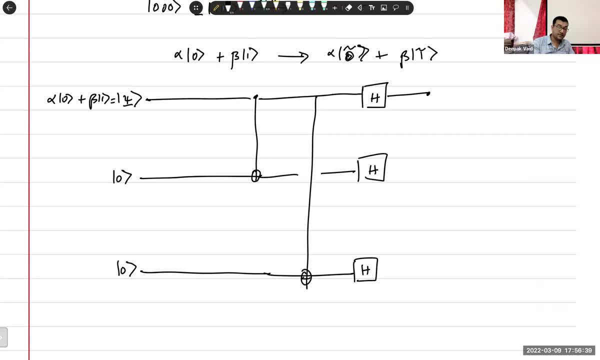 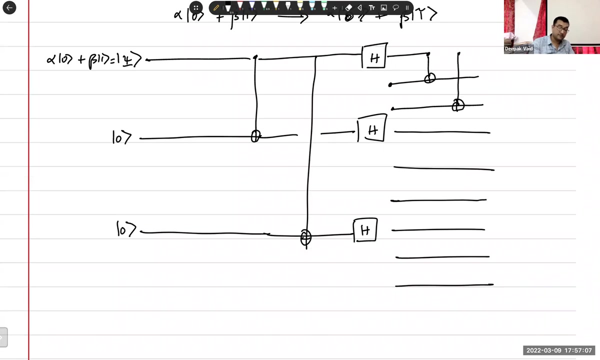 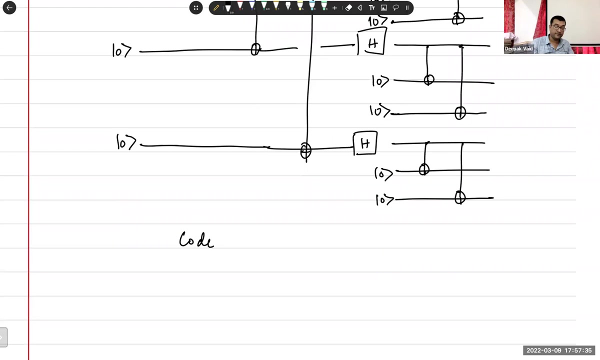 right. so nesting means we have another level of complexity nested within this one. so that means we introduce two qubits here and we'll introduce two more qubits at the next level, at the next level. so this will be zero, zero right here of the of the circuit. 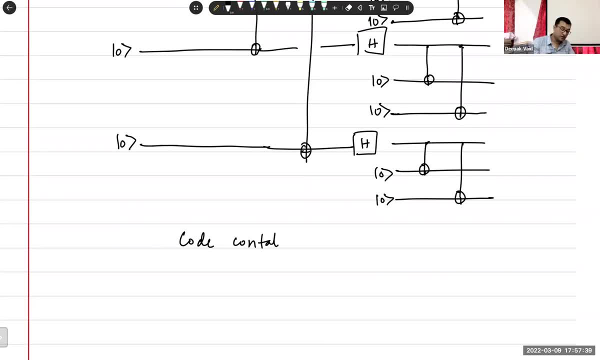 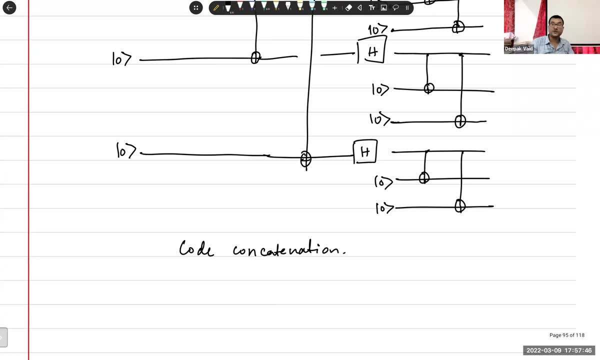 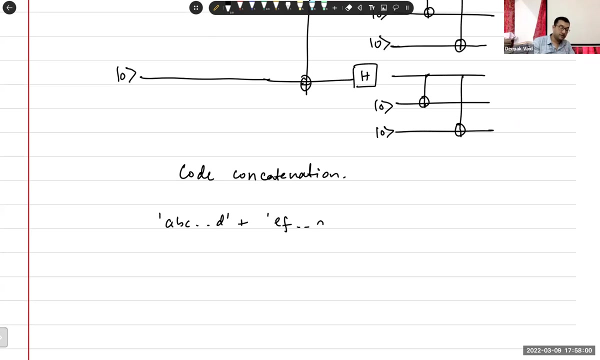 this kind of code, concatenation right. so it's like you have taken one code and concatenated it with another node. so concatenation is the term that you use, for instance, when you want to take two strings in computing right and you want to join them together. that process is called concatenation. of course, in this case concatenation has a 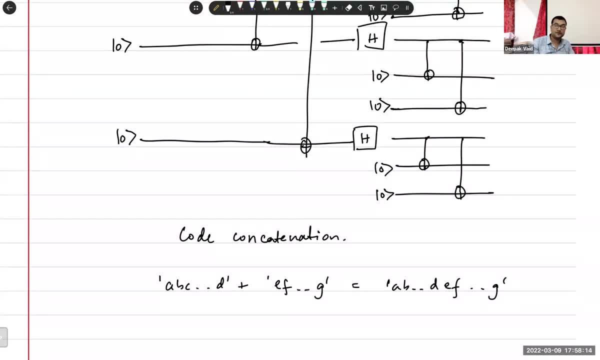 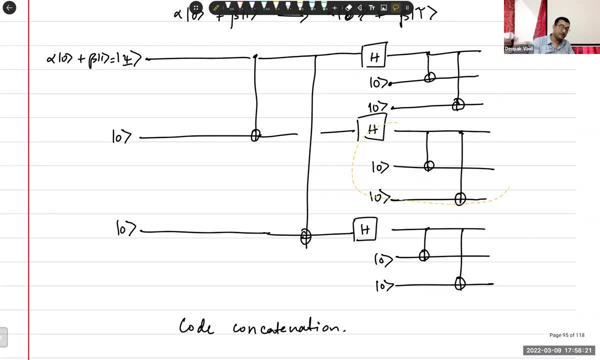 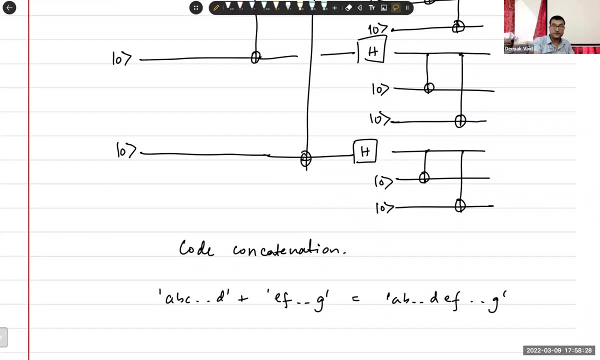 slightly different manifestation, in that it is a something that is happening in a as a nested procedure rather than as a linear procedure, right? so, rather than concatenation, I mean I would call it something else, I would call it maybe nesting or something else. but anyways, now what? okay, so now let's try to see what. 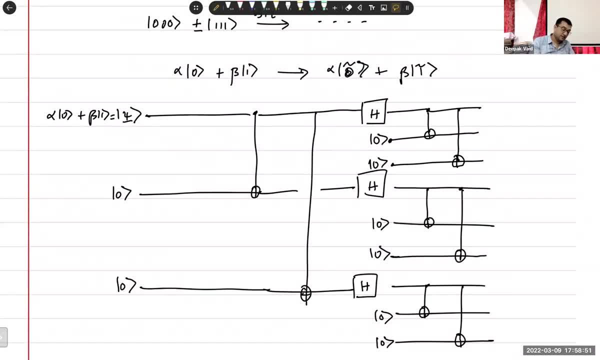 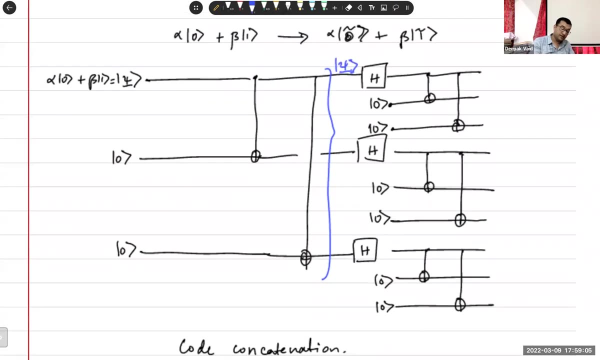 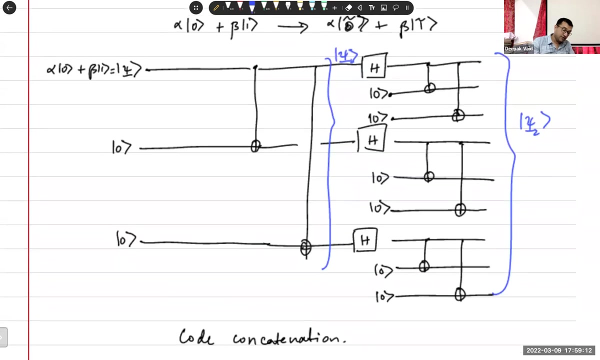 happens once again through this circuit, right? so as you come out of the first two c0 gates, right, let's say you end up with with psi 1 over here, and then we'll call whatever you get out here, psi 2, so psi 1, right, of course we know what that is. 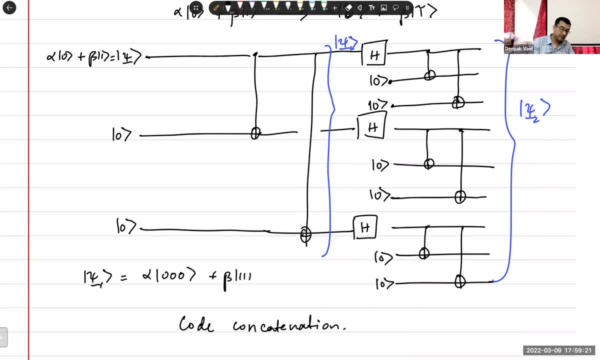 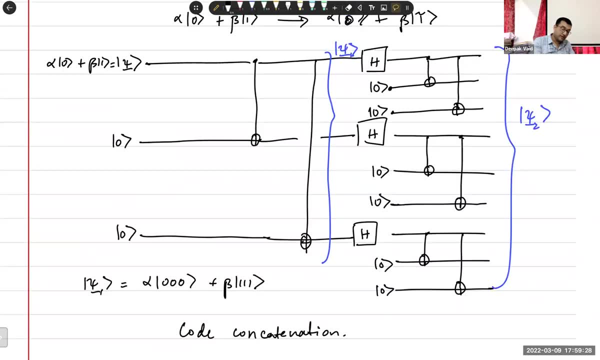 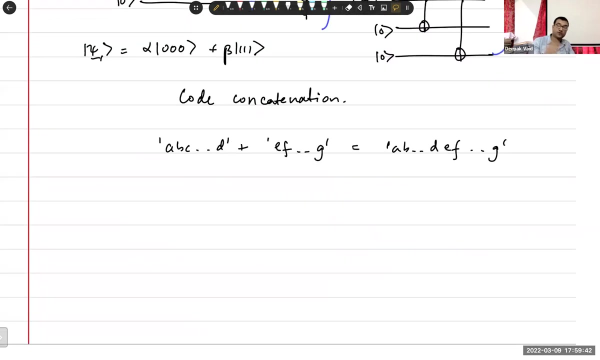 that's alpha 0 0 0. beta 1 1 1. right now, when we act, let's look at what happens with this sub circuit. right, and this sub circuit acts only on the first qubit and then it concatenates two more qubits. right, so we have alpha 0 0 0. 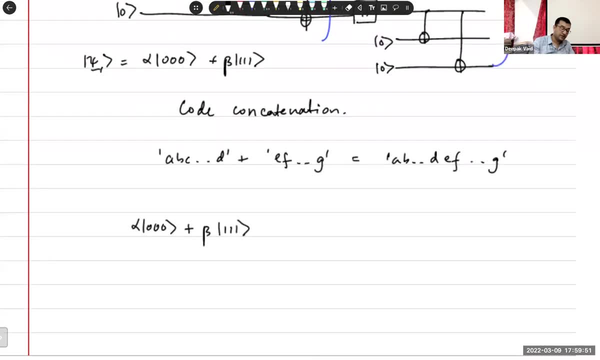 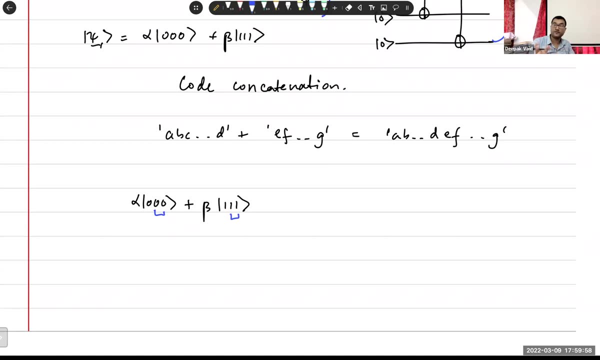 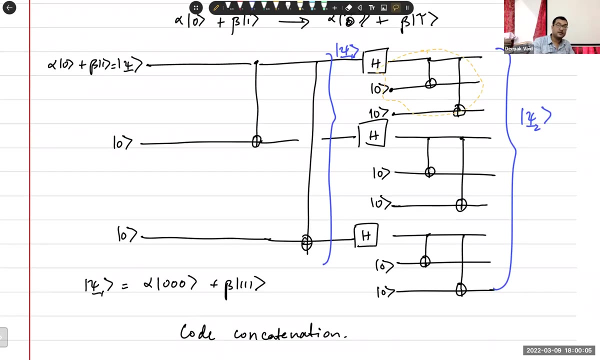 beta 1 1, 1. right, but we can. we can just take these two qubits and put them aside for the time being. right, because because these operations over here at the second level of this uh code will not affect the second and third qubit, right? 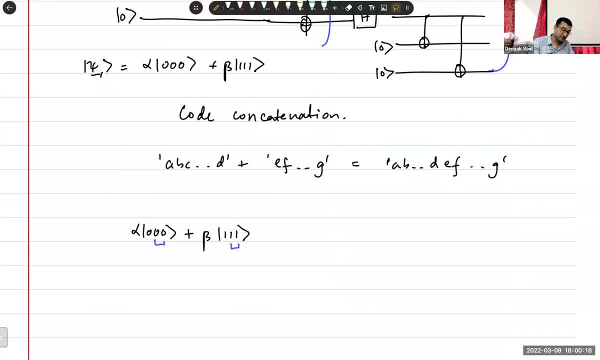 and so. so what will be the effect of of this you will go from if you apply the hard amount. you'll go from alpha by plus beta. you'll go to the hard part, basis, right and now what I'm doing is I'm working only with the first. 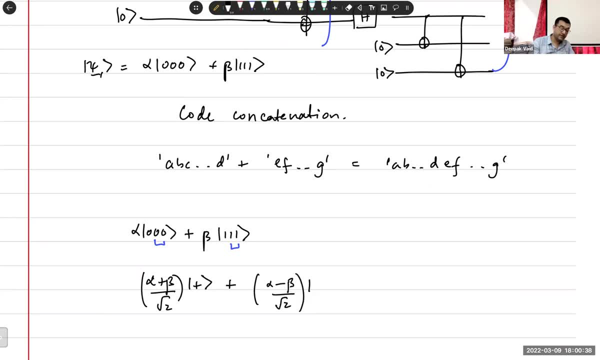 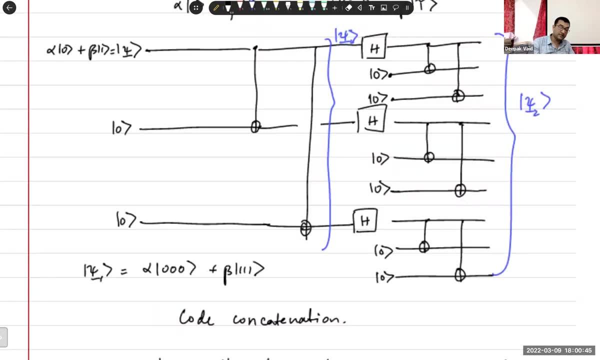 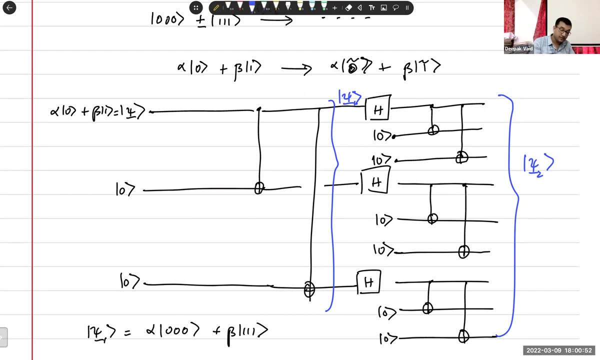 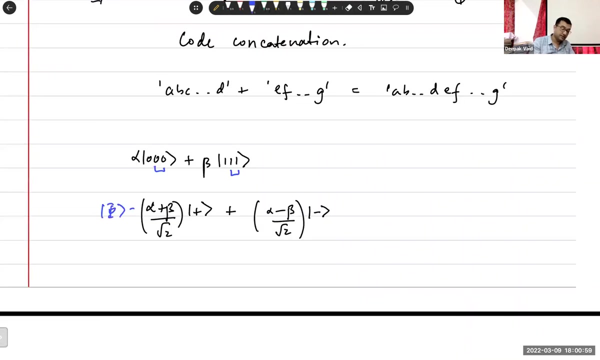 qubit. I put the second and third qubit in hibernation, right, and then, after this hard amount is applied, So let me call this uh state something else over here. let me call it phi. this state is phi okay, with qubits two and three hibernated. okay, meaning they are there, we're just not worried. 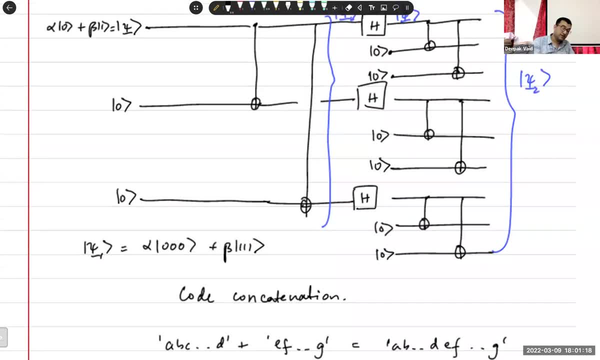 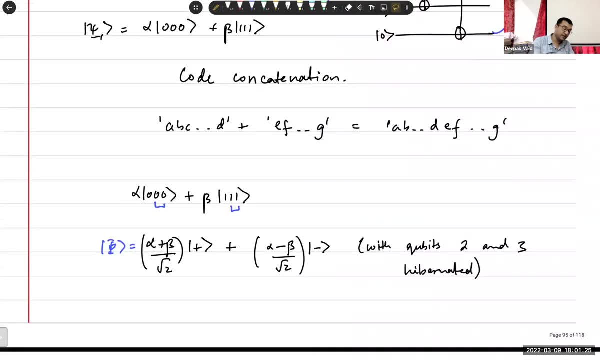 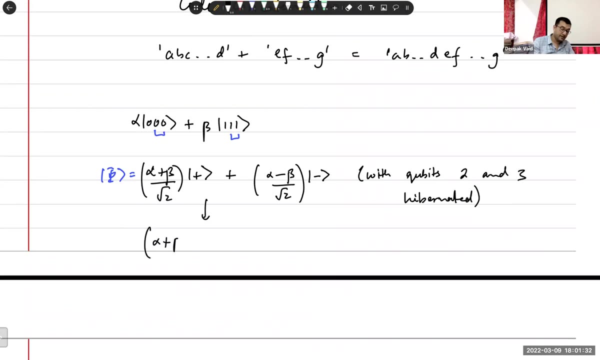 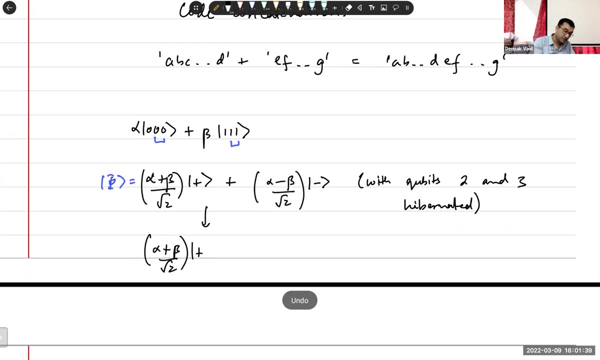 about them. we know what the state is, And then, once again, we are applying the c0 gates. what will happen if you apply the c0 gates in this order? uh, we will get alpha plus beta, by root, two plus, and now I'll just put the other two qubits in a different color. 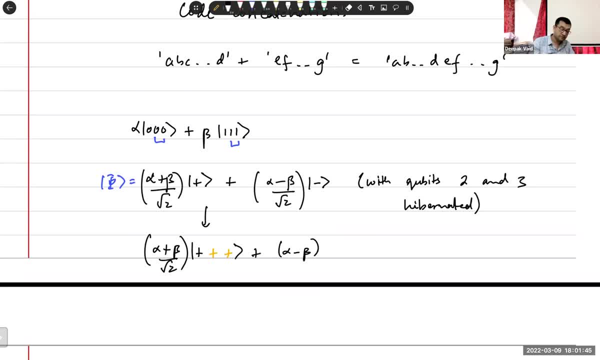 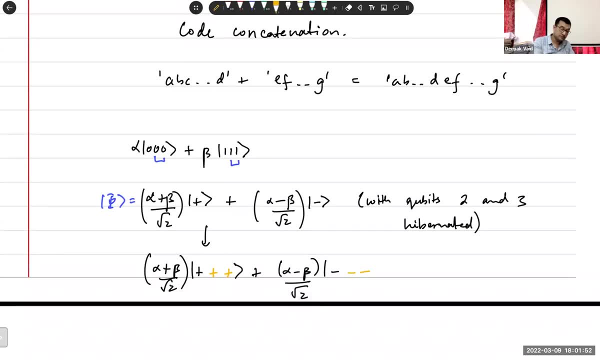 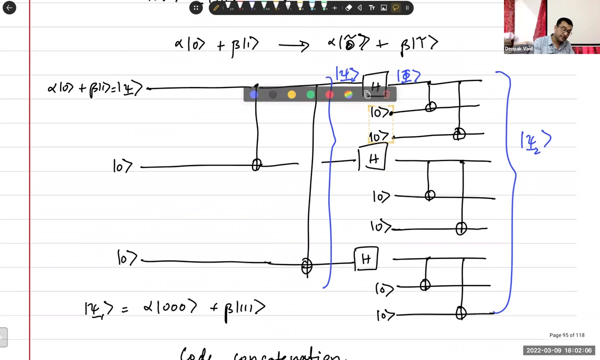 Okay, Okay, Right, and what are these two qubits that I put in a blue color? these are my, my second level over here. right, these qubits which I've introduced at the second level of my code. this is what I'm writing with the with the orange color. 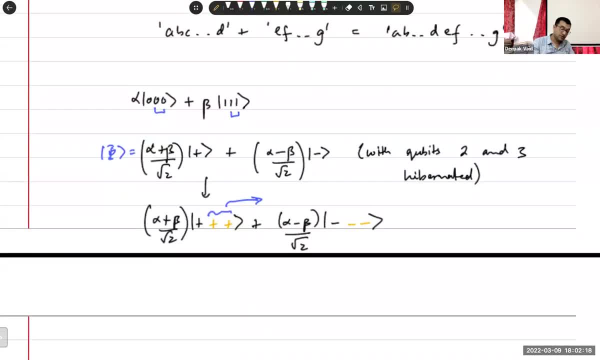 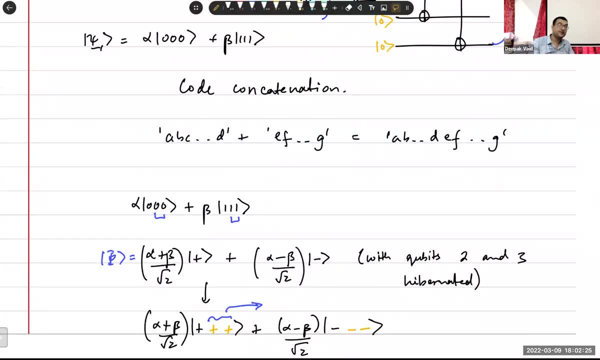 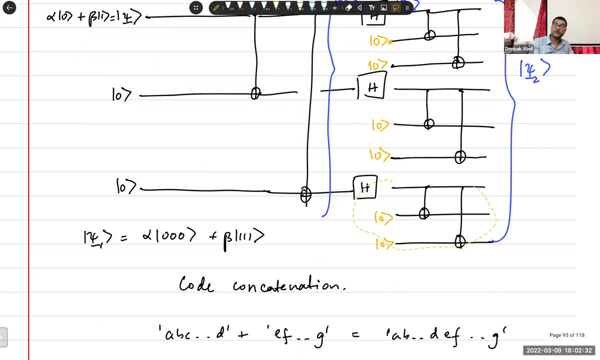 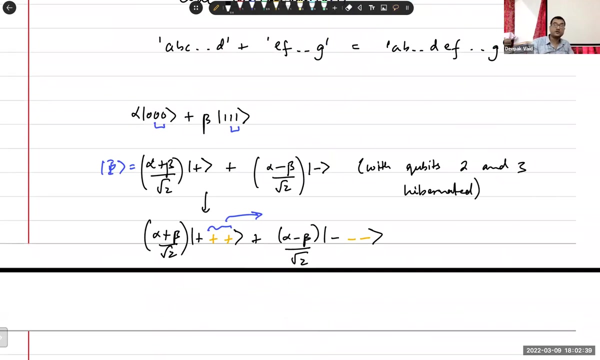 Okay, Okay. So this is what happens, uh, to the first qubit right, the same thing happens to the second qubit in the in the middle, and then the same thing happens to the third qubit, again in the middle right, and I'll leave it as an exercise for you to work out to show that the circuit. 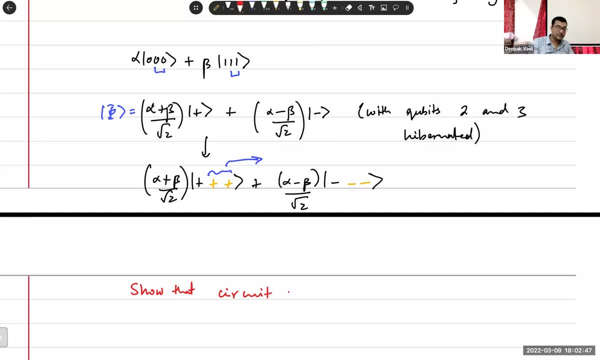 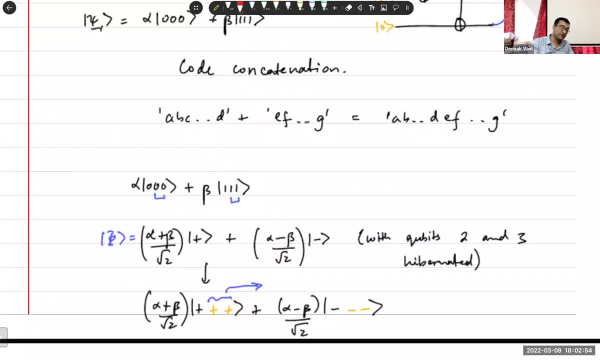 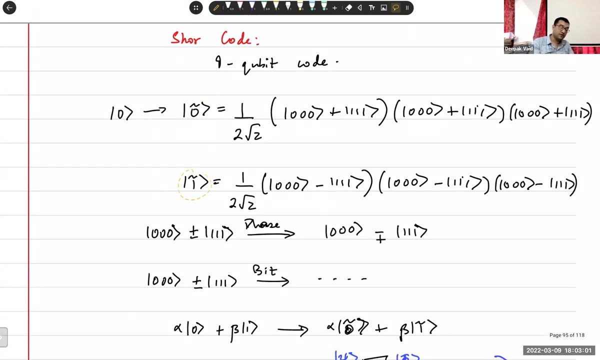 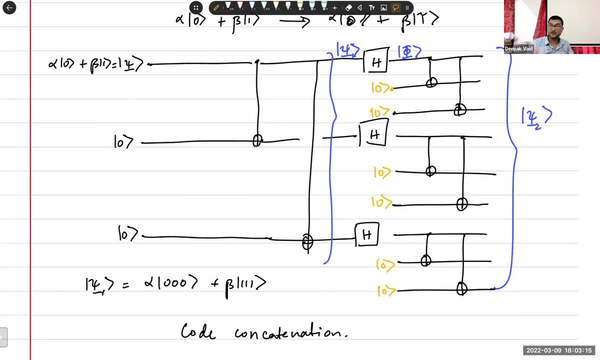 uh uh works as intended, meaning that it takes our state alpha plus beta and returns the state alpha times, logical one and logical zero, where logical uh zero is this state and logically one is this. okay, but I hope that, uh, you, you all can look at this. 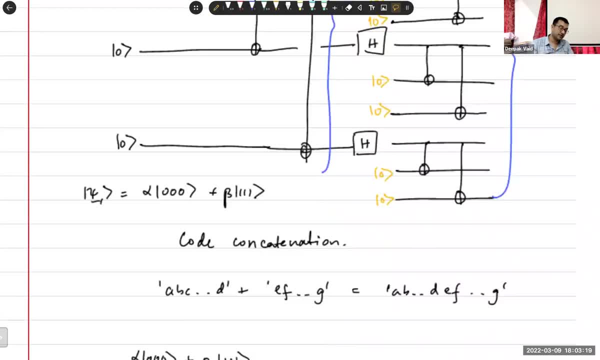 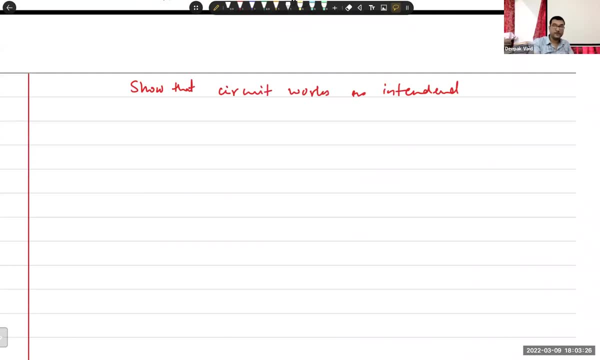 I hope that you feel reasonably confident, from what you know so far, that this will indeed be the case, but it's not completely trivial. so you should definitely sit down and work it out, because there are all kinds of signs, pluses and minuses that one should take into. 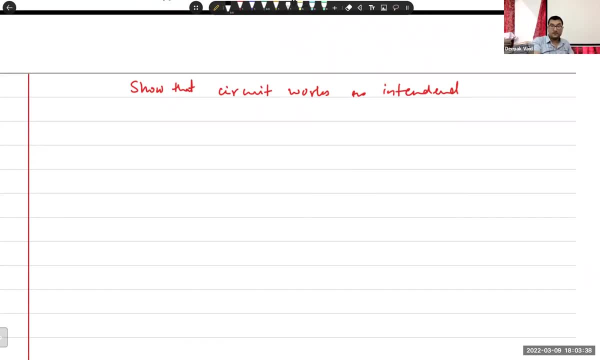 account, Okay. So now, um, what about? Okay, Okay, Okay. So what? what? how do we perform the? uh, the error recovery? right, how do we? how do we do the error recovery? so let's say that there is a bit flip error on the first qubit. 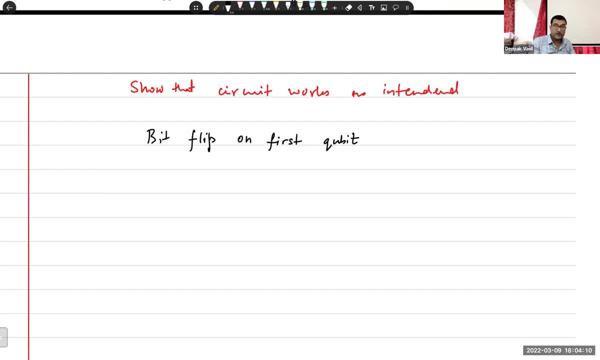 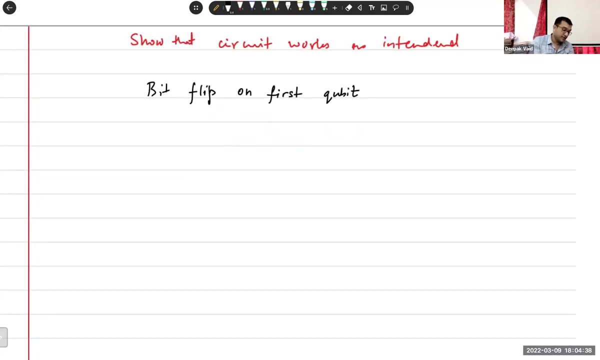 okay. so if there is a bit flip error on the first qubit, um, um, we, uh okay. so before that, actually let me go back a couple of steps and uh tell you a little bit about um, the syndrome measurement from a slightly different perspective. so I skipped that part. let me go back to that. 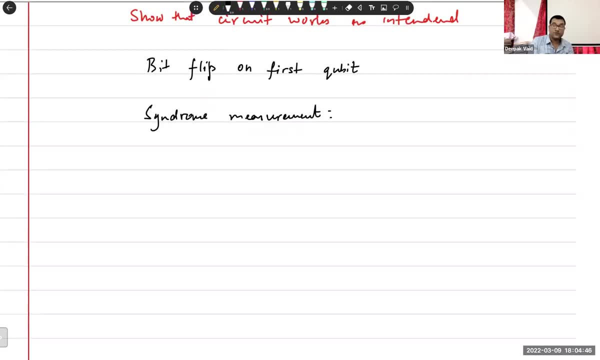 so we'll go back, for for time being, to our three qubit uh code. So we remember that you have these three, these three projectors, right for the single bit flip. Now, instead of using these projectors, let's say that we use a different set of observables. 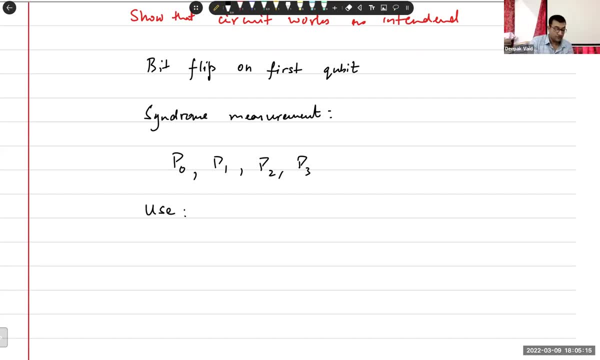 okay, Okay. So the set of observables are as follows: Z1 and Z2- okay, Z1, product Z2.. Now, whenever I have an expression of this form, what does this actually imply? Z1 is acting on the first qubit, Z2 is acting on the second qubit. and what is acting on? 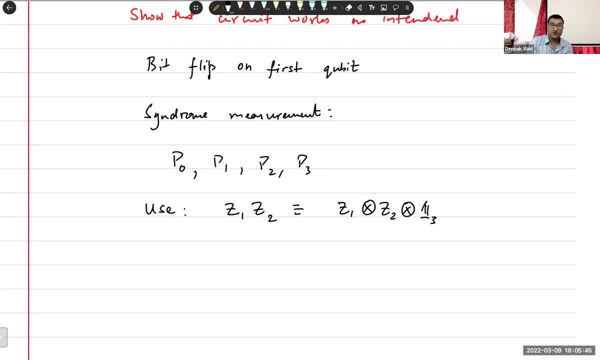 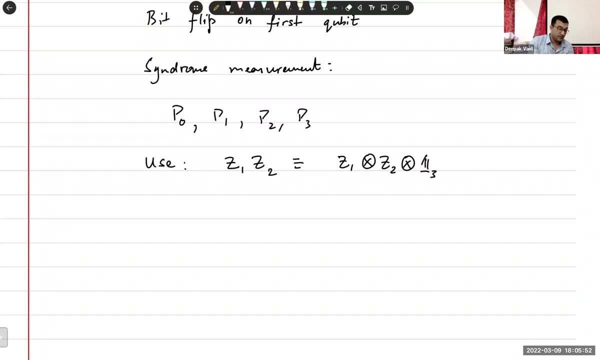 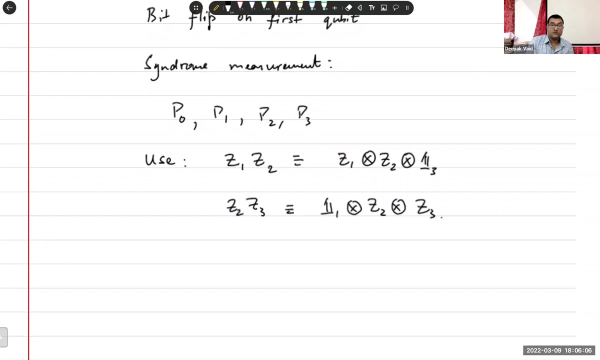 the third qubit, Identity. okay, so we'll be using this kind of an uh of notation. so, for instance, Z2, Z3 will be I identity, then Z2, then Z3, and so on. okay, um, now if we ask, what is the eigenvalue of? 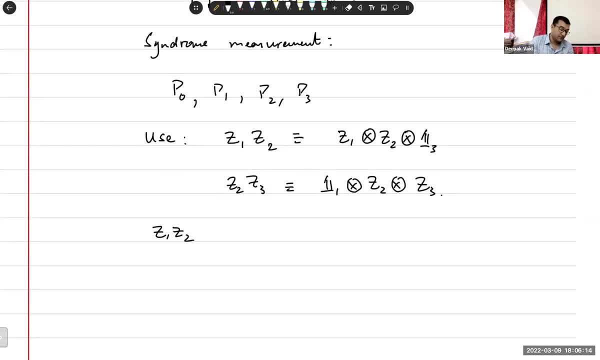 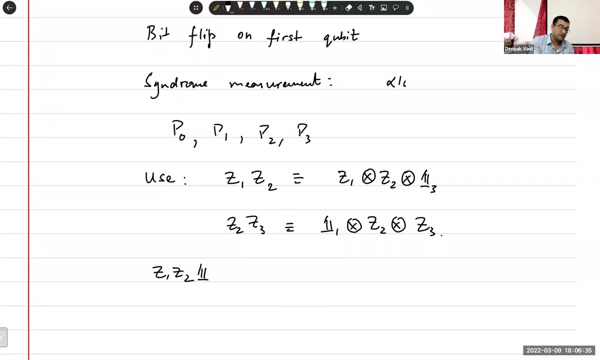 this of this observable Z1, Z2. okay, so just to be um, just for the sake of clarity, I'll put a one at the end. okay, to indicate that fact that this is a three qubit operator. and now we are going back, we are talking about our, uh, three qubit state. 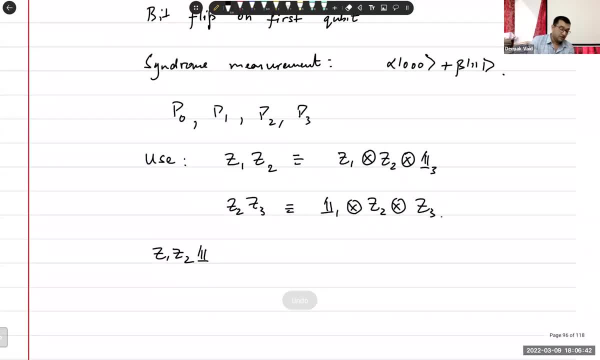 Okay. So if I ask, what is the eigenvalue of this, of this operator, right, what are the possibilities, what are the possible eigenvalues? what is the eigenvalue of the Z operator on on a single qubit, the Z operator, poly Z operator: One, zero, zero. 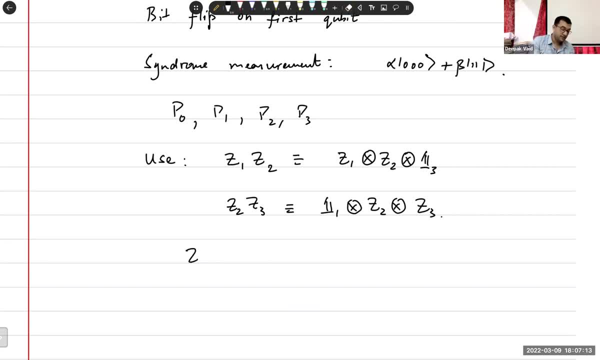 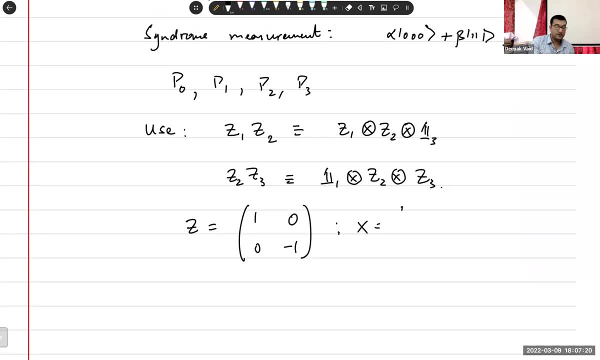 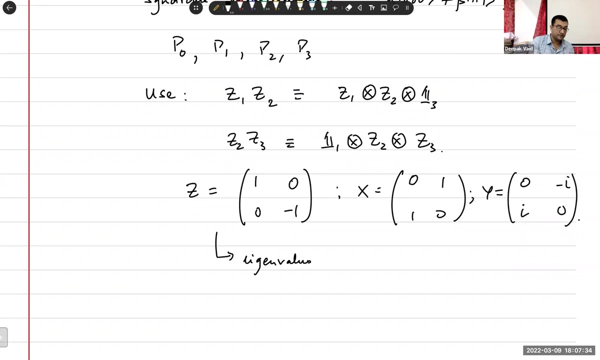 Poly Z operator. Okay, Is one zero, no forget about the H bar- just one minus one. so the eigenvalues of this of the Z operator are one plus and minus one, right? so what will be the eigenvalues of any product, of, of Zs? 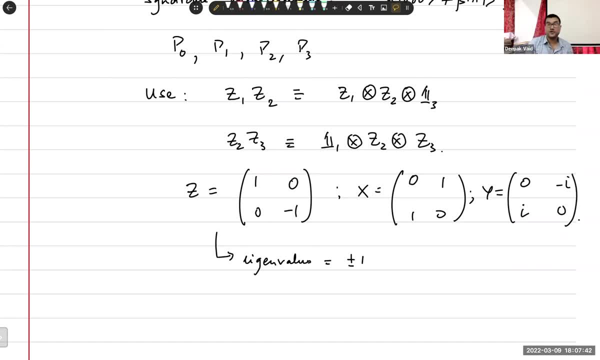 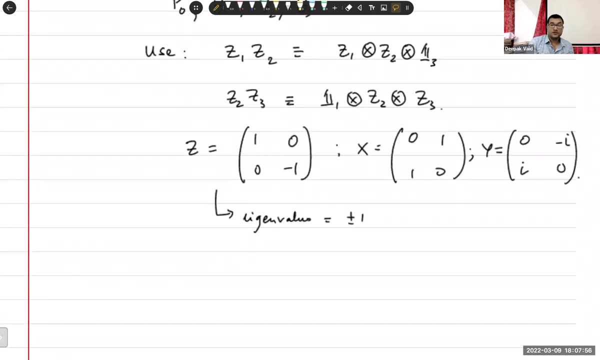 It can only be one, Okay, Okay, Maybe plus one or minus one, right you can. you will have some combination of pluses and minuses that we give you at the end, plus or minus one. So, uh, so let's say that we have, we use two of these observables, we use Z1, Z2 and then 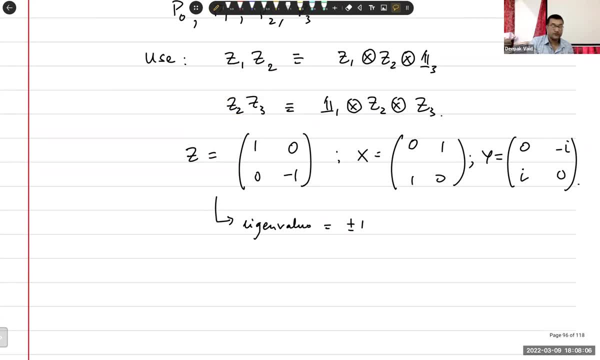 we use Z2, Z3 and we perform a measurement of both of these right. So this, This gives us as a. as a result, if you perform a measurement plus or minus one, This gives us a, an eigenvalue Plus or minus one. 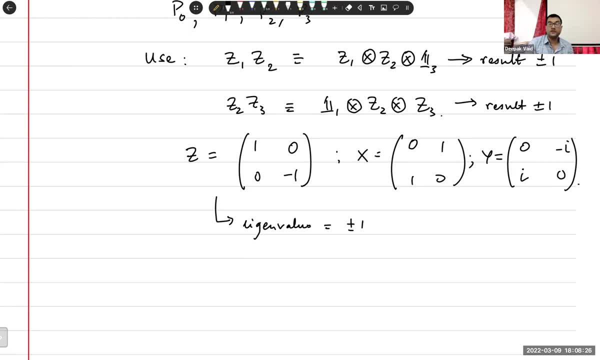 Right, So each one of these is giving us a single bit of information. Uh, Utsav, can you just go and, like, tell those people to be quiet if they are still there Or not. Okay, Go and shout at them, Yeah. 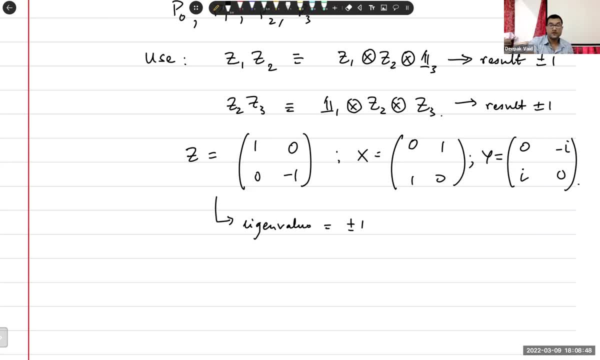 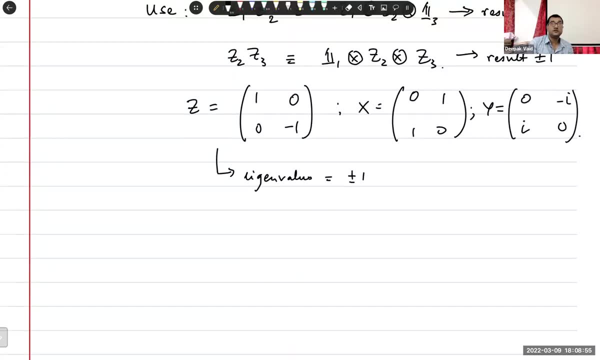 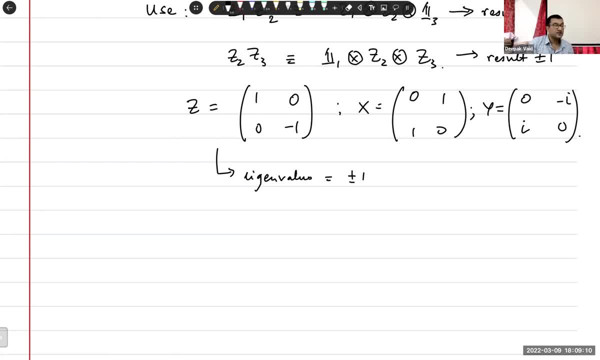 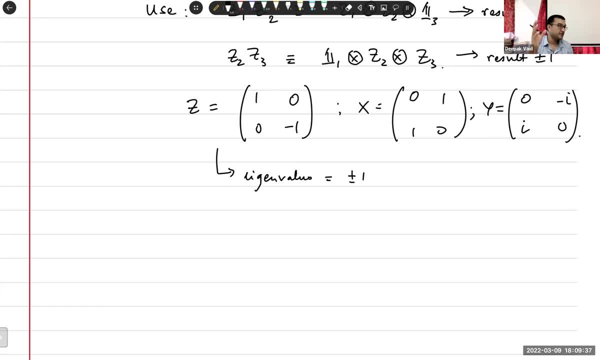 So you do. you cannot be one be one denser Identity Eight already a three qubit operator. So if you take P with tensor identity, how many qubits are you acting on? Nine? No, so we are not talking about the nine qubit code yet We're talking about the. we're looking 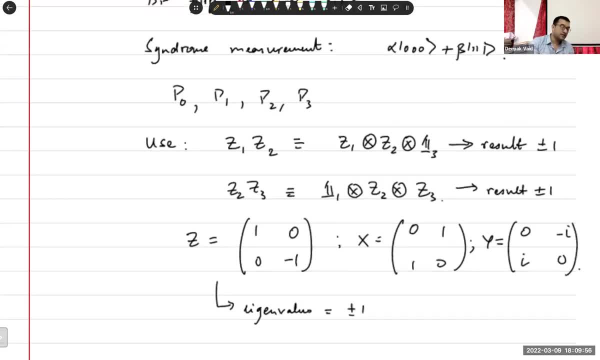 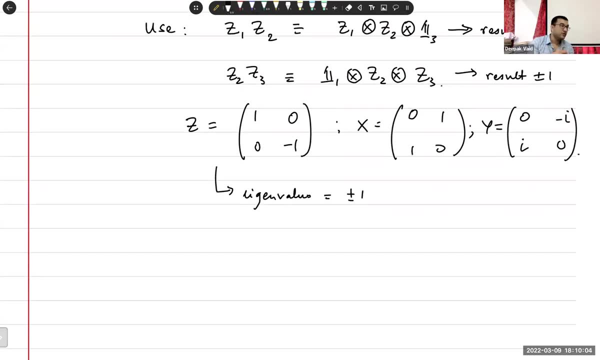 at this three qubit case and instead of looking at these projectors, I'm talking about doing measurements on a different set of operators And then in the nine qubit case, because this will lead to a simpler way of doing things. what you are saying is technically correct. 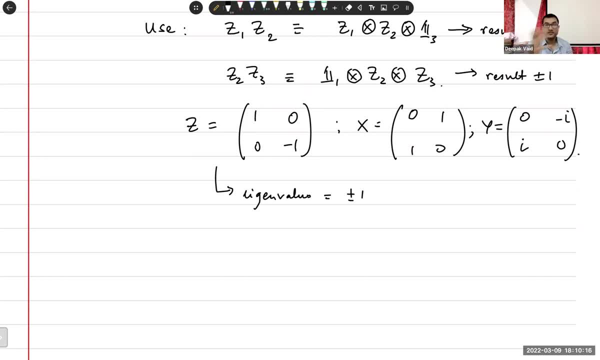 That in the nine qubit case you can construct a set of projectors, as he said, which goes as PI, tensor identity on three, tensor identity on three. But there is a simpler way of performing the measurements. So Okay, The reason for this would be: well, we'll see as we go, Okay, But yeah, technically, 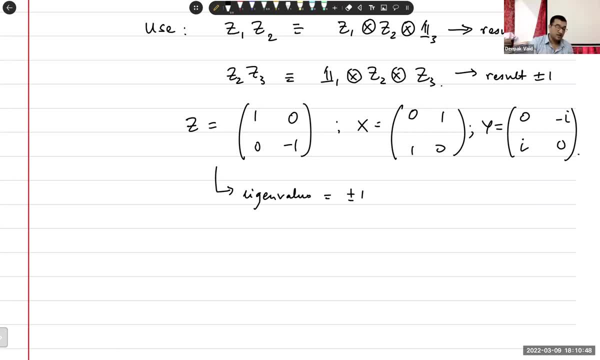 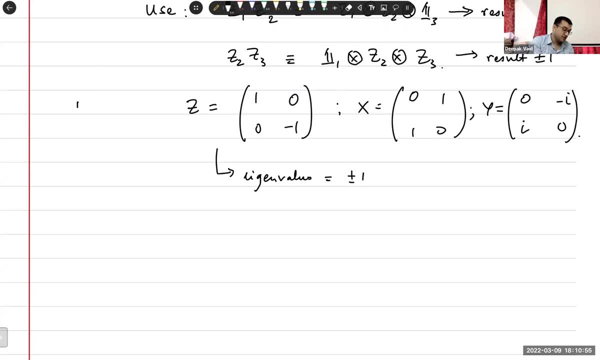 I mean, I suppose you are correct Now, and so these are called polys. by the way, These are known as these are all the poly gates, but when we talk about them- multiple strings of such operators- we call them polys. 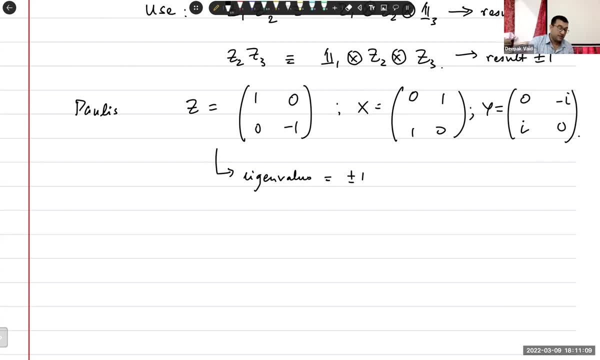 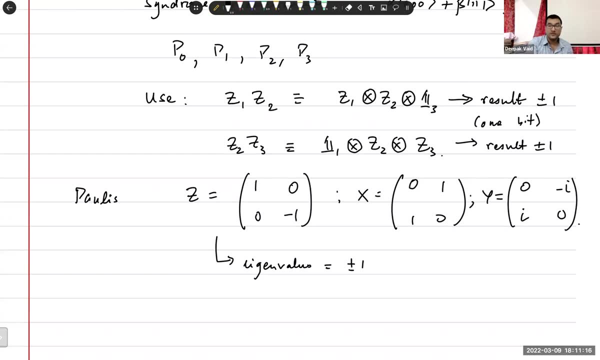 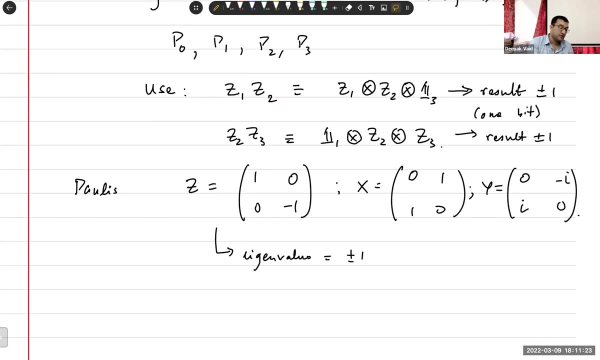 And each, each such poly is giving us one bit of information, right, Because it's plus or minus one. So that's one, one classical bit of information, right? So if you make a measurement of two such operators, what do we get? We get two bits of information. 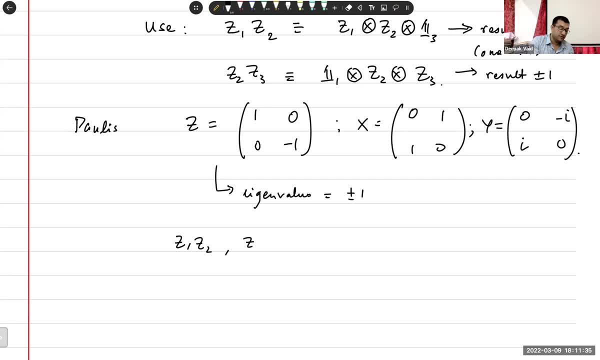 right. So Z1, Z2.. Z2, Z3 together gives me two classical bits of information about the state. right. That means I will get two classical bits, means I will get four possible outcomes right: 0, 1,, 2, 3.. 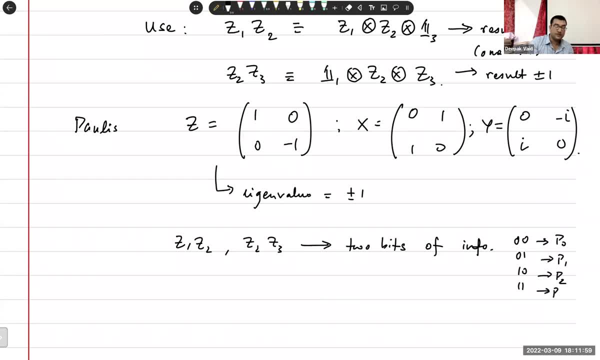 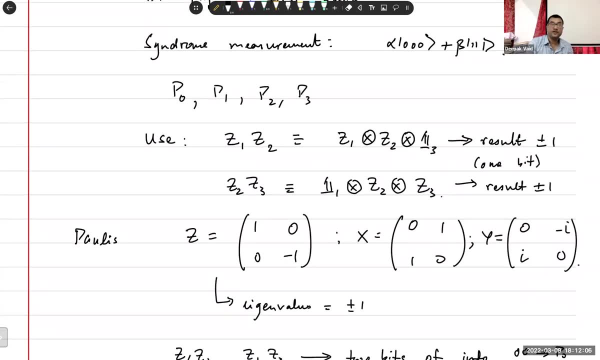 These can be put in correspondence with each of the syndrome measurements: P0,, P1,, P2, and P3,. right, Because P0,, P1, and P2, and P3, their measurement gives me either 0 or 1, right, And there are. 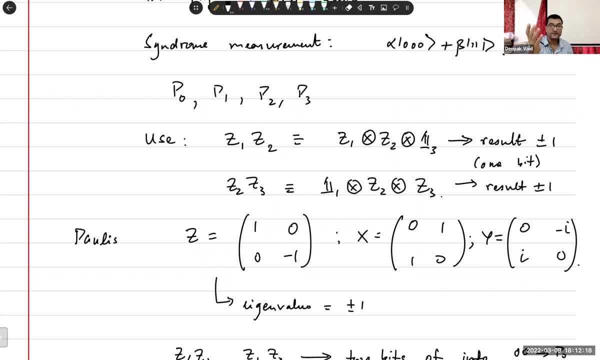 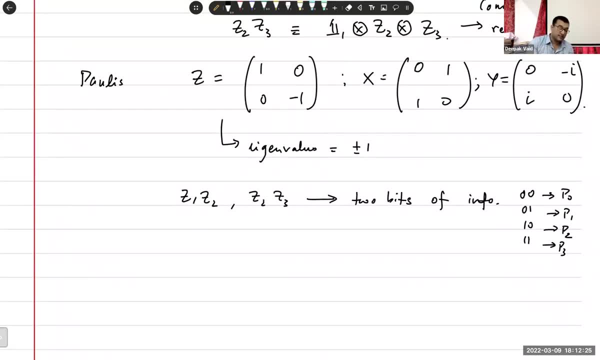 four such values Right Now. this, this first measurement: Z1 and Z2, what is it? Why is it called P0, P1, and P2?? Because P0 and P2 are the same values. right, Z1 and Z2 are the same values. 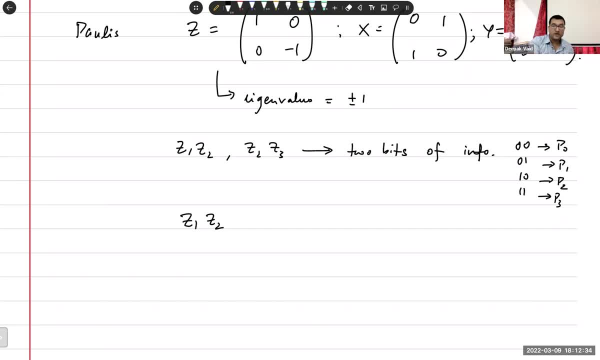 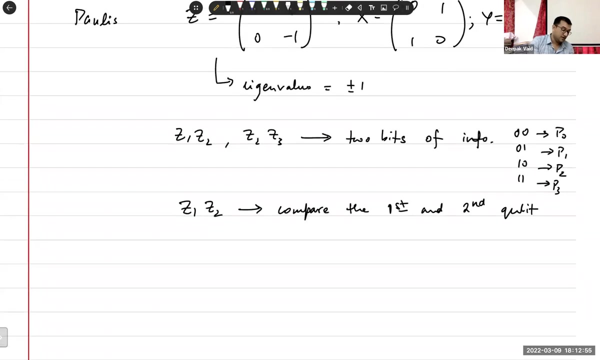 Right Now. why do we use them? Because they are the same values. Why do we use them? Why are we doing it? What does it tell us physically? It basically says that what we are doing is compare the first and second qubit to see if they are the same or not. 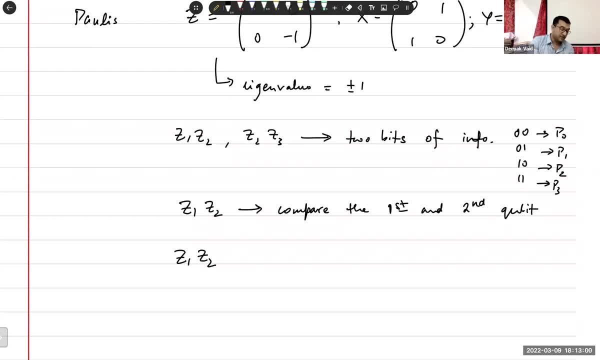 Why is that the case? Because let's take z1, z2 and act on this state or on the state. What will be the eigen value Plus 1? and if the first two qubits are different, then the eigen value will be 0.. So what's the eigen value If the first two qubits are different? 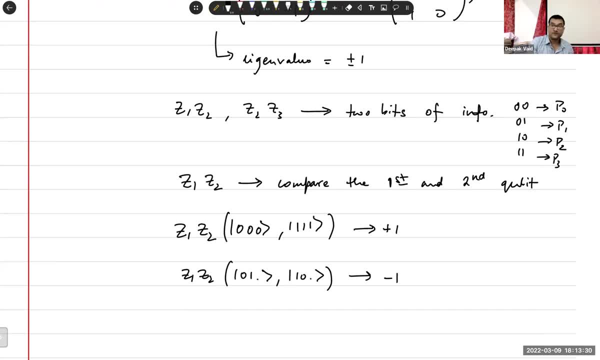 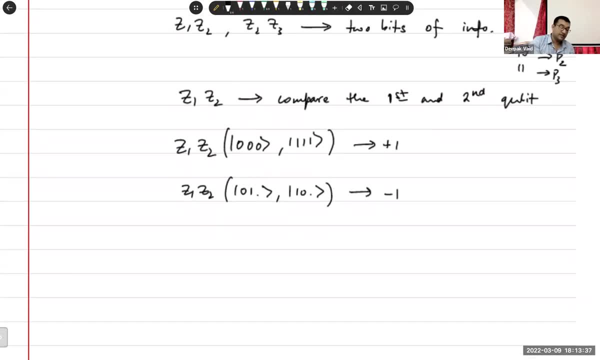 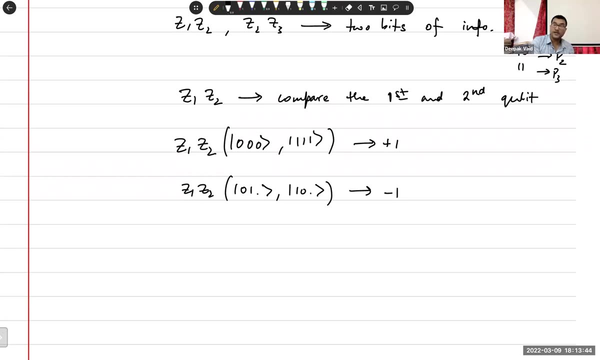 then the eigen value will be 0.. If the first two qubits are different, then the eigen value in value will be minus 1.. So the result of z1 and z2 gives us a comparison of the first and second. We can also rewrite: 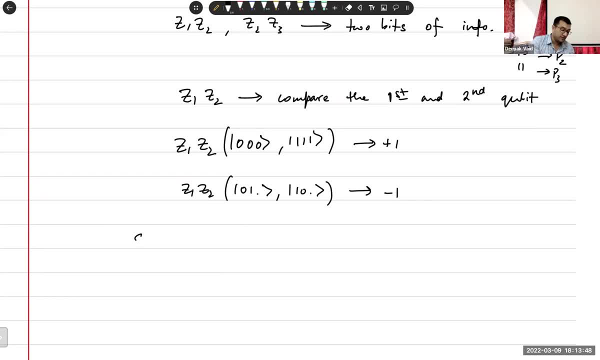 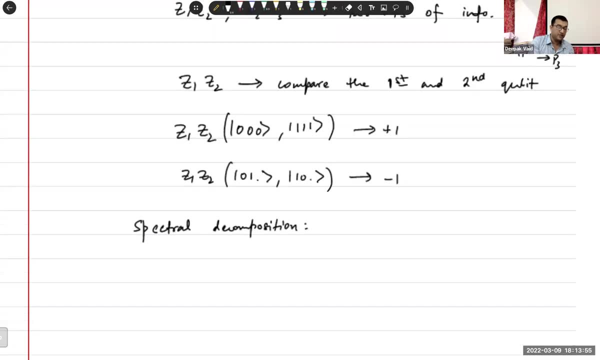 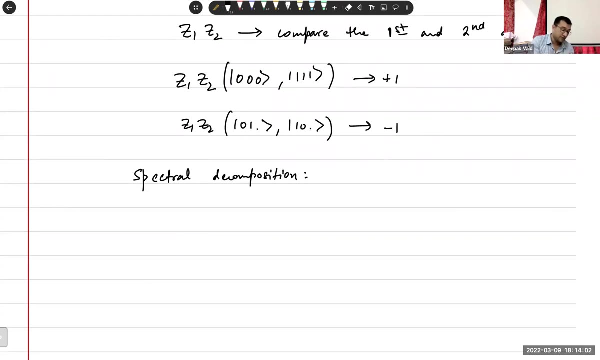 We can ask: what is this spectral decomposition of this operator, which will give us the same information, but in a slightly more mathematical expression. So, first of all, what is the z operator? The z operator can be written as follows, in terms of projection operators: 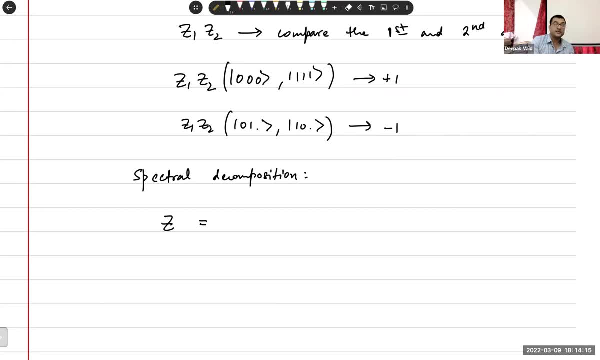 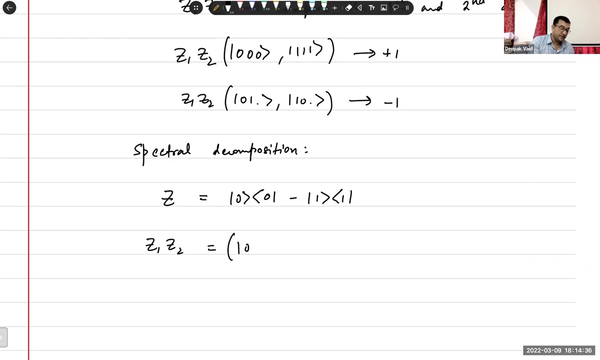 What is it? Does anybody remember? If I want to write z as a sum of projection operators, what will it be? 0, 0, then minus 1, 1.. So z1, z2,. I can write as this only. 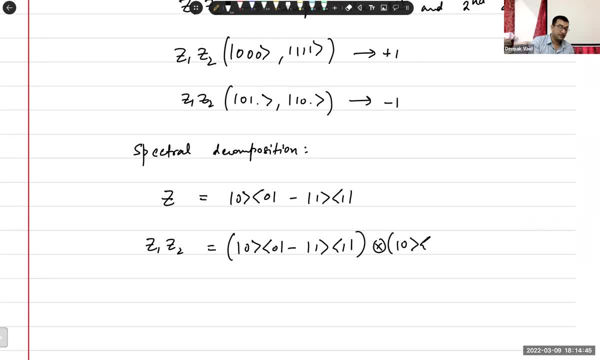 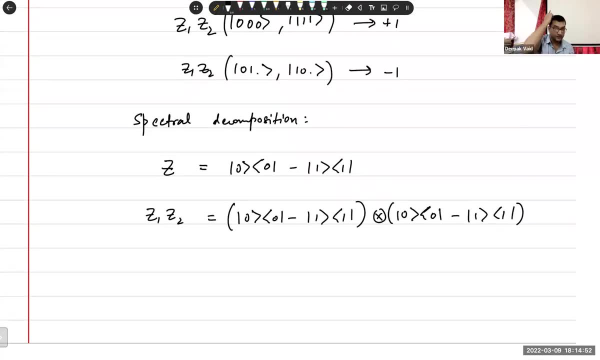 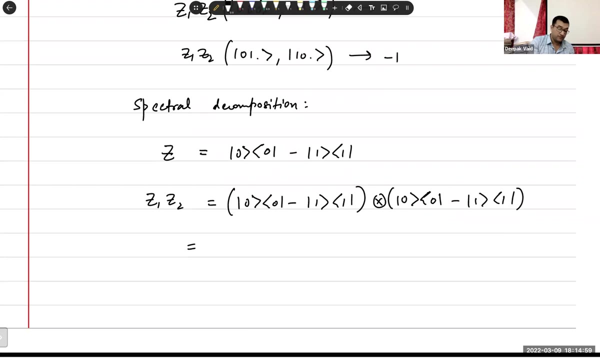 And then tensor with the same expression, but now acting on the second qubit, And I'm not putting those indices because that would take up too much space. So when you tensor all of this out, what will you get? You will get 0, 0, 0, 0. 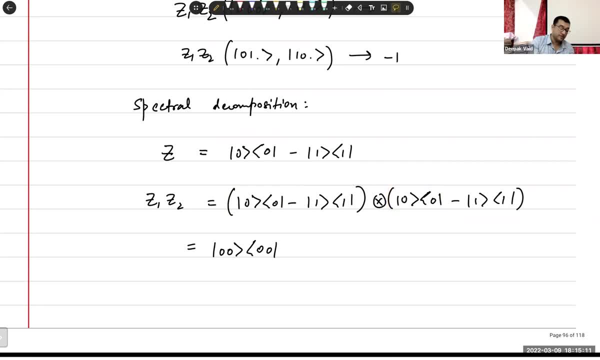 So if you look at the first two terms, for instance, that will give you this: 0, 0, 0, 0.. Then you look at the second terms: 1, 1, 1, 1.. 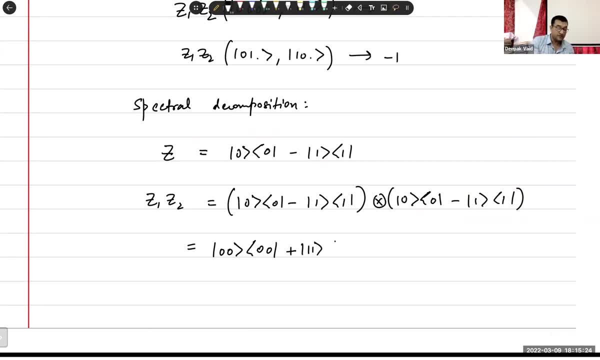 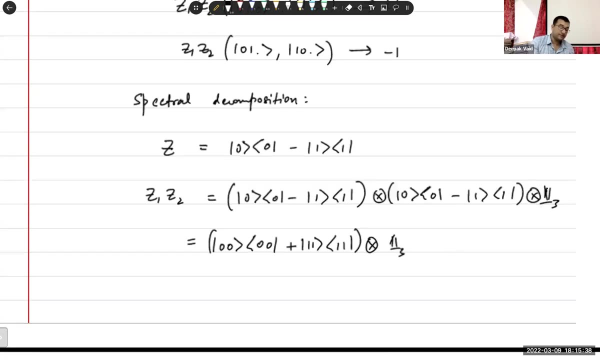 That will give you plus. Then we can write that as: and then all of this is tensor with the identity on the third qubit. So we'll put an identity here on the third qubit And then we'll get two other terms. 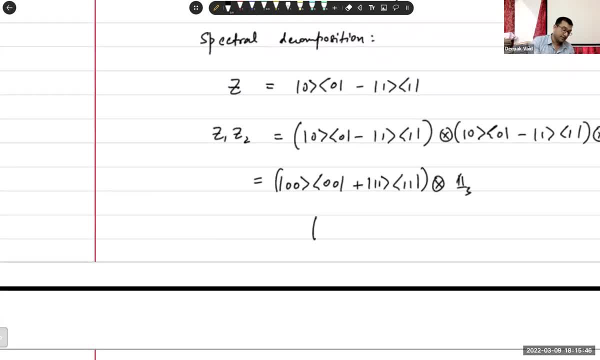 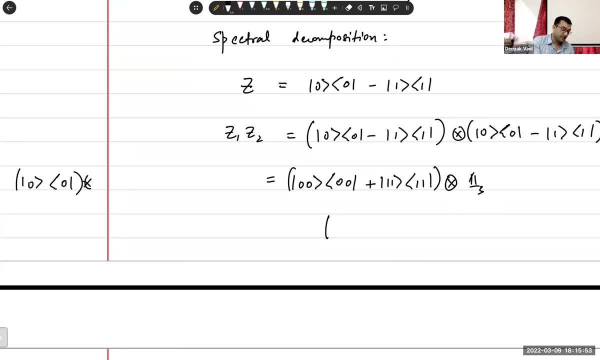 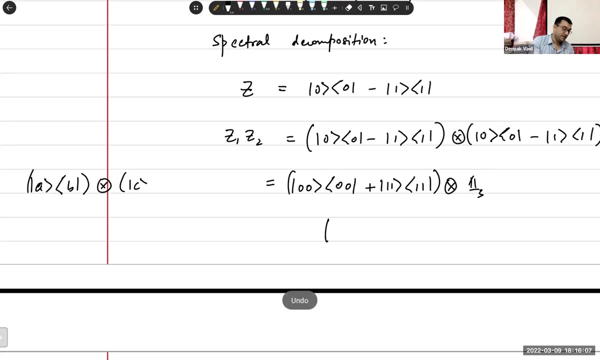 What are those two terms? So I hope that you can see, just to clarify that when I take this 0, 0. And when I tensor it, or to be a little bit more general, I guess, if I take a, b and I tensor it with c, d, what do I get? 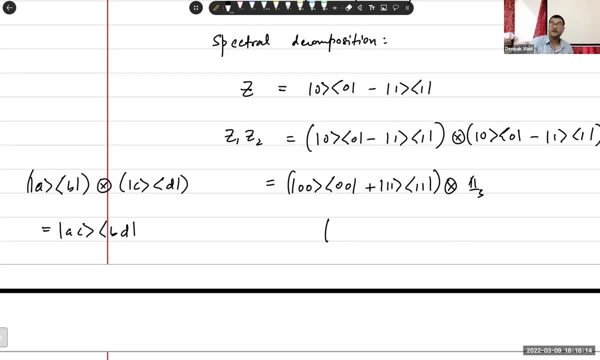 I get a, c, b, d, where a and c act on the first qubit. Sorry. a and b act on the first qubit, so they're in the first, And c and d act on the second qubit, so they're in the second slot. 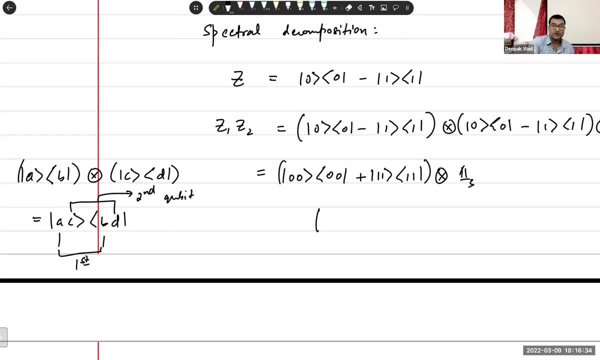 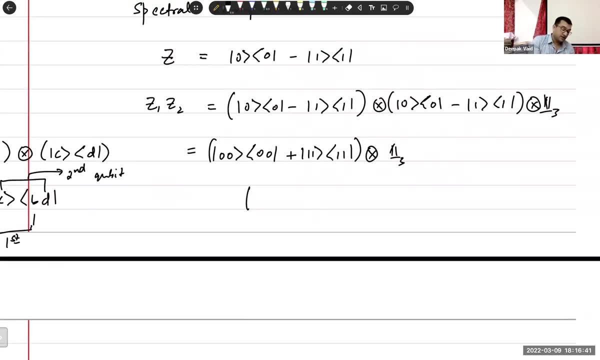 Please make sure that you get this notation. If you don't, you will face confusion later. So we get these two terms And then the cross terms will give us what. The cross terms will get: a minus sign. Then we'll get 0, 1.. 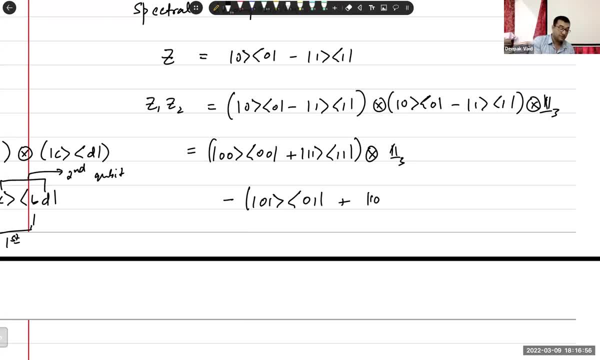 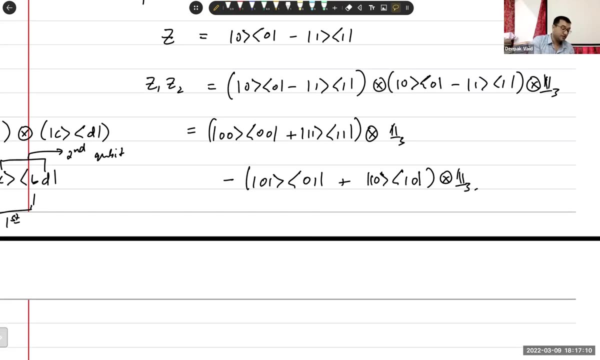 0, 1.. Then 1, 0.. 1, 0. Like this. So this is z1, z2.. OK, And we can see that it is a sum of. we can think so this is a projector. 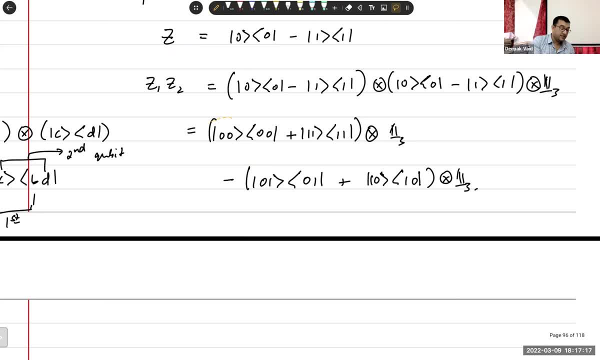 And this is also a projector. This is the first term is projecting onto the case. When the first term is projecting onto the case. When the first term is projecting onto the case. When the first two qubits are the same Right. 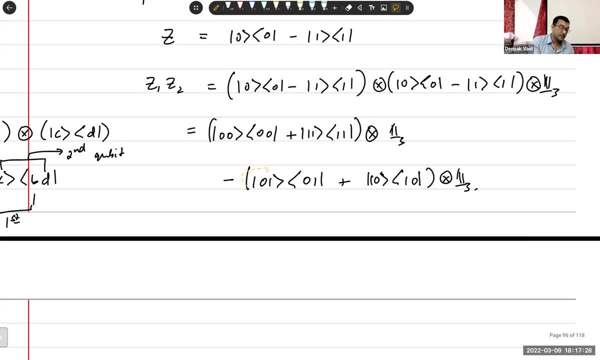 So if the first two qubits are the same, The action of this part of the operator on the state will be 0. And if the first two qubits are different, Right, So so these are. these are projectors. So in this sense, z1 and z2 gives us a measurement of whether they are the same or not. Same thing for z2,, z3,, z4,, z5,, z6,, z7,, z8,, z9,, z10,, z11,, z12,, z12,, z13,, z14,, z15,, z16,, z16,, z17,. 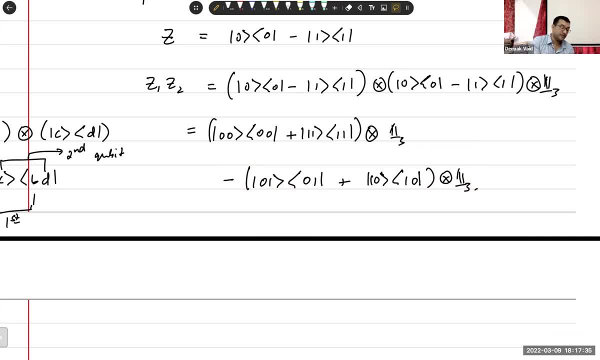 z20, z21, z22,, z23,, z24,, z25,, z26,, z27, z28, z29, z30,, z30, z31, z33, z34,, z35,, z36, z36,. 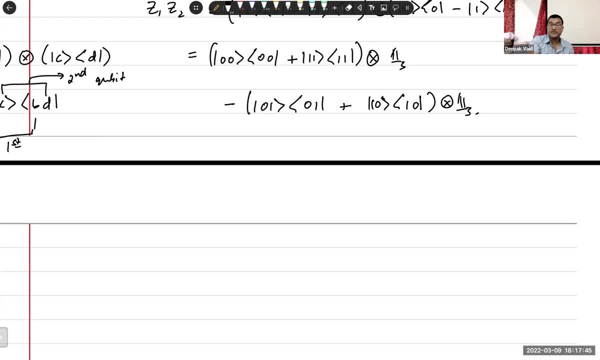 z37, z38, z48, z49, z49, z50.. So in this sense, z1 and z2 gives us a measurement of whether they are the same or not. Same thing for z2, z3, and z1, z2, and so on and so forth. 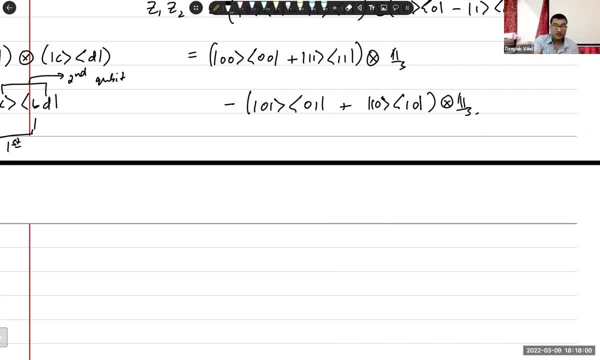 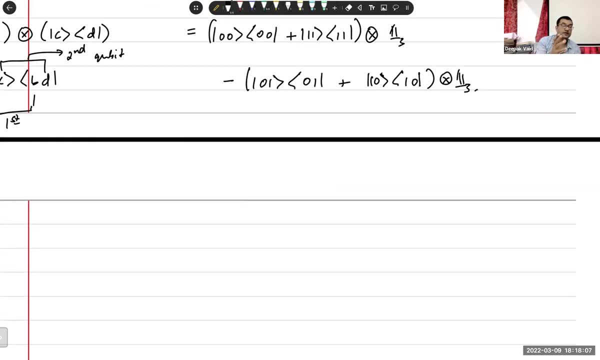 Okay, Now, Let's see, Let's see Now. so now what we can do is we can take these different sets and we can measure them in success. Okay, So let's combine one of these right. So let's say that we measure z1, z2 and this gives us plus one, okay, 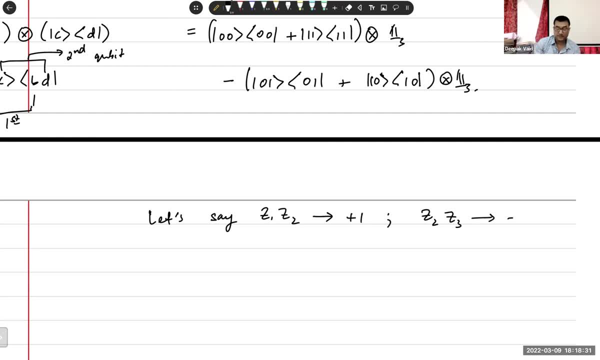 And then we measure z2, z3, this gives us minus one. What can we say about the state? What information does this tell us about the state? Third qubit right. So we can say with confidence that it is the third qubit which has flipped right. 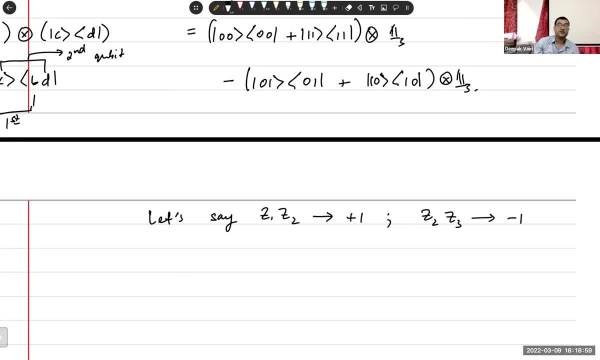 Assuming what One, One qubit error, Because if there is a two qubit error, then you can again get the. well, you would actually need a. yeah, you would need a two qubit error. So, assuming there are no two qubit errors, this tells you that the third qubit has flipped. 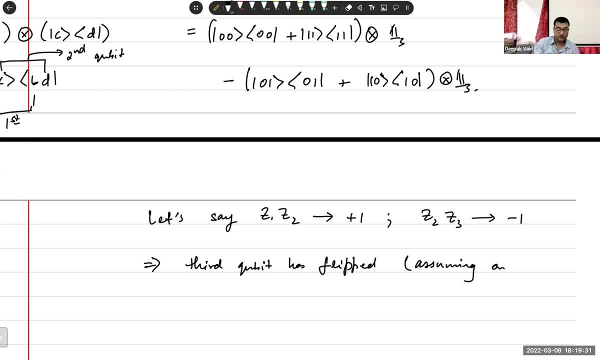 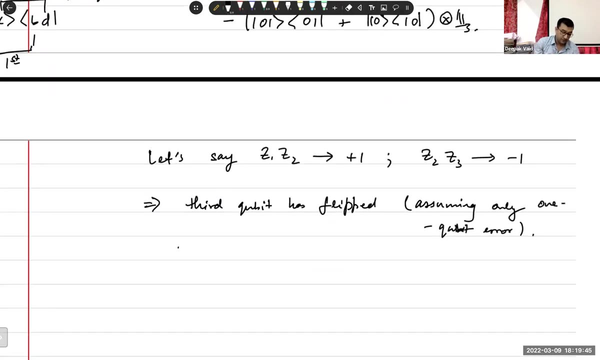 Assuming only one qubit error, okay. What if both of these give you minus one right? Then that tells you that it is z2, right. z2 has flipped Right. So qubit two has flipped. qubit two, q2, okay. 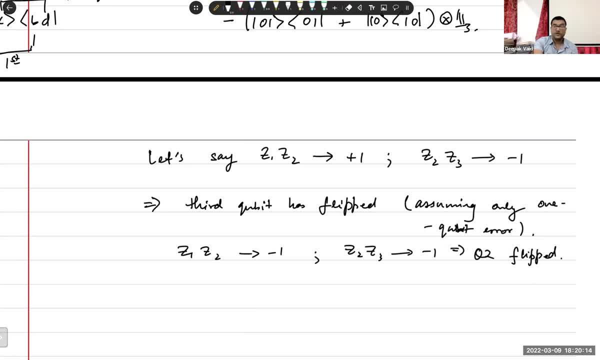 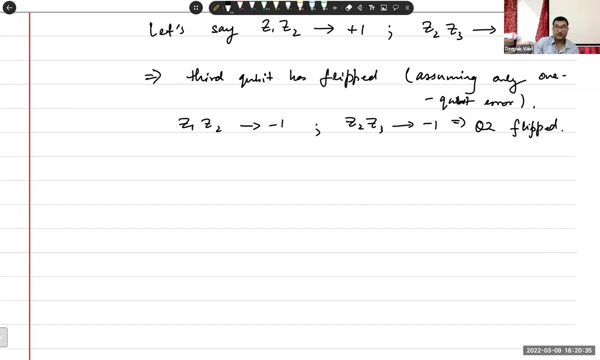 Now again, one might ask: in doing all these measurements, am I not destroying? destroying my state, okay, So? so let's, let's look at what happens when you take one of these measurements and act on the state, okay. 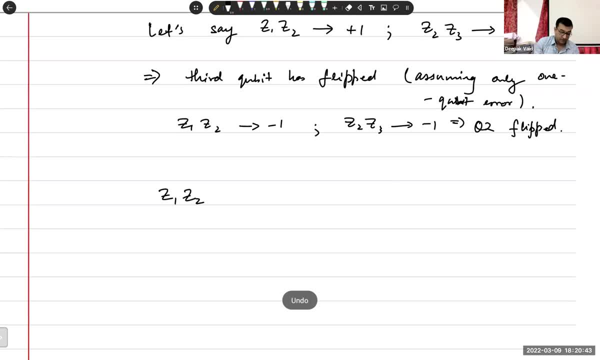 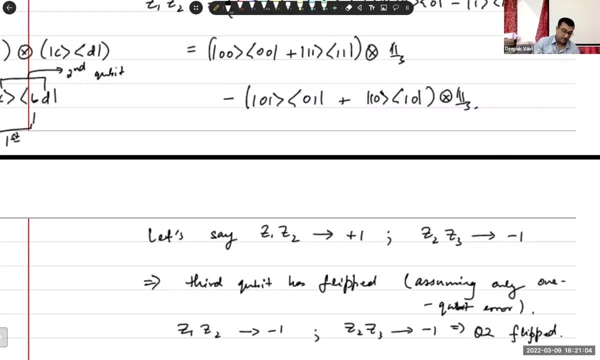 So if you take z1,, z2, right And you act on the state alpha, well, I'll write it like: how should I write it? Well, let me just say 0, 0, 0.. Let's beta: 1, 1,, 1, right. 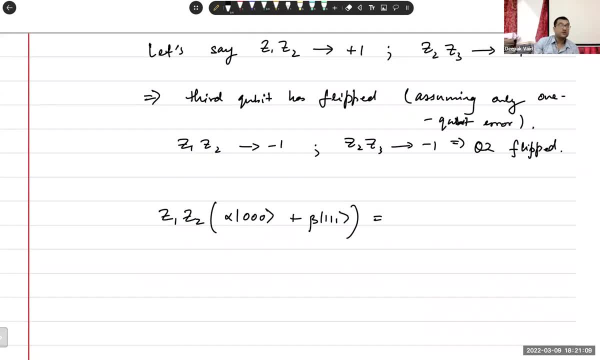 And what is the answer? This is: this is an eigenstate of z1 and z2, right? So if I act on this with z1 and z2, will the state collapse into something else? No, Why, Because it's already in an eigenstate. 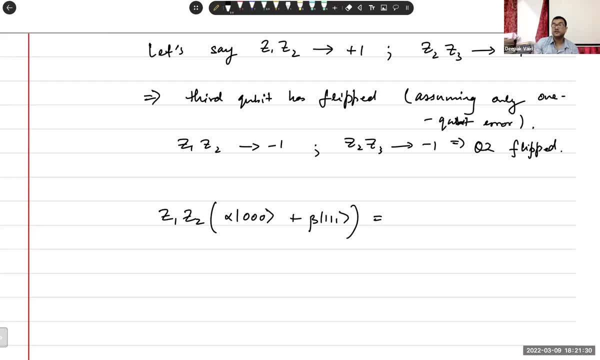 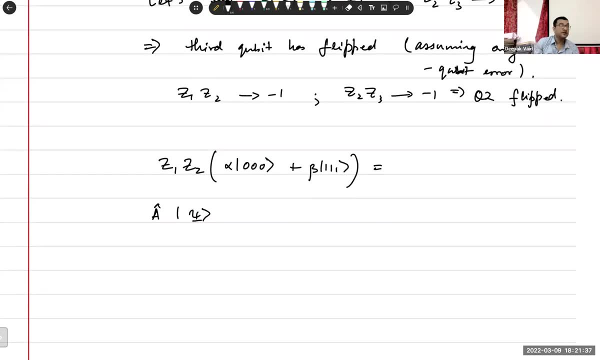 Right, It's already in an eigenstate of the operator that is being measured. So if you measure an operator A on some state, psi right- What does the measurement postulate tell you? Measurement postulate tells you that the state collapses into an eigenstate of A right. 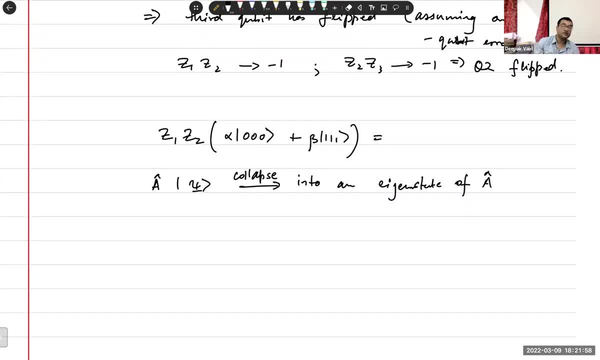 But if you are already in an eigenstate of A, then it collapses Right, Your state will not be changed. So this is the sense in which these measurements are not changing our state. Is this, Aditya? is this, is this making sense? 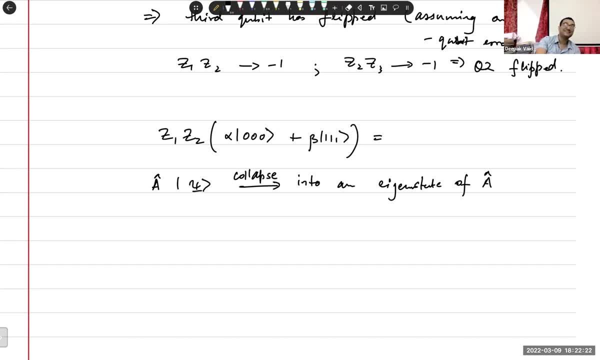 Little bit, Huh, Little bit, Little bit. no, That's why I could, I could feel that there was a disturbance in the force, Right, Yes, Disturbance in the force. At this stage, Star Wars is also so old that none of you get these, get these references. 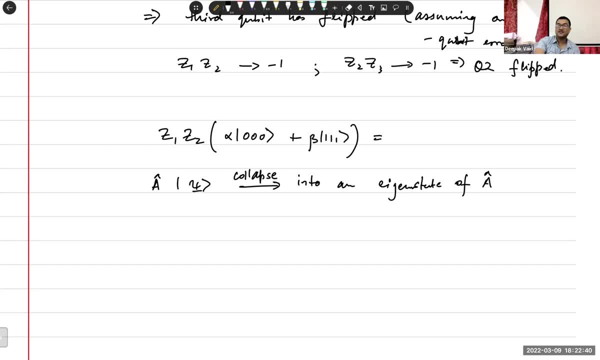 right, Right These days. I mean the Fast and Furious references. you might have understood them, or that too has become a classic. Hmm, That too has become like Ramayana right, Something like that. Yes, Yes. 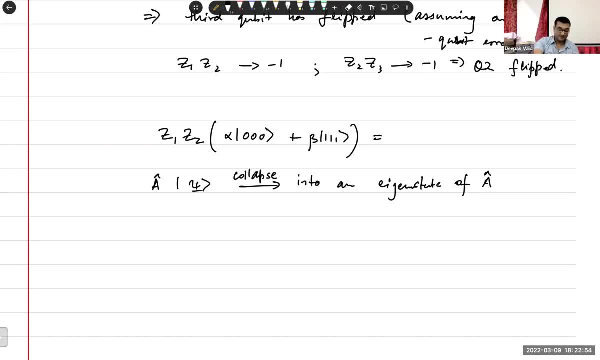 Yes, Yes, Yes, Yes. In maybe like the 20th version episode of Fast and Furious, you'll see like Vin Diesel lying on a bed of arrows or something like that and somebody like sitting at his feet saying Pitama giyandijiye ki gadi kaise chalao theiss face. 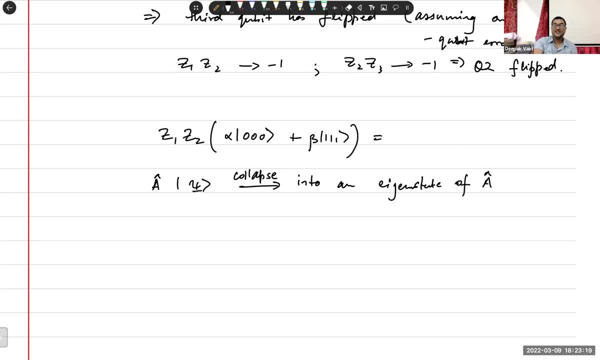 Anyways, Aditya, Can you give me some more time, Aditya, Yes, what is the measurement? just state it for me. what happens when you measure an operator A on some state, sign eigenvector of that state A of that operator A. 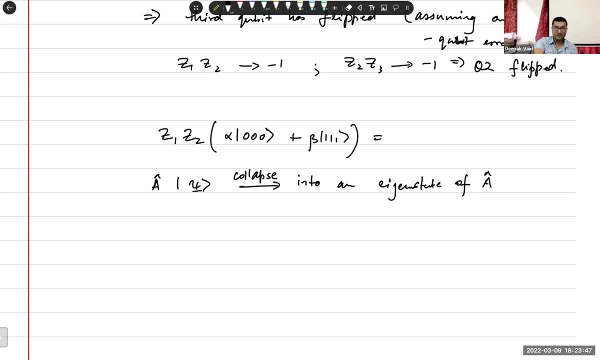 now if the operator A is Hermitian, what can you say about the eigenstates of that operator? right, but what about the eigenstates? they are orthogonal. what else? so? no, that's, you can normalize any state, all of the eigenstates of an Hermitian operator. 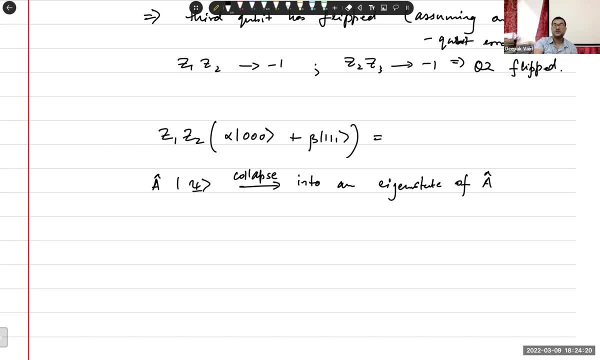 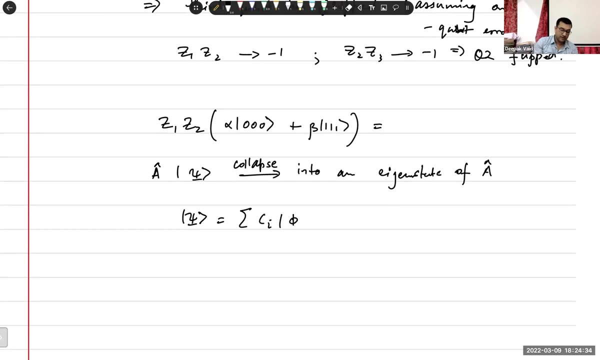 span the entire Hilbert space. they, so they give you a basis for your Hilbert space. this is the important part. so you can take any state psi and write it as a superposition of eigenstates of this operator A, if A is Hermitian right. 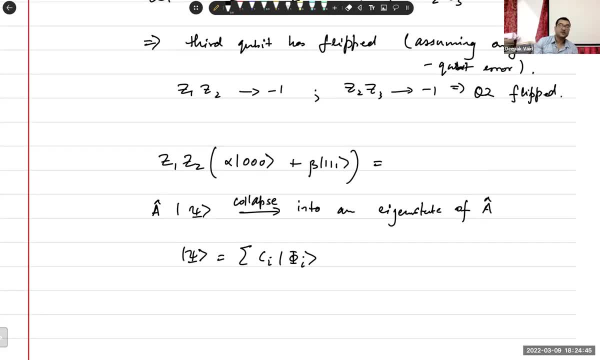 and all of these operators are Hermitian: Z1, Z2, Z1, Z2- all of these operators are Hermitian. so this properties are nothing but Hermitian and, moreover, the states that we are measuring are eigenstates, so there is no collapse. so you understand that if you measure, 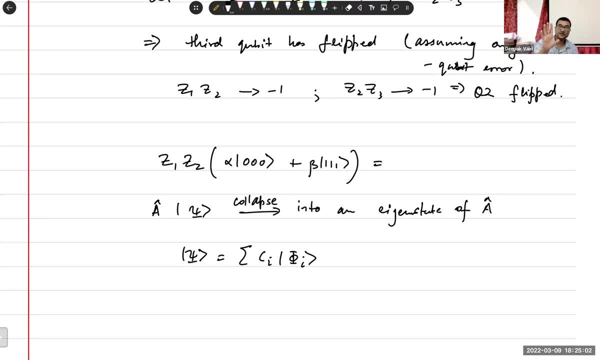 if you have a qubit which is in the spin up state, fine, I measure the poly Z on that qubit. what will be the state of that qubit after measuring? so after measuring, is it plus minus 1 or minus 0? No, If it's in the zero state up state, that is already an eigenstate of the z operator. 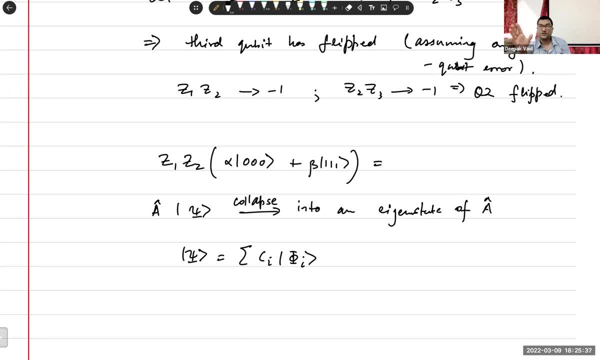 It's an eigenstate of z with eigenvalue plus one, So there is no reason for it to collapse into anything else. There are two eigenstates of z: zero and one. If I start with zero, I'll stay in zero. Make sense or not? Think of it like this that you have a Bloch sphere. 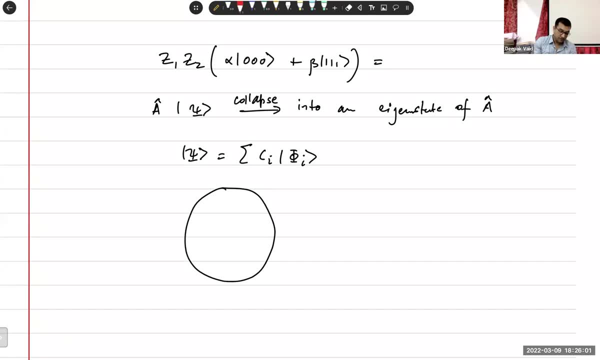 You think of this Bloch sphere picture. Your state is a dot on this Bloch sphere And there are two eigenstates And you're talking about measuring zero and one. Now, I know many of you get this, but I'm just emphasizing this. 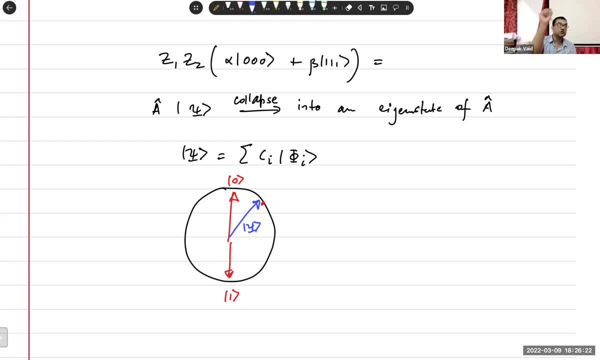 And so your state, psi, let's say your dot, is closer to the North Pole than it is to the South Pole. Now, when you make a measurement of z, is your state going to be more likely to collapse into the North Pole, which is zero, or the South Pole, which is one North Pole? 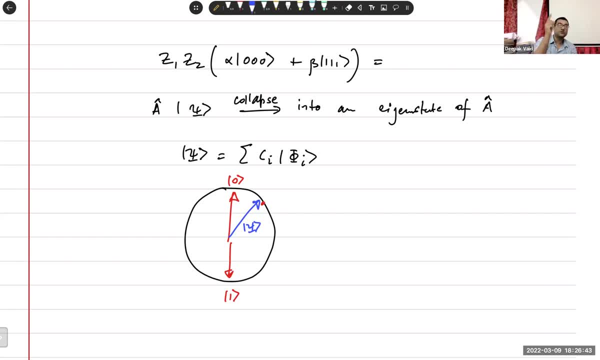 And if your state so, as you go closer and closer to the North Pole, the probability of collapse will become equal to one. You can think of it that way if you want. When you're talking about plus and minus states, plus and minus are eigenstates of which operator. 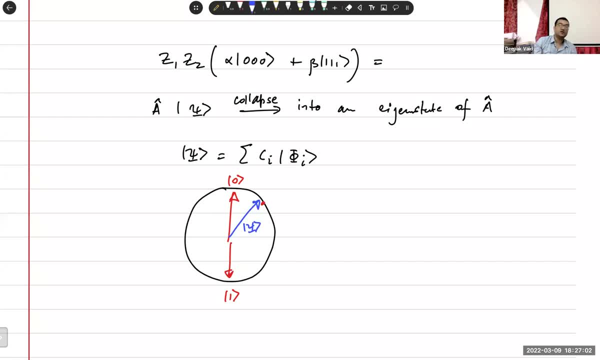 X, X Plus and minus are eigenstates of X and Iy, Iy. Okay, So if you are measuring, if you are measuring the X or the Iy state or Iy operator and your initial state is zero or one, then it. 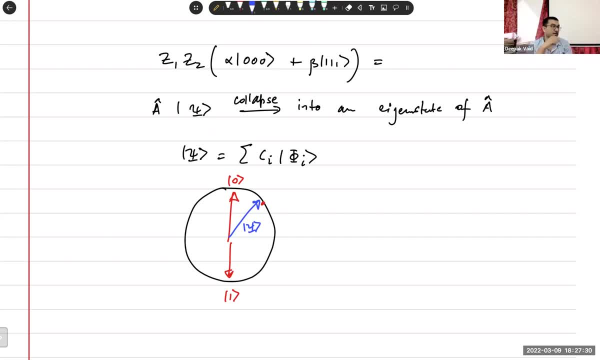 will collapse into which state? If your state is initially to begin with zero or one, and you measure the X operator, what will be the outcomes? One, What are the eigenstates of the X operator? Plus and minus, Plus and minus. So what will be the outcomes? 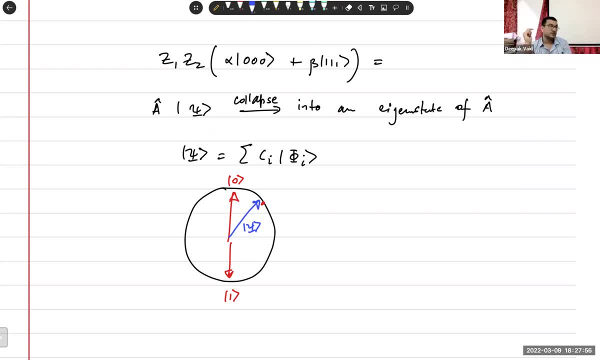 One and plus, Either the plus state or the minus state And, with probability, Half each. Okay, If you don't understand this, Zoom people and people here. please just think about this. This is a seemingly very minor point, But it lies at the base of everything that is going on: The fact that you can perform. 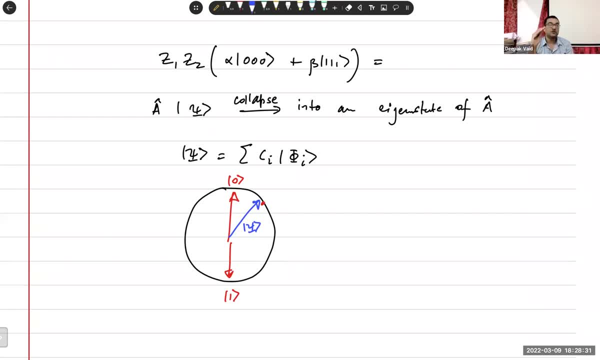 a measurement of these operators without destroying the state, Because if you cannot do that, then nothing that you want to do as far as correcting your errors without changing the state, without destroying the quantum correlations, is possible. Okay, So I have a question. 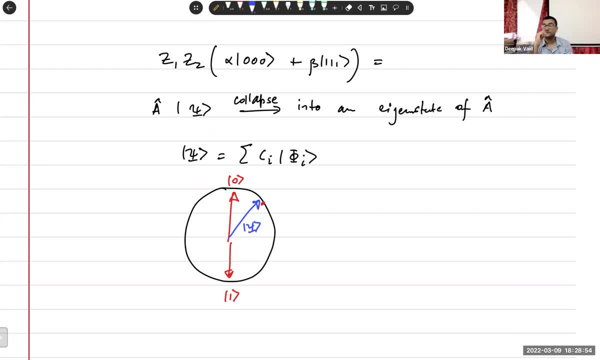 Yeah, So this is fine, but are we able to measure that measure of systems in plus or minus? If you are doing X or on or minus one state, are we able to measure that without arming that state? No, no, So that depends on what your state is. This is the whole point That see in. 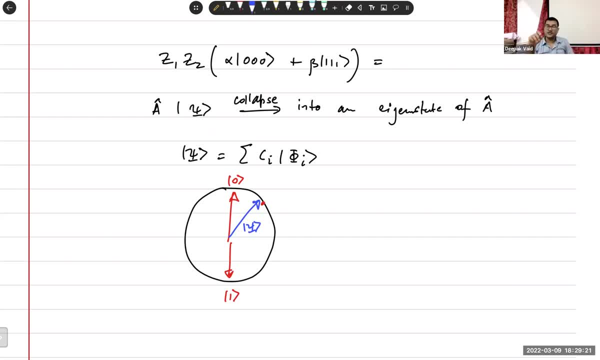 this setup. all our states are superpositions of 0 and 1.. So if I measure any of the Z operators right, I'm always in some eigenstate of those operators. So my state will not collapse. So it won't collapse. 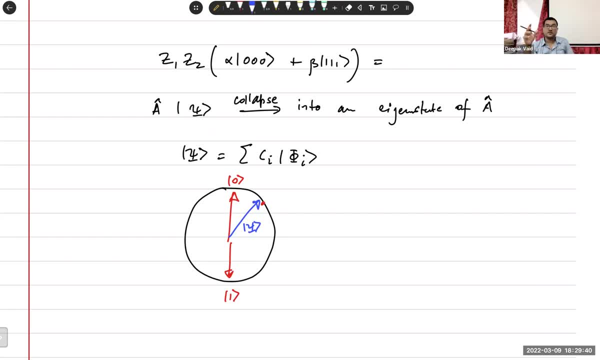 Right? Are we able to make out that it is in the plus state? Or the issue is, if it is in one state, will it collapse? No, No, No. So if it is in one state, we can say that there are no. the bits are the same. 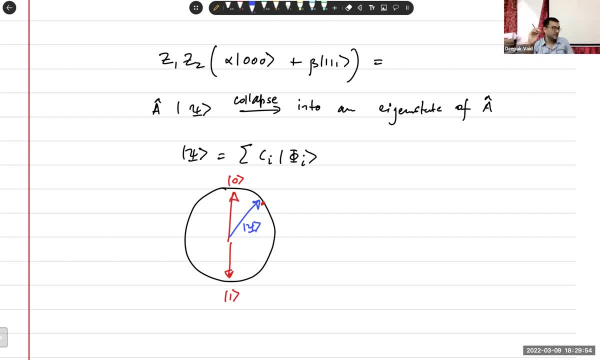 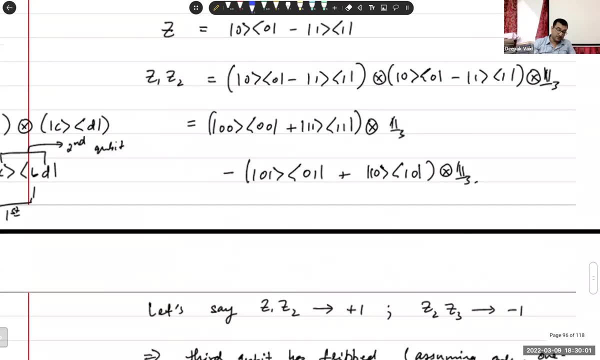 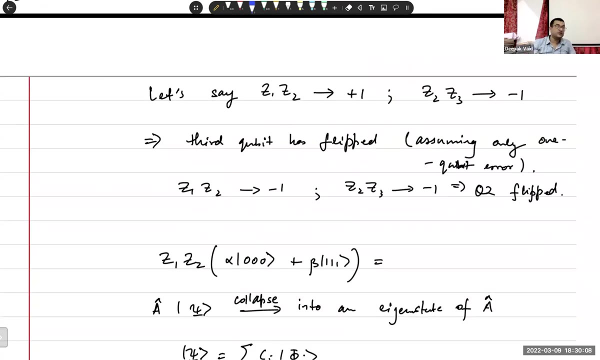 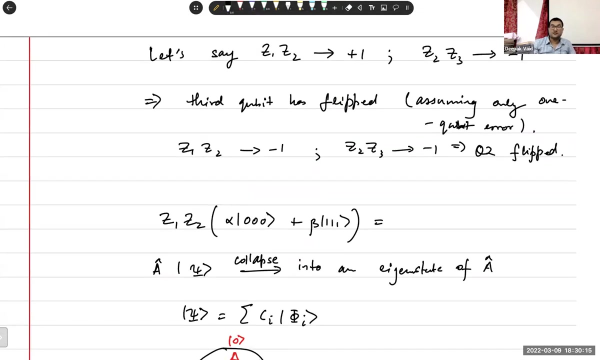 But the thing is so. the thing is so. here's the thing. That. okay. So let me show you again: If you take Z1 and Z2 and you act on alpha 0, 0, 0 plus beta 1, 1, 1, what is the result? It's equal to alpha 0, 0, 0 plus beta 1, 1, 1,. right: Is the state changed? It didn't change, But do we know that it changed? Like if we know that the state didn't change. 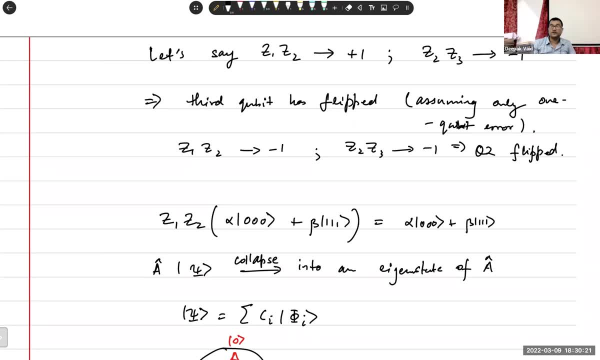 then we can say: the bits are the same, But we do not know that right. No, no. But as far as the mathematical theory is concerned, these two operators will not cause the state to change. no, Practically, No, no, So practically. there might be some errors in the measurement, in the way. 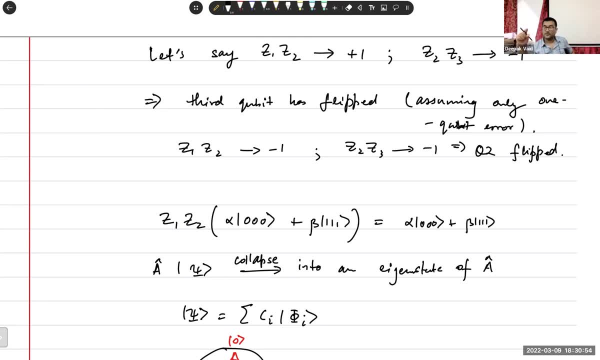 you implement this measurement, which might constitute a separate source of errors. right, So there might be an error in the syndrome measurement itself, But assuming that the syndrome measurement can be performed without making an error right Now, your question actually has a very nice answer. I just didn't go into it because it 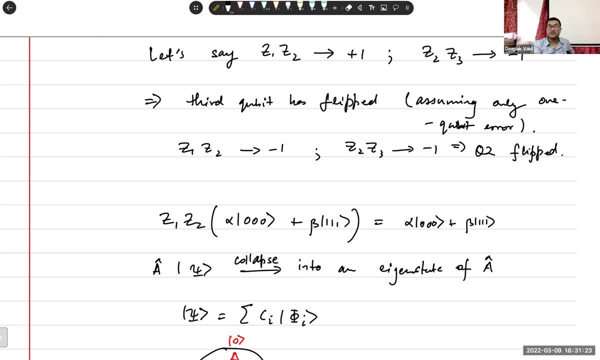 requires a little bit of math, which is? it involves something called the notion of fidelity and mixed states, right? So exactly what you're asking is that how can you tell whether there is an error, which is big or which is small? Okay, Why? Because these quantum states live in this continuous space, right? So let's? 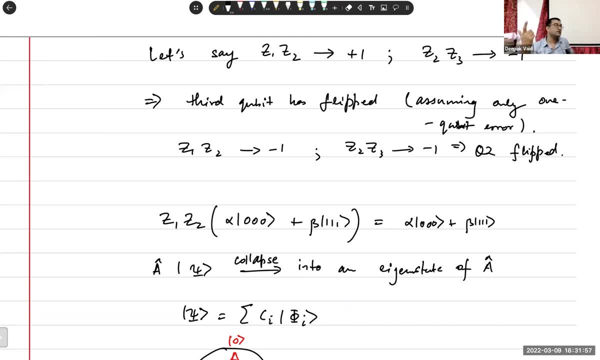 say that you have a bit flip error which is generated by which poly Aditya bit flip is caused by which poly X, X, excellent. Now if I start with the state plus and I act on it with X, what happens? 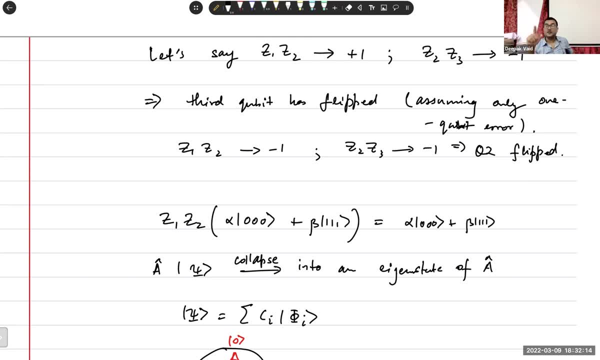 to that state: Zero, Zero, But is the qubit flipped? The qubit is flipped. no, Zero goes to one and one goes to zero, But nothing happens to that state. On the other hand, if I start with the zero state, 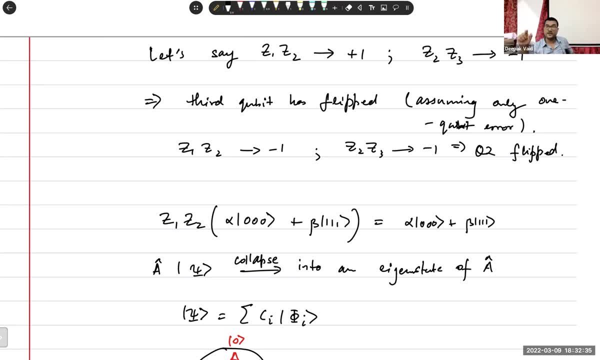 and there is a single qubit error generated by X. what happens? It goes to one If I, if the error no, no, X acting on zero will give me one. So my point is that, how do I quantify? So in one case, in both cases, an error is taking place which is a bit flip, is happening. 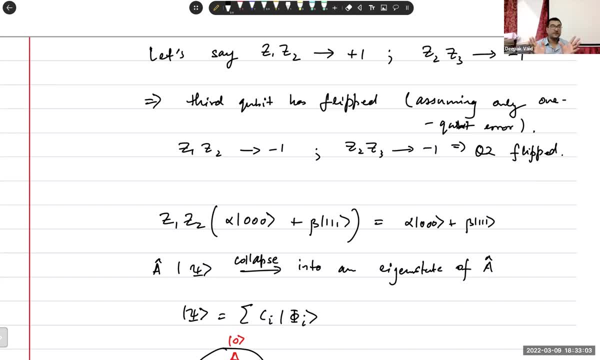 I know that for sure. right, But in one case the bit flip leaves the state invariant. In the second case, the state becomes orthogonal to itself, Right? So in the first case I should not worry about that error. I don't care, because I only care. 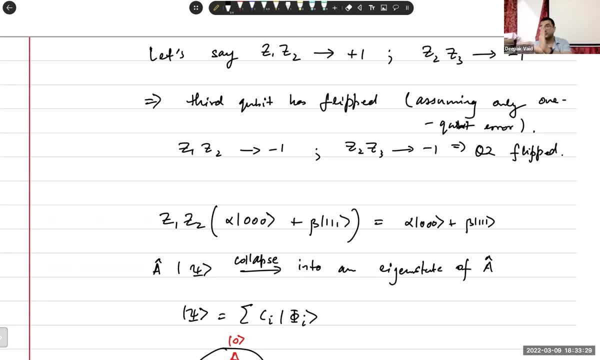 about those errors which cause my state to change into something that is orthogonal to itself. So this question is answered. this is answered by the notion of fidelity. Right Fidelity is the term that one uses: Right, One uses to describe the quality of sound, right normally, or a signal fidelity. How? 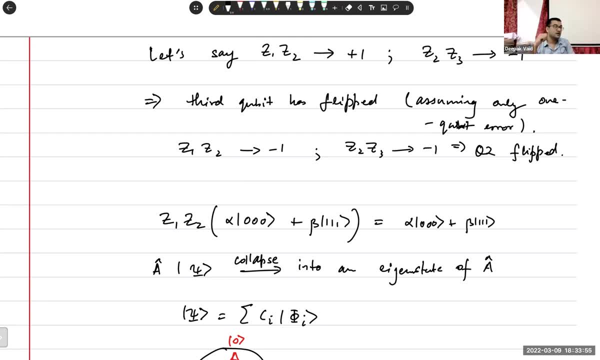 true, is it to the original. So so for this, fidelity is basically the overlap of two states. Okay, So if you take two states, psi and phi, and you overlap, you take the inner product. If those two states are the same, you get one, otherwise you get zero Right. So the fidelity is essentially 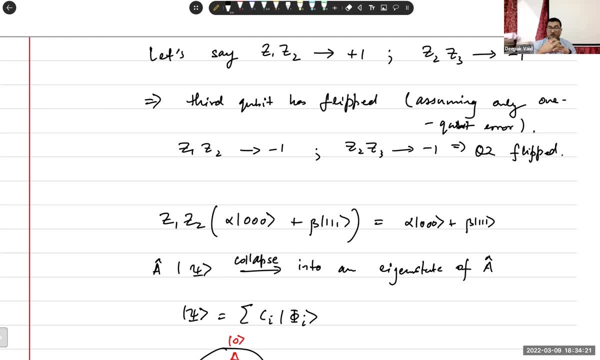 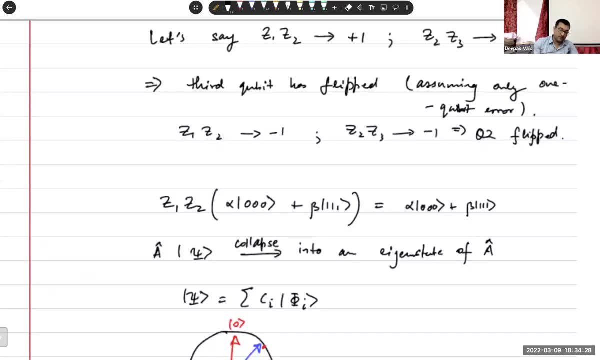 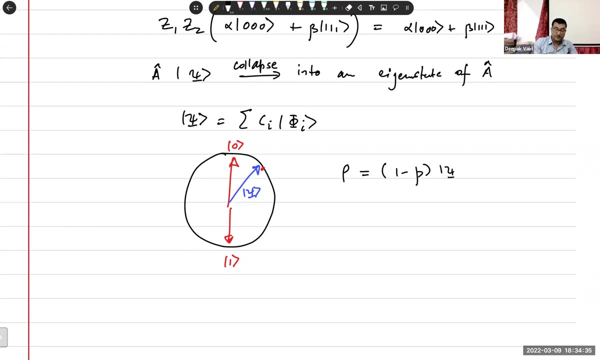 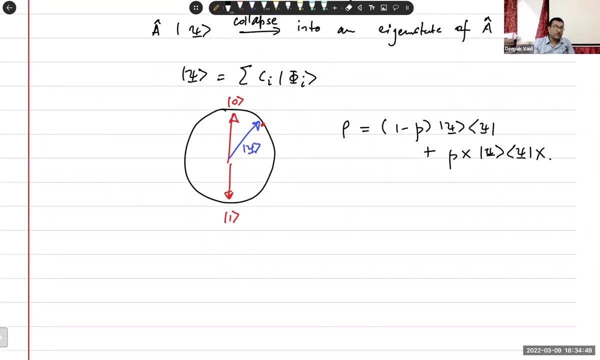 given by, by this quantity. So now, what one does is the following: You write down an operator which looks like this. I'm assuming that all of you can see what I'm writing. Okay, What is this operator doing? Our state phi or state psi is the state of interest. Okay, this is the one that we care. 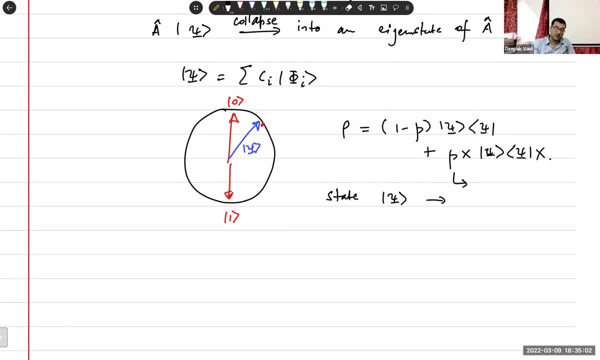 about The number p is what Number p is the probability? What is it the probability of Of bit flip, Right, What does the first term tell you? The first term tells you that no bit flip is happening. If there is no bit flip, then the first term tells you that your state doesn't change. 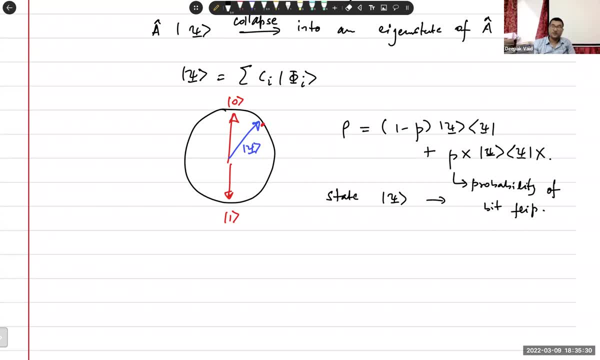 What about the second term? The second term tells you that there is a bit flip that is expressed by the presence of the x operator. But note the way in which this projector is constructed. We take our state psi and we flip the bit so we get x psi. This is the state with the 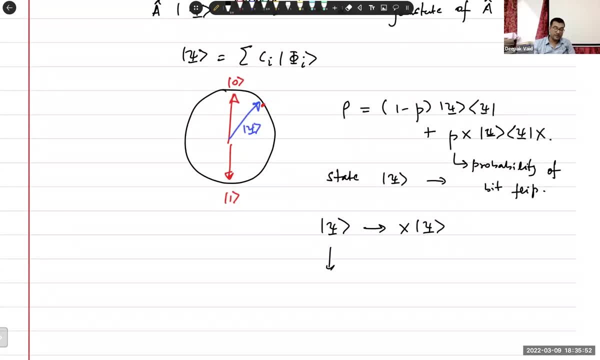 flip bit Right. So if you want the projector for the state psi, you get, you take bra psi. so you take ket psi and then adjoint ket psi. If you want to construct the projector for the flipped state, what do you take? You take. 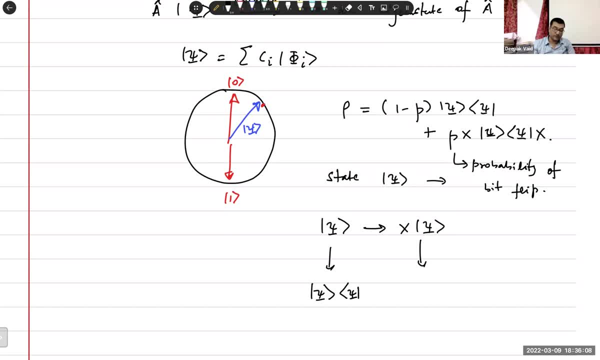 the adjoint of the x psi. So you will get what You will get: x, ket psi, adjoint psi and then again adjoint x. What is adjoint x? It's x only. So this row that you have here. 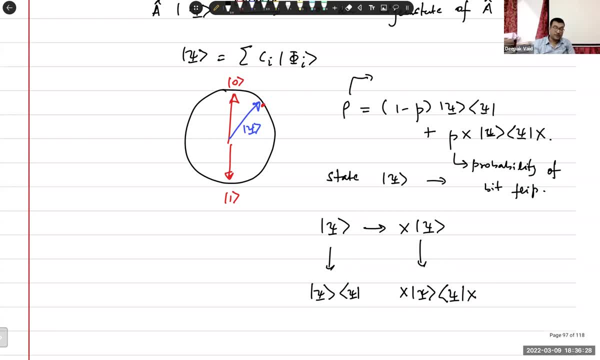 Right, This row is what we refer to as a channel, Okay, It represents. So something is happening. You are sending your state from point A to point B, Right? And presumably it comes out on the other end. Something happens to it. 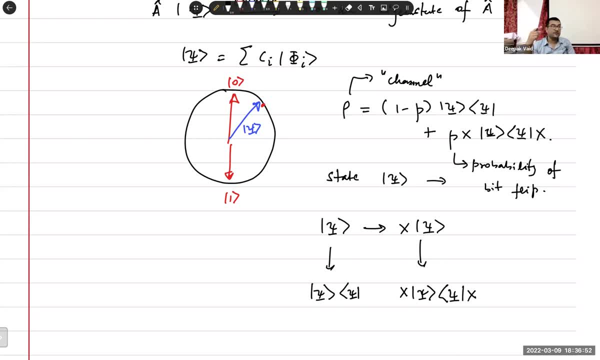 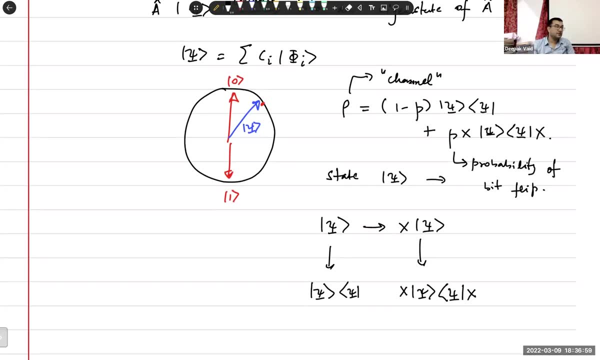 Right. Either there is a bit flip or there is no bit flip. If there is a bit flip, that is represented by the second term. otherwise it's represented by the first term, And so this row is an operator Right And it's called a. I mean, that's how you represent channels in quantum information. 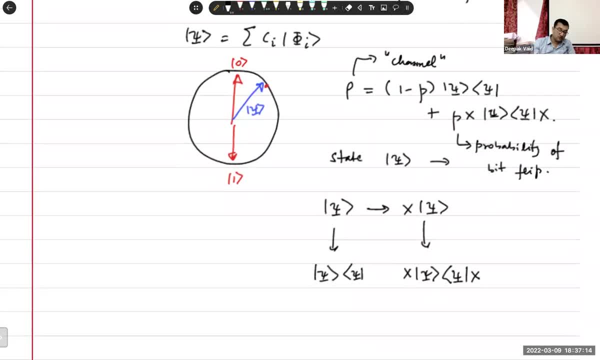 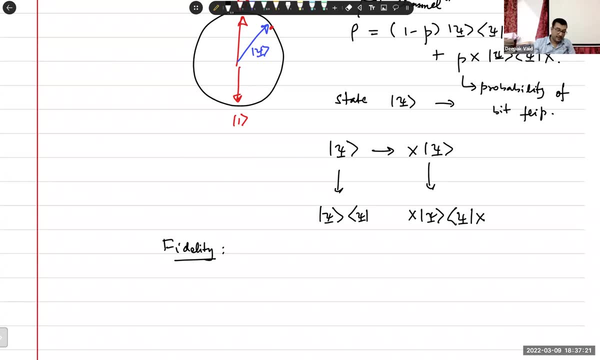 Okay, Now how do I define the fidelity? Okay, So the fidelity is written defined as follows: And technically, what rho is? rho is what is called a mixed state, And this is the Greek letter, rho, by the way, not p. 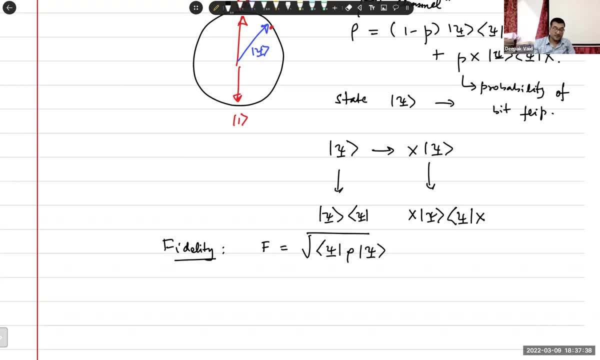 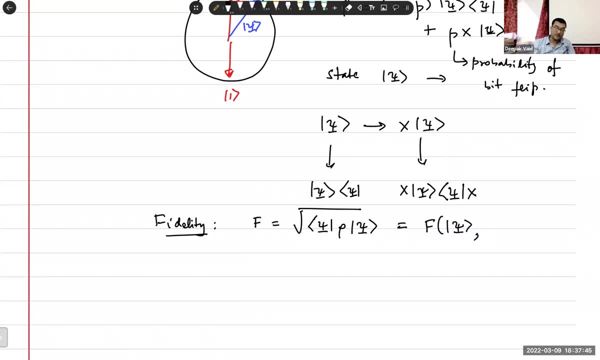 Okay, So the fidelity is defined as this expression. So the fidelity is a function of two things, two inputs. It takes in a pure state, psi, and it takes in a mixed state, rho. Okay, And that's what this rho is. This is a mixed state. 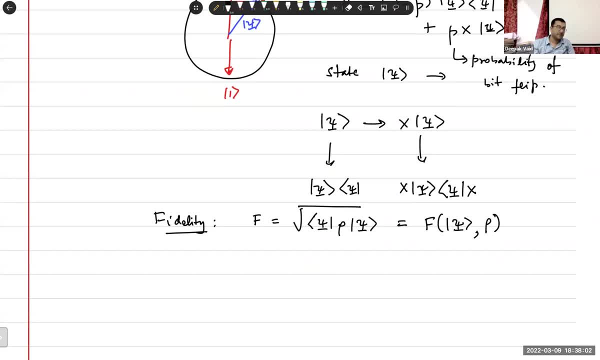 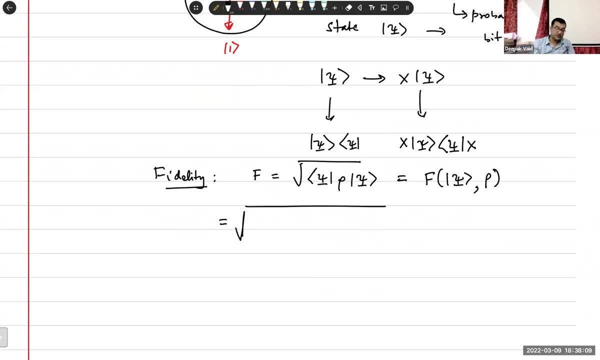 Okay, And don't worry about what mixed states are for the time being. Now we can do this calculation by putting the expression for rho in a product Right, So we get psi, And then we put one minus p Right, Plus x p times x psi. 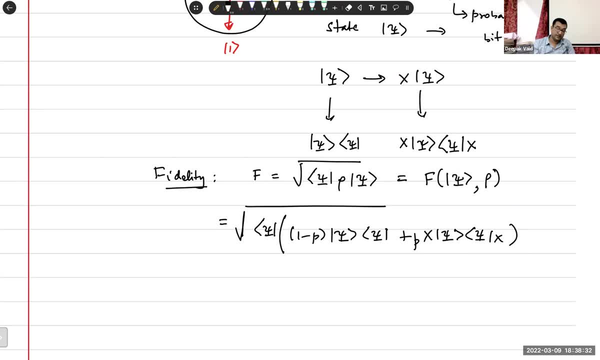 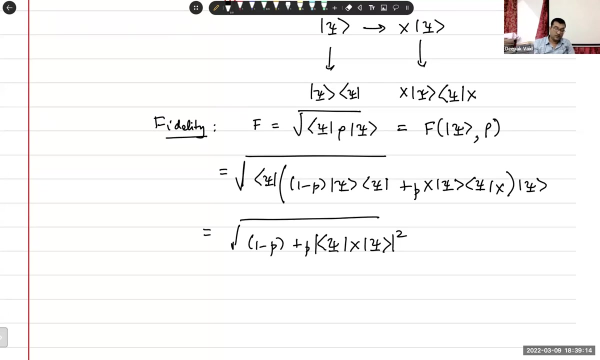 P times x, psi, P times x, psi, x Right. Okay, So this is our fidelity. Now what will happen? The first term will just give us one minus p, Right, And the second term will give us the following: expectation value of p times the expectation value of x acting on Psi: whole squared, okay. 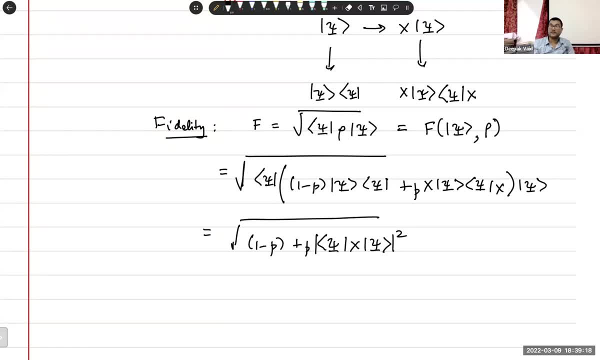 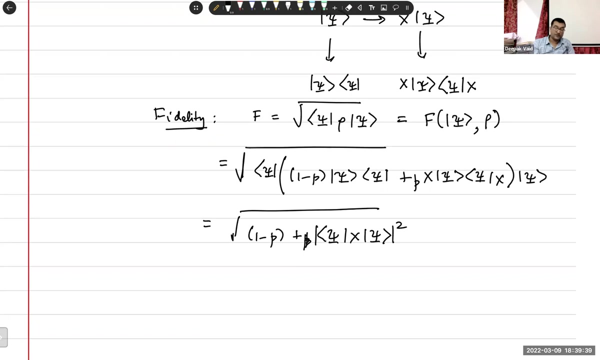 You get Psi x- expectation value Psi, and then Psi x expectation value of, so you get that twice. so that's why I'm writing that as whole squared, And there's a magnitude because there's an adjoint in there. okay, Now, both of these terms are positive, definite. so this fidelity, 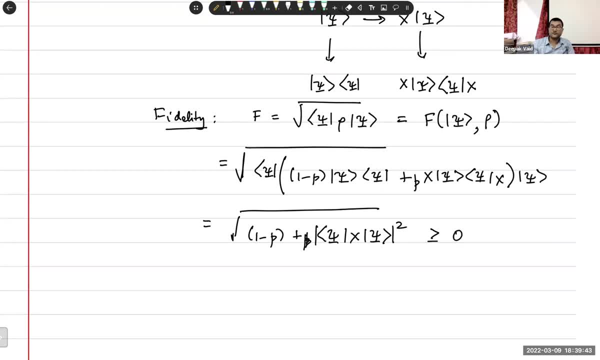 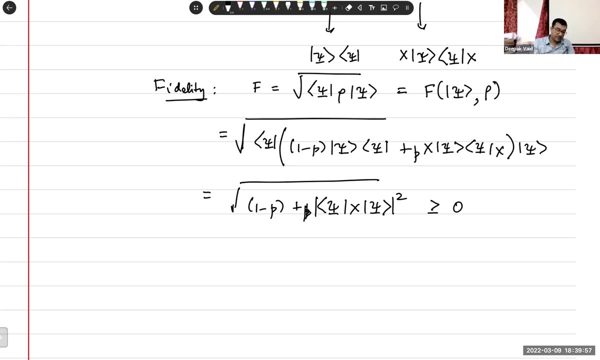 is always greater than or equal to zero right And the second term. so the second term is also non-negative. When is the second term zero? When Psi is equal to either zero or one, the second term goes to zero right. So now the second term is positive, definite, so that 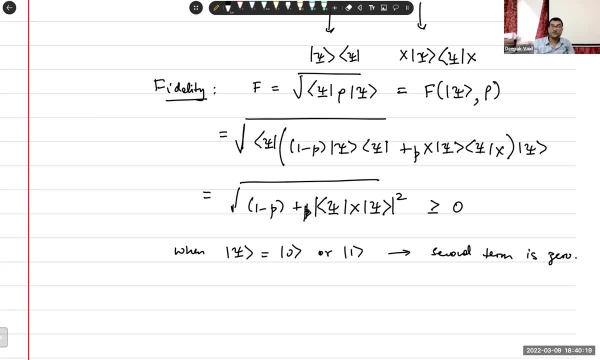 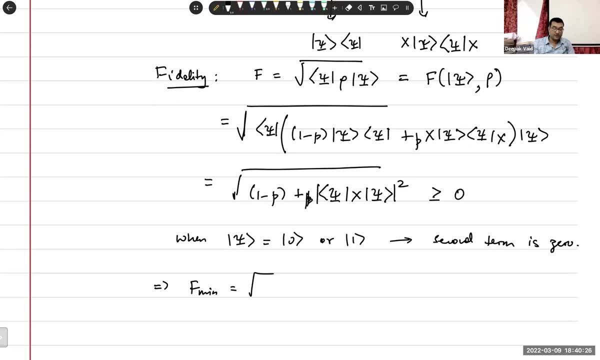 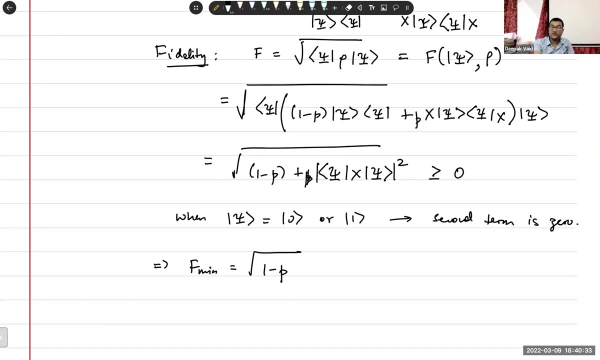 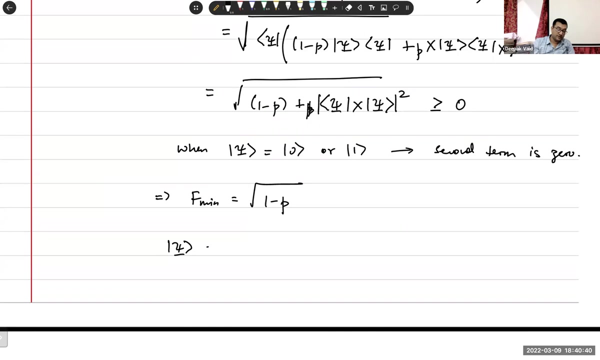 means the minimum value it can have is zero, right? So the minimum value of the fidelity is what It's a root of one minus P, right? This is the minimum value of the fidelity in this particular case. Now let's go back to that three qubit encoding alpha, zero, zero. 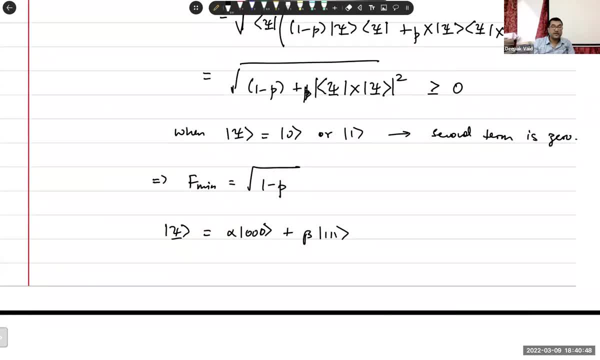 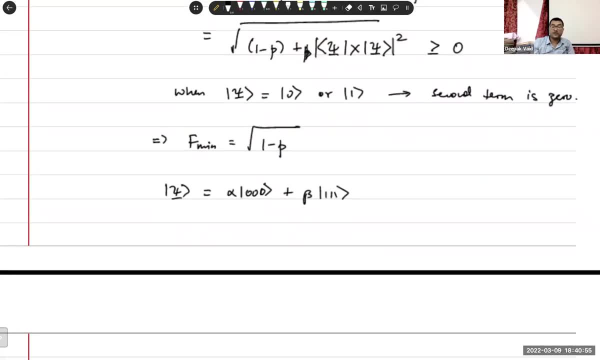 zero beta, one one, one where we did this probability analysis right, And what did our probability? what was the probability of having a bit flip on either one or less of the qubits It was? I'll write down the expression: it was: one minus P cube plus three P, one minus P squared. 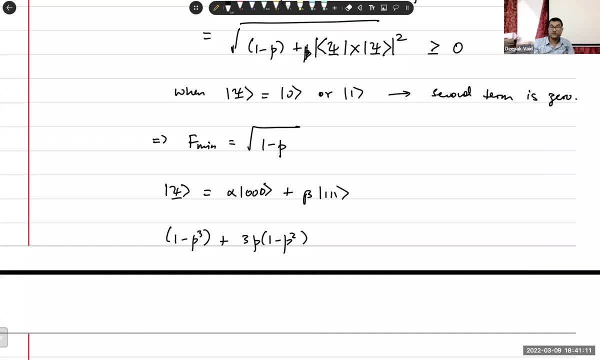 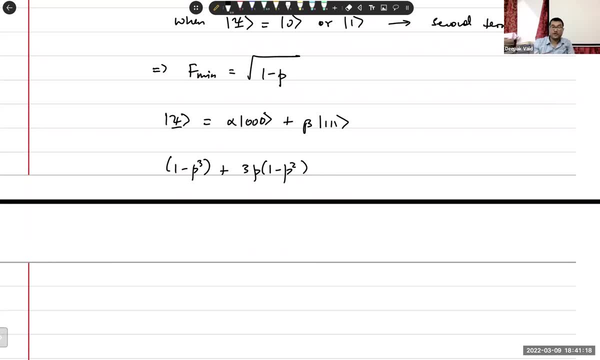 right, We derived this in the last lecture, I believe right. So we can write this in terms of rho. okay, We can translate this into an expression for the minimum value, And then we can calculate the minimum fidelity, The minimum fidelity.